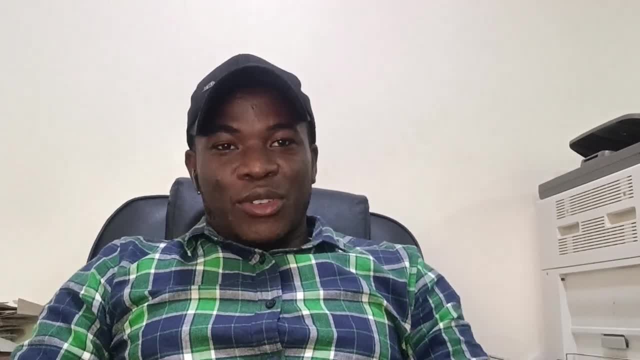 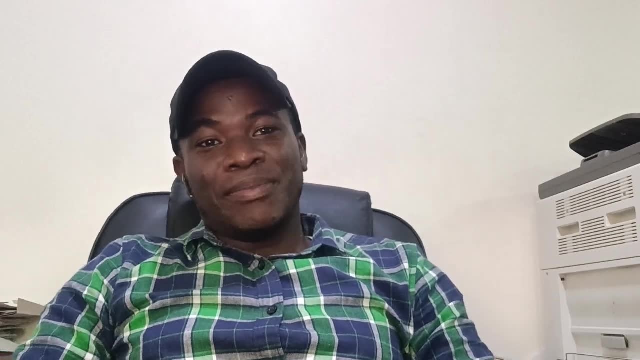 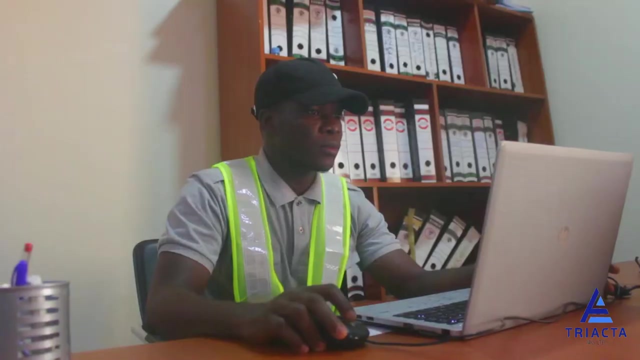 northeast of Nigeria. I've been designing highway infrastructures for over two years now. That is not small a time, because I've been part of the design of the first grid interchange in Yola, Adamawa State, And it comprises of flyovers, underpass and pedestrian. 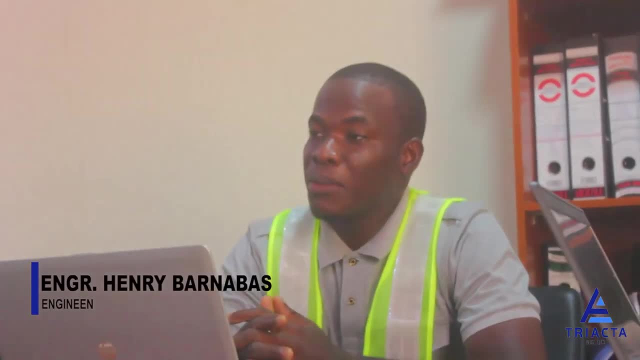 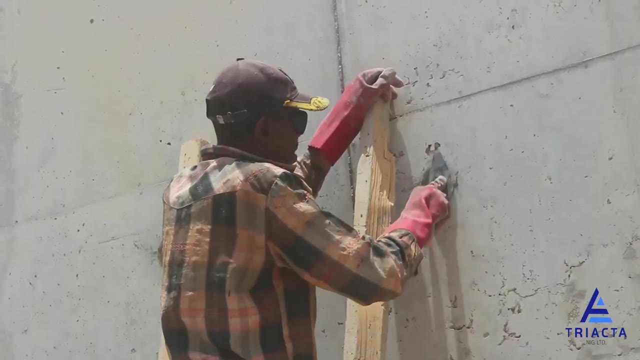 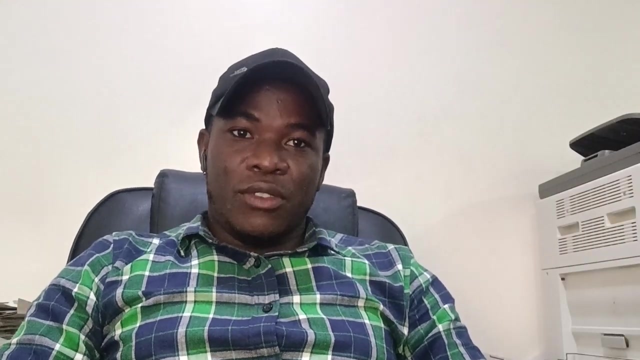 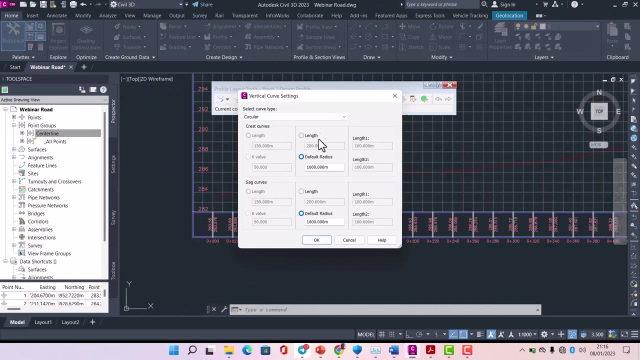 bridges. I designed the geometric, performed the geometric design, So I've also designed over nine roads, from start to finish. In this webinar, I've taken you through a comprehensive overview of the design of a highway using civil 3D. That is, starting from importing your points through to your design. 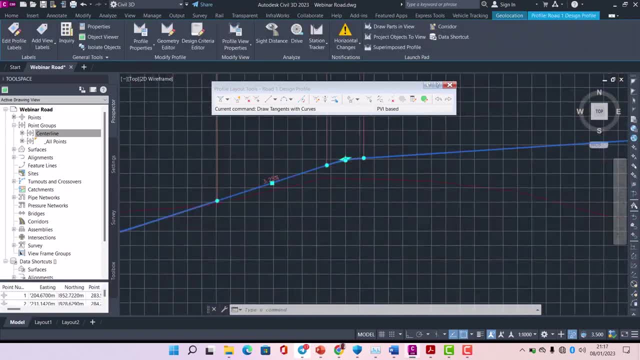 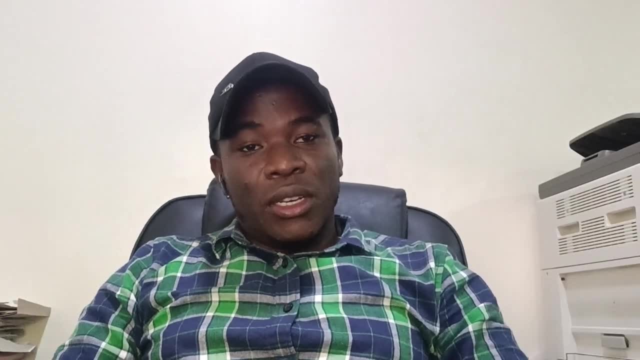 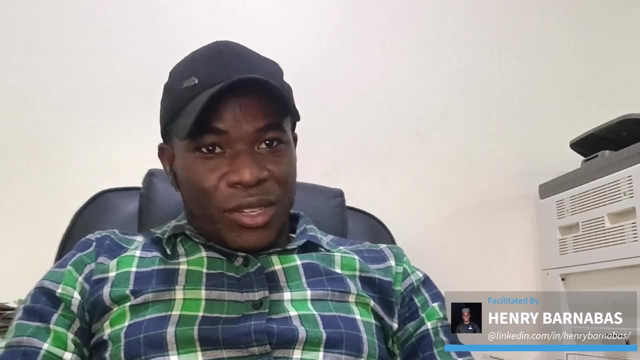 and then eventually extracting your design data for setting out on site. I've also shown you how to import your design codes that will automatically be checking your design while you are working. So, whether you are new to civil 3D or new to road design, or even both, this video is. 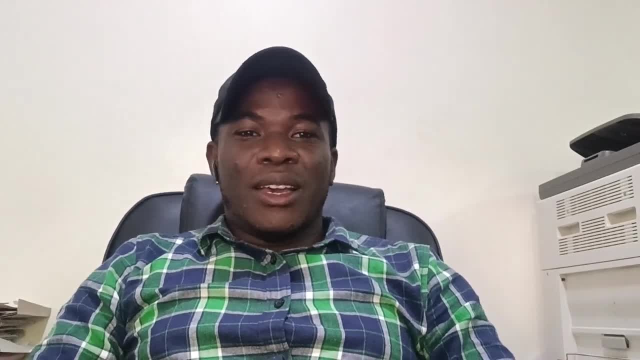 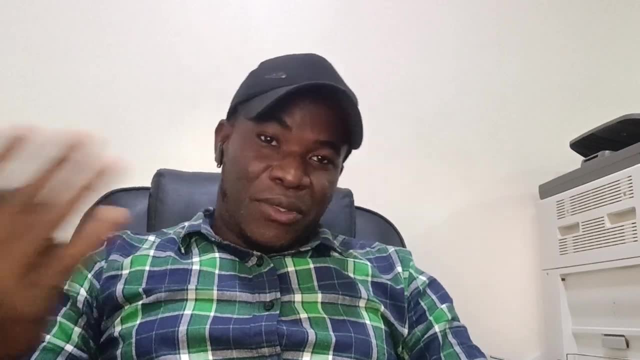 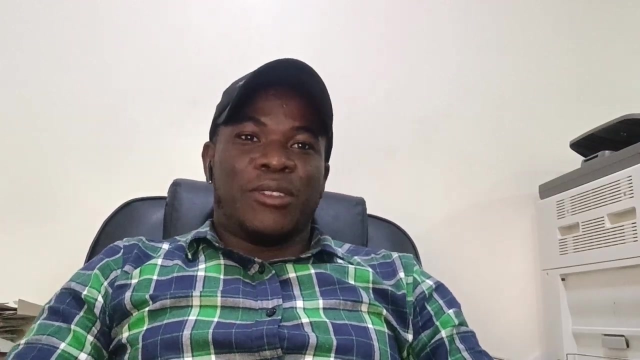 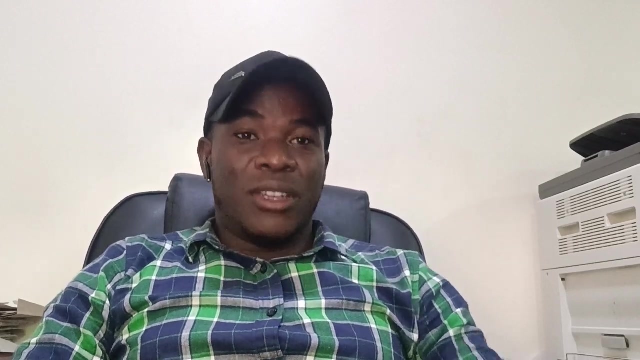 exactly what you need to move you from becoming a novice into becoming a very good highway design engineer And also, if, probably, you have already been designing. this video will help you learn some valuable insights from my experience, Because I've been designing, and I don't just design, I also supervise the designs during their construction and 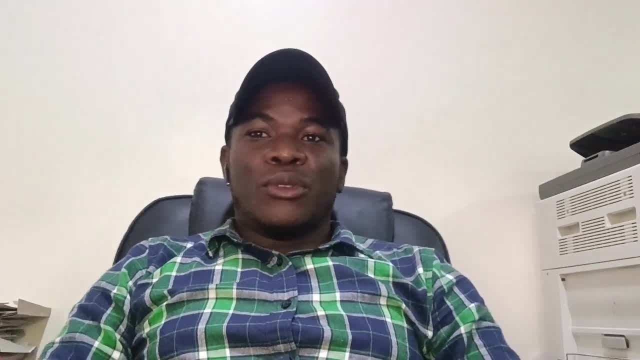 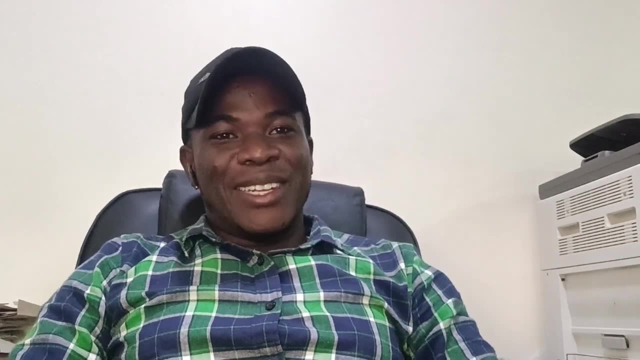 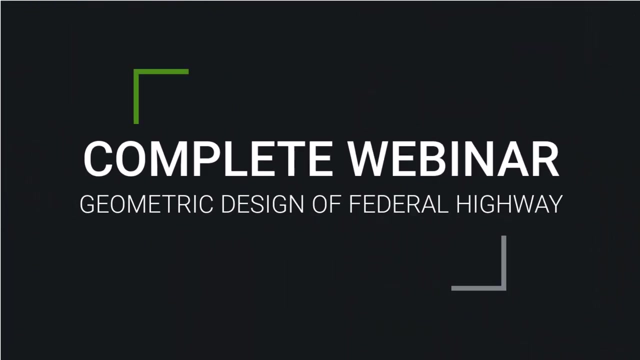 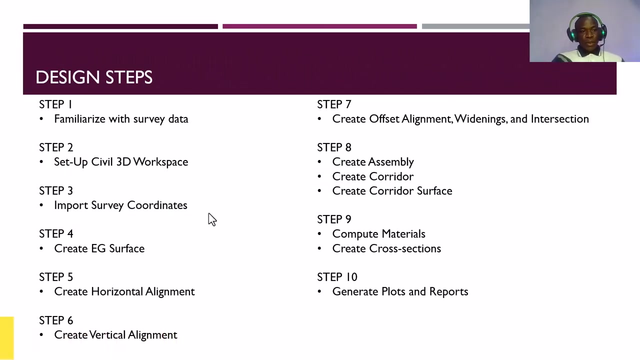 also perform revisions where necessary. So you will be learning from a hands-on, project based design. All right, Having said that, let's get into the video already. Okay, Okay, Okay, Okay. steps, sorry, okay, the design steps. first we are going to. the step one is familiarize ourselves. 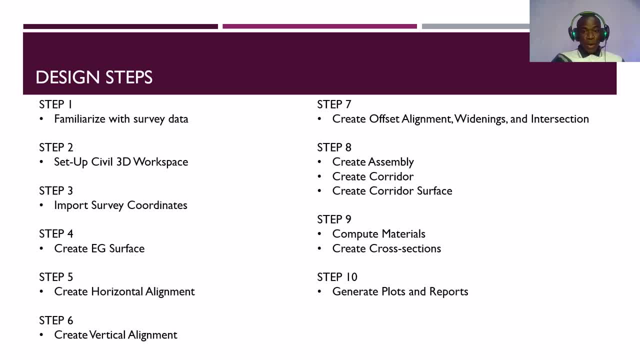 with the survey data. you have to know the survey data that you are working with very well so that you can accurately import them to civil 3d. then, secondly, we are going to be setting up the civil 3d workspace. then, thirdly, we are going to import these survey coordinates. fourth, we are going to 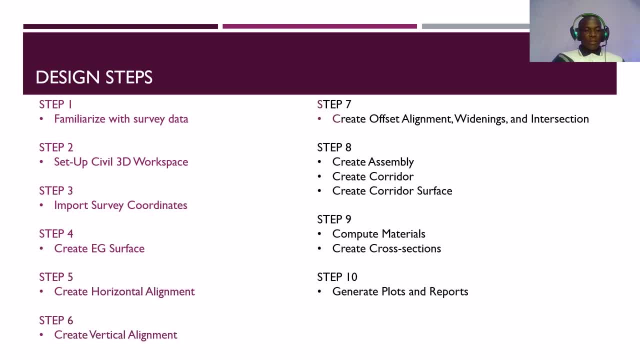 create an existing ground surface. then, fifth, we create the vertical, the horizontal alignment and then proceed to vertical alignment. seventh, we are going to create offset alignments and widenings and intersection. okay, then we, in step eight, we create assembly, create corridor and corridor surface. step nine, we are going to compute this, the materials that will require a cotton field. 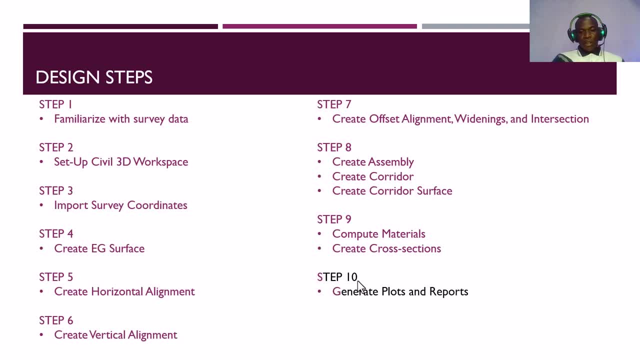 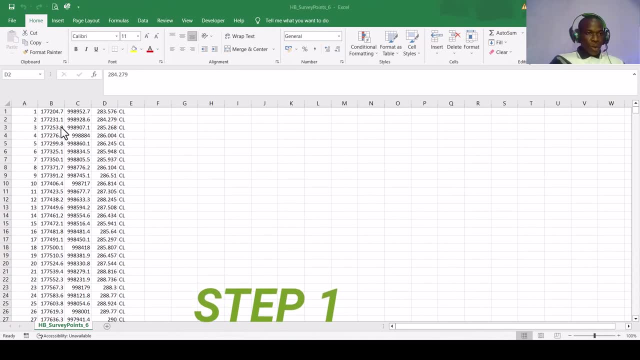 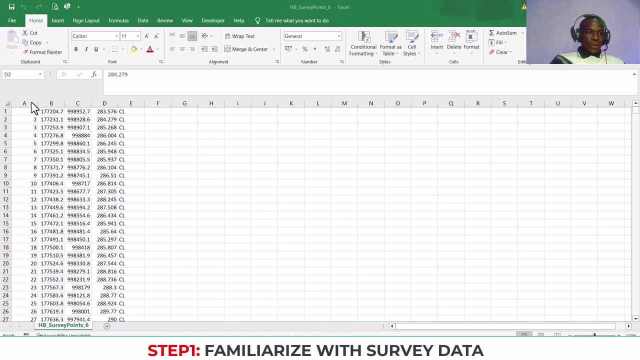 and then we'll create our cross sections. um then, step eight, we are going to generate plots and reports. all right, welcome back. so this is where we get ourselves familiar with our survey data. okay, so, based on the design steps. so, if you see, we have five columns here. this is column a. 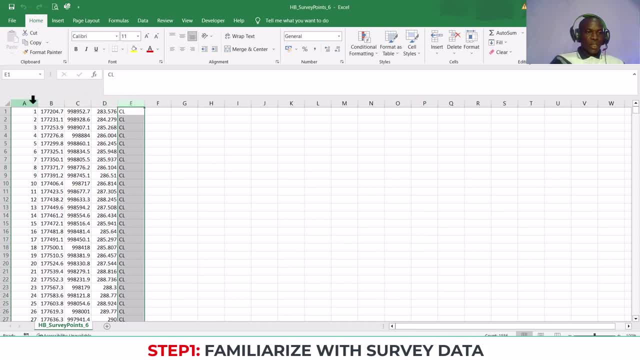 a, b, c, d, e. now these are the descriptions of the point, of the columns. this is the point numbers, or p, then this is the eastings, which is e, and then this is the northern n, and then this is the elevations z, and then this, uh, this is the. 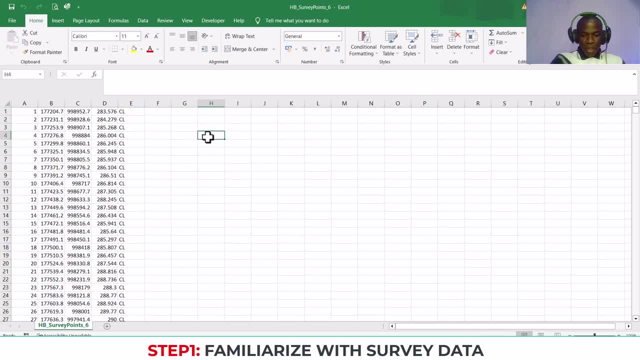 description d p e n z d. let me just write it here: p e n z d, sorry. d. this is the point code, you know? just yeah, i'm just saying this because you will see it shortly. when we go to civil 3d, you have to understand how your points are arranged. so it's arranged in this format here: p e n z d. 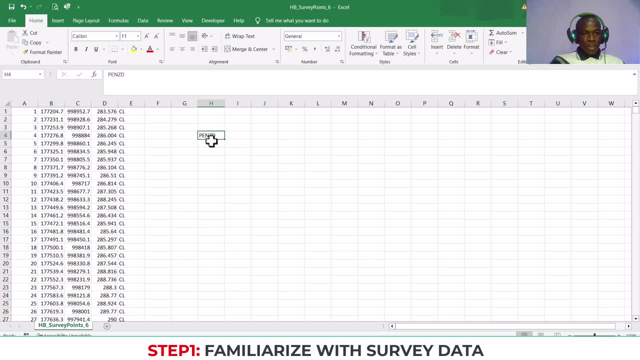 points, eastings, northings, z elevations and then d descriptions. so what are these descriptions? we have c? l here. c l means center line, so if you go down you'll see g, r and d, v, r and d is short for ground. okay, so, yep, as we go down, let me go down faster. oh wow, we have a lot of ground. 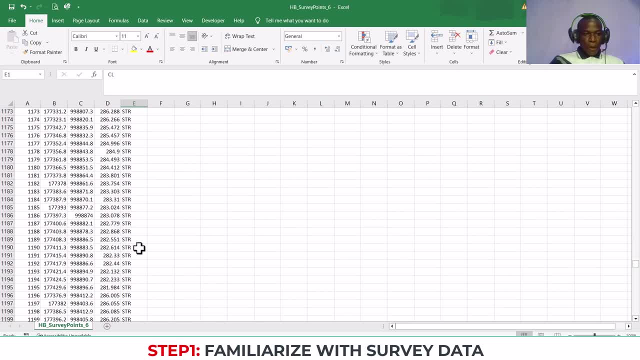 points here? yeah, of course we should. then s, t is string. okay, i know this because i'm not going to do this, because i took this away data with the surveyor, so all right. so then of course the surveyors will give you the descriptions. okay, they have to tell you what the point stands for. 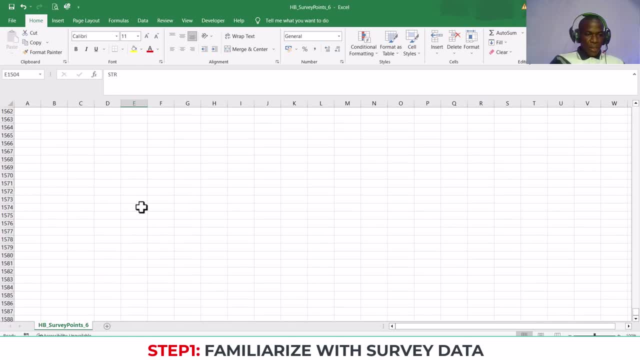 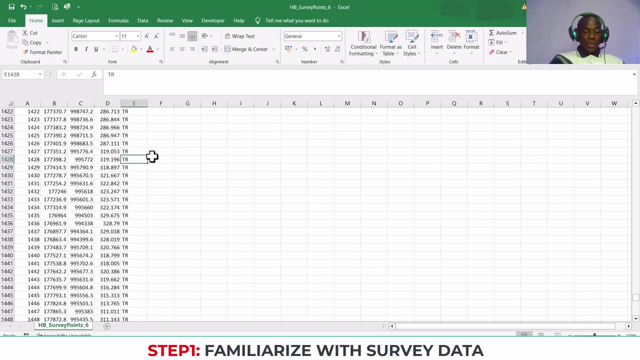 so that's. there should be full description, but for now we have this like this: so this is str stream, okay so, and then we have tr somewhere here. okay, yeah, three, we have three. i usually take the tree, the points for the tree, so that if i need to 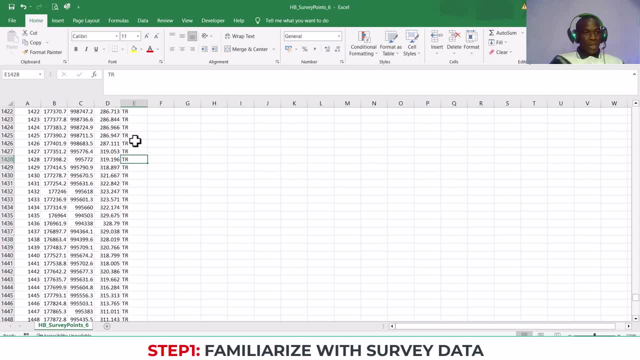 avoid some trees, avoid cutting down trees. i will do that, okay, because i'll see those, these points in my workspace, okay, which is important. i encourage you to always do that when you are designing, take the coordinates of the trees so that you can preserve these trees. we don't want global warming. 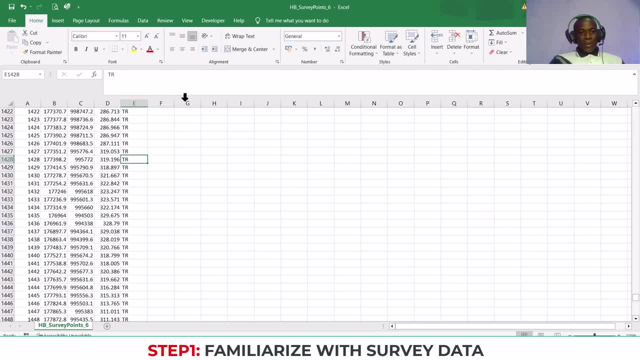 all right, that's on a lighter note, but very important, okay. so let's move on. so this is an excel file, but it will be saved as a csv file. there are two ways you can import your- uh, you know- drawings to your computer. so let's move on. so this is an excel file, but it will be saved as a csv file. there are two ways you can import your- uh, you know- drawings to 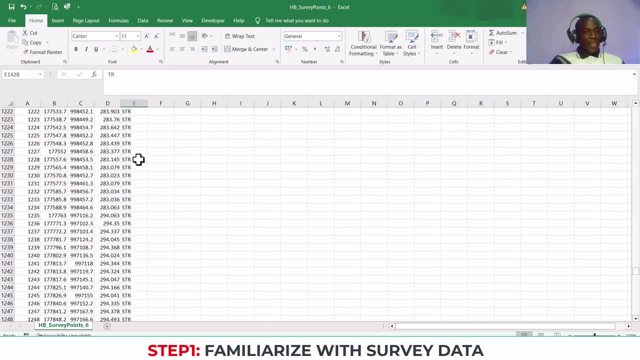 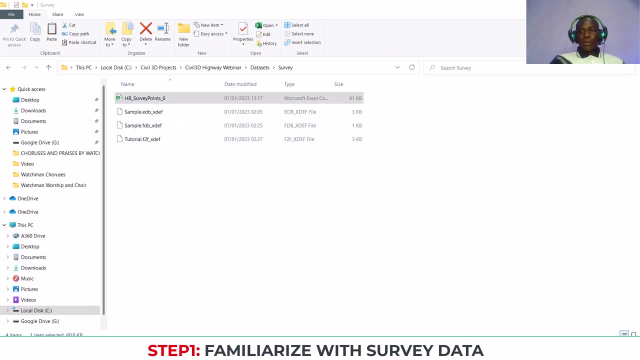 your points to save 3d. it's either going to be in text format or or a csv format. okay, so, but in this case i've saved it as csv uh points. so i'm not saved that. so this way i've saved it. okay, this is the name. so now let's go to uh, civil 3d already. so, okay. 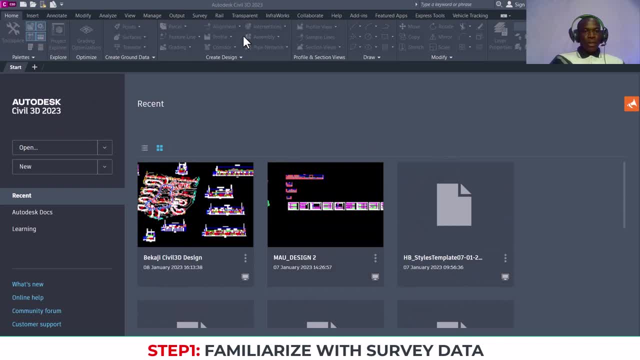 so here is my civil 3d. i've just opened it all right. so this is civil 3d 2023. so, like i've said, have said, I think, I said if I've not, I'm saying it now. so, whatever I'm doing with 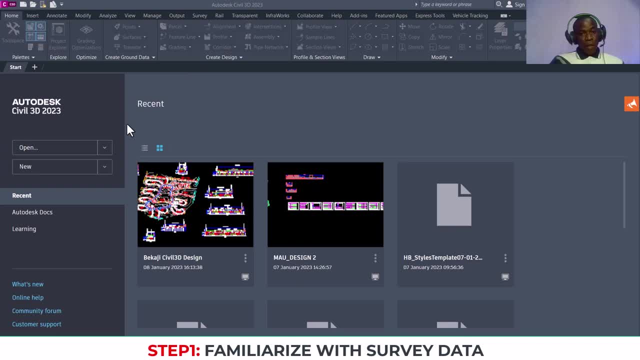 this into the 2023. it can be done with any lesser version, so you must not have symmetry 2023. of course, there are advanced tools out. you can do is simply 2023, but it's not related to what we are doing now. alright, so if you're having 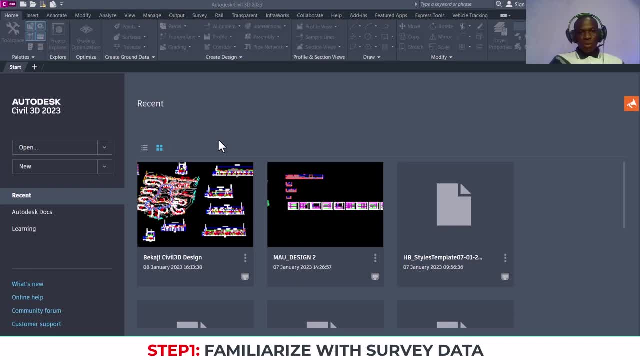 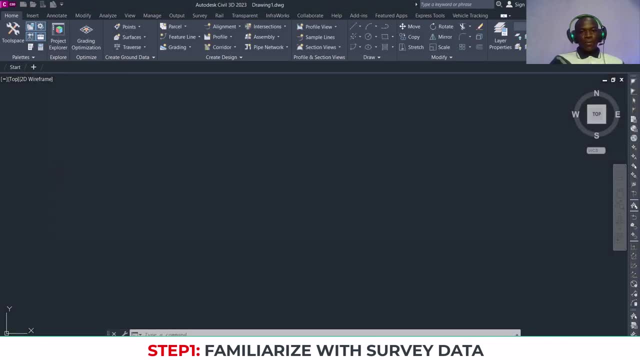 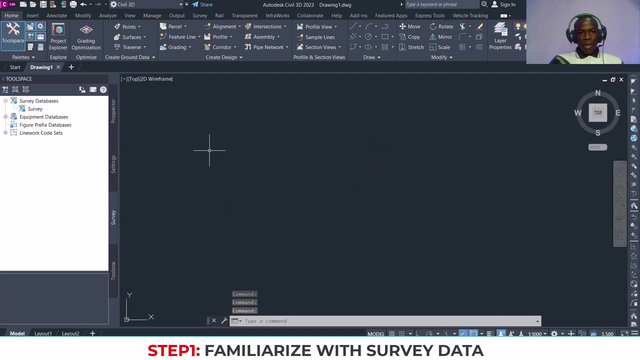 for 2015, you know, up to 2023, you can do everything that I'm going to do now. so what you do is you create your new file. okay, so we have this workspace here, this our civil 3d interface, our workspace, alright, so, yep, if you look. 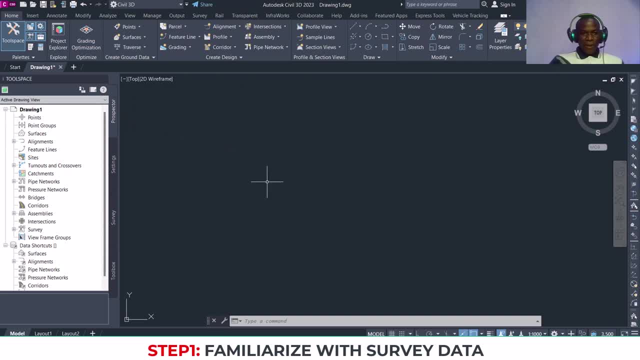 here is similar to AutoCAD, just normal AutoCAD, but of course it is having civil 3d capabilities. if I go switch to AutoCAD from here, if you just click on this drafting annotation, it becomes AutoCAD. yeah, that's it you. but once you switch to civil 3d it brings in all these complex ribbons. so 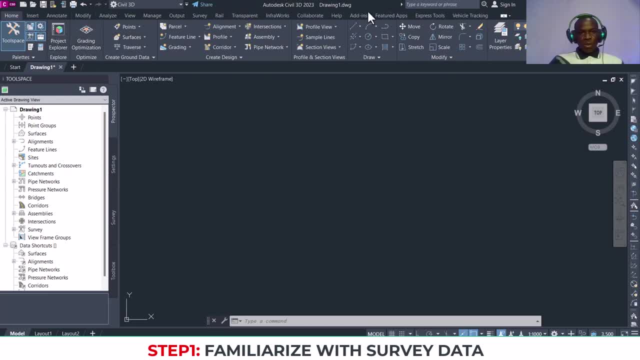 it's not complex too much like that. these are similar things if you have used AutoCAD, but you have, uh, you know, place to create alignment here which are which is not in AutoCAD. okay so, and then right here, by my left, you would see the tool space. okay, this is the tool space. it has four tabs, which is a prospector. 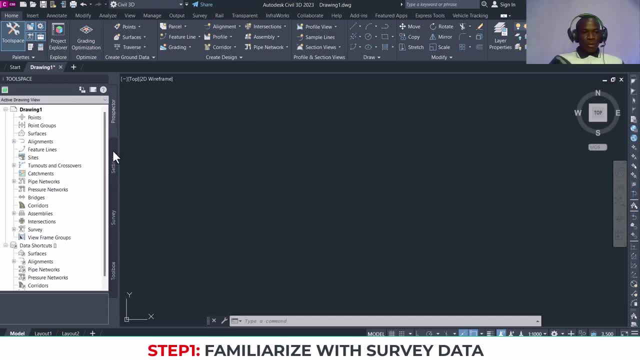 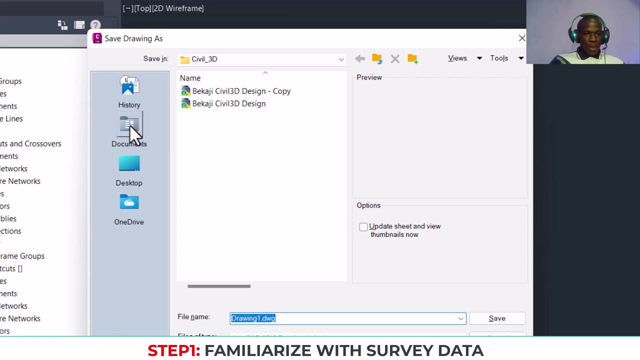 settings, survey and toolbox. so we're going to be using, uh, some of them in a while now, in the short while now. so now the first thing you're going to do is to set up your workspace. okay, first of all, let me save this drawing. I'm going to save this runner. I press ctrl x, ctrl s. okay, let me. 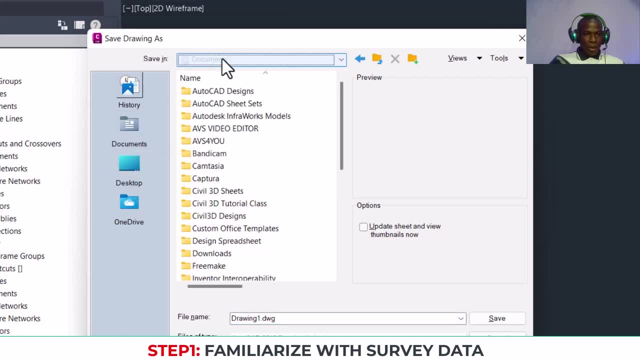 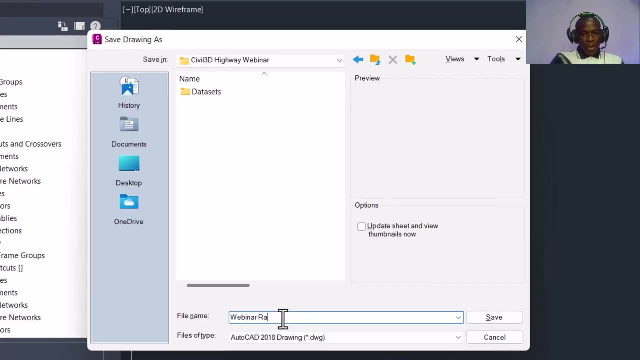 go to my desktop or or here. okay, let me find something to save that. okay, you know, look at the civil 3d projects in the 3d webinar. let me just save it here. let me call it where mode. so save it anywhere you can locate it. this way, I've saved mine, so I've 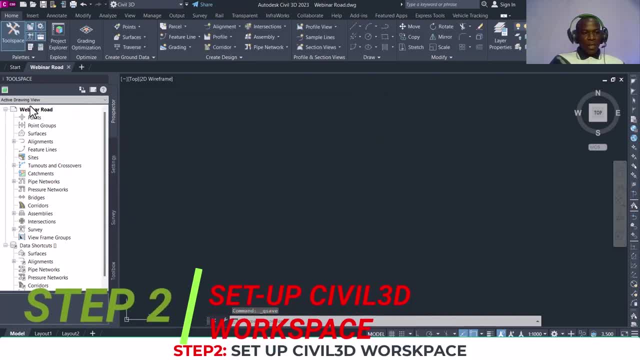 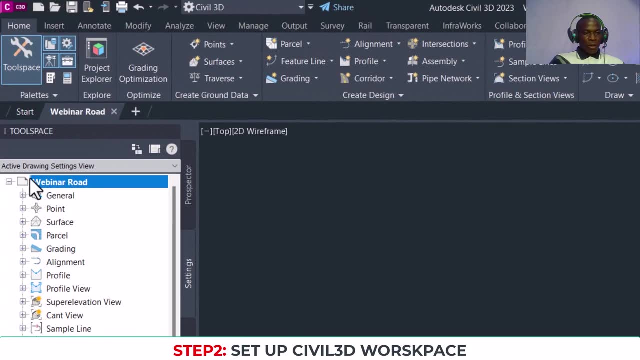 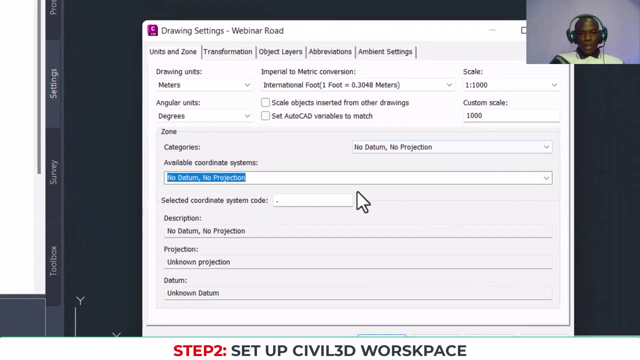 saved it so automatically. you see the name and civil populated in this perspective. so the first thing is to set up your drawing, go to settings and then go to the web on this webinar or the name, you right-click and do edit drawing settings so it brings up this wizard or dialog box. alright, so you will see. 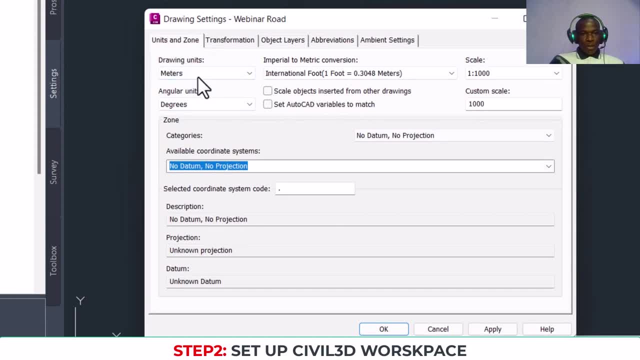 under the unit and zones, you'll find a drawing. you need to be meters. okay, so we are working in meters, because I'm in Nigeria, we use metric. okay, I'm, by the way, this civil treaty is civil to the metric. okay, so we have similar to the. 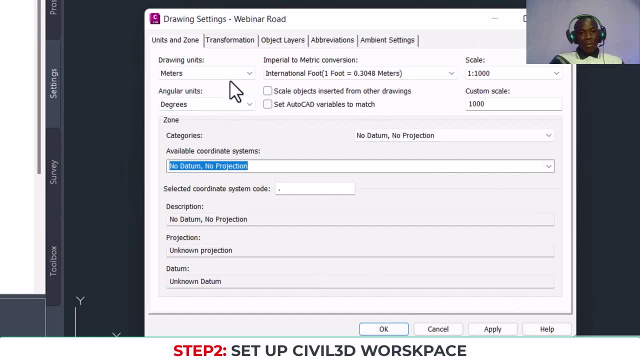 Imperial. if you install civil treaty, it stores automatically metric and Imperial. so, but I'm using metric because we use metric system here. if you're in the US, you are going to be using imperial, of course. so this is: is the meters? okay, everything here is meters. so if I have any foods- okay, if I have foods. 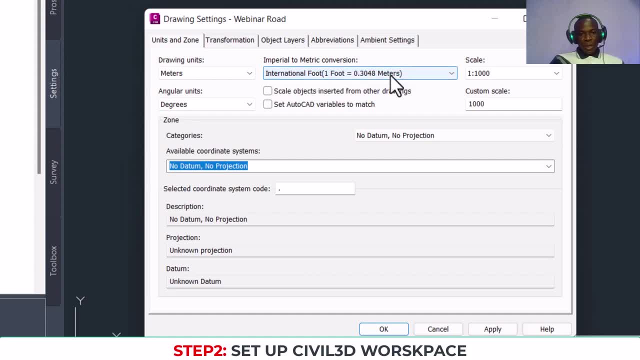 sorry, Imperial unit which is in food, it will convert it to meters. for me, using this conversion rates, which is 0.3, you know for whatever, for meter for food, sorry. so this is the default scale so you can change it. but no need, all these things can be left default by default. all this is so, my angles and degrees, all 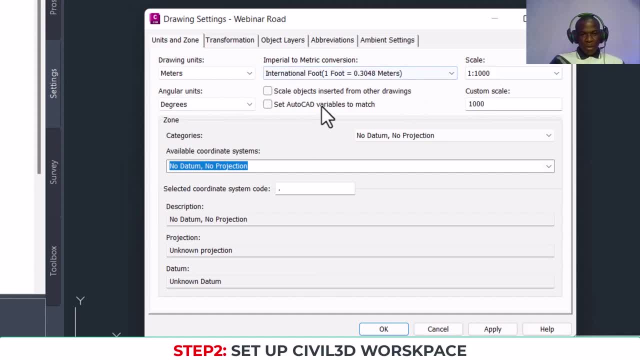 this and gives you on default what you need, so you may not have to change it. I won't be making any change here. where I want to making change is in the zooms. okay, under the zooms you have your data. you have to select a data, so where are? 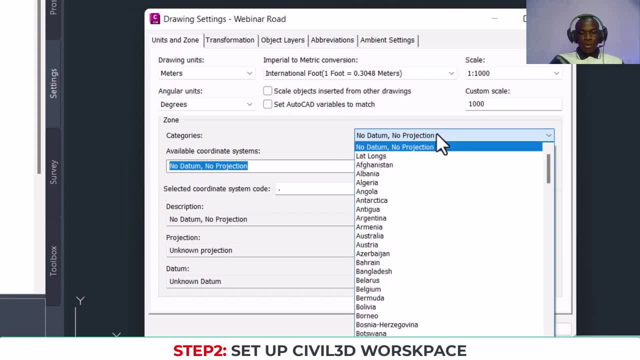 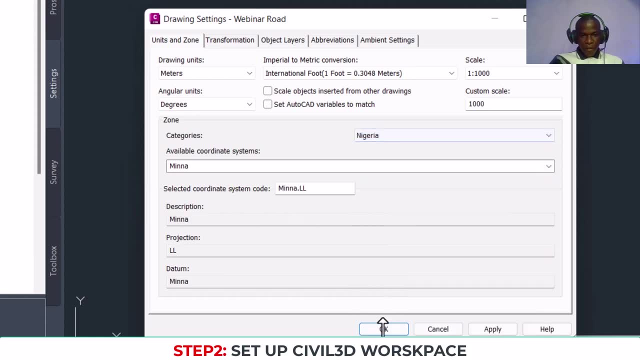 you working at. you have to select the country where you're working at. I'm in Nigeria, so I'll scroll down to Nigeria. I can just press n to snap quickly to where n is. so I've found Nigeria right. so then, on the coordinate system we have 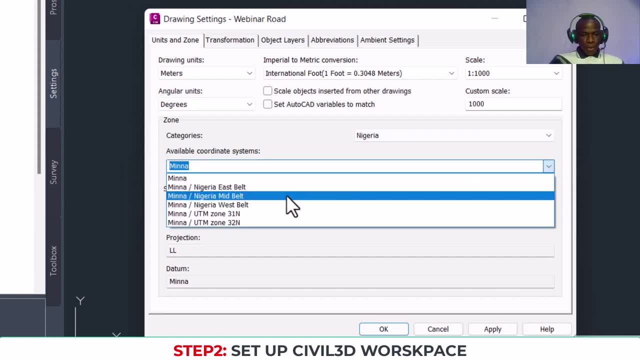 about six of them on this drop down menu. in this drop down you can see. but we work with Amazon 31 in. okay, there's a reason for that. it's just what we usually work with in Nigeria here. so once you do that, every other thing here is populated, so you. 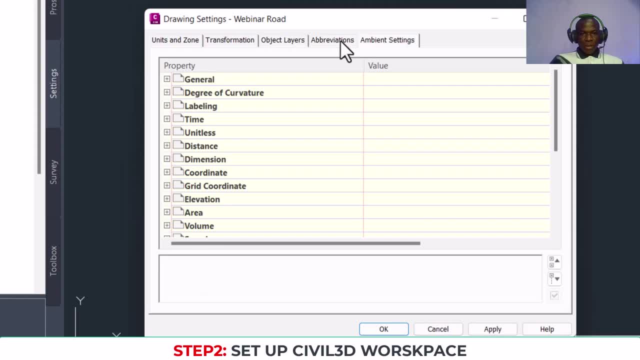 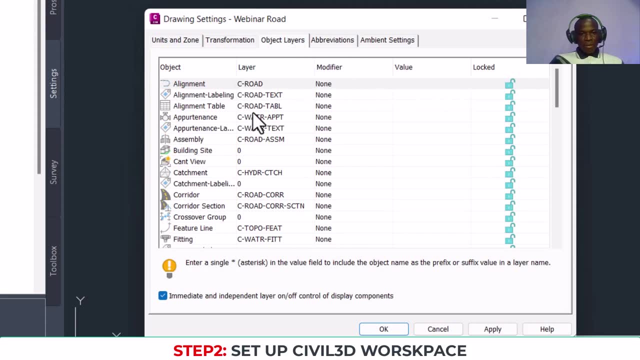 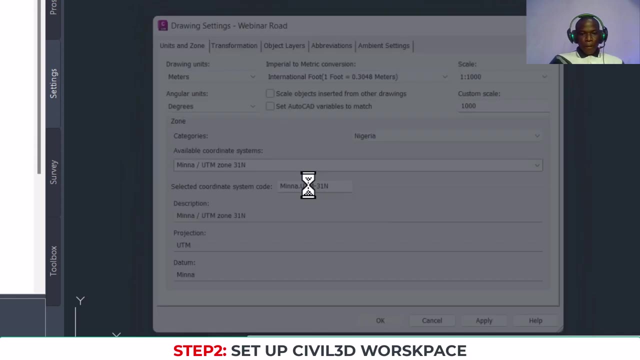 leave it now. I'm not going to go into these other tabs, because there are things you can set. when you have been frequently working with civil 3D, you might find the need to come here and set some things before going into the design, so you can set the layer whatever here. so let's just go, let's apply and then 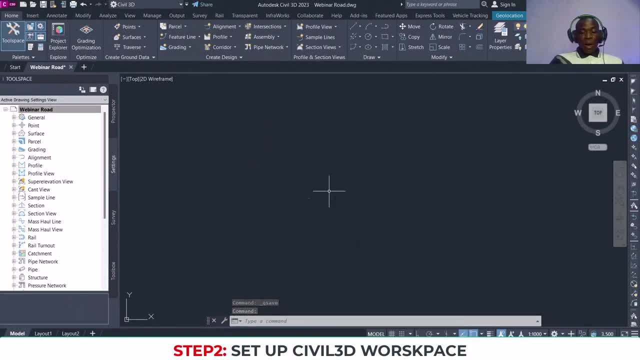 okay, so we have set drawing to our coordinate system and once you do that, automatically you will see that this geolocation over here appears. it won't appear if you have not done this. okay, it allows you to also, you know, on this geolocation you can open your maps and things like that. but I'm not going on to 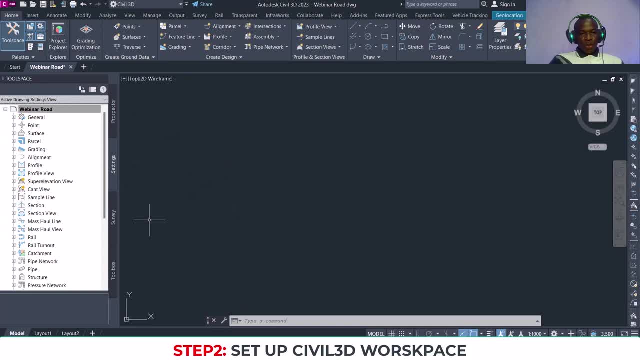 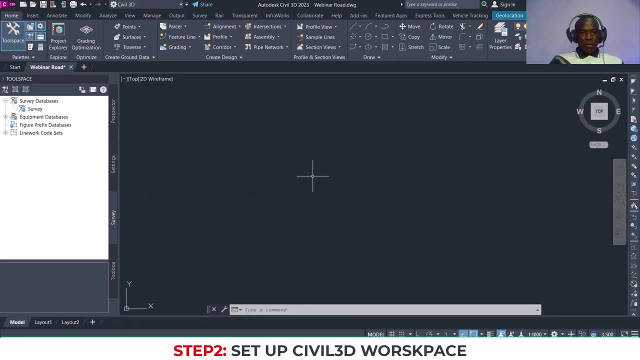 you all of that. all right, so let's go to import our survey points. all right, so you can import your survey points in two different ways. okay, you can import it number one, as a cogo point, that is, coordinate geometry point, or as a survey points. now a quick difference between survey coordinate. 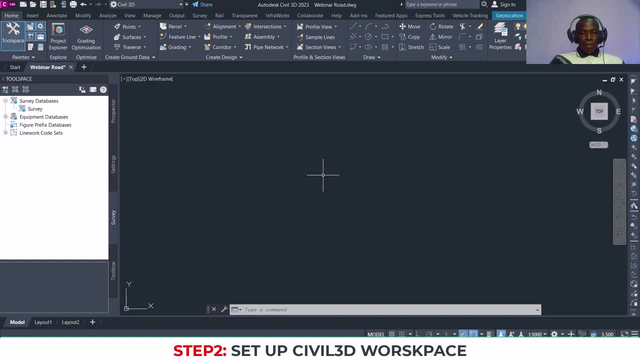 points, coordinate cogo points are in cogo points. you cannot. you can easily move the points around in the workspace, but when you import it as survey points, you cannot move it. you cannot move it because until you use specialized commands now again in cogo points, it is local to your own file or your own laptop. but when you are 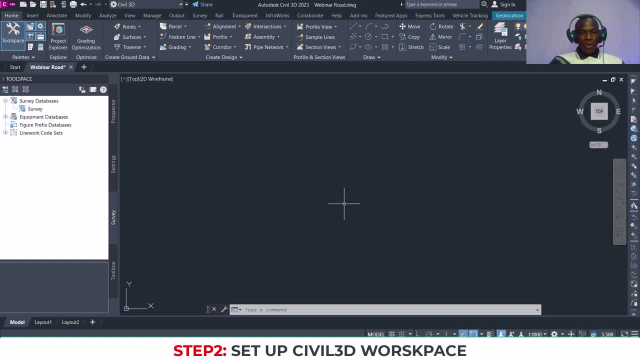 using you import it as survey points, you have the opportunity to collaborate with another person using working on the drawing, because you can be able to save the points in such a way that in a cloud system where another person can work with it. okay, right, so that's just a quick little difference between survey points and cogo points. 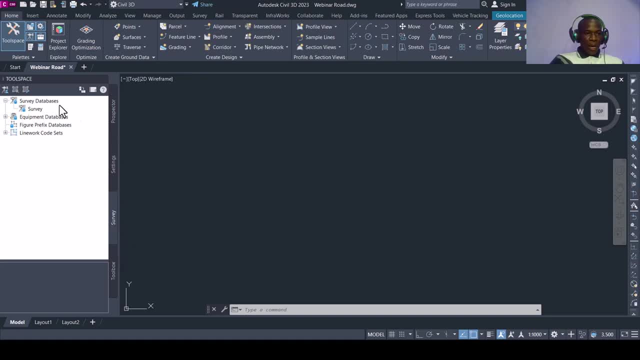 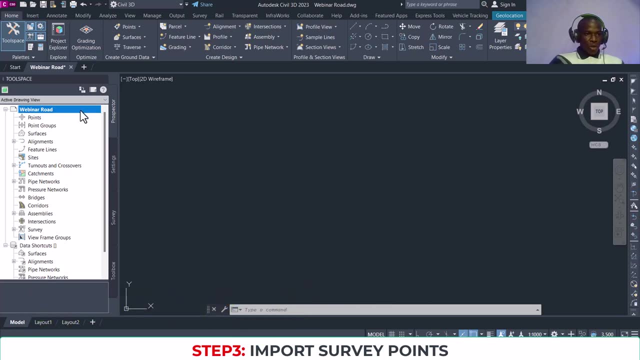 so now under this survey points we have. okay, let me just import it as cogo points, all right, because going through survey points is quite tedious and I don't want to take too much time here, so let's go to the prospector tab. we have the points, all right under these points, you right? 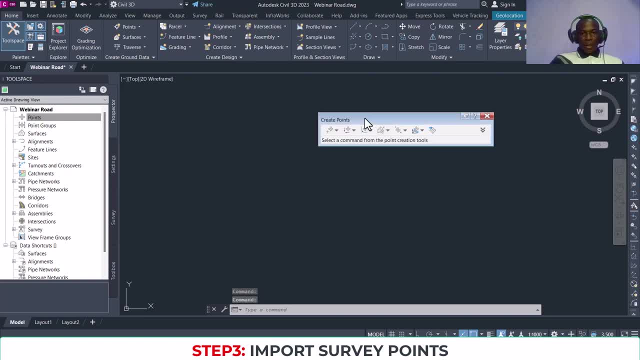 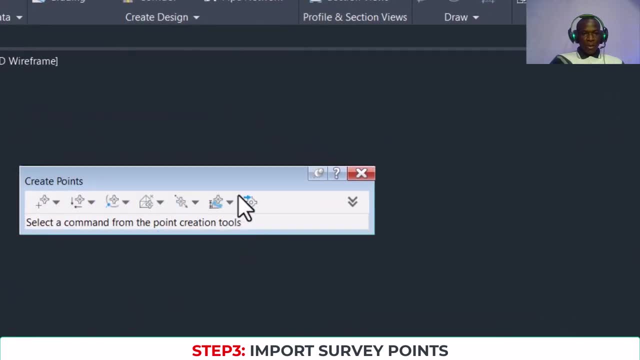 click on it and then create okay. it brings up this ribbon for you. you have all these styles from about six of them: one, two, three, four, five, six, seven. so the last one, okay, is what you're going to take. if you hover your mouse, are over it, you will see it say import. 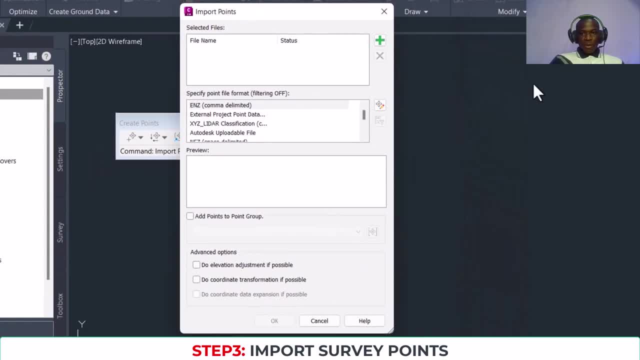 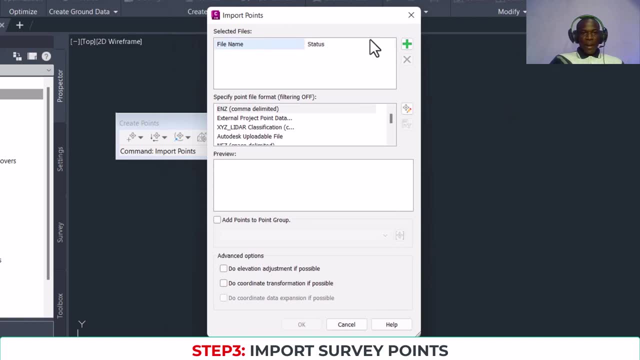 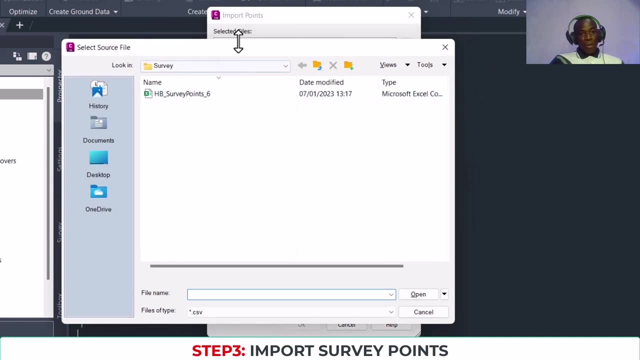 points. so you import points, all right. so if you look at this- sorry, okay, if you look at this- you have to select the file where the point is located at. so it takes me straight to where my pointer. but this will not happen if you have not previously maybe worked on that folder. so you have to you. 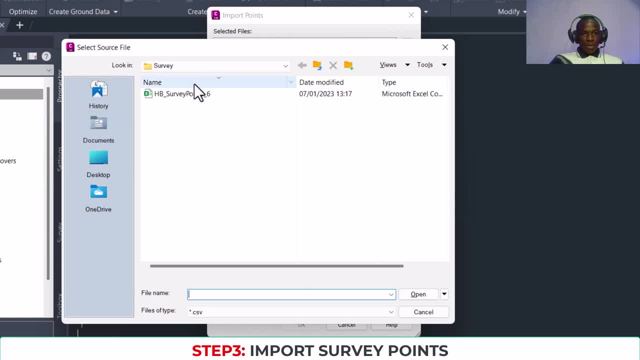 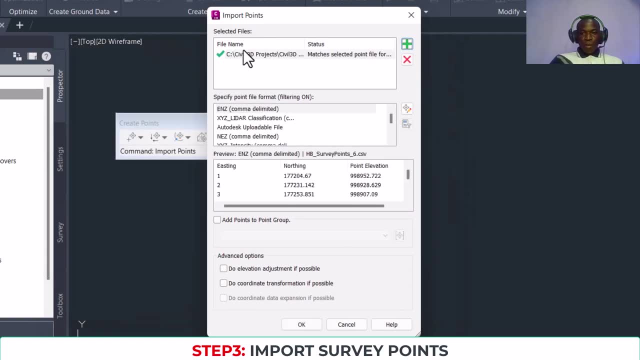 know, use this uh things here, you know, to navigate to where the folder is. so this is my points directly. so I open it. okay, if the points, if if it was set up correctly, it will show you a check. okay, but if there's an error with your, the way you saved your file, it will, it will not be able to play. so remember I. 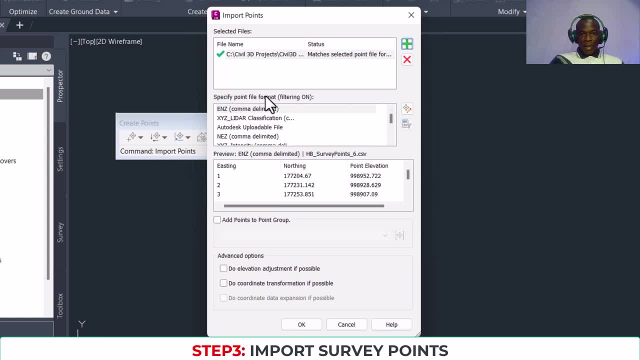 said, the points are you have to put the point formats. now you have to select the point format. it's p, e, n, z, d, so let's look for that here. very good, so look at it and it's comma delimited. okay, you would have another format which is maybe. 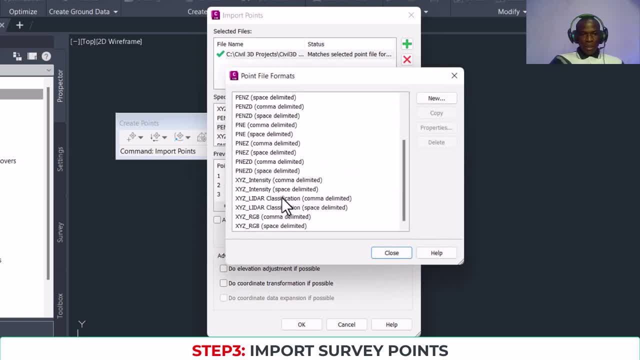 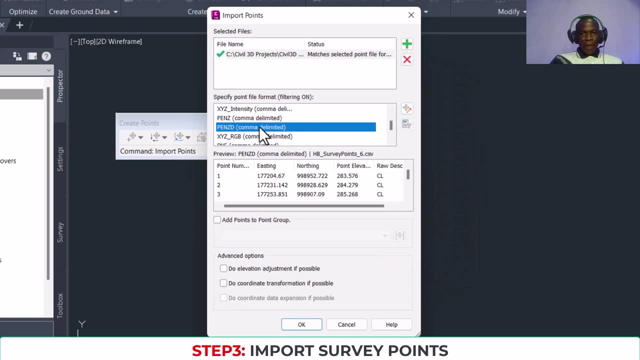 not comma delimited. if you open here you will see a lot of other formats. okay, you have space delimited and comma delimited, but we are using comma delimited because it's csv file, comma separated value. that's what csv means. so if you just click on that, you will see. it will preview. 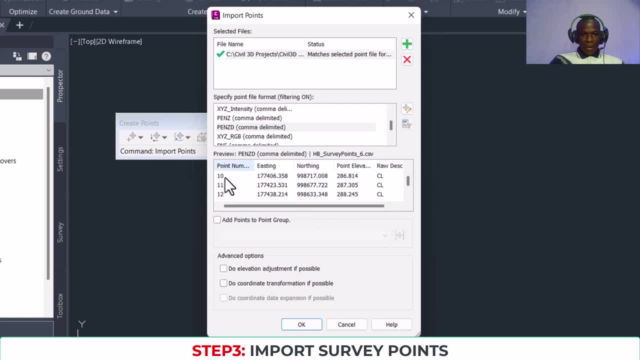 those points that we saw on the Excel. look at them. so once you have done that, yeah, you go straight. leave all these other ones unchecked. okay, all right, because there are some points where you need to add them straight to a group, but we're not doing that now, let's just add them directly. so we just press okay. 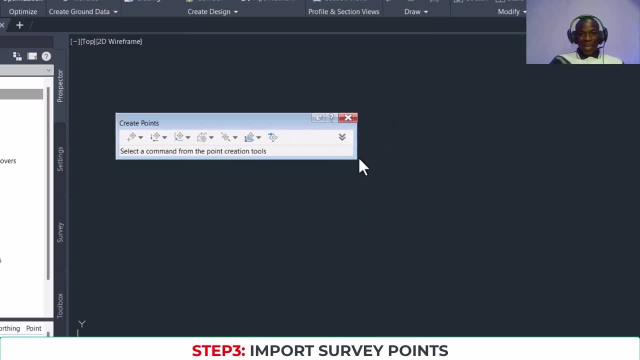 okay. so once you have done that, the point is somewhere in your drawing. you can close and then press enter. so what happen is you more, you know, like I said, almost 3 Phase, which is why, if you want to go back in the преступ sleeve, you have rarely never do org it. once you it's. 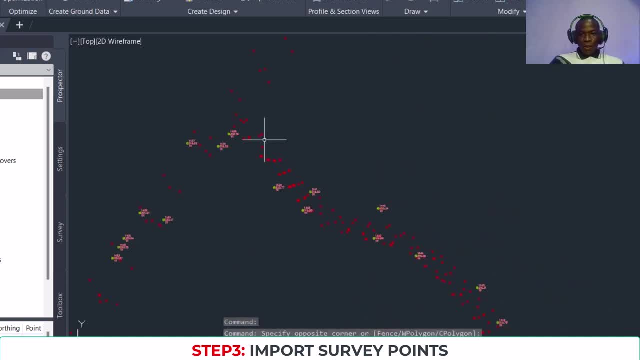 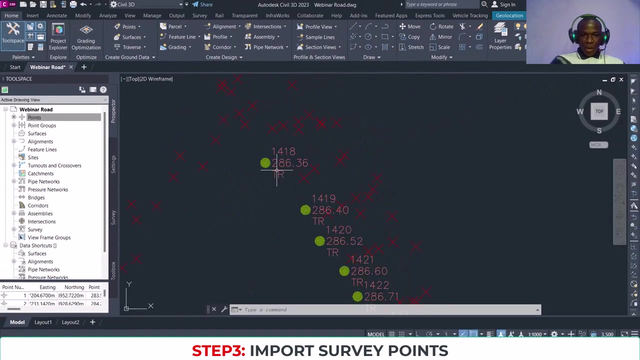 only when you- it's only a little bit. first, if you enter, it'll be. you press enter, it'll be. zoom right to where you are. you click zoom to see to three points. okay, look at the points. yeah, right now you don't see what, which, which point. the descriptions of the points. okay, you can you. 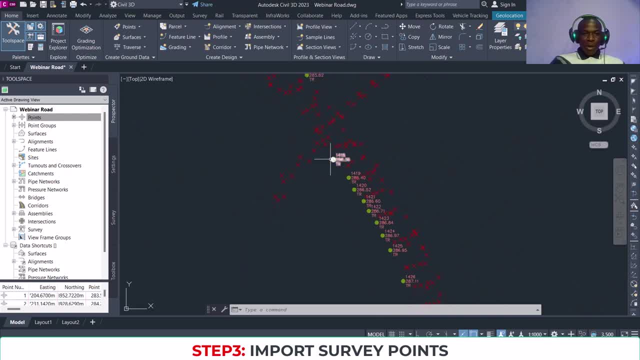 can add the descriptions of the points. it's already three points. right here you can see the descriptions- that's because of what we call the screenshots here- and then the points you use- the key sets. under the settings. you'll find something on the points description key sets. okay, this way you find, but I'm not going to that. all right, let's just go. 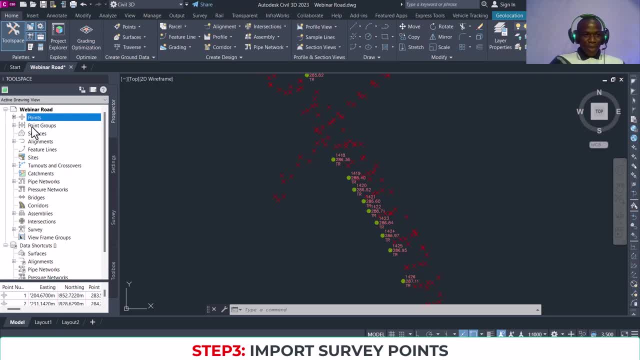 let's just go on. I don't to complicate this thing, please. let's just be simple, alright, so let's have our points groups. you see all points. well, when you expand it, you see all point. these are all these points. they are all grouped into this. 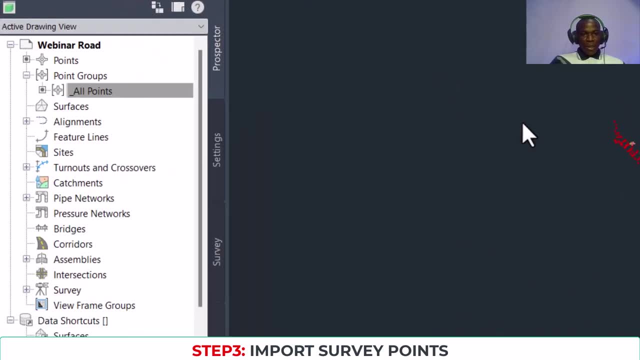 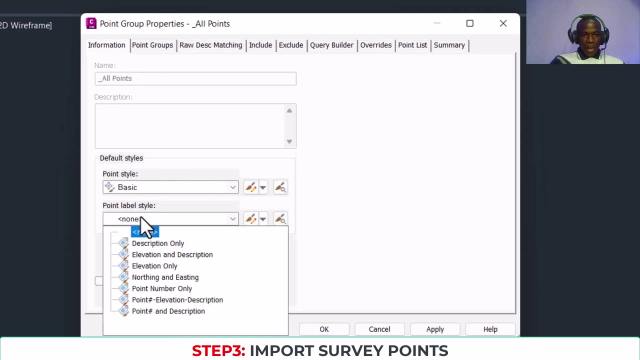 all points. so if you right click on it and go to properties, you would see the under information tab. you see the point style, okay, and then you have the point label. so for now you don't have any data. that's why it was not labeled. so if you 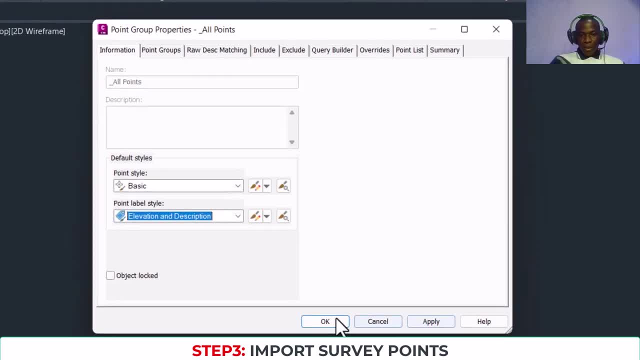 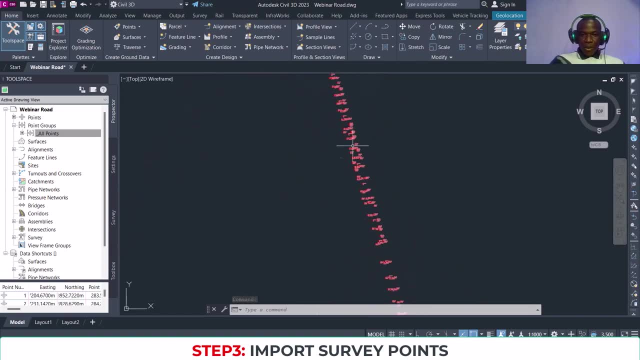 choose, let's say, elevation and description, and then press ok. ok, you see that it automatically populates. you know the descriptions of these points, so you can see all these points and see what they mean. these are stringed. these points are. this point is called stream. you know why I took these points. 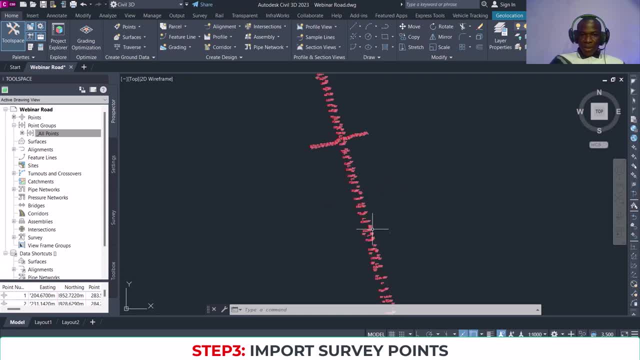 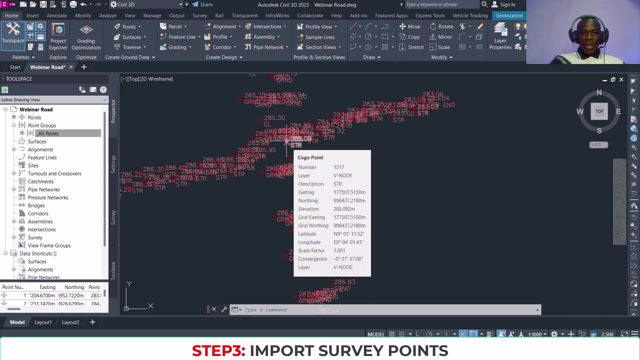 is because you know in the roadway, you know sometimes water is passing across the road. okay, all right if it's an existing road. so you have to take those points so that I can see the elevation, see the direction. okay, so that I can place my bus culverts accurately, all right, sometimes you have your bus. 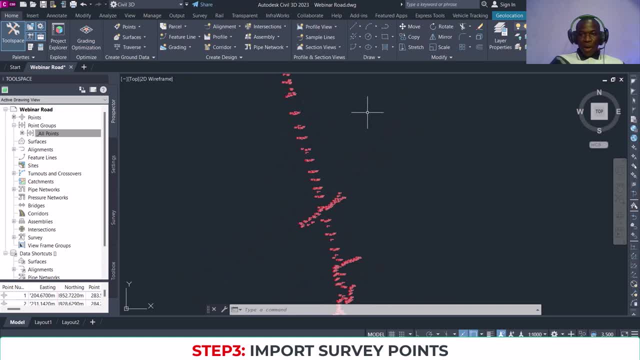 culverts will be skewed, that is, it's not going to be perpendicular to the route. okay, it can be skewed. for instance, in this place, I'm sure I want to have a skewed bus culvert, okay. so that is. that is the reason why I have taken the stream. 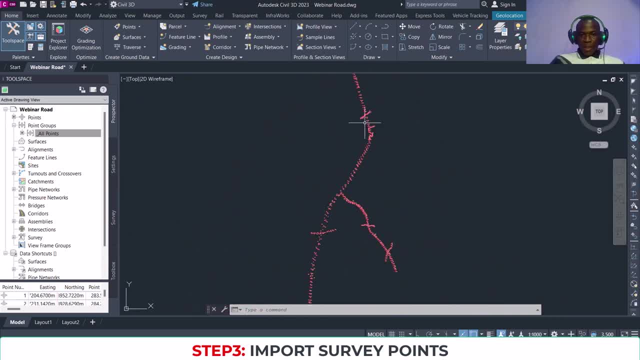 points. all right, so yeah, so that's a much about the. you know the points. so if you see the points, the the description are overlapping. okay, that's because of the skin. if you reduce the skin somewhere here to, let's say, 1 is 200, you. 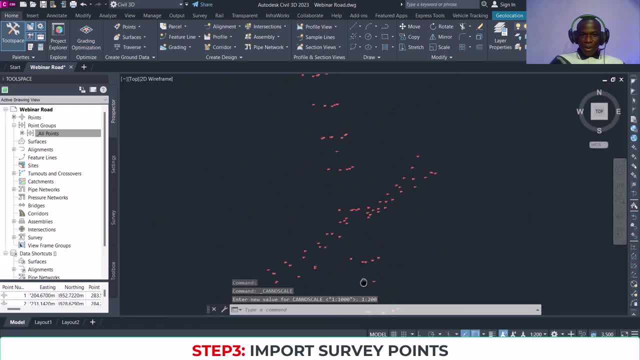 see that this points: yeah, it's, it's not overlapping, it's not so big like that again, so let's go back to one to one thousand. so yeah, that is it for this. so let's now go to the second, the next step, okay, which is to create surface now. before we go to that now, I 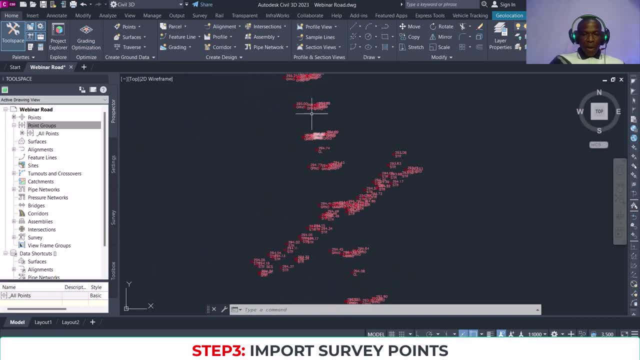 have remember, I have center line points. okay, I want to work with the center lines. these are the existing center line, the existing centerline, of course, as you know, as you may know, this an exit, this an existing roadway that has not been designed. so you know, you take the. 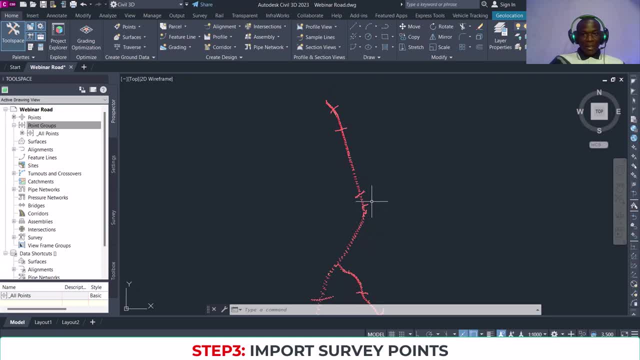 proposed centerline. okay, the existing centerline, which is you try to, you know, follow the existing centerline, of course, when you are designing, right. so I have to group all these points in the centerline. as you can see, it's here, so we here, and then there is another one here. so if I say, let me be checking it, 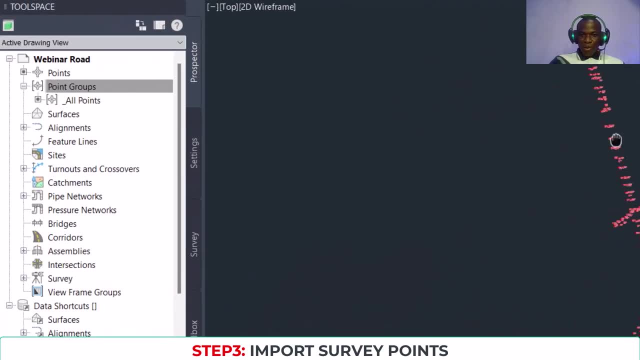 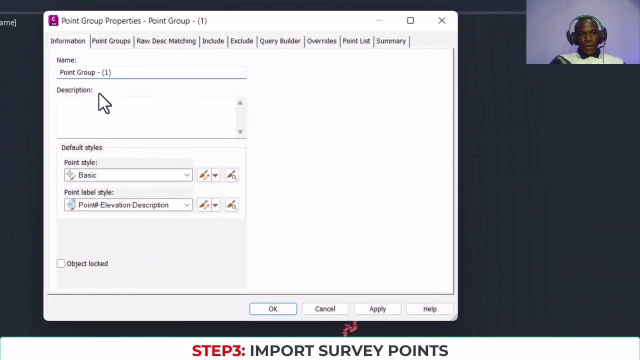 checking them. I would have issues because I'll not be fast enough. so let me create a group for all the centerline points. so I'll right click on point groups and go to new. so on the names, I'll call it centerline, okay, so when you 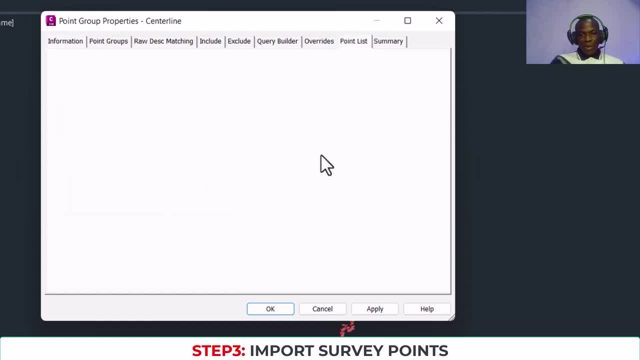 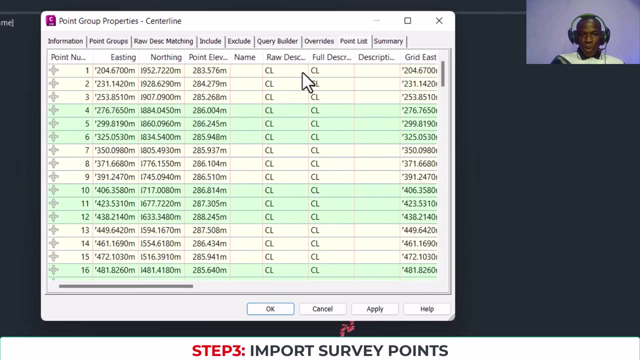 go to the point list. you don't see any points here. that's not that, because nothing has been added yet. so let me add it using all the points with raw description ending with C. I put aesthetics. okay, once you do that, you go to point list. you see, in that it. 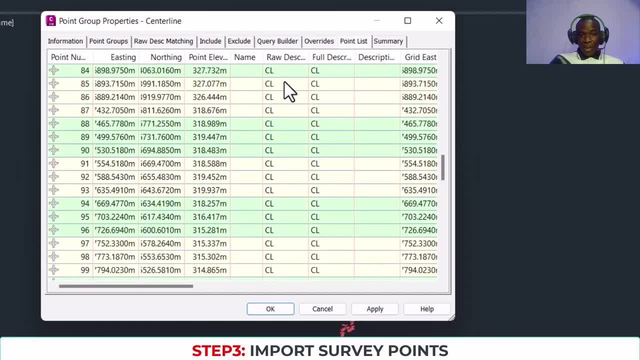 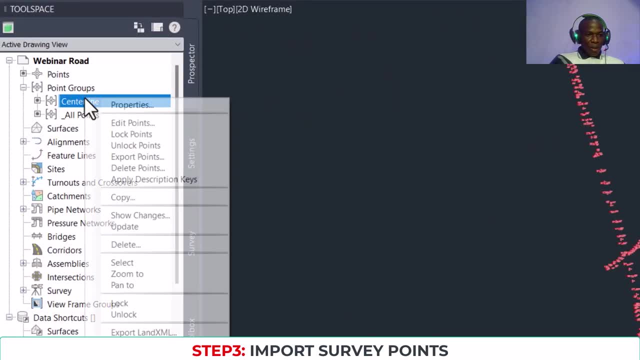 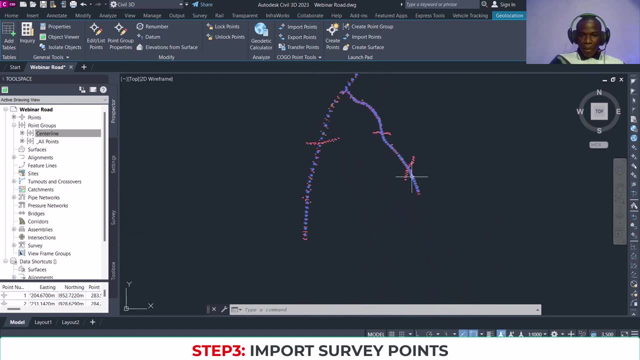 takes only all the points that have. see them okay. so once you do that, you apply and then press ok. so you see that point group here. so click on that right click on it and you select. you see it have selected all my centerline points, highlighted all of them, and let me do something. I submit if I type isolate on 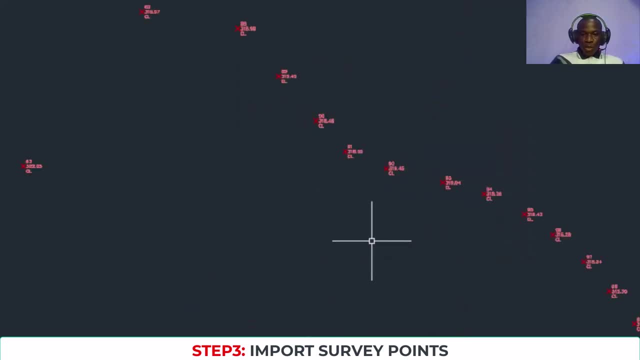 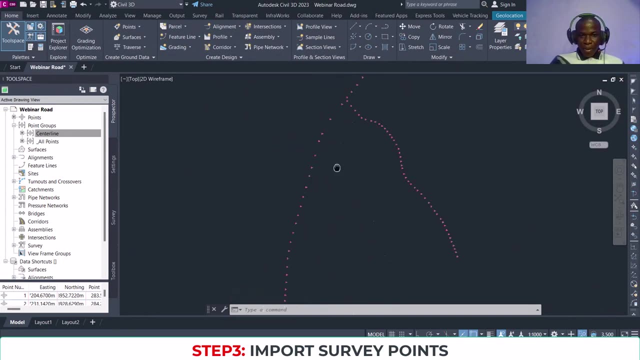 my keyboard and then press Enter, it will isolate only the centerline. so this is my centerline. of course it looks like it's. it's a very nice part, but when we are designing you may see that the course that is kind of coming here may not be sufficient. so it's going to of 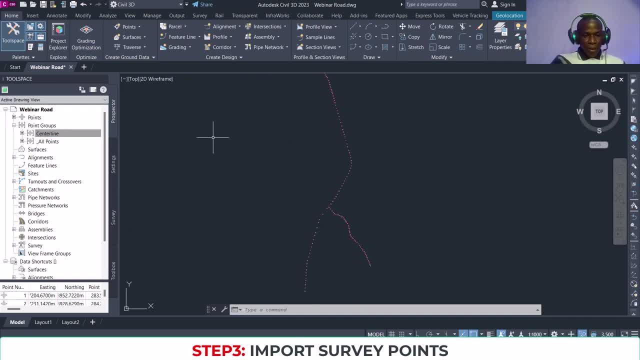 course, be based on our design code. so that's it, let's move on. let me on isolate, on isolate. okay, so I have all my points back. so that's the good thing for creating point groups. I like doing that. now I can, I will create point group. okay, for all these points categories. remember when we reviewed our 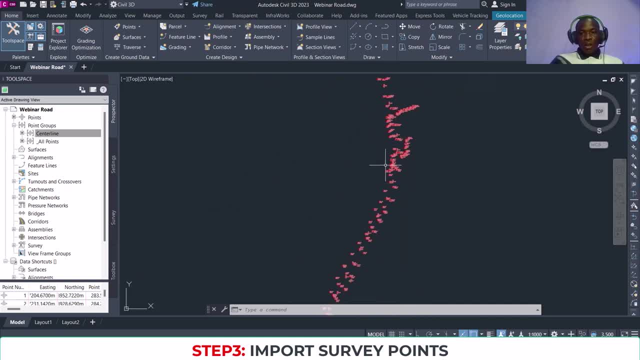 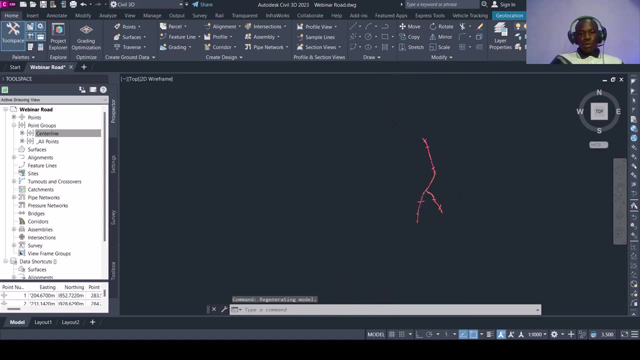 points, our survey data. you should know all the points, descriptions and then create a group for all of them. okay, I won't do that now. okay, so sufficient is the center line. now the next thing on our design procedure is to create the surface. so still on the prospector tab. 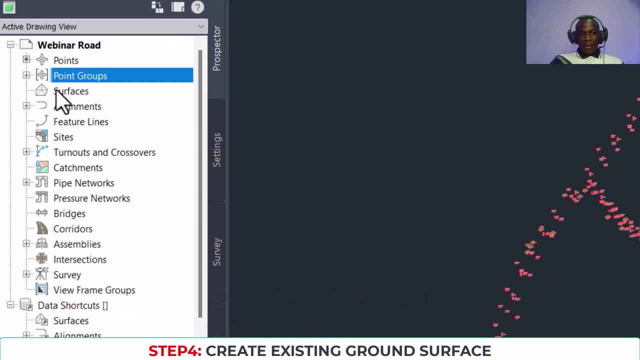 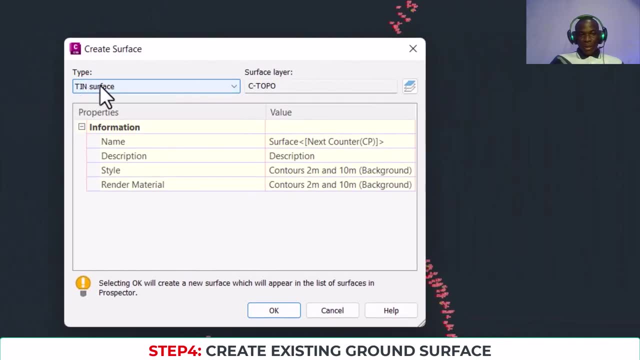 let me minimize this. we have the uh surfaces. okay, you right click on the surface and create surface. we are going to create a thin surface, okay, automatically it gives you thin surface. so and the surface name: we are going to name it: uh, eg surface, eg surface. okay, then you press. 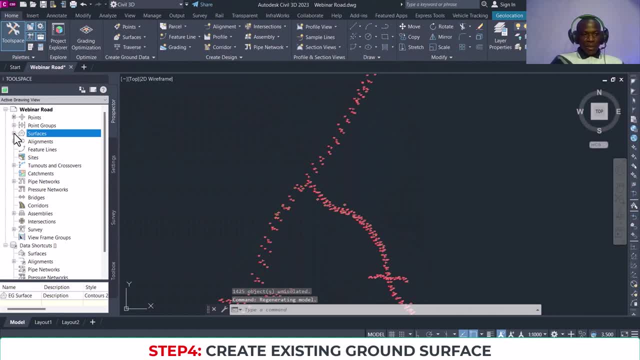 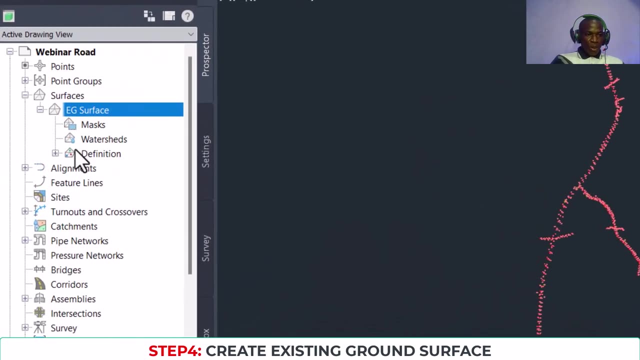 ok, now you have created the surface. you see this uh button comes up for you to expand and then see that surface you have created. okay, i've created it, but there is nothing showing because you have not added any points to the surface yet. so you have to expand the surface. you find descriptions. 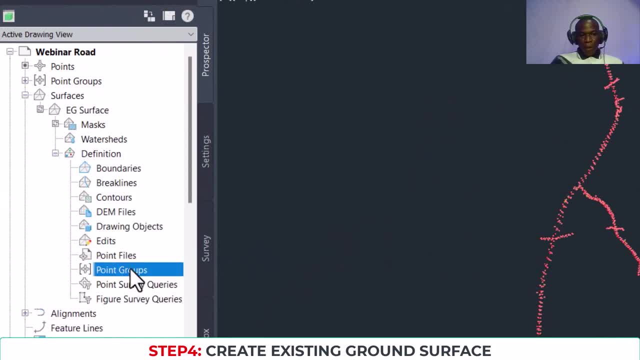 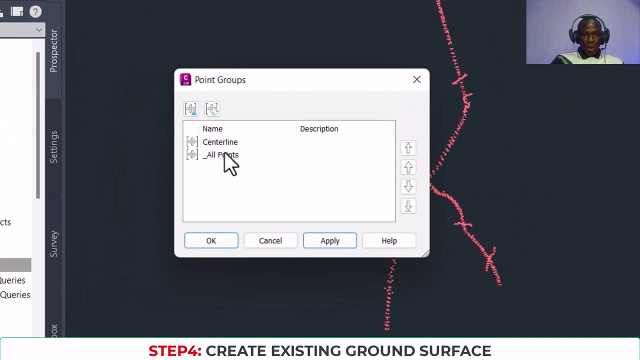 expand descriptions and then you find the point groups. here you right click on the point groups- add, so it brings you all the groups that you have so far. we just have two point groups. that's because we only created one more, which is the center line, and remember this center line is: 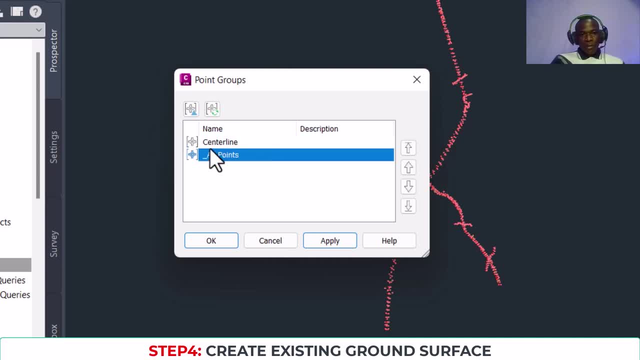 still contained in these all points. it's not the center line. it's the center line. it's the center line. it's not like it took it away from the all points. this all point is all the points in this. so this is what we're going to be creating our uh surface from. so we press ok. now you see our. 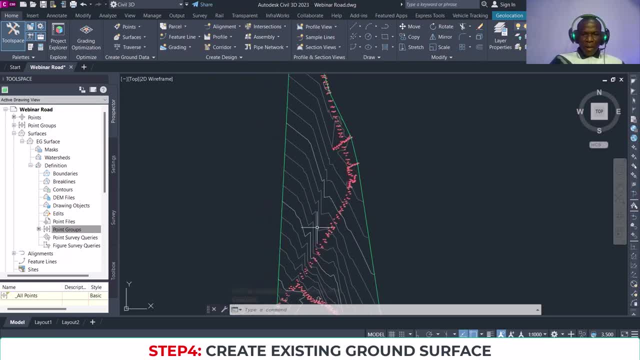 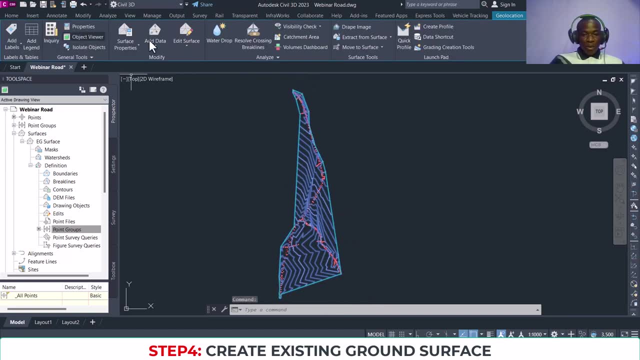 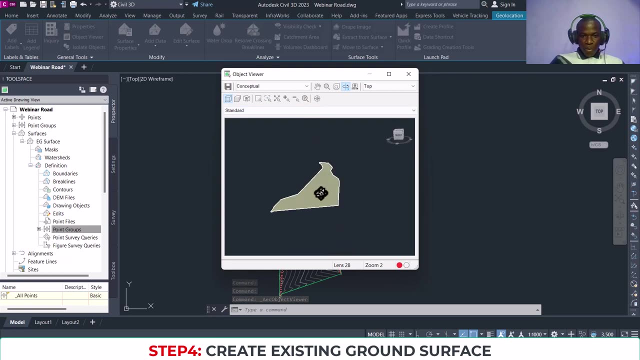 surface. this is our surface, beautiful, but it's over, uh, it's, you know, triangulating over a large distance. you can view this surface. okay, this is what i like doing always when i'm designing. i kind of visualize what i'm doing. so, if you, if you press object viewer, you can see the surface. 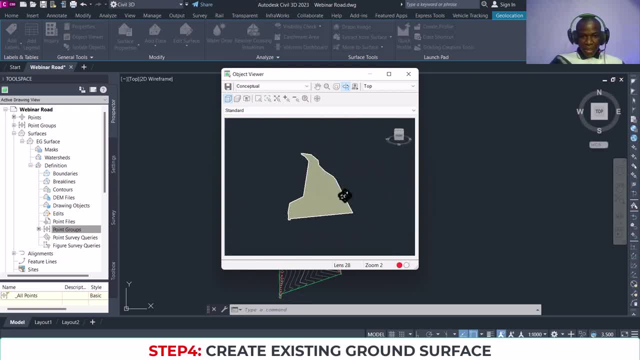 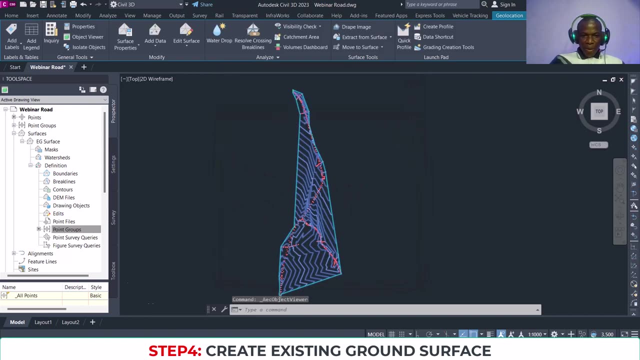 okay, yeah, as you can see, this is relatively flat. that's why you're not seeing. i see there are, you know, variations in the levels. okay, if it was maintenance, you see, you see it showing, okay, but i don't like the way it is, because i don't have data around here, but this surface have triangulated. 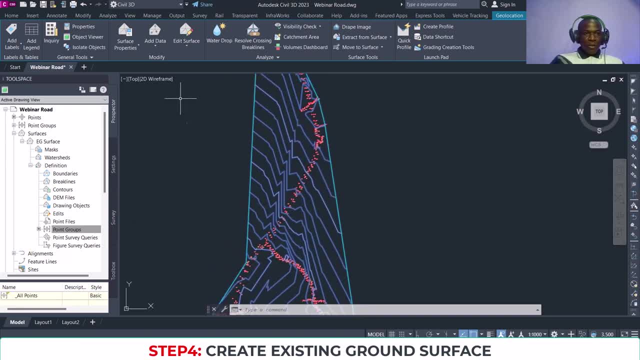 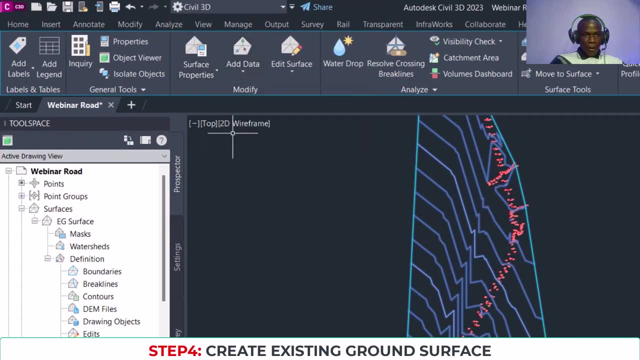 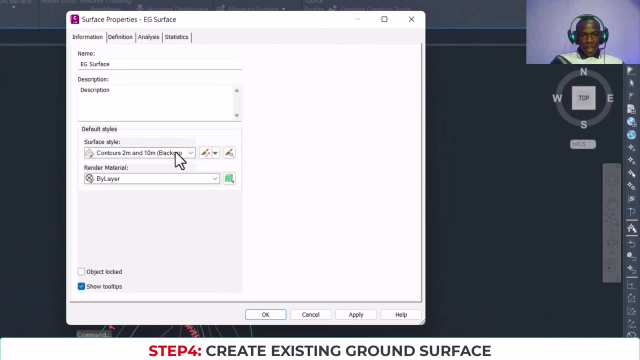 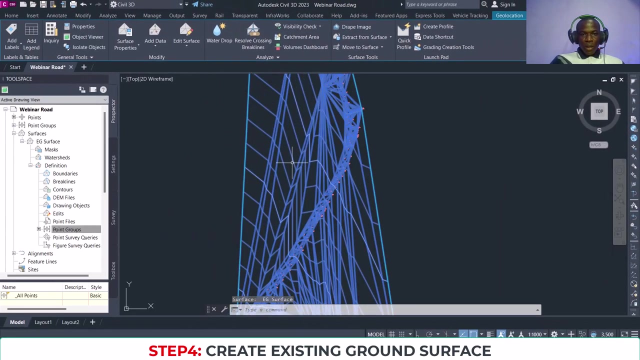 um, you know all these places. i can delete it, but i have to first of all change the surface to triangles. okay, i can find that here and this modify tab. you go to surface properties and then you'll see the surface style. change the surface styles to contours and triangles, then press ok. okay, then you can use this edit okay. 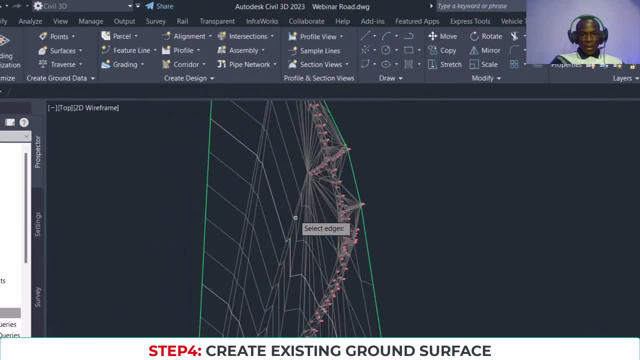 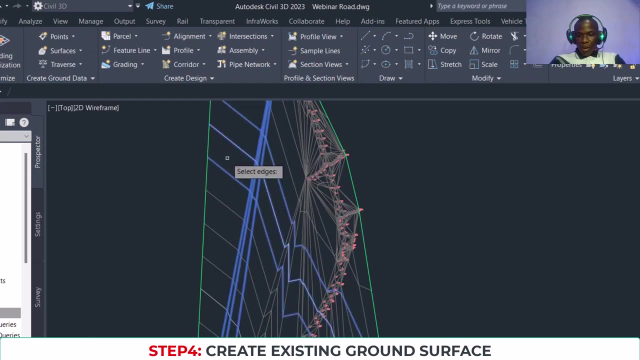 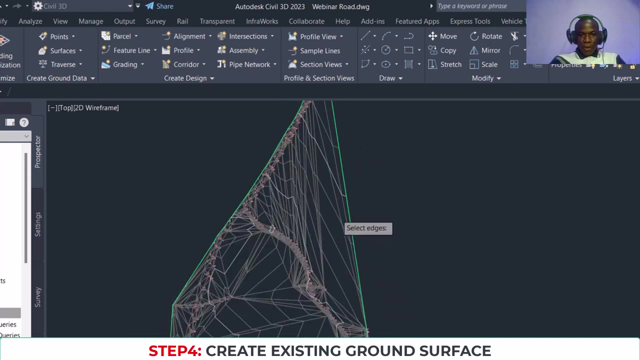 edit surface and then delete some lines. you can go to deleting some lines like this: okay, i'll press delete. okay, hold on, i'll just delete some lines. okay, i'll delete. you also request enter when you, how, when you have highlighted some points so you can see the surface is coming fine now. 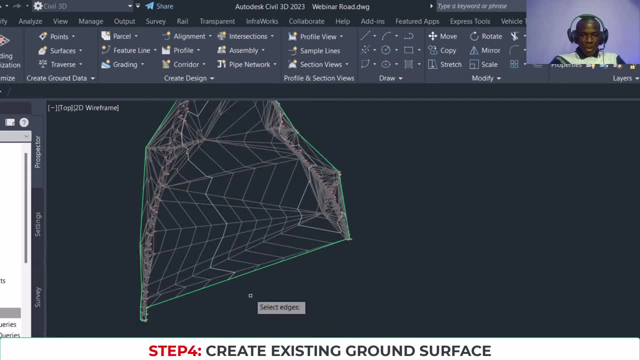 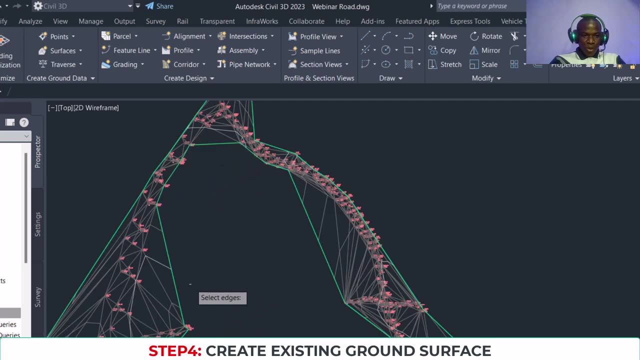 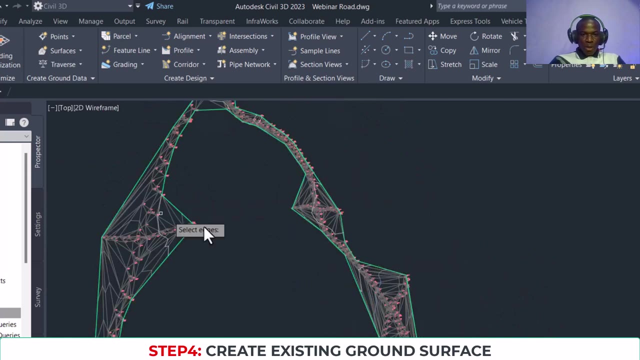 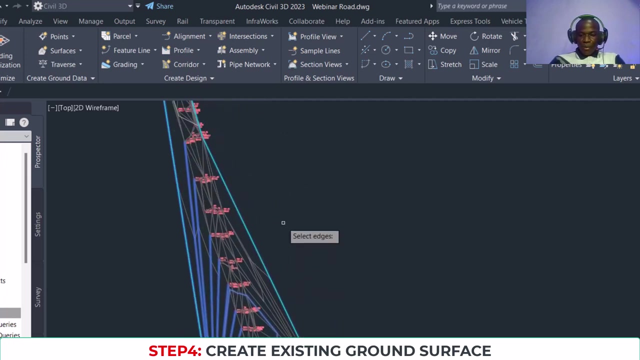 which you know about the boundary. okay, it's coming, fine, so make sure you don't you don't go too much into your proposed. so i will do that continually until i have a very fine you know, remove all the excesses, okay, but uh, let's, let's just move on. okay, you, at least you see how to do. 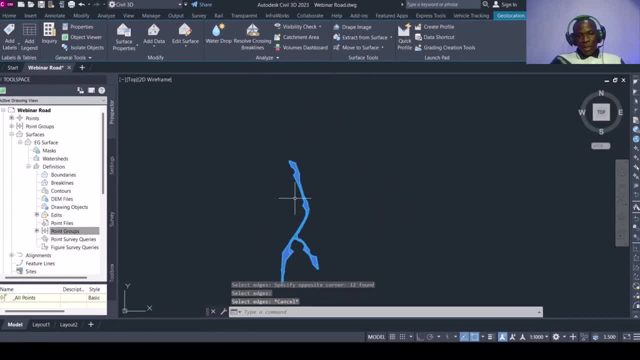 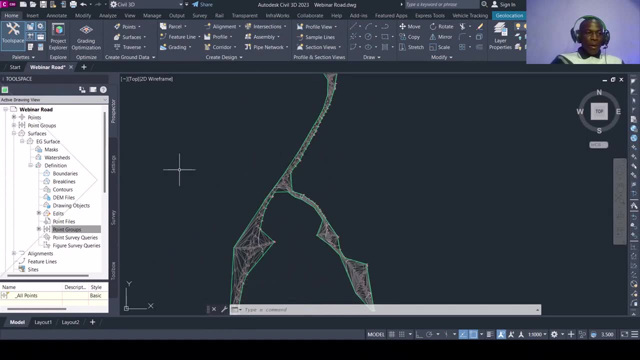 that you can do that for the rest, at least, if you not jeopardize our design. okay, for now. yeah, so let's move on. let's move on. we can now proceed to creating our alignments. all right, so moving on. we can now proceed to creating our alignments. all right, so moving on. we can now proceed to creating. 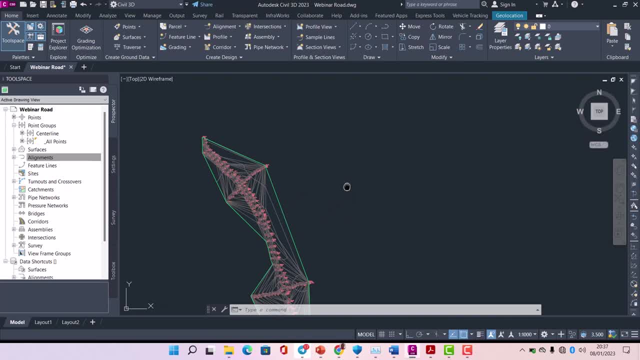 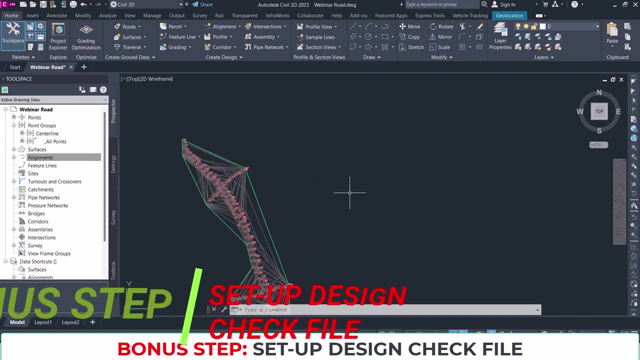 our alignments. all right. so, moving on, we can now proceed to creating our alignments. all right, so, which is to create a horizontal alignment. but before we do that, of course, we need to have our codes set up so that it can be checking our design for us. so to do that, just type design criteria. 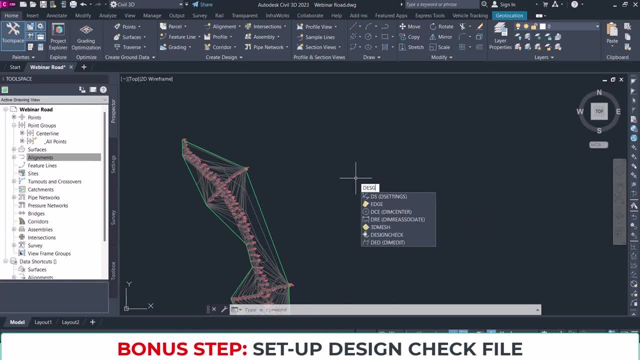 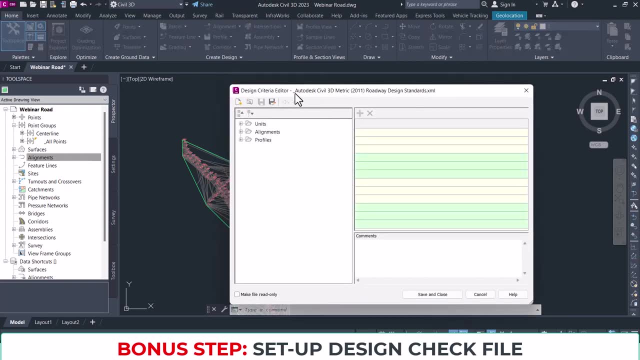 design design criteria editor and press enter. so by default you have the autocad civil 3d uh 2011 roadway design standard. all right, so you can modify this into your country's codes and then save it into civil 3d. okay, that's the simple thing to do. so, um, look at under units we have 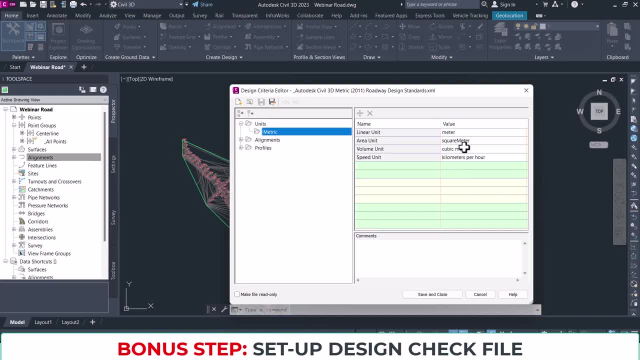 metric whatever. so this is just a normal unit. okay, if you're using metric system, which is for nigeria, we're using making a system, so you leave all this one by default here. so unless there's a need to change them, but here's where you make the changes. so in the minimum level you can change the. 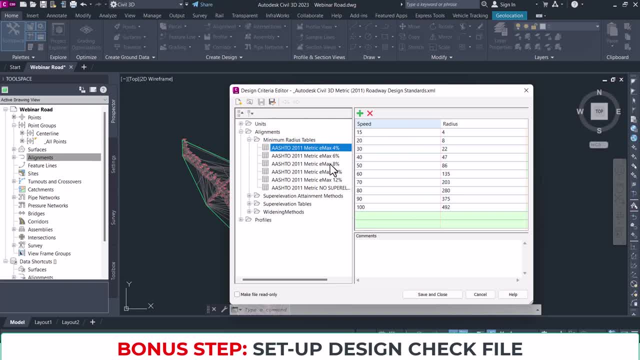 minimum radius table. okay, it might be different for your country, so this is where you just adjust it. all these things are editable, so you can edit all these files, all these things, and then save it. so let's look at this first one now. okay, let me open our manual. the federal means of works on. 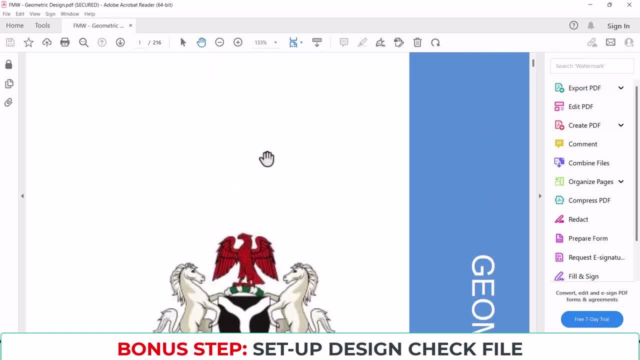 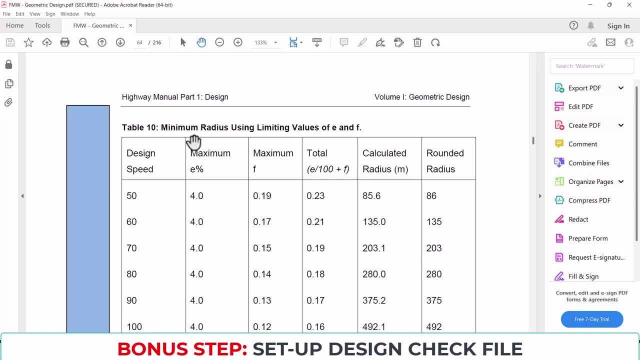 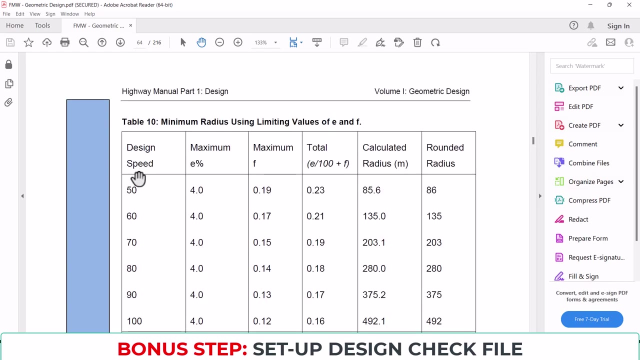 highway standard manual. okay, this is it. this is how it looks like. this is the first page. okay, let me go to separate 64. that's where what i'm looking for is higher. p64 contains the minimum register. okay, as you can see, for a design speed of 50. now it looks like we don't have design speed of. 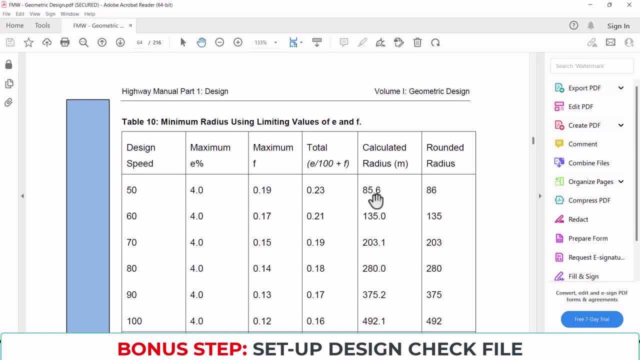 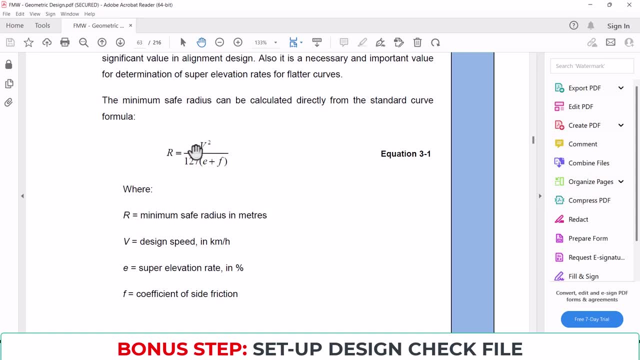 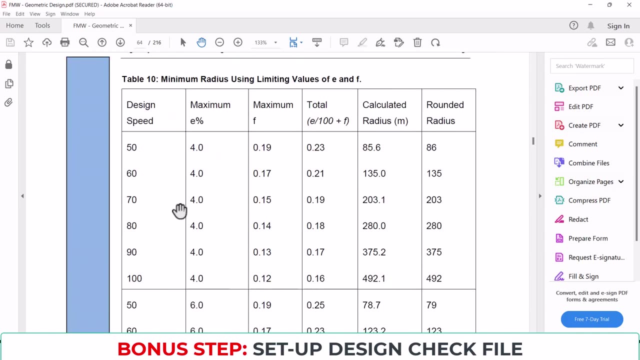 anything below 50. okay, so on this table. but actually we do, because this is the formula here, right here, for calculating the minimum radius. so it is, you know, you can look at this later. okay, let me not describe it. so if this table is what you are constrained to work with, 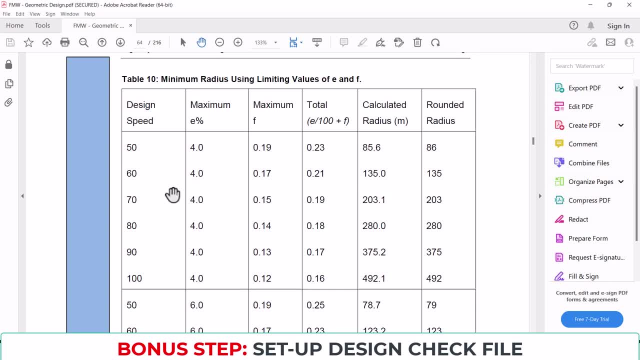 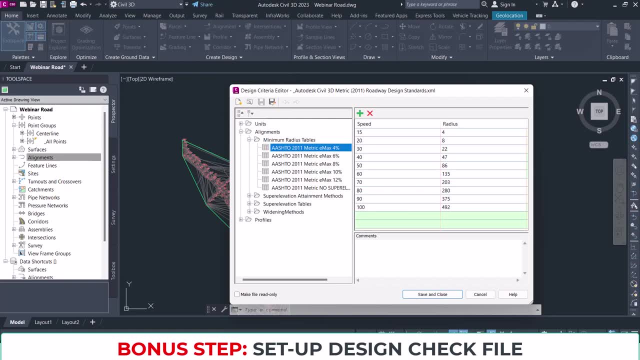 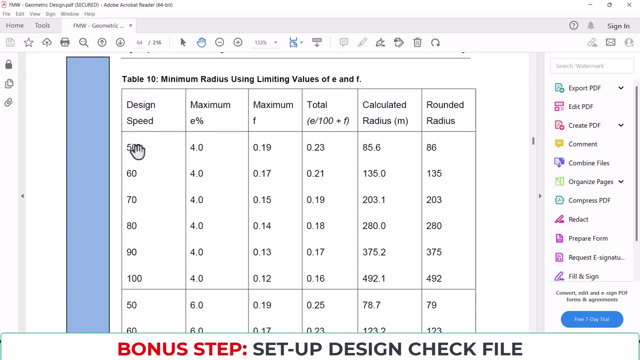 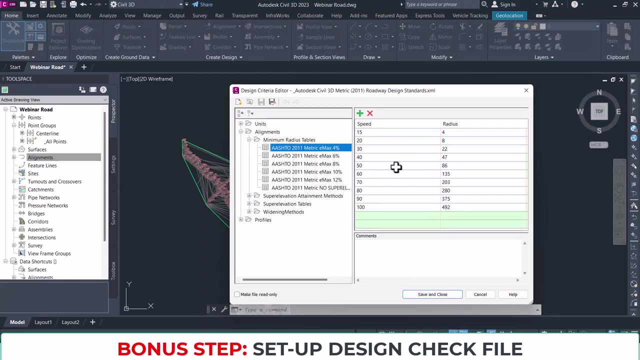 based on your country's code. you can all, you can program it in that interface that we just saw. okay, here is it, let's say, maximum for a maximum super elevation of um four percent. okay, all this was for four percent. at 50 designs, the design speed of 50, we have the radius to be 86.. so if you look at here, for 50 it's 86, it's almost the same. 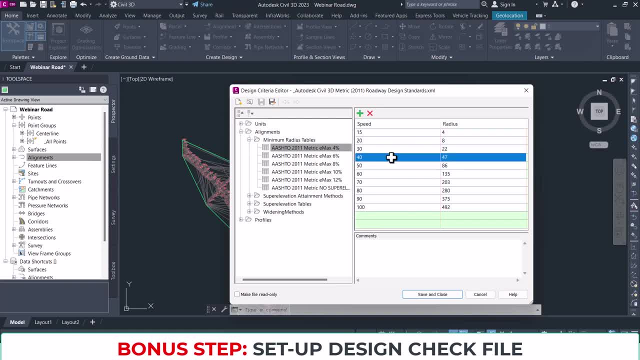 i mean, it's the same for us too, just that in astro we have lesser design speed. so, for instance, if i want to have this ones removed so i can just click on them and then click this button, all right, then remove them. so i'm left with from 50 up to 100. is that what i have here? yes, for 50 up to 100.. so yeah, 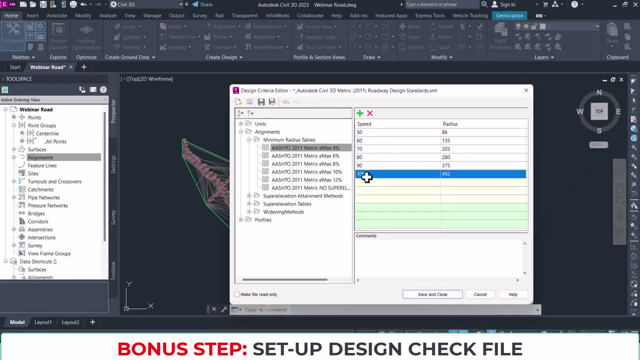 so this one is already. i'm beginning to customize already. so let's say, my all is up to 120.. all you need to do is click here and then add 120. okay, then i said maybe, if i've calculated it, maybe 700. it is there i put it. so once you do that for your own country's code, calculate everything, all right. 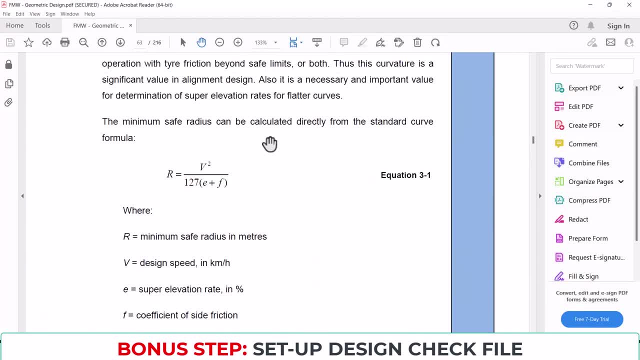 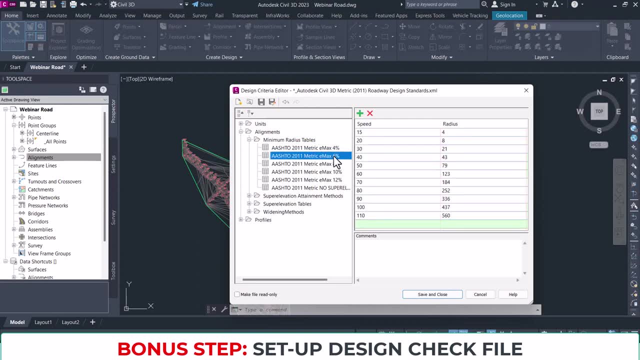 if your own formula happens to be different from from this one. here you can calculate everything and then infuse them. for a maximum spelation of four percent, then for mass exploration six percent. you do that once you change everything. while you are changing it, you can change the name here. 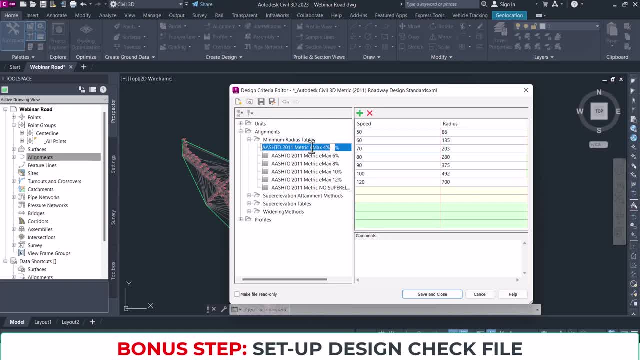 okay, let's say i change the name here. you just double click, i change the name. instead of h2, i call it mwh- federal resort worker housing highway manual. then it's 2013 hours. so i'll just delete it as 2013 and press enter. so can you see i've just saved it. so i do that for all. 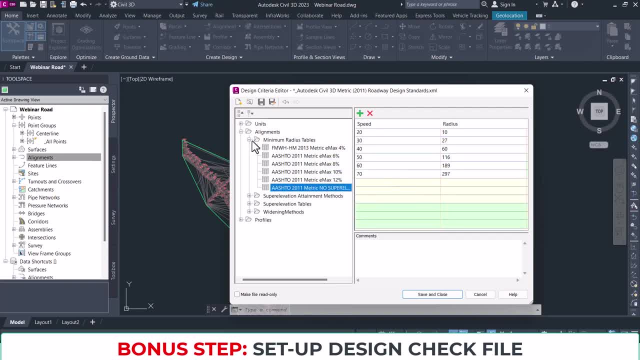 all assuming there is uh is different. okay, so when you are done with that, you go. you go to super elevation. then if there is need to change this one, these are formulas. if there is need to change the formulas, you change them. this is the attainment method for super elevation, okay, so. 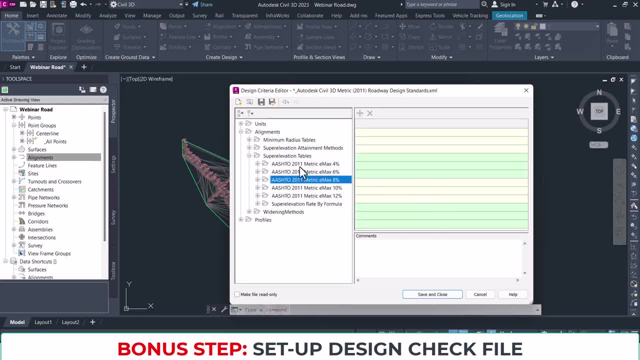 when you go to the super elevation tables. okay, as you can also change them. once you expand it all, you can change these things if they are different from your own countries. good, it's quite. uh, you can see, you will spend a lot of time, some time doing this, but once you do that, of course you're. 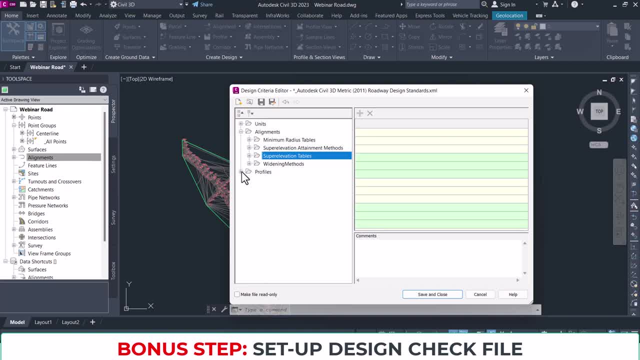 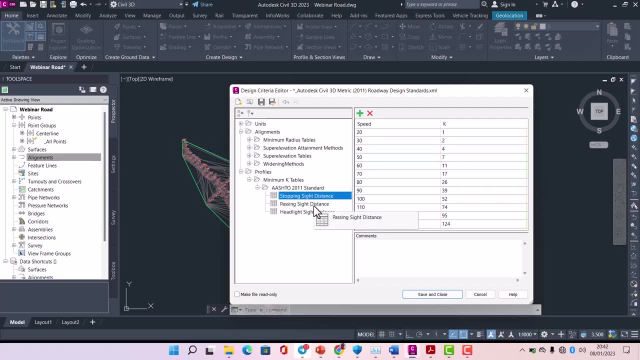 going to save it and then use it for future uh designs. so, minimum k table, like for our, our minimum, our k table. it's almost the same thing, of course, with h2, so but if there's any difference with your country's own, you know, you just adjust it here and then, when you are done, 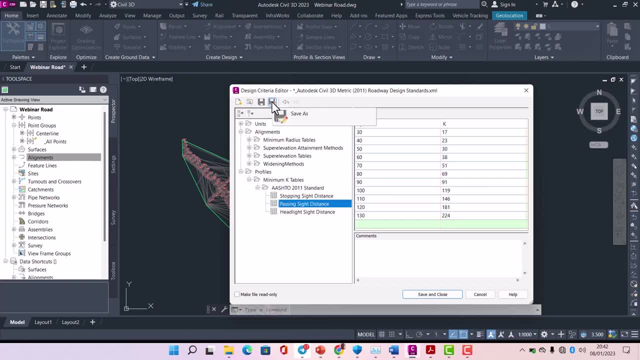 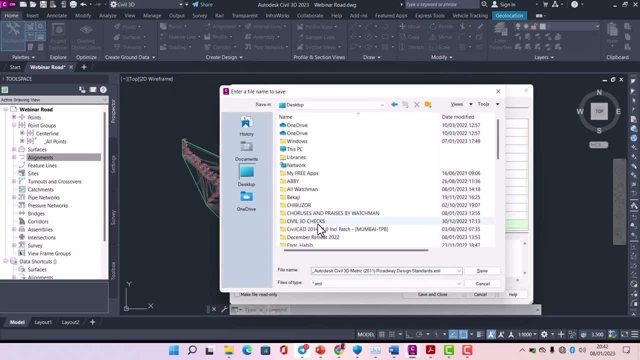 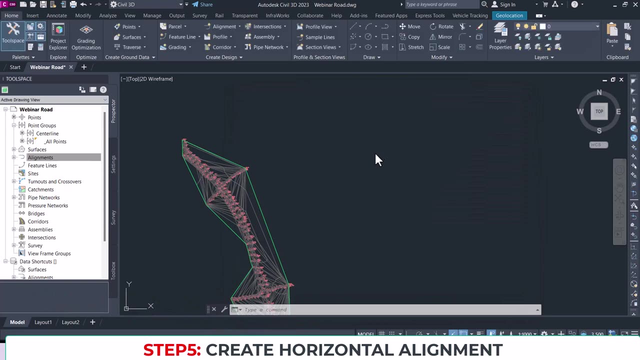 look at this button right here. it says save us. so when you click on it and save us, then you find your browse to somewhere in your file, uh, where you want to save it to, and then save the the file. let me cancel, so i'm not saving anything because i already have it done. okay, i just need to in. 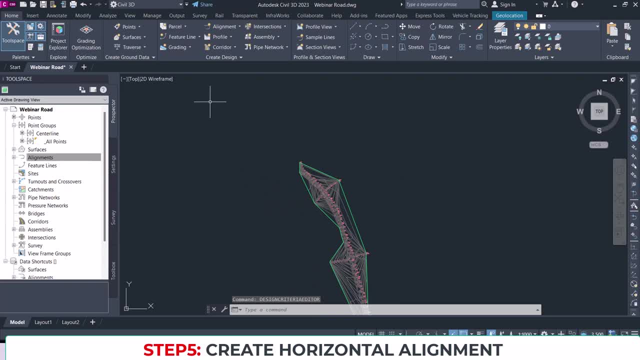 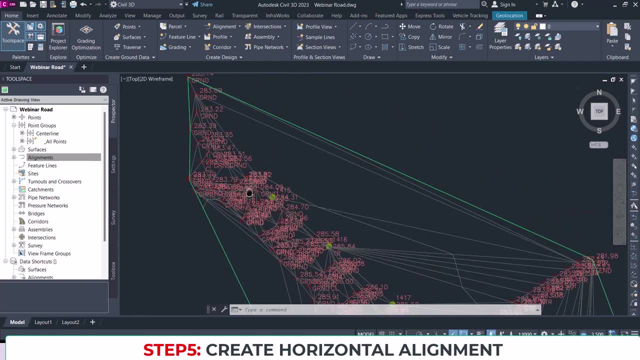 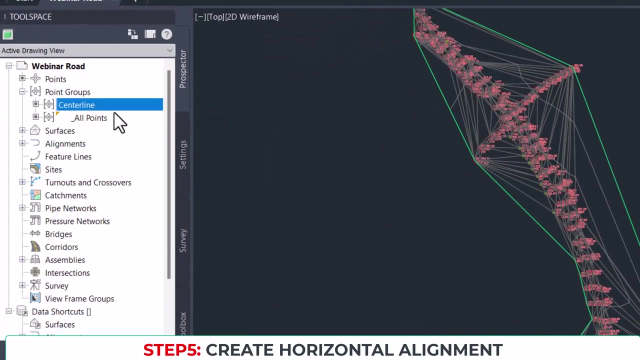 my part, my while i'm designing. okay, so let's quickly go to design our alignment. so before we do that, remember i'm going to be working on the center line. okay, only so. remember, we created a, a group for a center line, so let me select that group and isolate it. 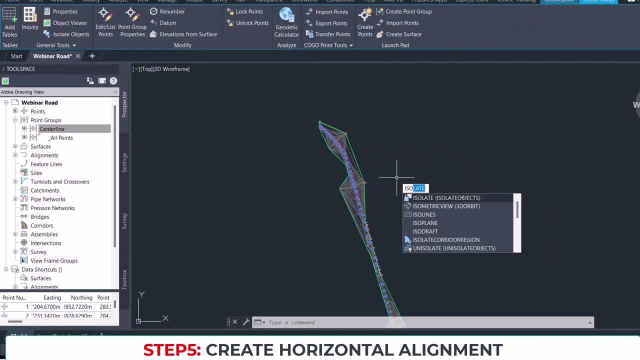 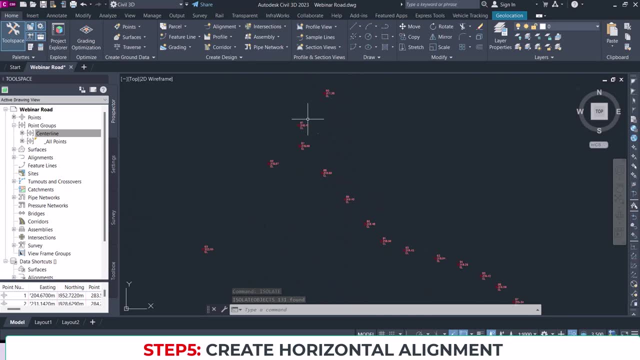 okay, let me select my center line and then isolate it. great, i've just isolated my center line, so i'm going to uh, i have less distance. so i'm going to uh, have less distance. and then i'm going to go to my center line. so i'm going to uh, i'm going to 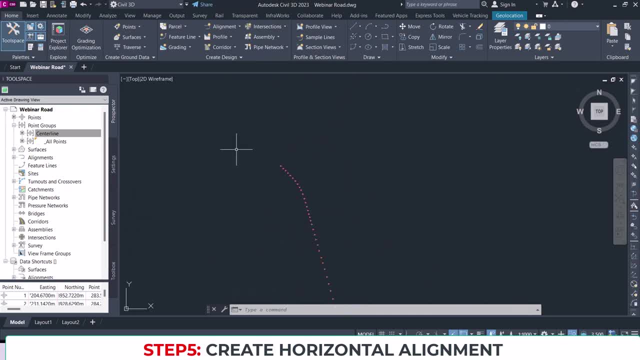 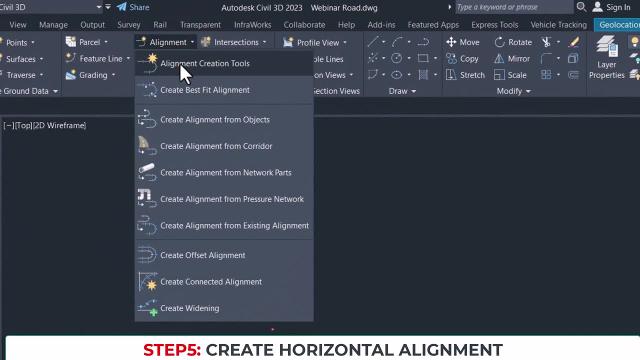 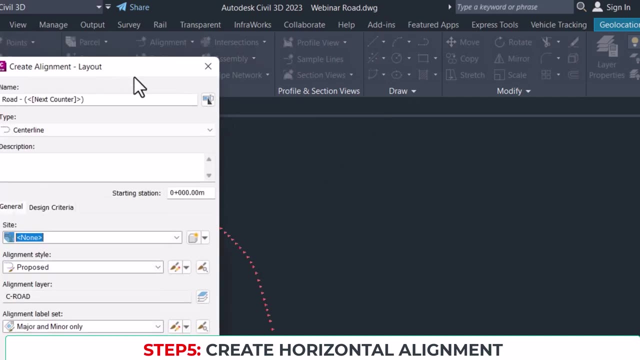 ovens while is designing my alignment. so let's go to design the alignment. so you find that on the home tab and then you go to alignment. on the alignment you select create alignment creation tool. once you click on that it opens up this dialog box for you. so you have to name your alignment. let's say you call it. 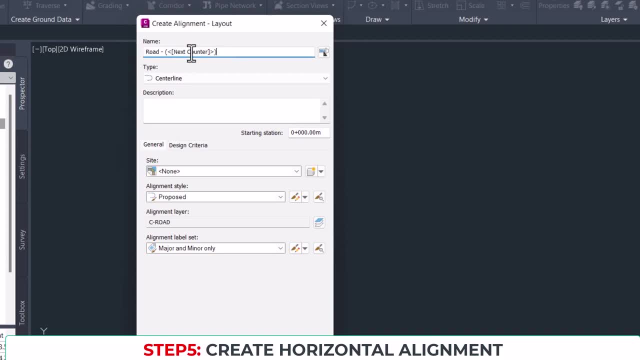 room one. okay, already we have this account, this, this thing, naming it for us. okay, I believe, if you open your own, what you see here is alignment one. all right, because I've worked on civil 3d before. you can use information that you have used before. okay, so let's say we want to name this one. you can name it manually. 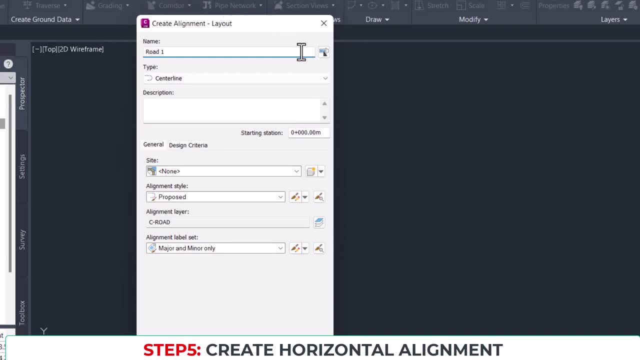 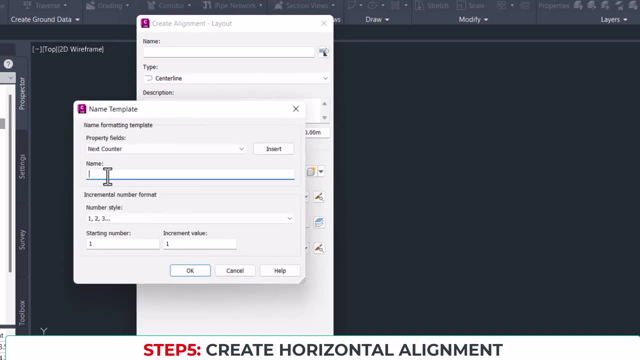 or you can have civil 3d. set up a template with civil 3d, just like was here before. let me just show you on this template. I can just call it. to name it: road Nescauta. I added an account. I added an account. this as next counter. so and the counter is starting from one and increasing by. 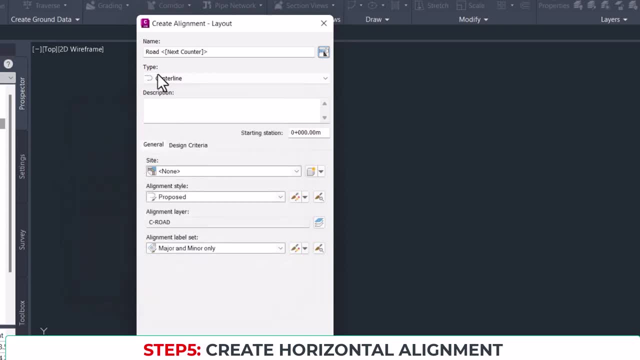 one always. so if I said okay, so you see it's going to name this alignment rule one, okay, and then if I this, the next alignment I'm going to design is going to be ruled true, okay, so automatically be naming it. so I don't need to feed any. 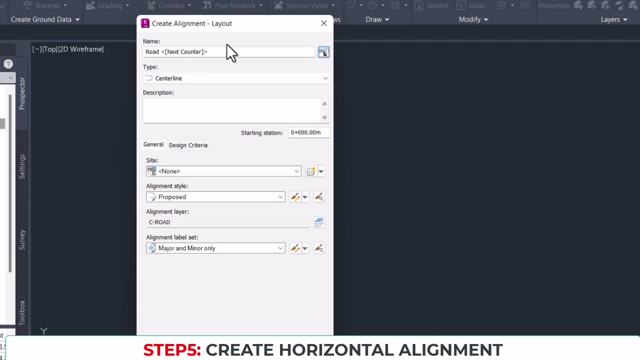 name on this place again. so that's the good thing. simply allows you to do: just automate the process. so let's go down. now we have the general tab. okay, we can save it to a site, or we don't have a site for now. so, and then the style is a. 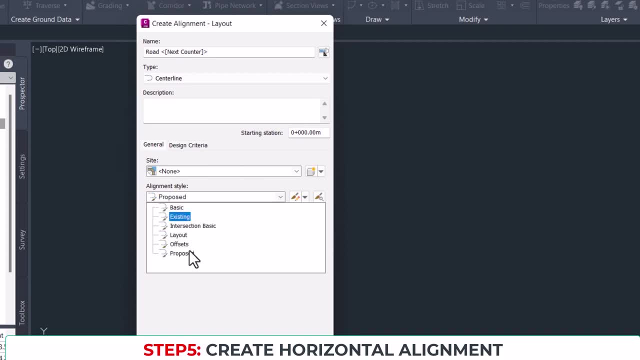 proposed alignment. these are, you know, default styles that are available for you. okay, you can always create your own side by coming here and create. create. this style simply shows you how your alignment will look. okay, the colors for the lines and the. you know the styles of the lines. 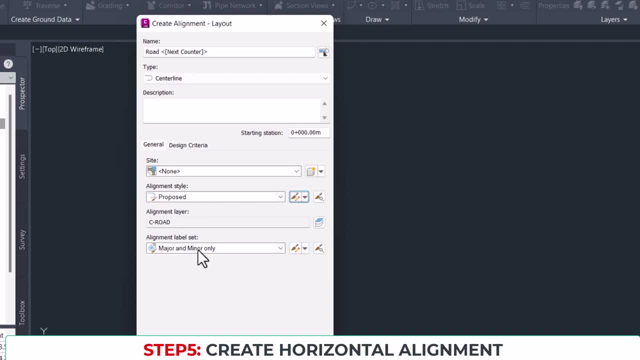 they labeling and everything. okay, here comes the labeling. so in this case, I just want to level the major and minor stations. okay, and that's good. so now let's go to our design criteria. now, by default, we have our design speed to be 100 kilometer per hour, which is exactly what we have derived for our design. but in 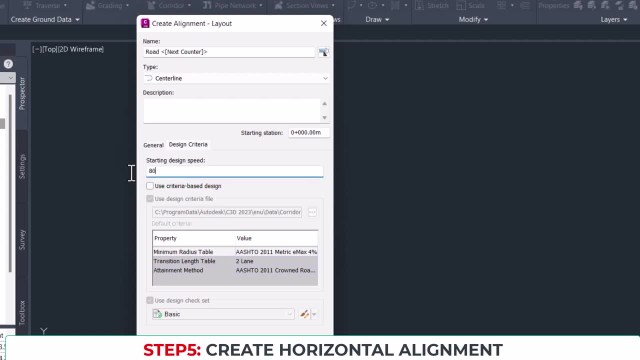 case there's a need to change, you just highlight it and then change it. let's say 80, okay, once you have 80, yeah, that's if that's your design speed, but let's go back to 100 because that's our design speed. well, unless I forget here, 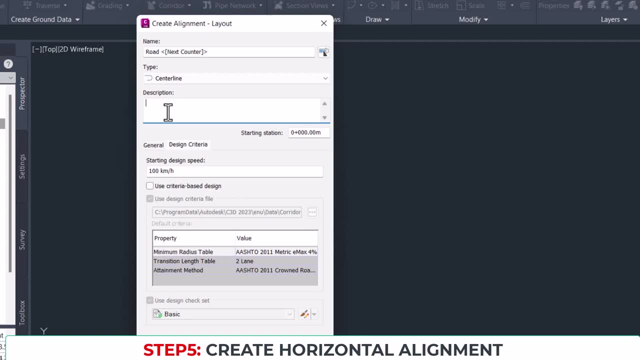 we have the description. you can describe that alignment. you know, assuming, because you're working with different engineers or even with yourself, sometimes you forget what the alignment was for. so you can do it. describe just anything that you wanted. you want, you wish to add to the naming. alright, so now, right under 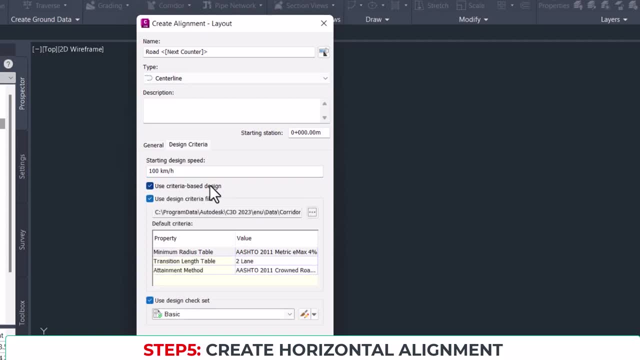 here you have to check use design base, use criteria based design. now, right on date, you will see the ellipse button for you to go and import your design. here you have to write under it to see the ellipse button for you to go and import your design codes. remember, i showed you how to save it. so if you have saved, if you have customized your, 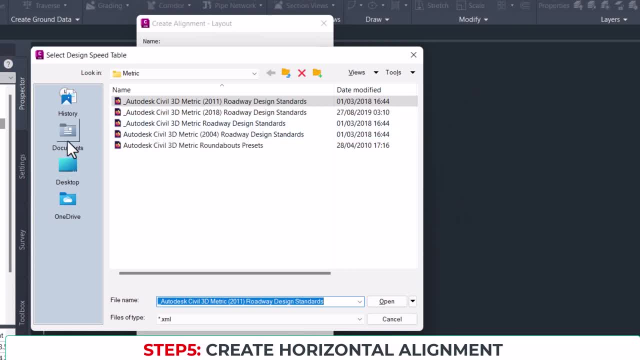 own design code and saved it, find it where it is. so let me look for where i've saved mine. so i'll go to documents and then i'll just quickly rush through where i have saved it. and here we have saved my own the standards for nigeria. so once i open that up you would see everything is. 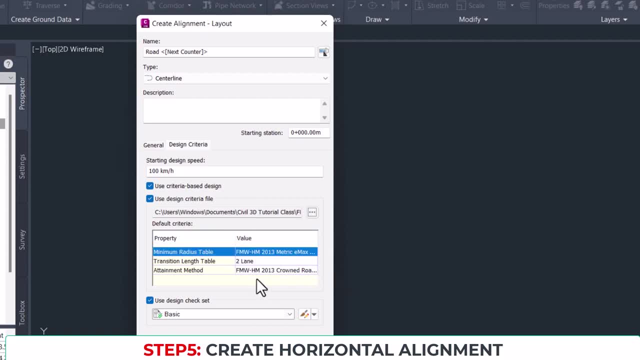 customized to federal resource works. all right, every manner, 2013. so you can see now, based on our design, uh, we have maximum elevation of super elevation of six percent, and then the transition lane- i mean it is two lanes, okay, and then the attainment method is, uh, crowned okay, so, uh, it's. 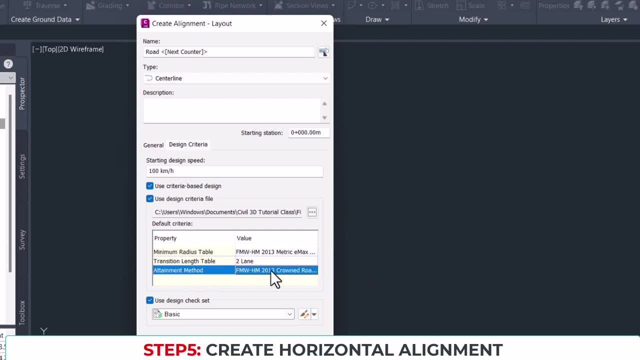 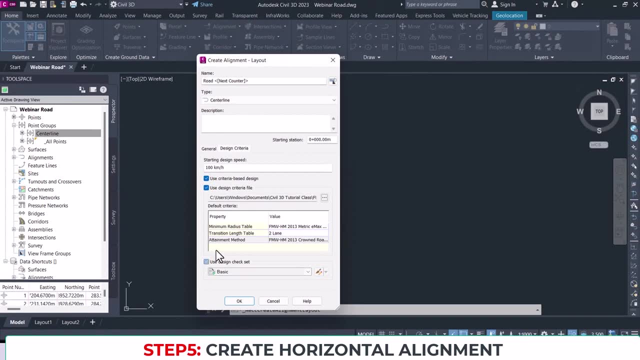 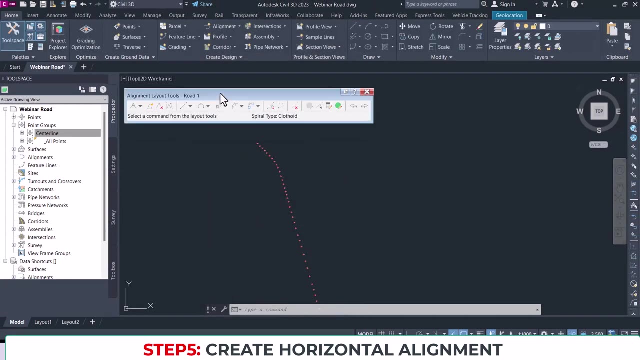 a crown. you know. crown means you know we're having a crossed slope. okay, the road is not. we have a camber, yeah. so now i don't want to use a design check set. let me uncheck that, okay, so, and then let's have one, okay, so it brings up this ribbon for you. as you can see, this is alignment. 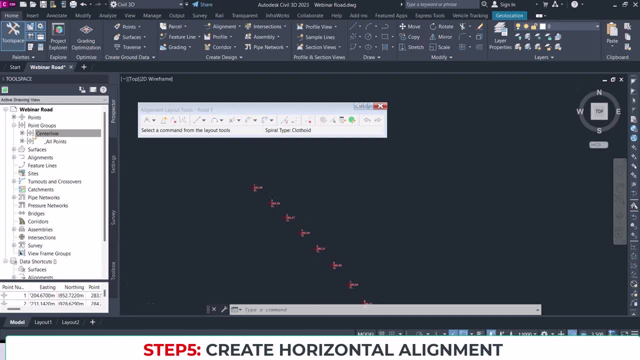 for one. so if we zoom in to where we tend to start, all right, we have this, all these tools allowing us to manipulate and insert our alignments. and you know, alignment is just made up of straight lines and curves, so from here we can just choose. let me show you, let me just quickly use the best method. i 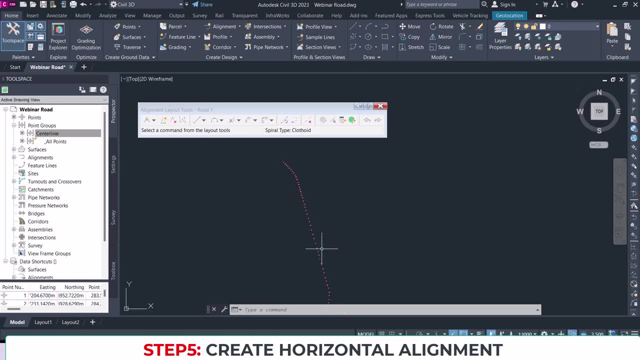 first of all, look at this alignment. of course i've studied this alignment and i've seen that, okay, from here we have a straight line and then we'll have a curve here, then we'll have a straight line, maybe going all the way up to somewhere here, and then we have a curve, then we'll have a straight. 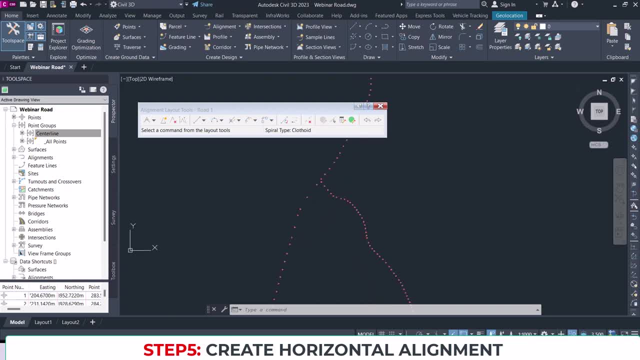 line and somehow i see we're going to have some- you know- dancing profile here, but it cannot dance too much because, uh, our design code will show us an error if we are below, so let me just quickly start. okay, i'll just pick up a line here and then start from the beginning. okay, once i use that, i 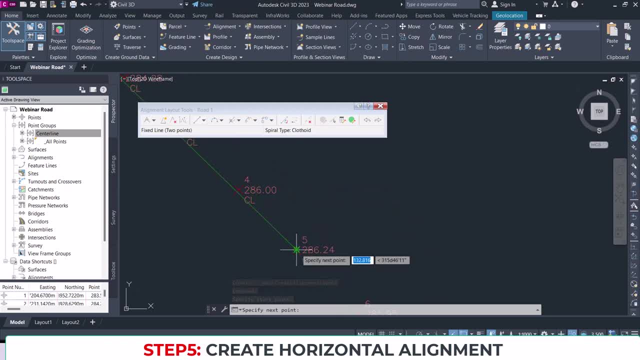 draw. i find a straight section and end it okay, like up to here. i believe my line is straight, so i press enter. okay, we are not done, of course, so we have to follow. find another straight section. okay, from here, let's say from here. okay, sorry that wrongly, let me pick it up again. so from here. from here, let's see. 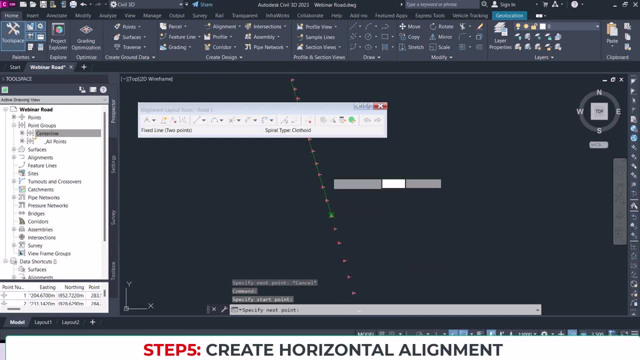 good. so going all the way, all the way to here, let's say it's a stress section. okay, let me zoom in. yeah, that's a stress session. let me, let me just enter. okay, so, as you can see, i need to add a curve here so i i can use the fillet command. i can find out here. 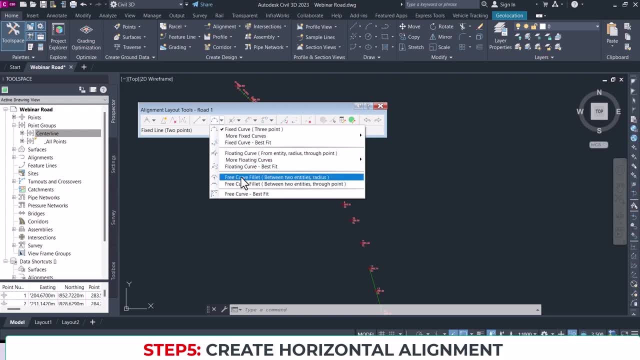 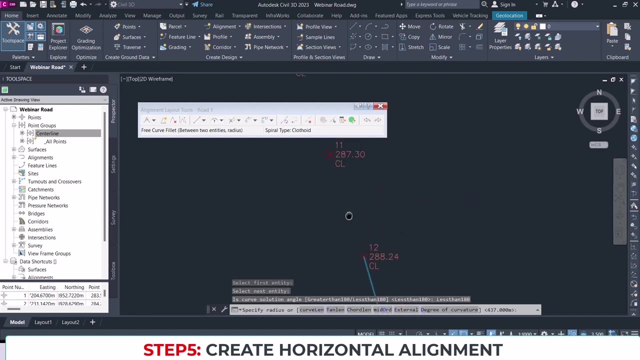 all right, you open up, you select free curve fillet between two entities with ridges. so let's put it here: we select the first alignment and then select the second alignment. it is less than 180? okay, the angle- okay, and then select one. i'm sorry. 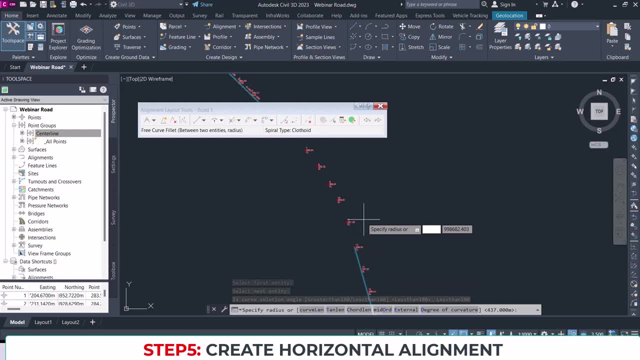 let's put a radius. remember our minimum radius was 437, based on our design speed, so let me use 450 here, for instance. wow, 450 is almost cool. okay, yeah, it's almost cool, it's almost going through our points. of course, these points are not design points. these are proposed center line. 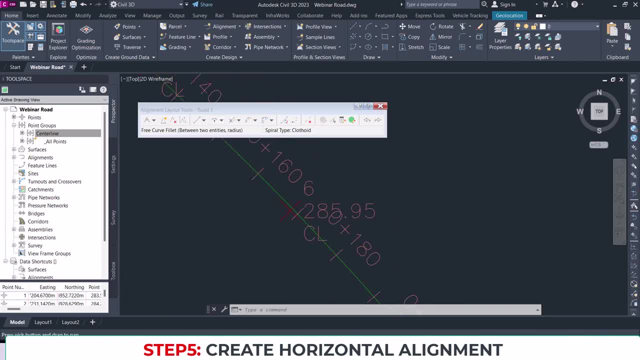 but we are designing it, so it's not going to pass through all the points, okay. so, uh, it looks good. it looks good if we, if there's any need to adjust it, for instance, let's say backward. this way i can see that we can move it backward, so we can drag it. you hold this circle and then draw it backwards. 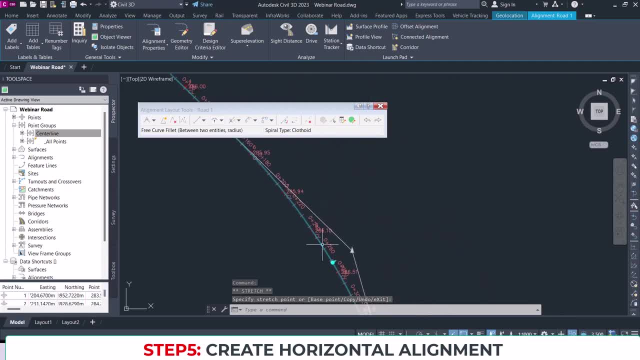 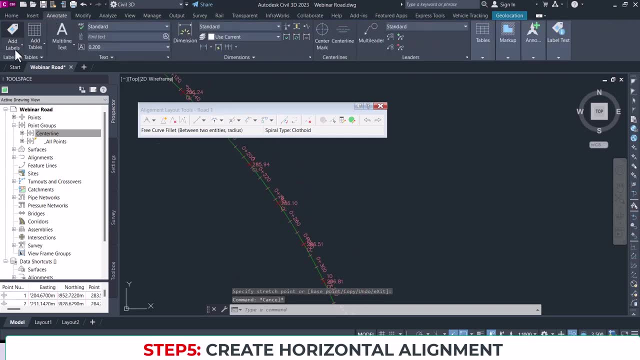 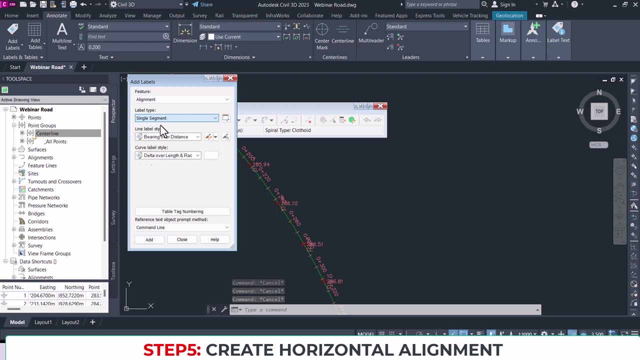 so in that case it will increase the curve radius. if you want to see what radius you have just done by what you have dragged, you can go to add a level, okay, and the level i'm adding is an alignment here, so i can label a single segment. 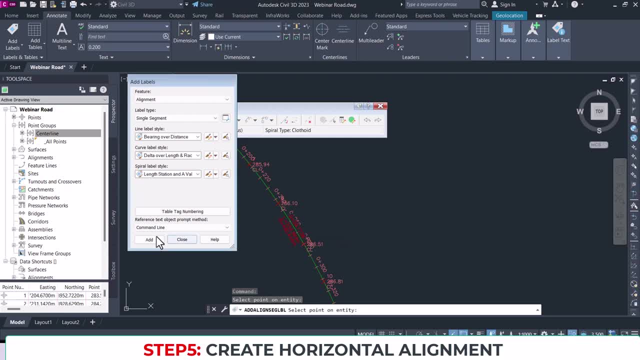 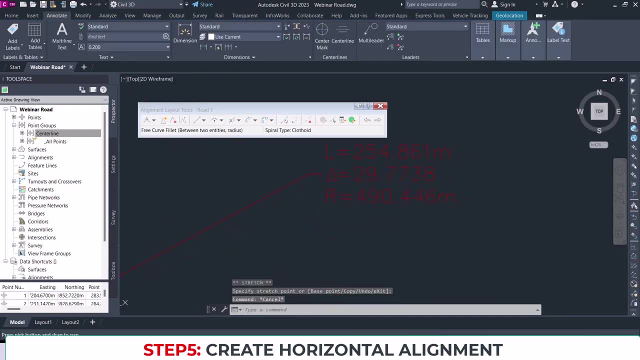 let me just add a level here immediately. okay, let me close that. let me, you know, stretch that out. okay, as you can see, the radius here is 490. okay, so it's well above our design code, okay, so, if there was, if it was below, it will allow us, let me just make it below and 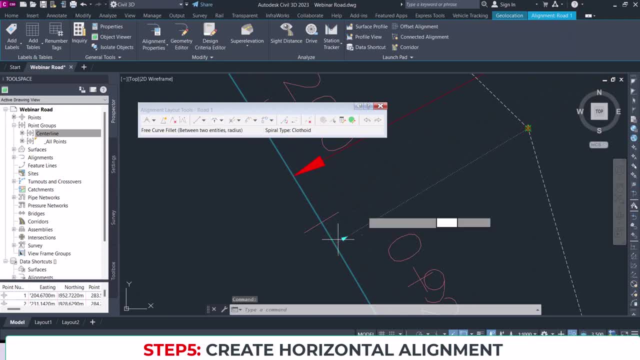 then show you how it will show an error. okay, let's say we push it upwards here. can you see a question, a warning sign here? so what does that one inside say? minimum radius is violated. so the current reduce is 344 and the minimum radius should be 437.. as you can see, the radius 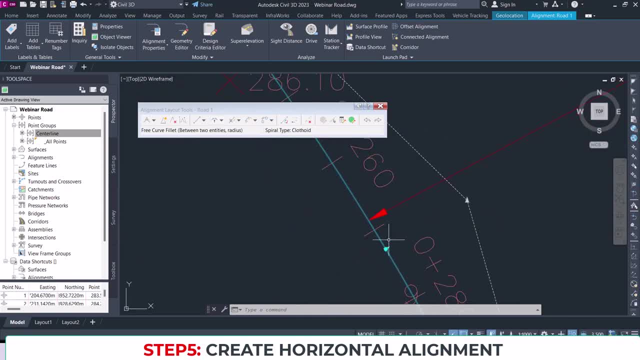 here is 344, which is below our standard, so we have to move it back in order for that error and that warning symbol to go. and our road is correctly designed, okay, so, yeah. so now we are back to 488. somehow, if you want to use a round figure radius, you can just do that by opening up this tab. 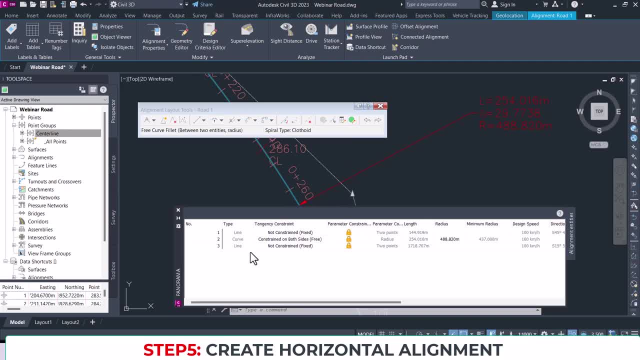 here. okay, you will see the curves here. this is the curve. okay, this is the radius here. you can manually add it here. you have to first. okay, you have to come on holiday. as it opens up you, let's say we type 500, also enter. as you can see here. it's updated here, so you can now close this thing back. 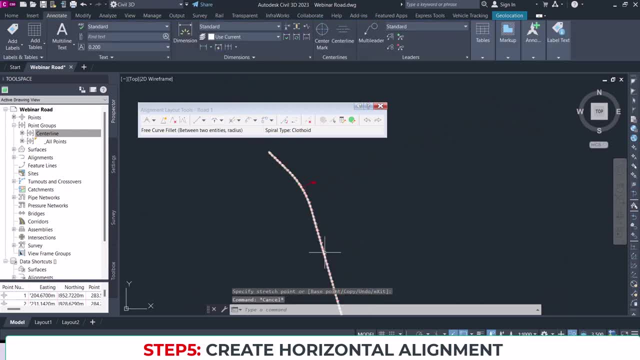 okay. so yeah, we'll do the same for the remaining um part of the alignment. okay, let me just do one more. okay, here we add another straight line. let's say we find a straight line from here, from here. okay, let's say, up to here. up to here, looks straight. 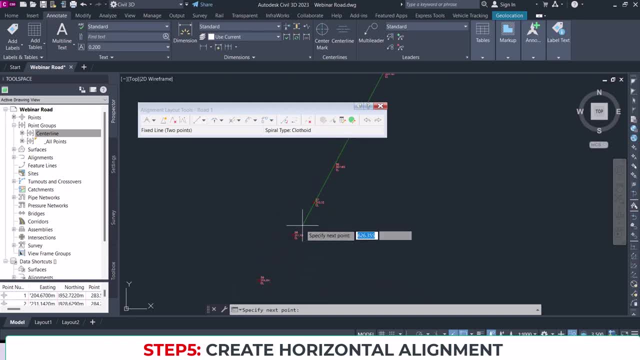 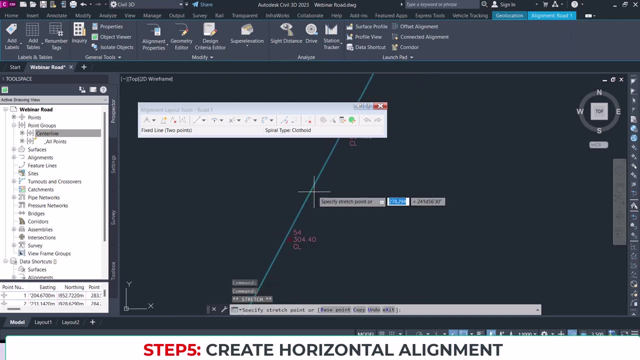 okay, up to here it looks straight. you must not even click on any line, you can just stop halfway. it looks like it's passing through somehow. i'm not going to go into all these details, so i'm just doing this, just to show you, to make you appreciate the process. okay, because you don't. 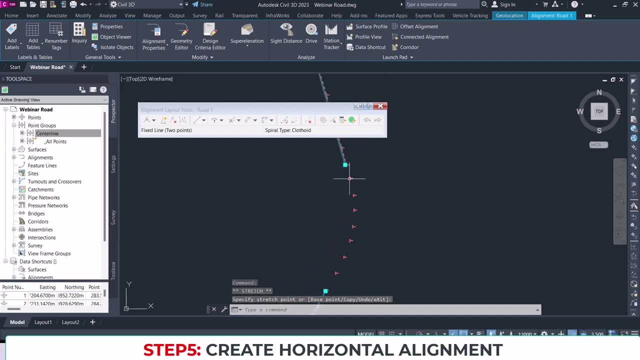 just put. you just draw it anyhow. okay, you have to. you know, since we are working with the proposed alignment, we can now try to match it. okay with it. but if we have the liberty to just design, when we have a large space of data, we can just choose randomly where we want to pass. but 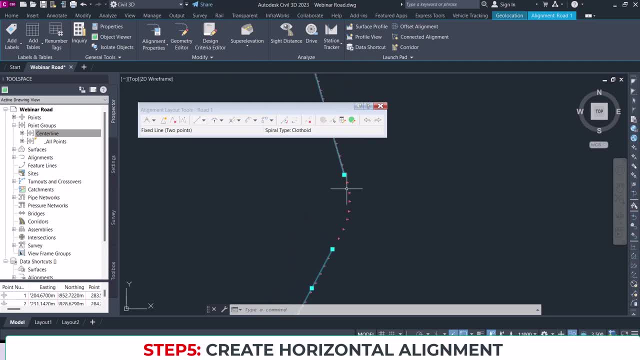 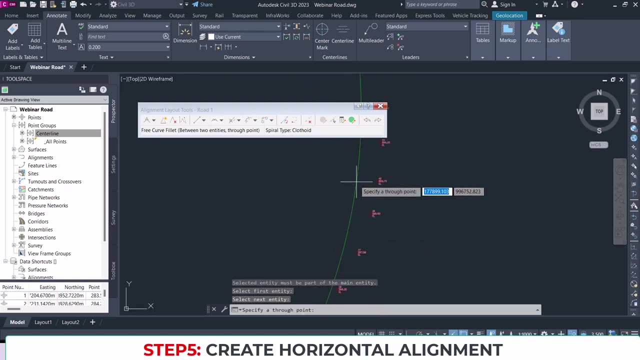 of course it has to be with proper information. so now let's go again and add curves. okay, now i'm going to use true points, not radius this time, so that it will be more dynamic. okay, if i click here, then click this place, the second one, so i have the liberty to just be playing around with it and then 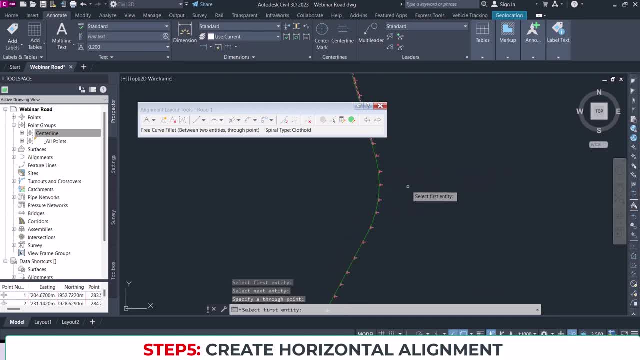 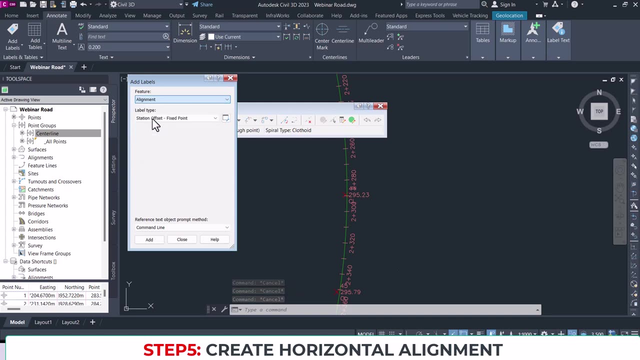 find the best fit and then drop it. once i do that, i press enter all right, so you can see i've put a. okay, let me also add a label okay to this place. i can add multiple level at the time. okay, but it's because i'm i've not designed the entire thing if i use multiple segments. 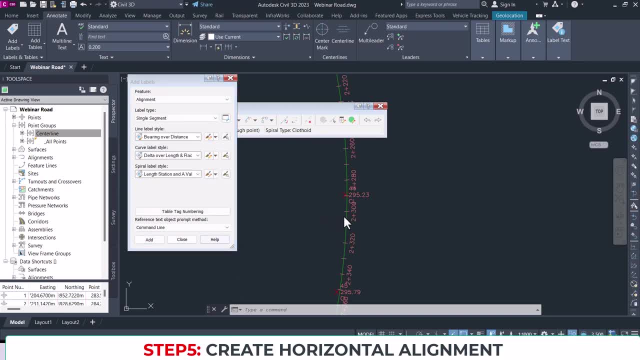 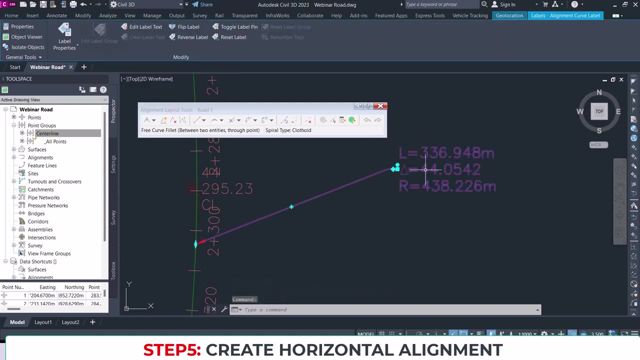 but let me just use single segment for now and then add the label here, okay, then you can see the radius is 438. wow, that's a little bit above the design. uh, the limit. okay, if i want to add that i don't like it, maybe i'll still go back to that conceptual ribbon. 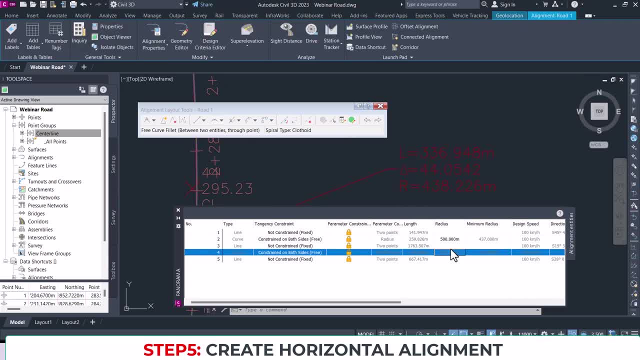 and then look at it here. so let me, let me add it, i need to. okay, if it's not opening up for any reason, you have to unlock it. okay, once you unlock it, it allows you to now edit it. okay, so let's say i want to use 450 instead of that, just to use something of round figure. great, so you can see it's 450 now. okay, so let's see if i can add it to this table. okay, so let's say i want to use 450. okay, so let's say i want to use 450 instead of that, just to use something of round figure. 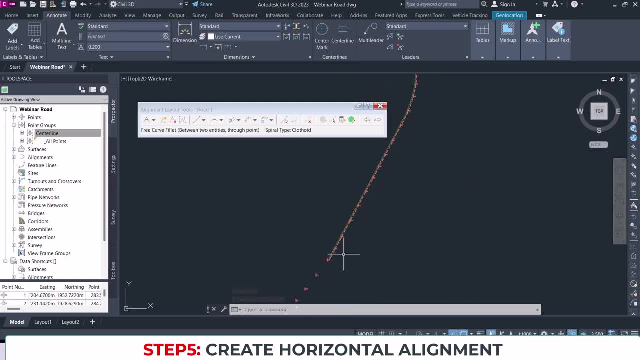 okay, i can make my, my radius, you know, a round figure. so that's what we keep on doing until the end of this alignment. let me do that quickly and then we proceed. all right, so i've completed that for all these alignments. okay, you can do that on your own. 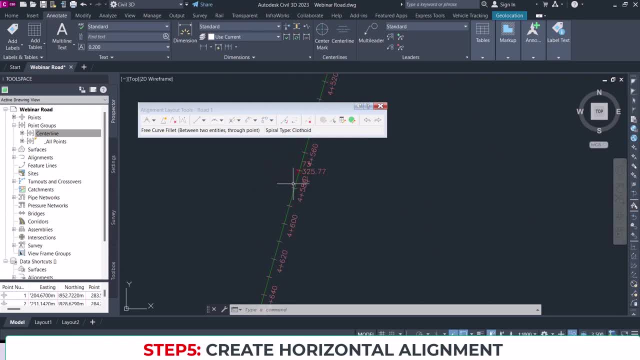 okay, you can see that there is no error. everything is moving fine and everything is, you know, coming close to my existing center line. all right, so the next thing is to just close this. okay, once i have closed this, i can now create the alignment for the intersecting. 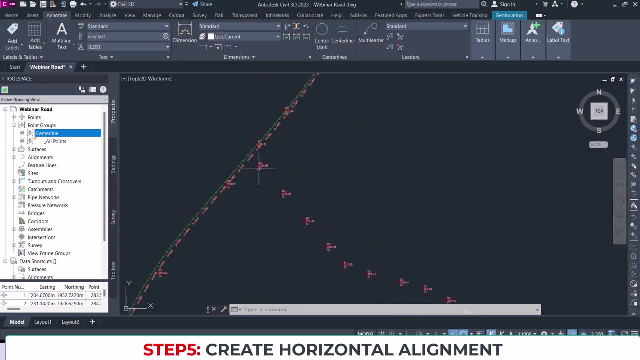 road okay and sorry, i forgot to mention that this road is, uh, 40, sorry, 60 kilometers per hour. the design speed okay. so because you can see there is more sharp curve here. if it was 100 kilometer you can't have this kind of sharp curve. how do i know it's a sharp curve? because i've had experience. 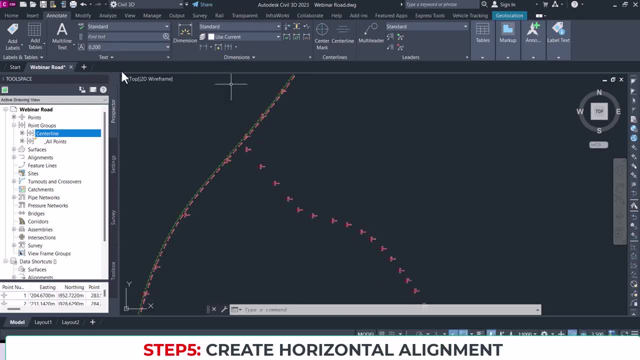 designing it. okay. so, uh, now i'm just going to close this, okay. so i'm just going to close this design speed, okay. so, because you can see there is more sharp curve here, if it was 100 kilometers, you let's design the nest alignment. so we go back to our alignment, okay, and click on. 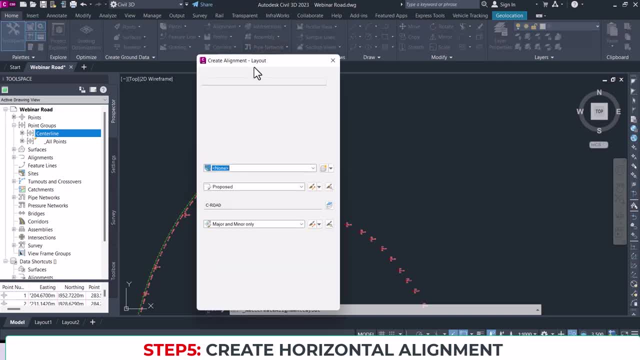 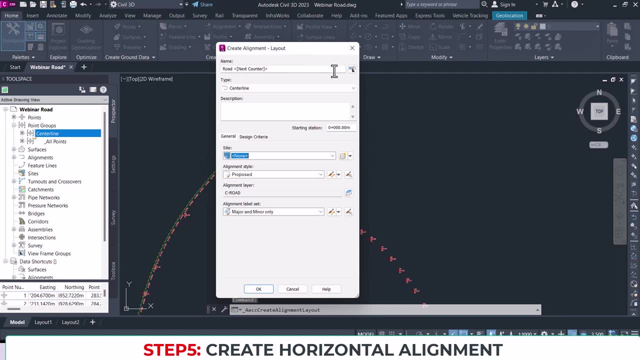 alignment creation tool again. so remember a good old template. it is going to save it as a rule to this time around, because the next counter is to. if you look at it here, you will see that it's also to here. but I'm not going to all. 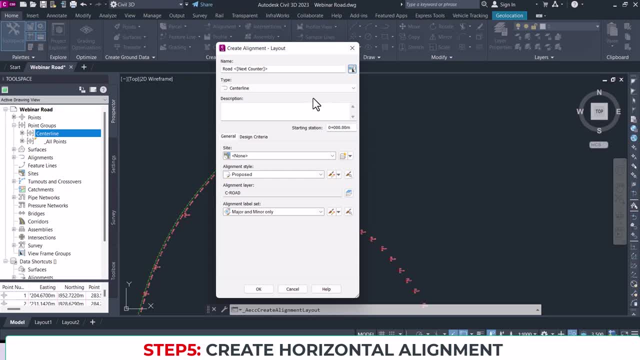 these things, you know. just just to show you how simple 3d automates things. all right, so let's go and put everything just as we selected before, then go to design criteria. now, this time around, I have my design speed to be 60 kilometer. 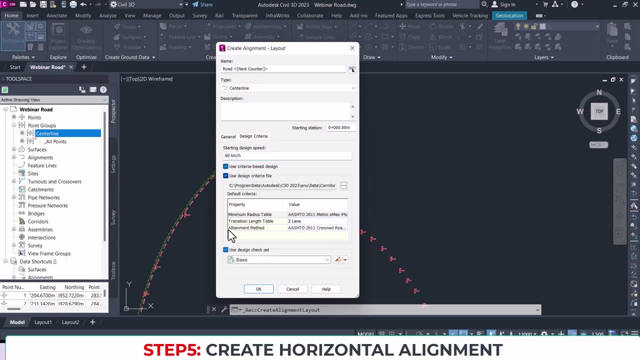 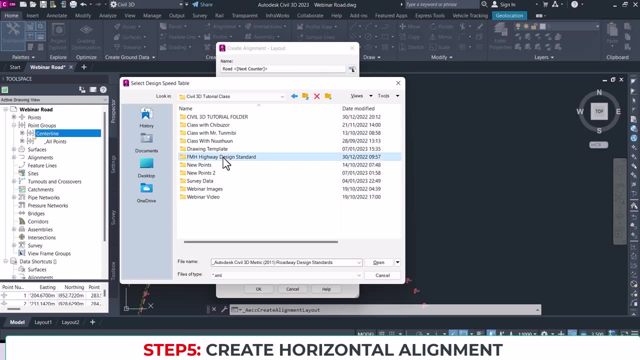 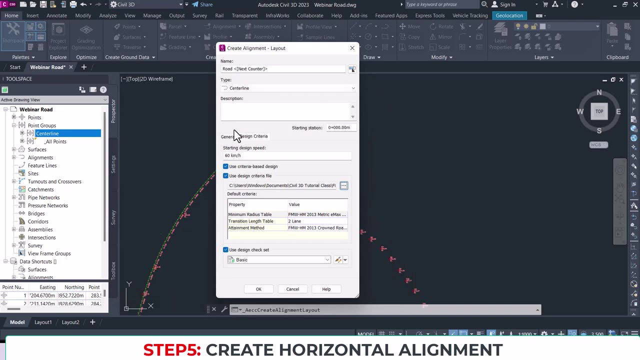 per hour. so let me use criteria based design, then I'll find where it is okay. let me browse to where my codes are. okay, I just selected it. okay, once I select it, it allows me to use the maximum spallation. in this case, it's maximum spallation with four percent. 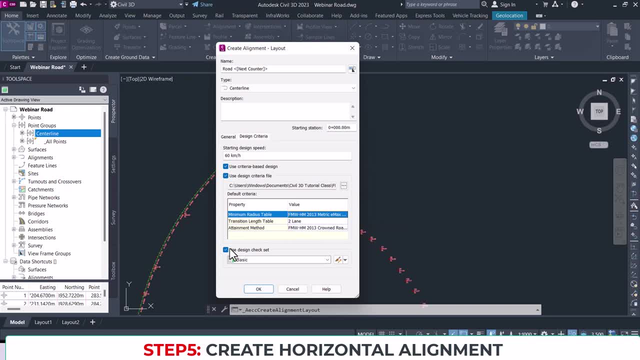 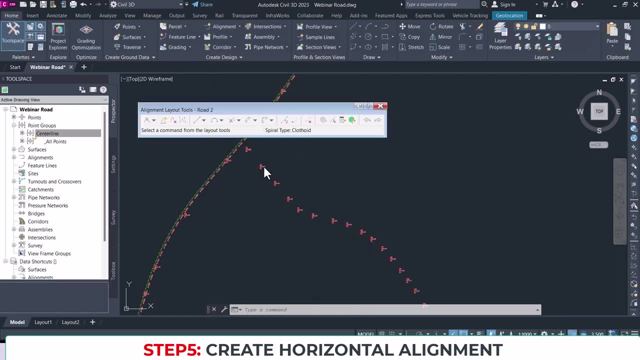 you know, for 60 kilometer per hour. you can check that in the design specification. so I'll uncheck this. so I press, ok, the same thing as I did in the previous one: I'll just look for a straight section and draw a line, okay, I. 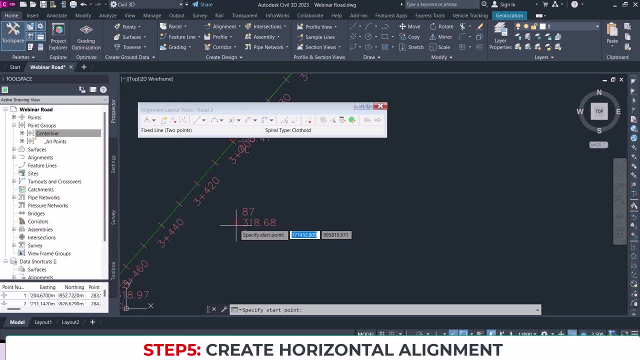 supposed to start from this intersection, but let me start here. I'll extend it later, okay, I'll just start here, okay, and then find the straight section. I think the straight section is going to be here and then I'm going to go to the end somewhere here. then I press enter, then find another straight section, okay. 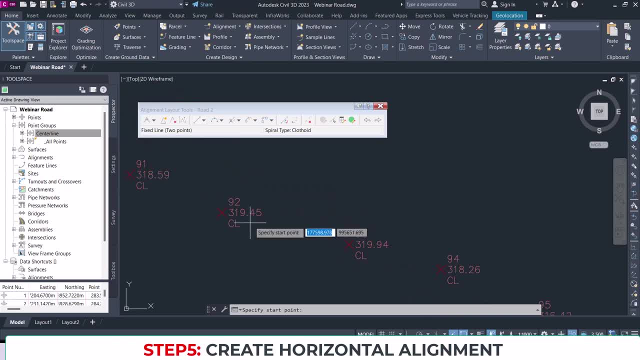 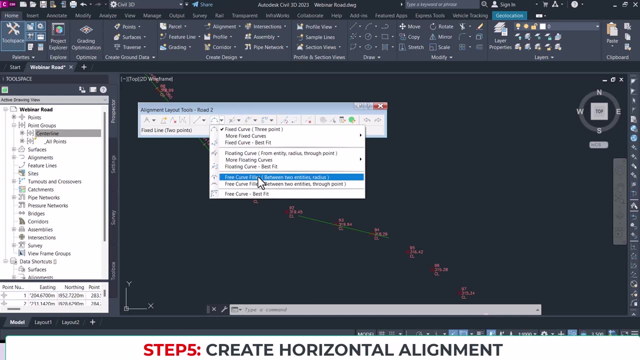 and then let's see from here. it doesn't hurt, I chose- and I'm making sure- just to draw something that passes through at least three points, okay, so yeah. so then I'll have to put in a curve, fillet curve, and then add radius: okay, is less than 180 PKG. interrupted here. so then I'll look into all of this. then I'm making sure there's nothing to do something that passes to at least three points. okay, yes, so then I will have to put in a curve, fillet curve and then other ages. okay, it's less than 180 PKG interrupted here. so then I'll look into all of this. 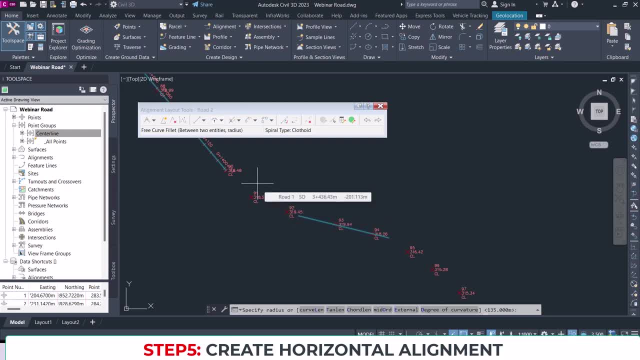 because I need. I can save lines if I need many lines running through these explained, then I will have enough bounding, but that's something I failed to do, so renew, and then we can use a radius of: let's say 400 is too much, so let's say 200. okay, that works. 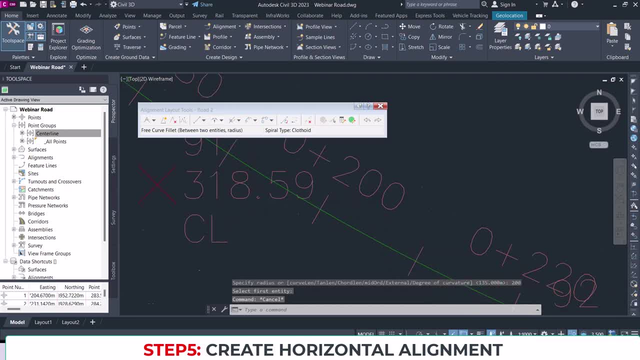 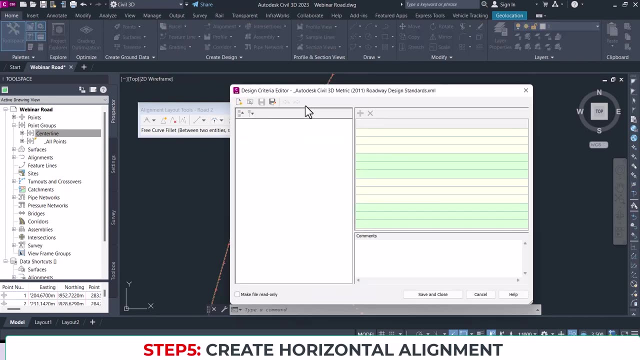 but is it within the design code? yes, because we don't have an error. okay, how do we know what is the minimum radius for a road of 60 kilometer per hour? you can find that on your design criteria editor. okay, you can just quickly check on that. well, it's still showing metrics. 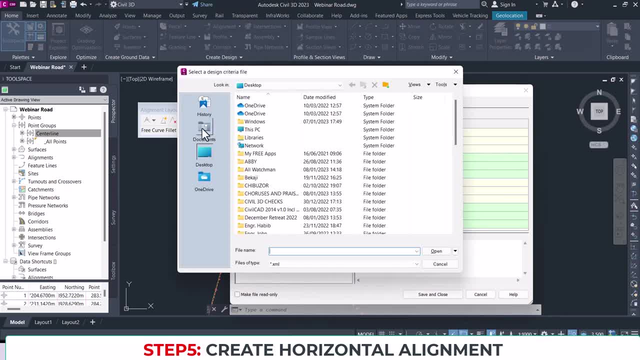 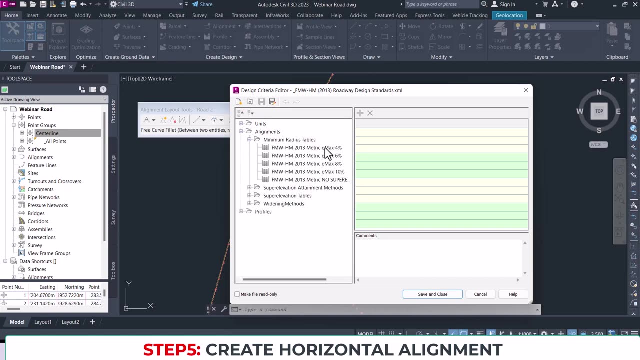 this rule. so let's let's quickly bring in our own here. and where is this okay? okay, if you look at it, on the minimum radius table for a 60 kilometer per hour, the minimum is 135. so, as you can see, we are within the 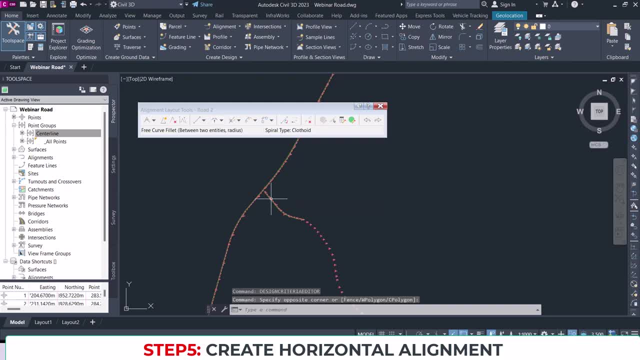 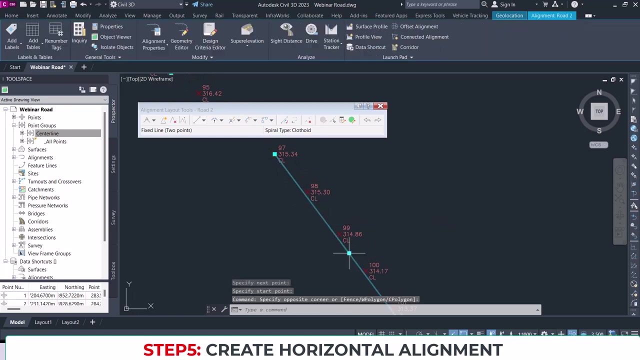 um, design, uh, you know specification, so let me just do that for another, another section. let me see, i think i have a straight section from here to here. okay, somewhere here, okay, i'm not, just i'm not going to, you know, be meticulously doing this thing. well, you know it looks like a tedious process, but i'm telling you once you do, 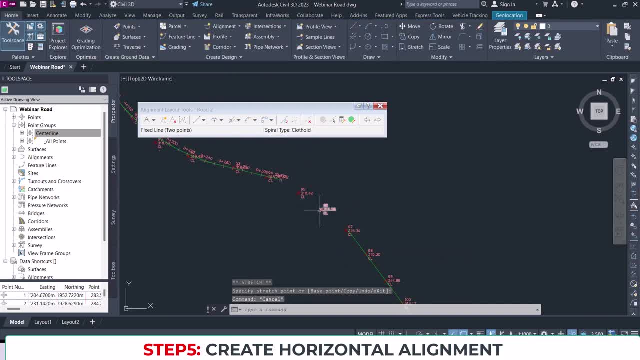 pass through all this process. you don't have to do much adjustments. you know there's a process of you using, you know, tangent tangents with curve. this is a popular way but I'm not going to use it because it's only when you have your PI's, your point of intersection, you know, given to you by the surveyors. you know. 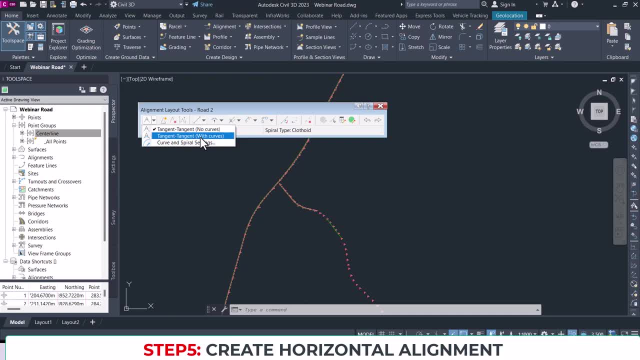 there's a surveyors that will do a standard work and propose the alignment for a strong. I mean when we have a real surveyor, you know, taking the data, he will even be proposing a, an alignment, so making the work easier for the engineer. so, but when we have just surveyors that takes the points randomly. 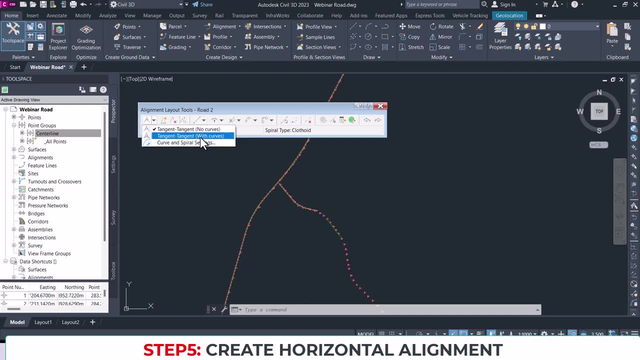 you wouldn't. you would have to do everything by yourself in the design. so- and that is luckily what I'm teaching you, because I do this constantly every day in my design processes- all right, so let me now add the cough. all right, so you are the call. 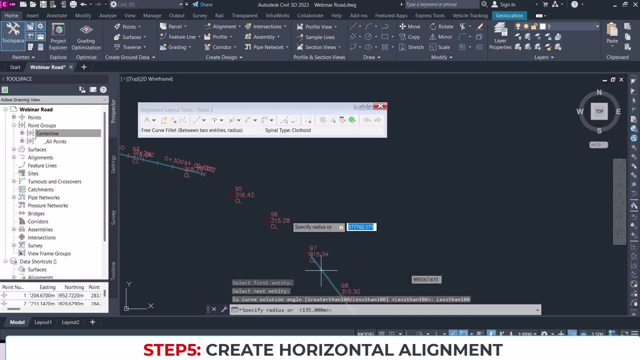 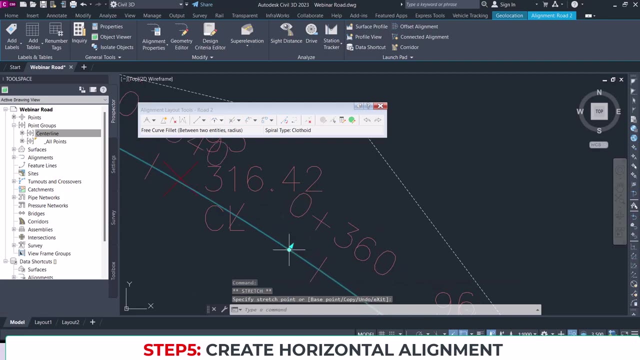 between between these two. okay, less than 180. let's take 200. okay, 200 seems to be working for us so far, but this one seems to need an adjustment. we can push it back. okay, as always, if you want to see the radius you have just done, now it. 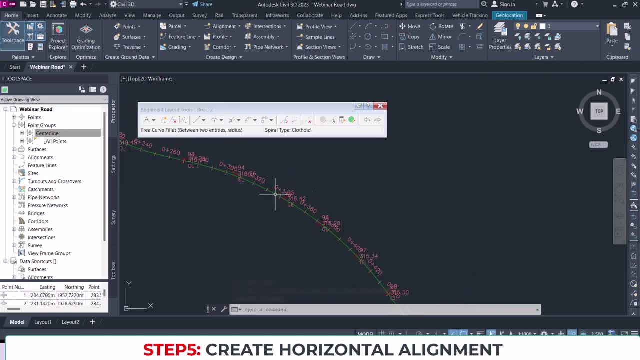 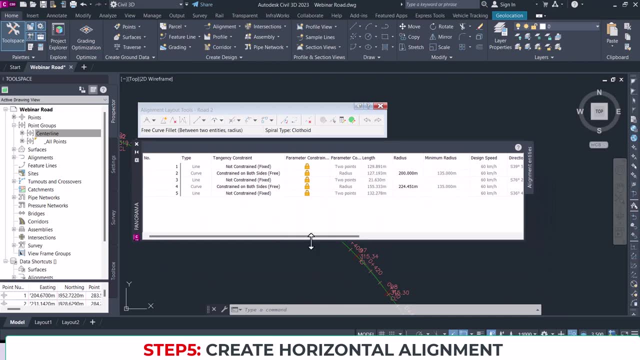 will show you here. you, you have to add a label for it. okay, once you add a label, you can be able to see it. or you can open up this: uh, wizard here, and then you will see that radius. I think the first one was 200, the second 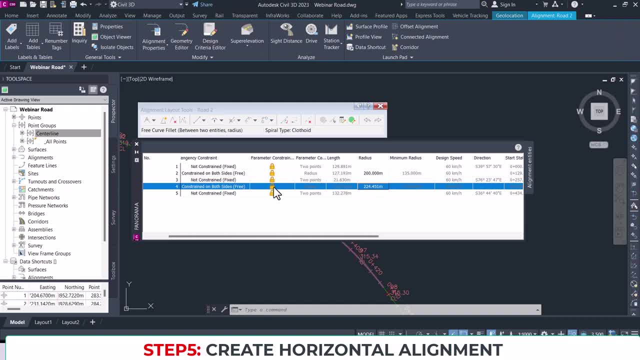 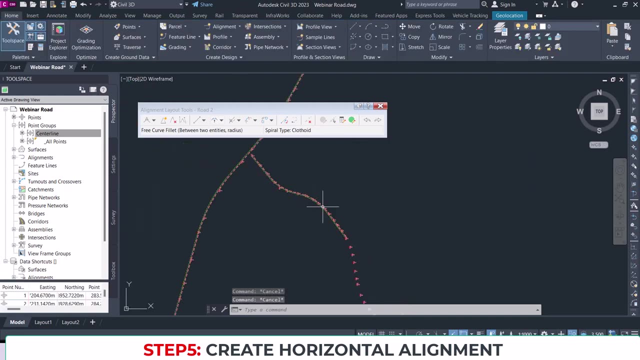 one is 224.7. if you want to make it a round figure, as usual, just unlock it and then let's, let's make it instead of 224, let's make it 225, just not to have any decimal point. okay, so once you do that, you, you can do that for the rest of the 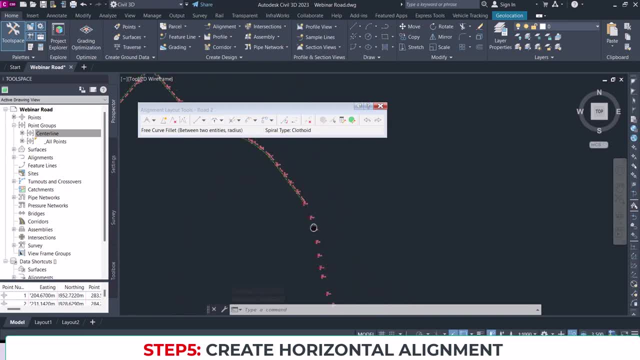 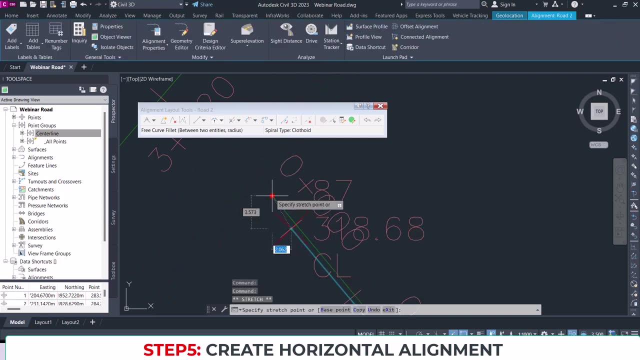 road, but in order to shorten this class, okay, uh, um, I will not do that for the remaining, I'll just leave it there. so back to this place where it's supposed to intersect. remember, I told you we have to make this road intersect, so I just have to stretch this. okay, pick this up and then stretch it, and making sure that. 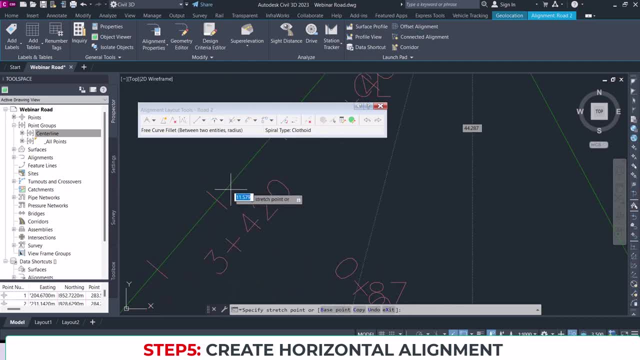 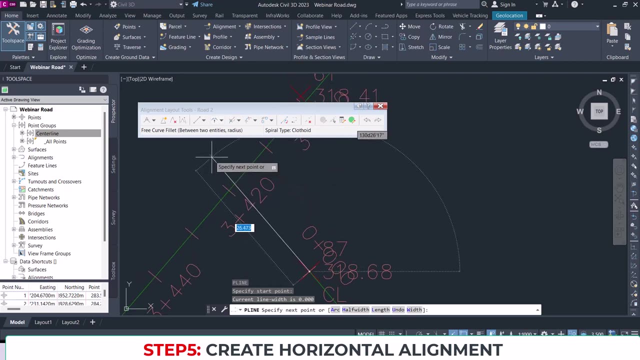 I'm in the same line. okay with um. okay, if that's not working. okay, there's a way I normally used to do it: I'll just draw a line, a poly line, just a PL, and then click from here and then allow it to intersect so I'm to move, and then drop it somewhere, so that I'll have. 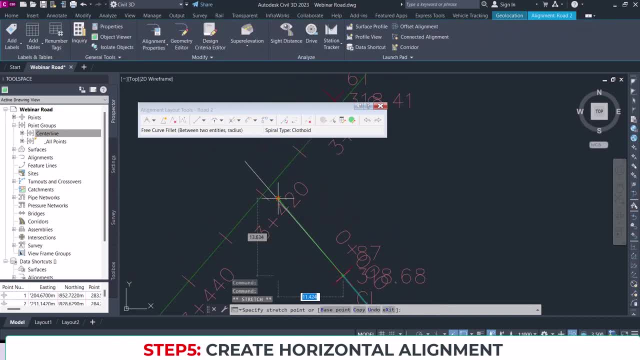 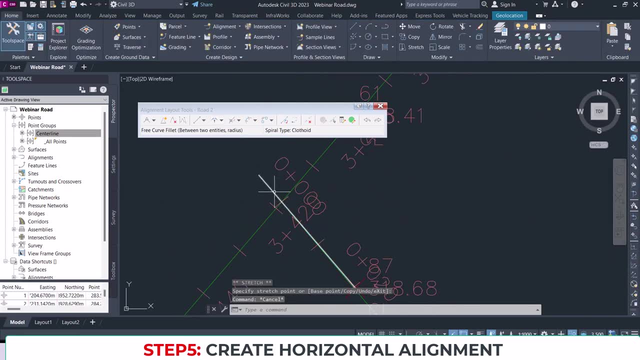 something to snap. okay, once I drag my alignment this time around, I can snap to where this to intersect- great, so then I can delete my holy line, okay, yeah, so I have to make sure you have a stretchy to intersect without interfering with, uh, the alignment. so great, that is it. 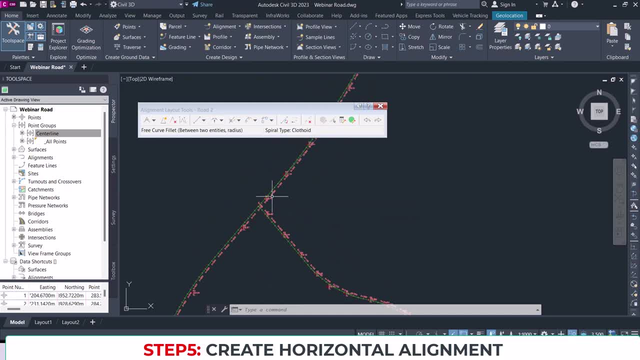 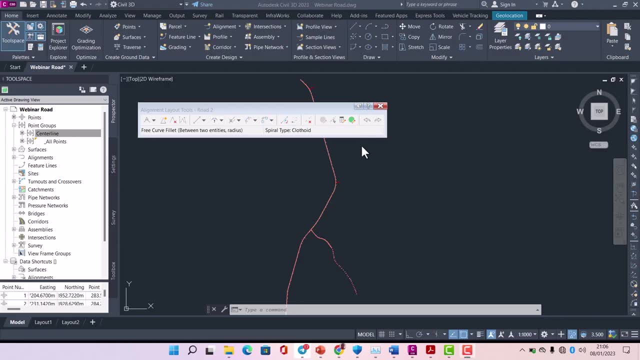 so we can now move on to creating our profiles. if we are satisfied with the alignments and completed everything, all right, so let's close this. okay, now we have to go to creating our profile, all right. so how to do that? just, uh, click any of the alignment and then this contextual ribbon. 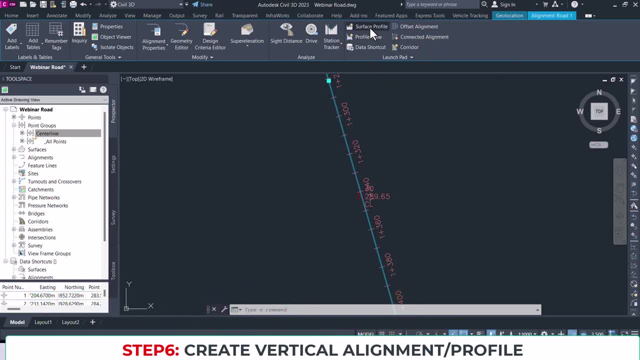 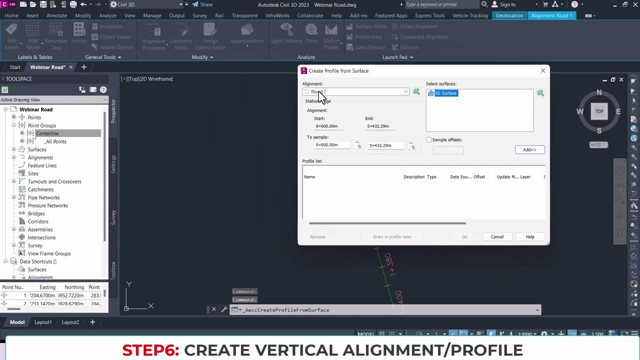 surface profile here. so just click on surface profile, okay, and then you will see that you have the alignment road, one which is this very road, and then you have to select a surface which is the existing ground surface, and then add it, and then it gives it a name. this name is not so good. 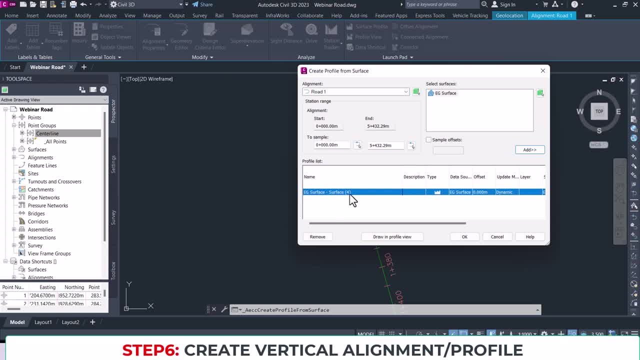 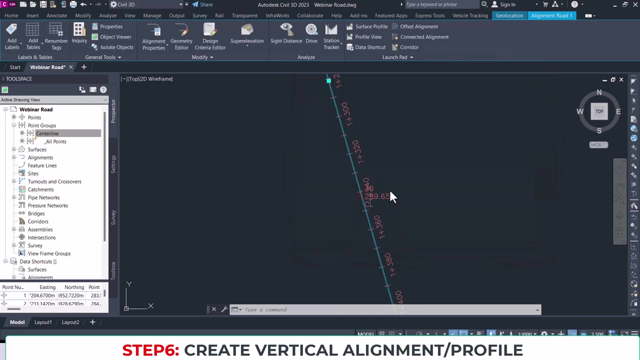 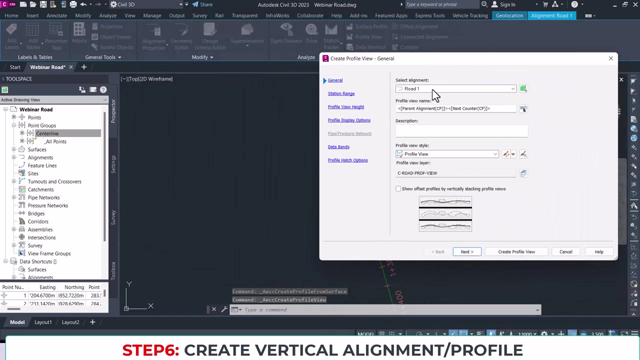 you can actually use, you know, adjust this naming system or however it's naming it. I don't like it. normally I used to create uh a, this template. okay, how it will name this thing. okay, this class. I cannot cover that. you can find a way to do that yourself, okay, so, uh, we draw in profile. okay, all right, so we have this uh road one. 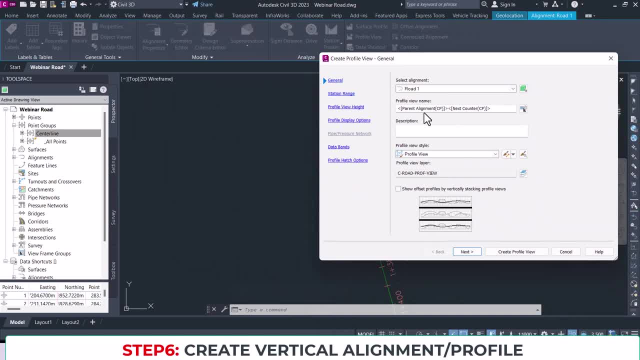 the alignments, you know all these things. let's leave it by default. but what this thing simply means- all this window, I mean, allows you to modify how the profile will look before you create it. okay, normally for me I'd have to just create it okay and then adjust anything I don't like, but let me. 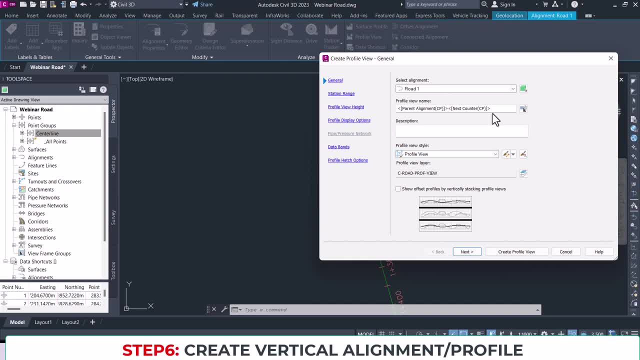 just walk you through all what you can do here so you can give it a name. okay, this is it's going is using a template here. okay, so we can just call it. uh, if you don't want to use that template, one profile view. okay, then add a description. if you want to, then the style. this controls how the profile. 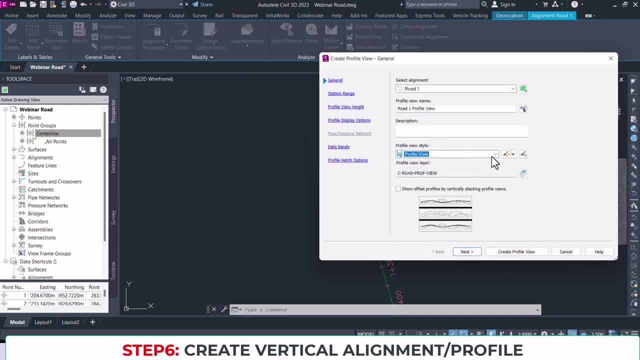 is going to look. so we are using a profile view style. we can actually create our own. yeah, so you go to station. okay, you see the station. this is showing you the length of the road, so you want to start from the beginning to the end. of course that's what you want, but 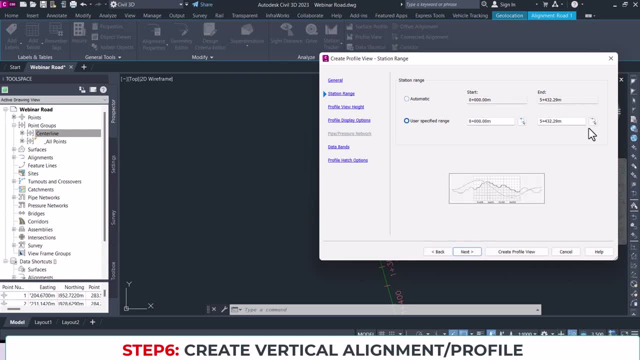 if you want to have a specified range, you can actually choose this and then add it range, but usually we want it for the entire length. so the profile view heights: okay, you will leave it as automatic. then the display options: um, these are things that you can always. 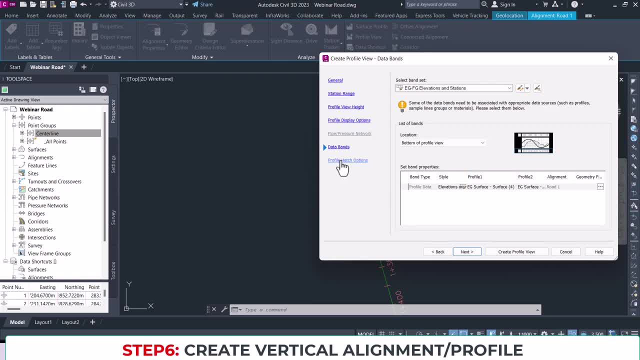 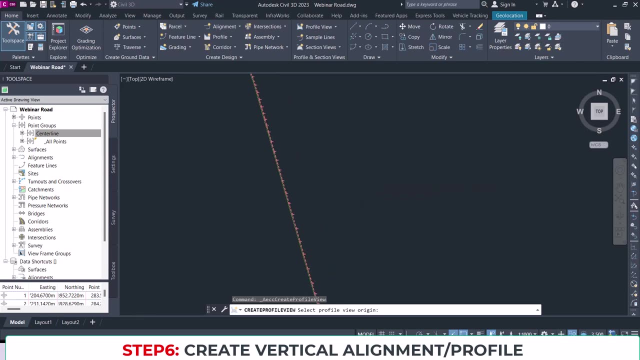 modify later when you create the profile, if you see that you have not found something that you are supposed to see. okay, you can always edit. so let's, let me just go down and then create this profile. leave everything by default, okay, so, because the default is exactly what you need. 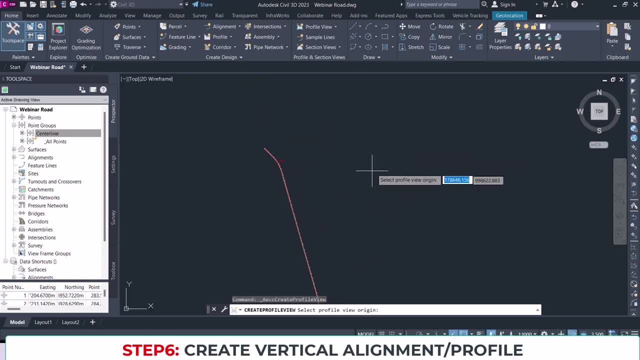 basically. so now this is: we are going to create the profile. we are going to find somewhere on our workspace. not go too far, but don't be too close so that you don't overlap on your alignment. okay, so let's find somewhere here, because it's going to create it to the top right. 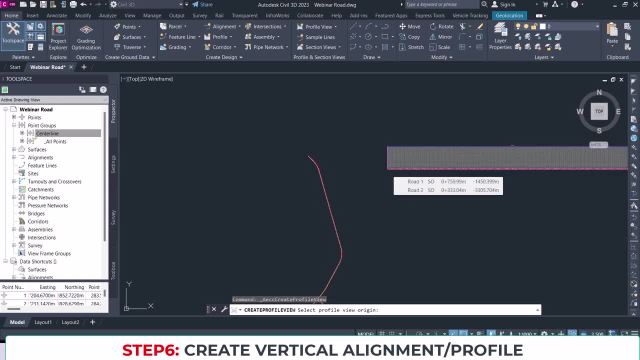 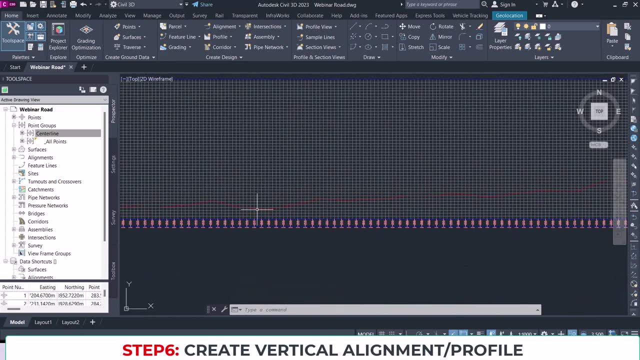 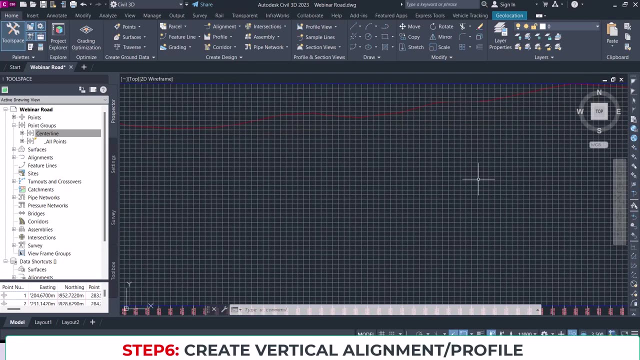 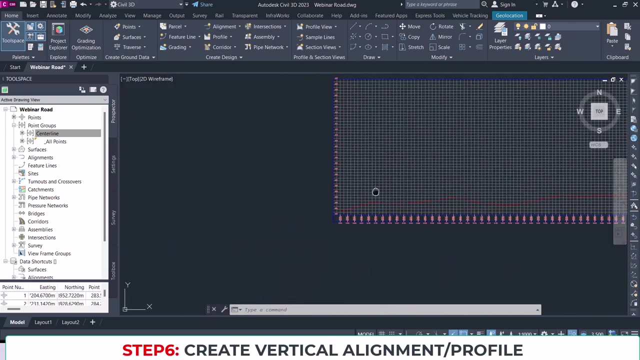 so just click here and then you'll find it here. so, if you can see, the red line is showing us our existing ground profile. okay, so now this uh grid, this vertical grid, looks quite noisy. okay, it's too bold. and it is looking too, you know, uh, too bold. 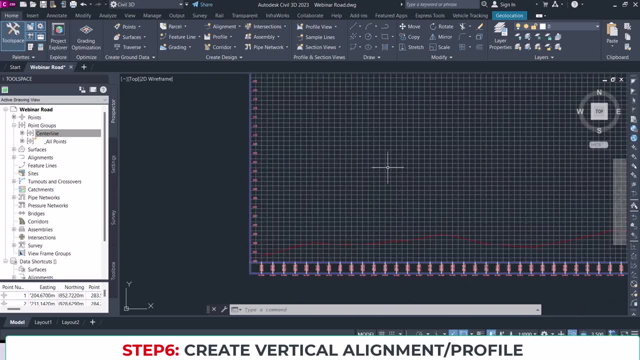 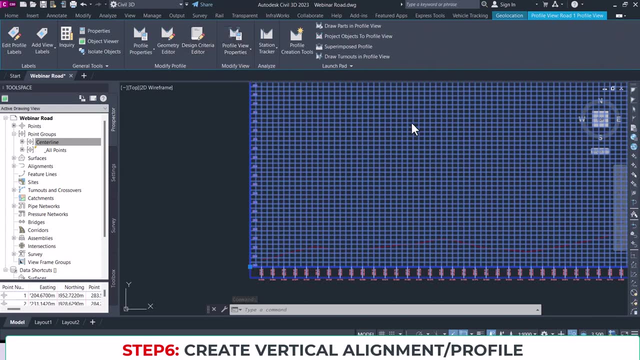 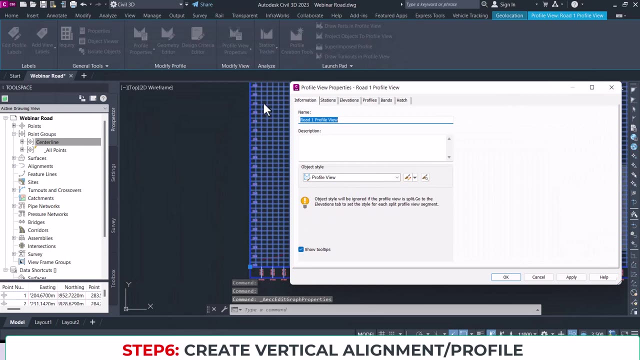 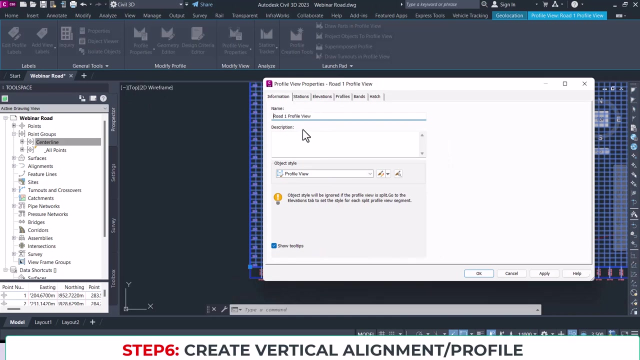 so we can actually adjust how it looks like. you can click on it and then on this ribbon here you can choose profile view properties. okay, once you choose that, it opens up this profile view properties, you can choose um how you want it to look like. okay, so remember the name we gave it on one profile view. all right, that's why you see it. 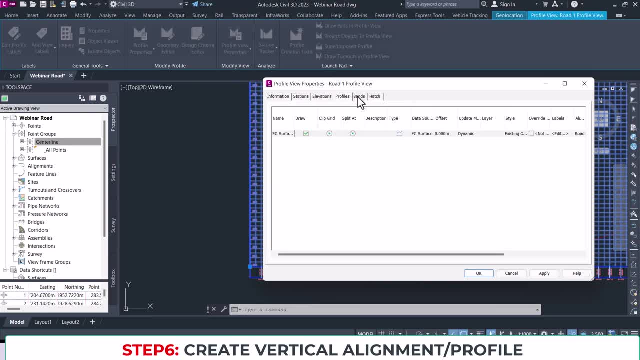 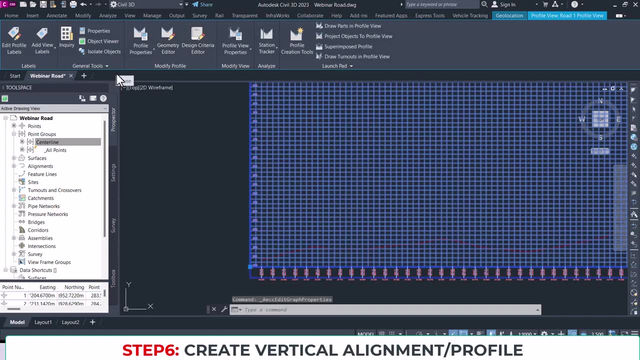 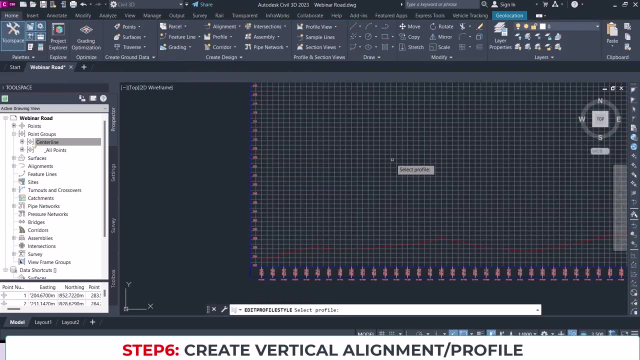 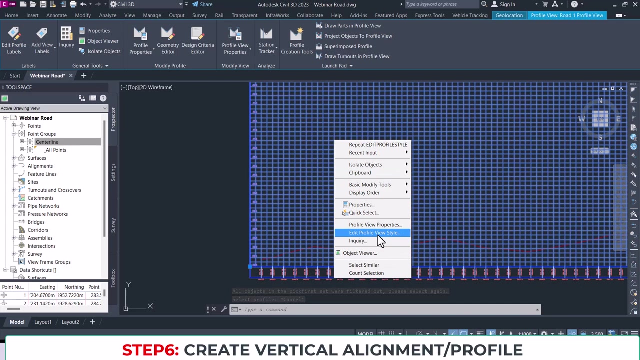 here, so the stations you can choose. um, okay, these are the bands. oh, not here, let's, let's use. let's use profile view style. okay, profile view style. okay, so select. oh, i mean, no, forget about that. let's just right click and then go to edit profile view style. 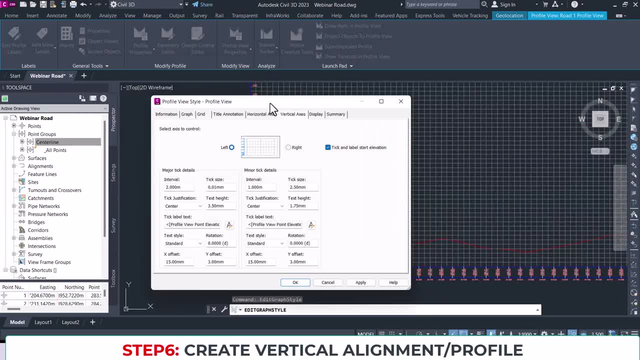 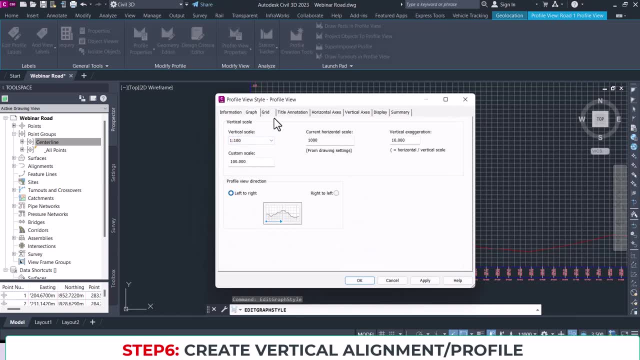 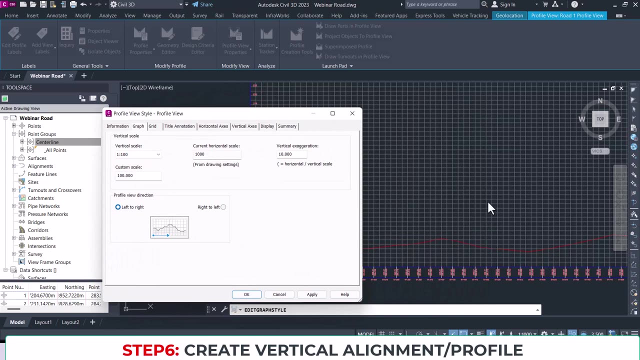 okay, it brings you this, so it allows you to select the grid you can add from the information. this is the profile view style. okay, you can customize everything here. this vertical acceleration shows you that this profile has been exaggerated by in the vertical, in the vertical direction, by times 10, which is always good for you to exaggerate your vertical. 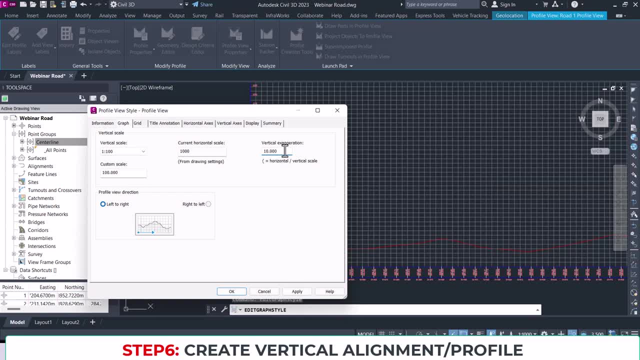 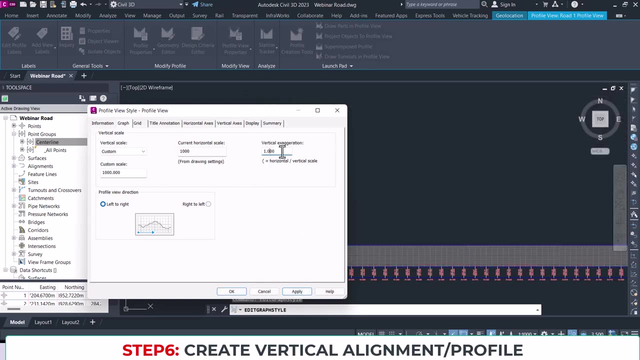 profile by by 10. okay, it allows you to see the ondulating nature of the road properly, because if you put it by one, the road will be relatively flat. let me just do that and show you. everything will just look flat. but that's not what you want. you want it to be exaggerated by 10. so 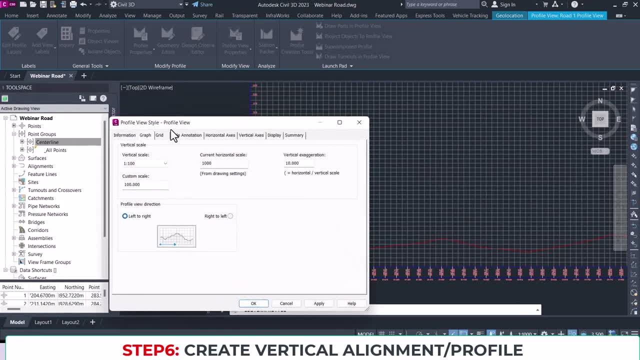 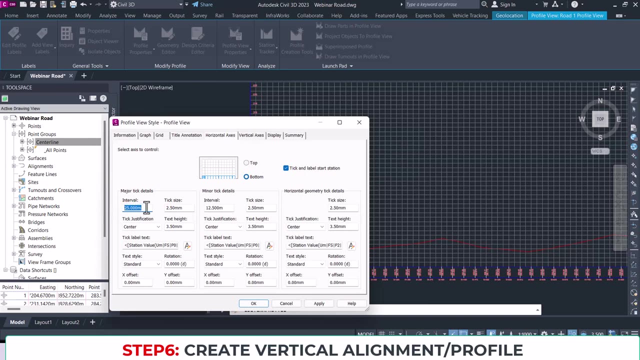 that you can. you can see clearly. now i'll break this down a little bit, but just to let you know, on on the grid, you can. there are so many options here. okay, i'm not going to go through everything, okay, but what is important here is in the horizontal axis. i okay, mine is a good, it's a 25. 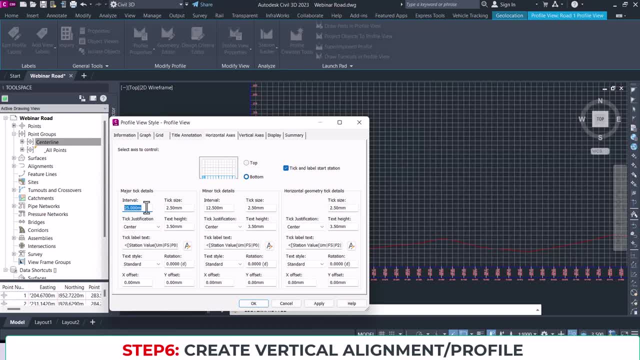 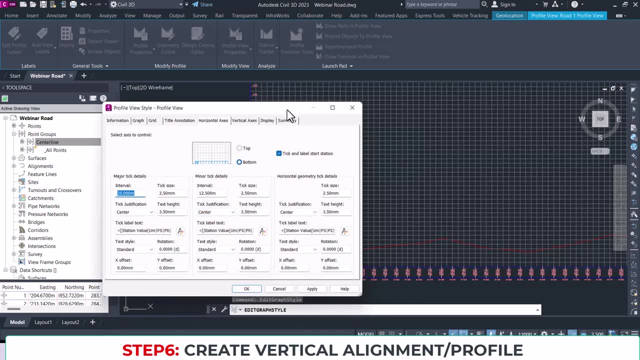 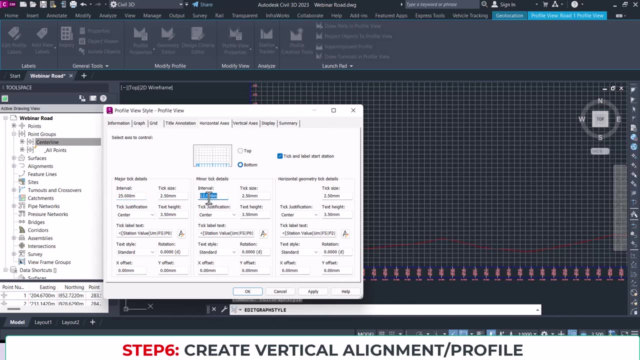 percent interval. so my change is is at 25- uh sorry, not percent. 25 meters, okay, so i'm working on a change of intervals of 25 meters. that's what you have here. then the intervals having the intervals is 12.5, so the major stations is 25 and the intervals is 2.5. that's exactly what i need. so 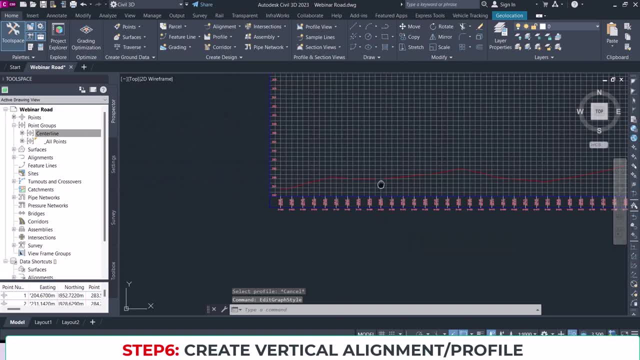 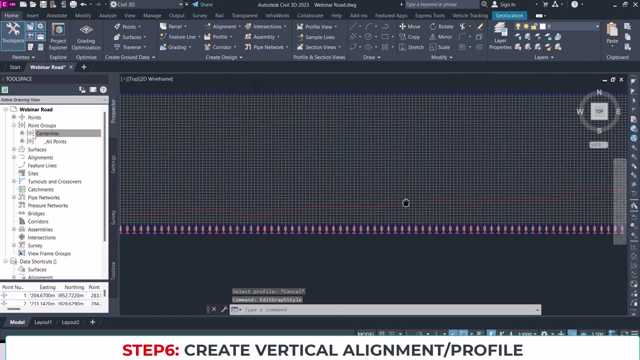 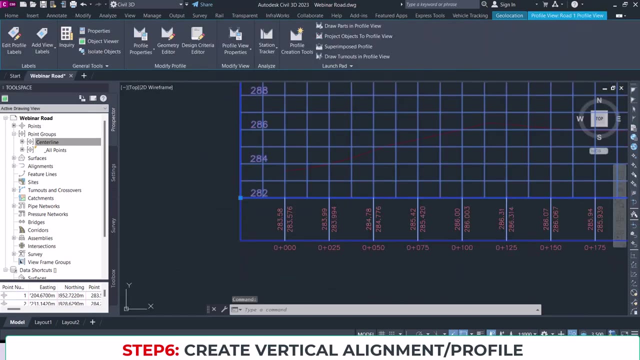 you can see that here already. it happens to be here by default because i've been working with the the file. okay, so if it's not so, you can just adjust it to whatever you. some people use, uh, major stations- 20 meters intervals, so you can change that. okay, let's change that to 20 meters. 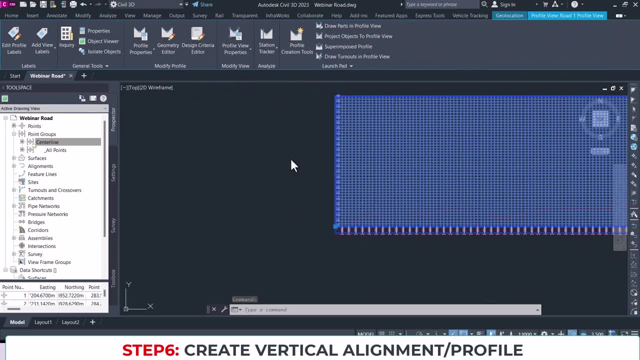 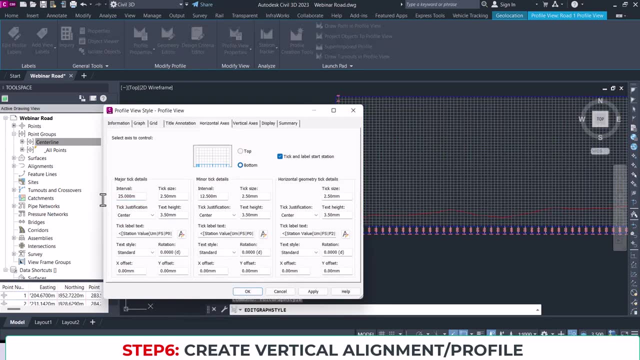 so you appreciate the class better. so you go back there to the profile view style. let's change it to 20 meters, 20 meters interval, 20 meters interval and then 10 meters. so 20 meters major station and then the 10 meters minus station. of course, let's apply. 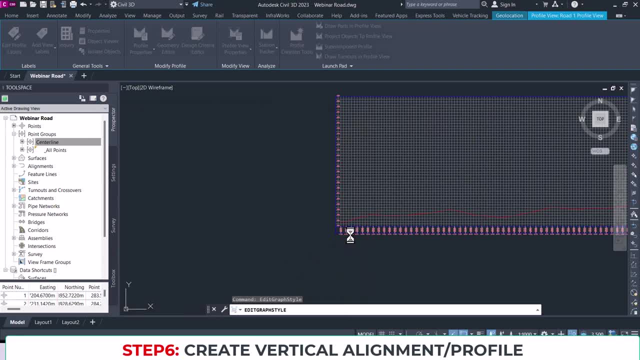 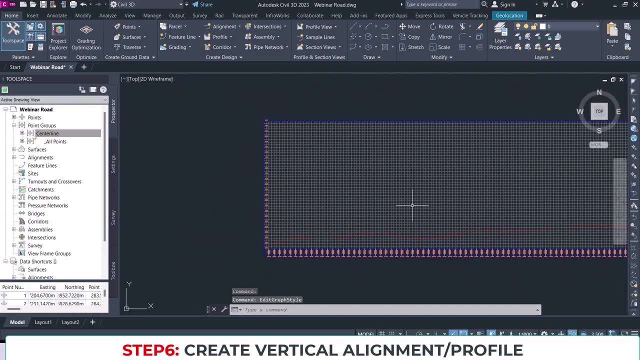 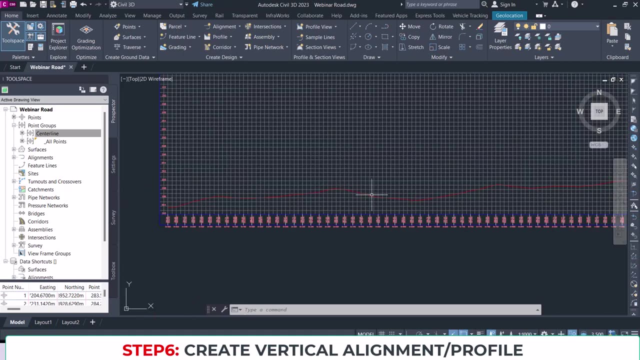 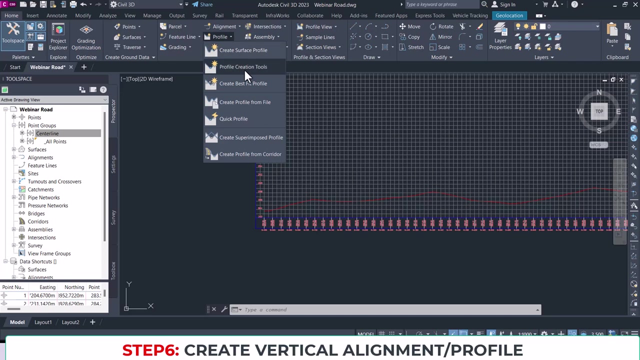 that, okay, as you can see. as you can see, it changes here automatically at 20 meters in covers. so that's great, all right. so let's proceed, um, to creating the design profile. this is our existing ground profile. let's create the design profile. so let's go on to profiles and then profile creation. 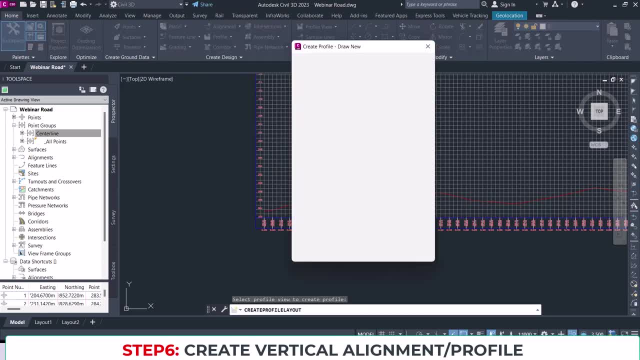 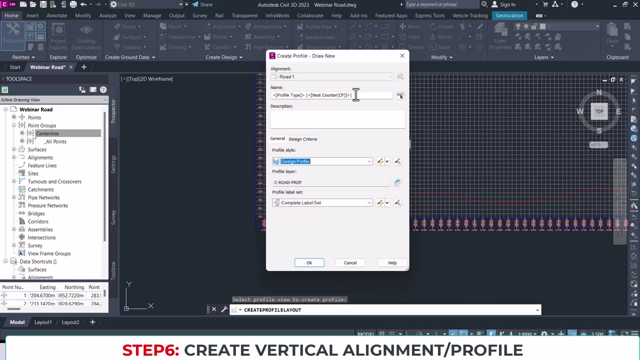 tools so you select anywhere on the grid. let's click on the profile. choose data only chapter 2 and' y, acid meat. it allows you to you know name. it opens up this ribbon allowing you to name your profile. let's say one once profile. okay again, you can create a template that allows you to you know. 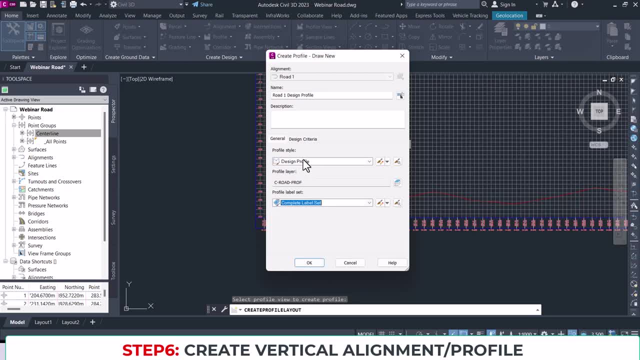 name it the way you want. so let's proceed, uh, to the and select the profile style. okay, and also we'll select the label styles. okay, and let's just leave it FisherPlan default here. the design profile completely set here. then on the design criteria, again you go. 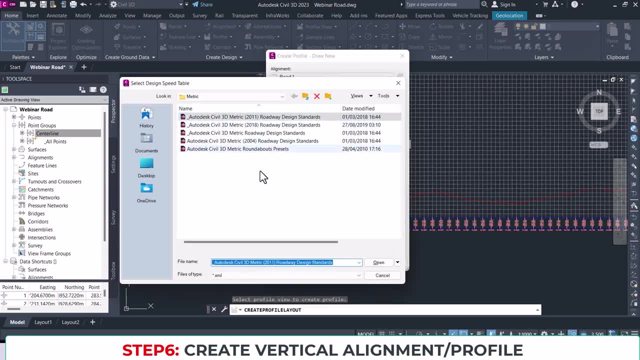 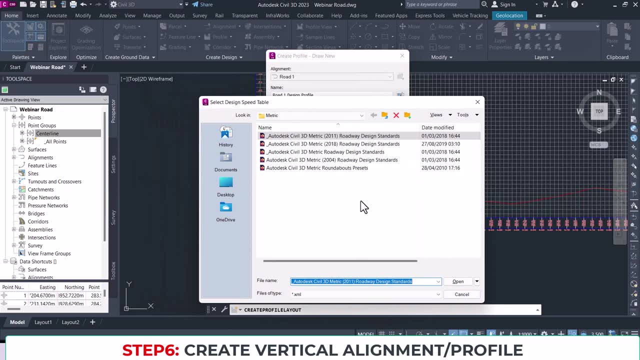 back to import your design codes now. if i wish, i would have just saved that design code here so that cv3d always sends you to a particular folder by default. so if i bring that my code here next time i don't have to start browsing through. okay, i don't have to start browsing through to find. 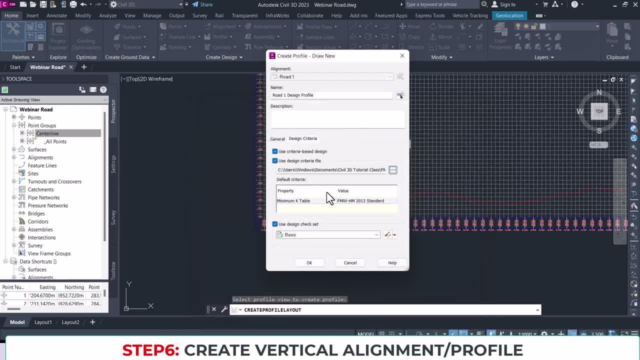 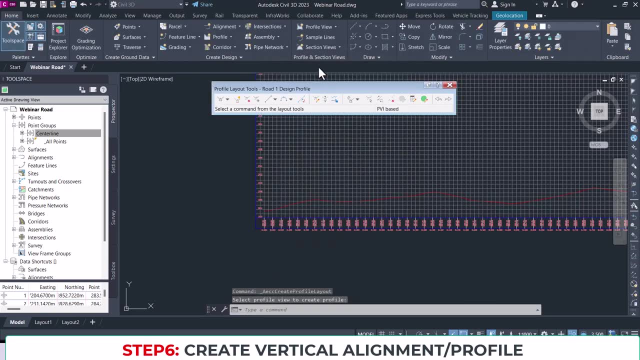 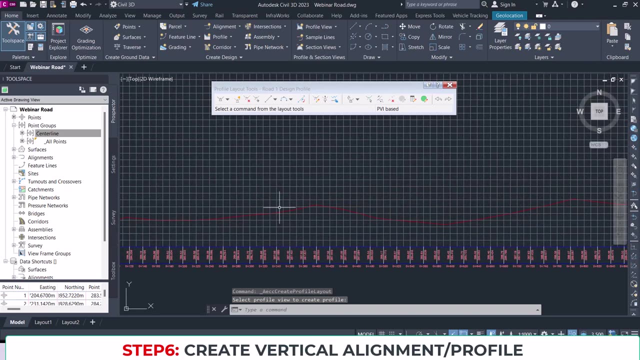 where i've kept it. okay, that's very important, so let me uncheck this. okay, so it opens up that ribbon, just like the alignment, you can create alignment, create it with straight. you find a place that is relatively straight and then draw a straight line. now, if i were to design this road, 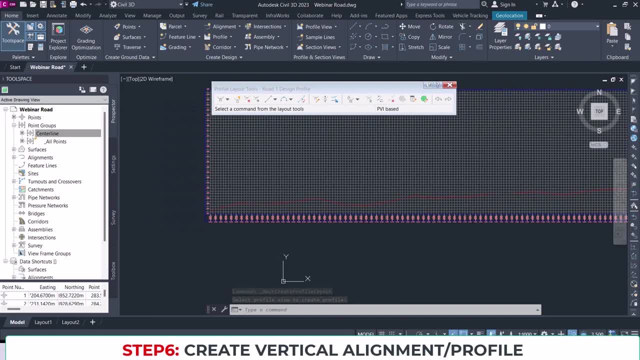 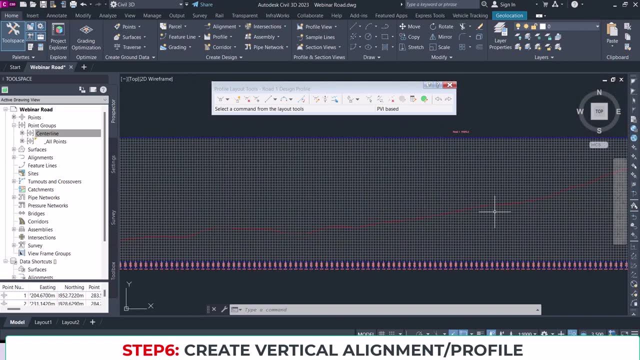 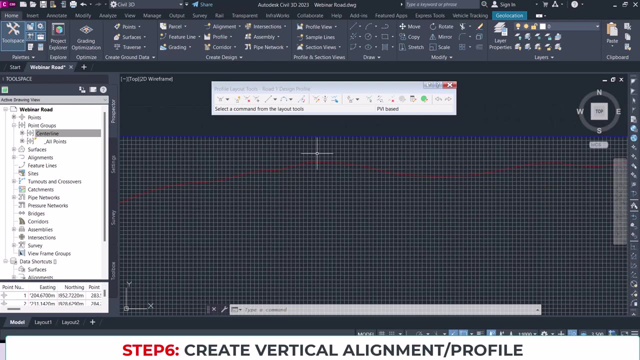 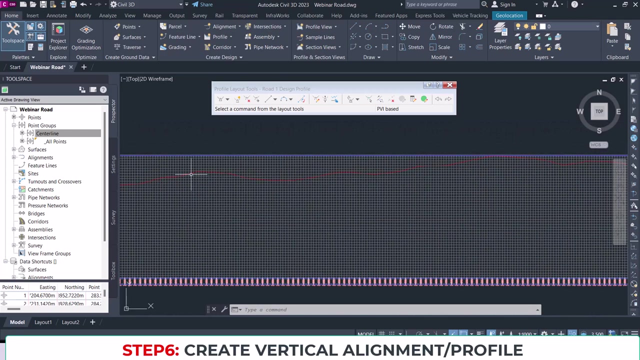 of course you have to study the profile first, and then, after studying this profile, i find out that i can just go straight from here all the way to here and then have a curve that will take me to this hill, and then i reach this crest here and then i have the high point, you know pi here, and then maybe go down a little or no, or just. 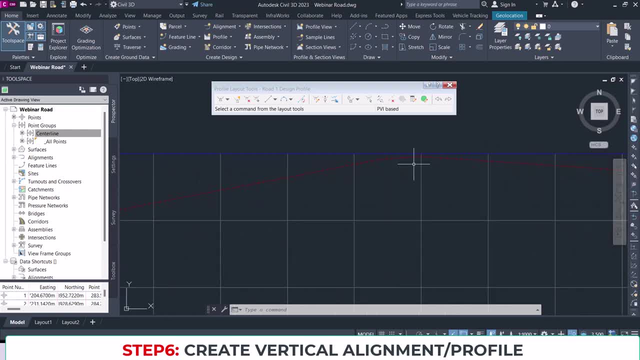 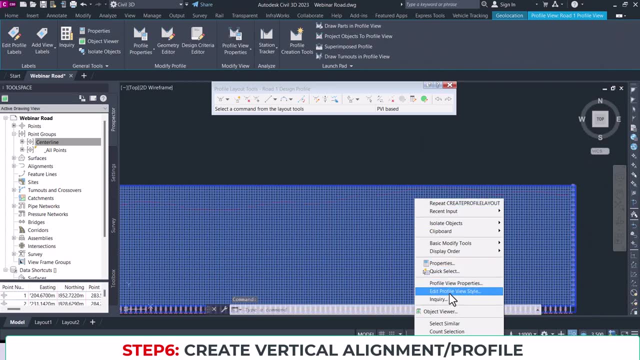 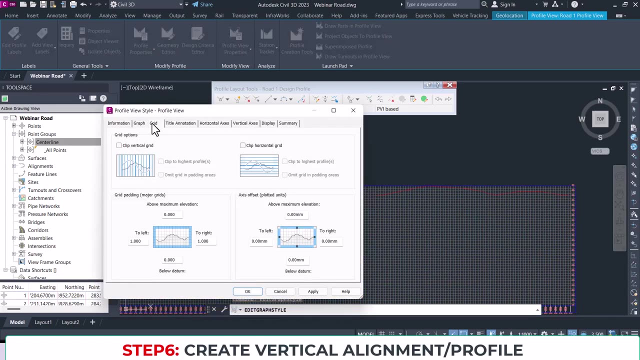 keep going high. now look at this roof. this place is quite close. there's no allowance here. i can adjust that on my profile view style. okay, right click and then go to profile view style. okay, it opens up. i go to my bridge. okay, and then above maximum elevation, let me have like two meters. 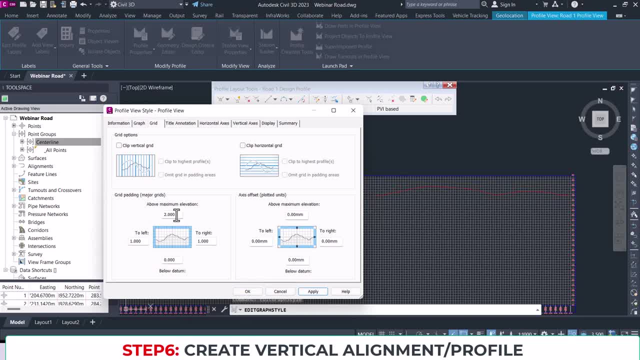 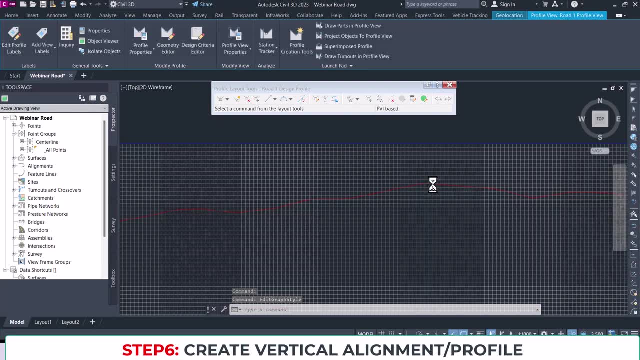 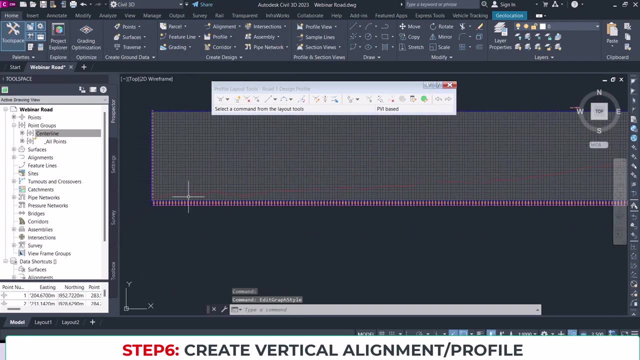 above that and apply: okay, let me make it five more. okay, as you can see, i have more room here, so that it's not just to not prevent me from adding a pi higher than that. so let's now proceed. i'm going to use: uh, let me do my. 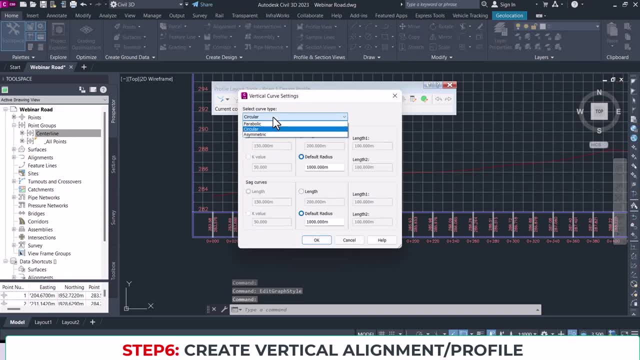 curve settings. okay, i'm using a circular curve. okay, so i'll use parabolic curves. parabolic curves is ideal, okay, but uh, circular course is easier to construct. i think i've made a post regarding that on my linkedin profile, so if you're not following me on linkedin yet, you can kindly do that, so you. 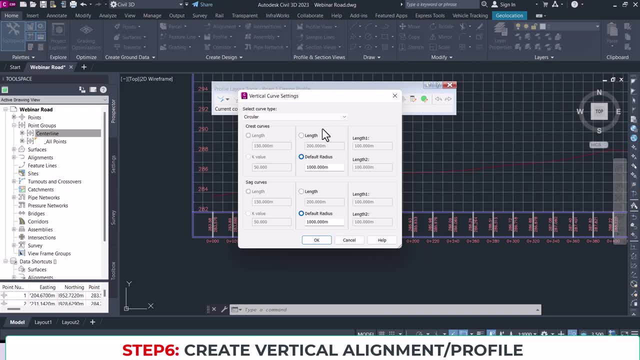 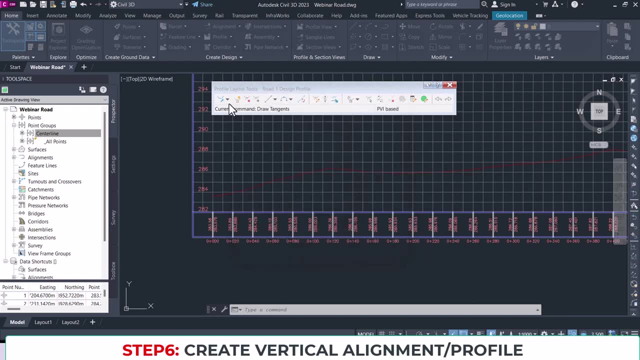 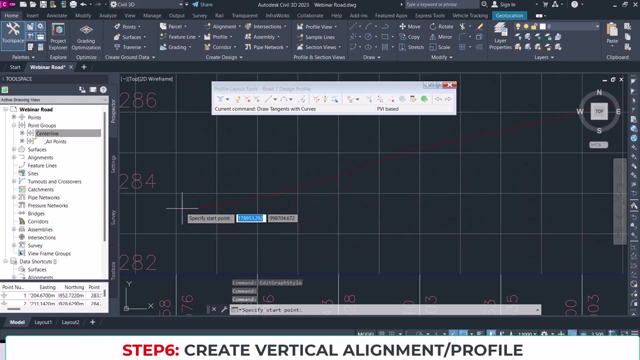 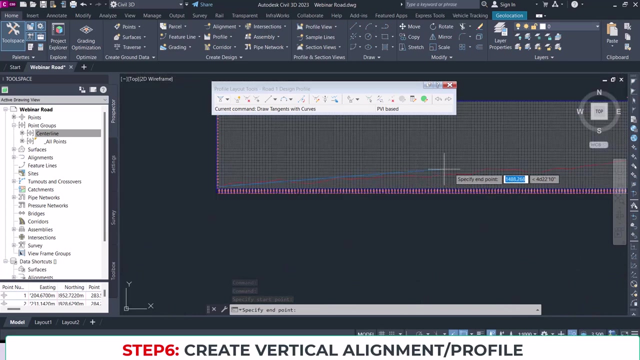 can find me when i make posts or comments regarding road design. so let me put the default ranges of 1000, okay, but for christmas, okay. once you do that, you can now select. uh, draw tangent, with course, okay. so now, assuming i want to start exactly from here, then i pick it up, then i, as i told you, if this were me, i would just go. 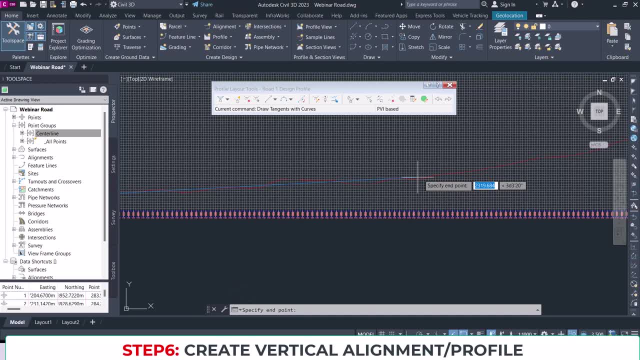 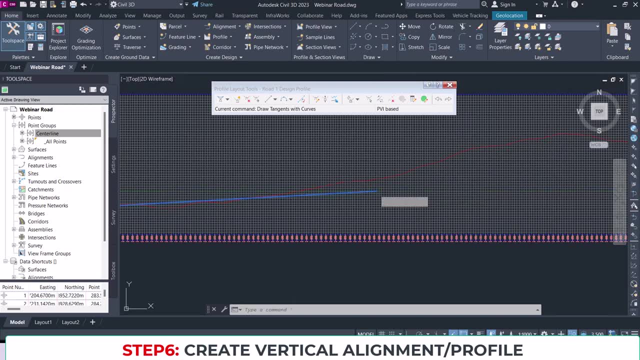 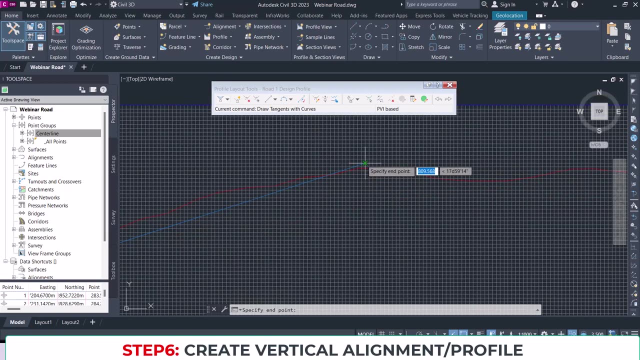 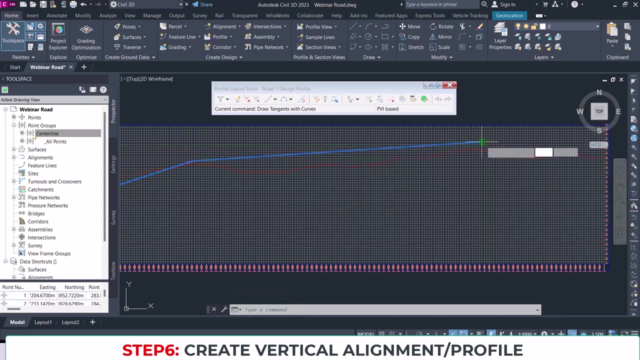 straight, okay, all the way, and then level all this place, level on this place, then find somewhere here and have my pi, okay, and then i'll go up the hill, okay, and then drop my pi somewhere here and then keep going up, probably drop my pi somewhere here. now i have a large field. okay, that may not be economical, but i 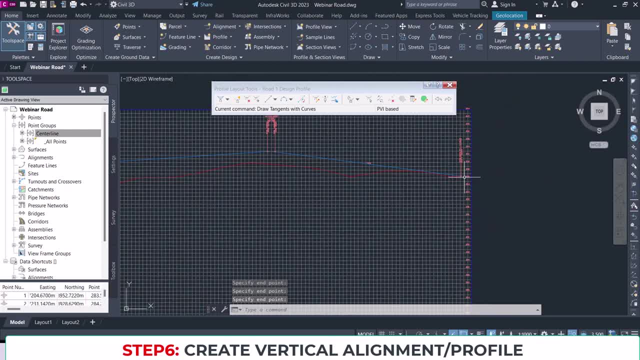 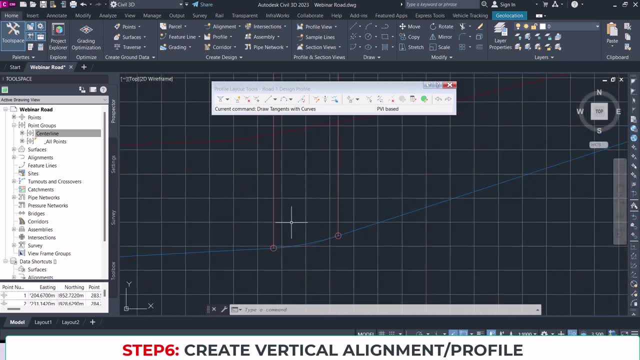 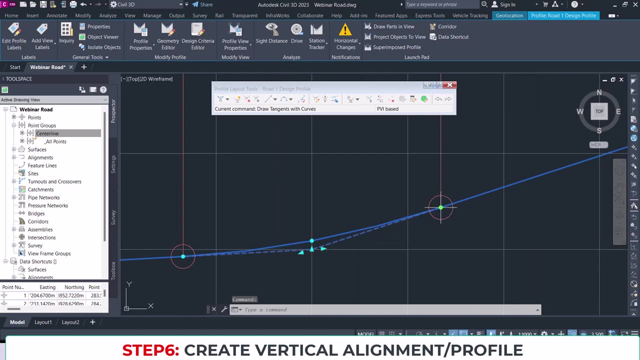 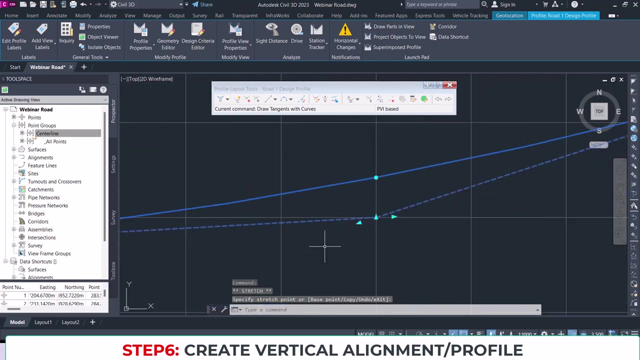 can adjust this later. so once i'm done, i press enter. i basically put my proposed- you know, you know profile, but i can always adjust it like. this curve is, of course, to small, okay, then you can just drag this and then increase it, okay, or you can just use this: 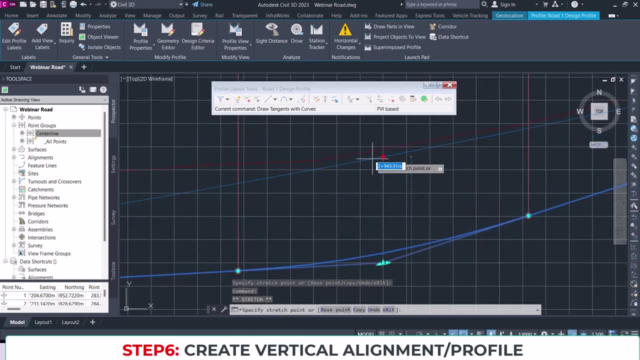 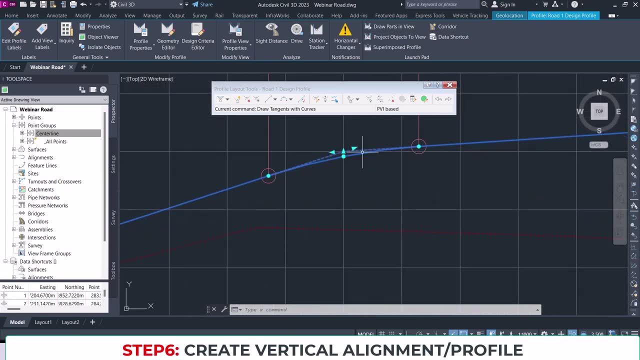 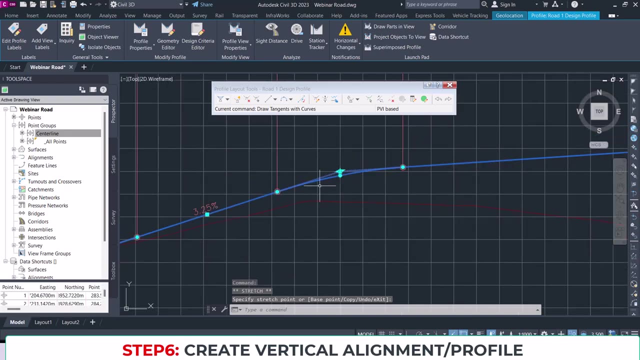 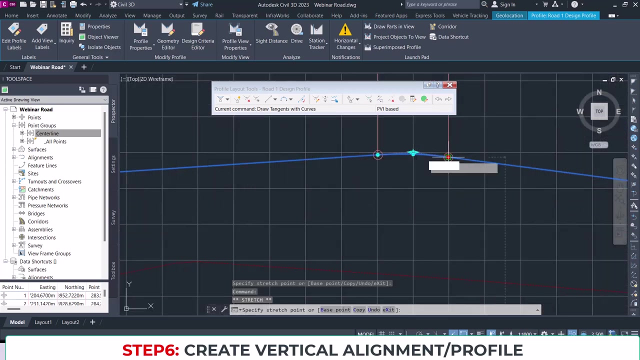 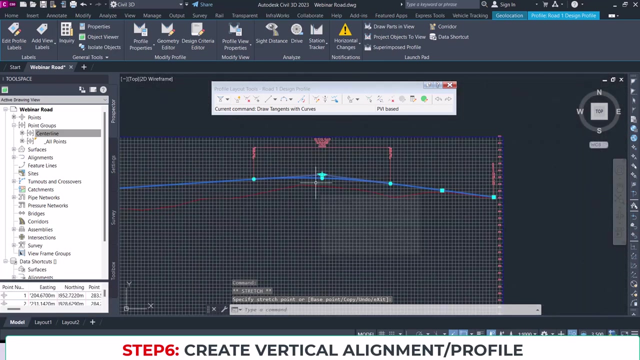 button here and then increase it up to here. okay, yeah, now this place looks quite small, okay, all right, so for the purpose of this class, i'm not going to go deep into all these. you know things, but you can adjust this thing continually, just like you saw me. so what's doing on my profile? okay, and then until you find a profile that is. 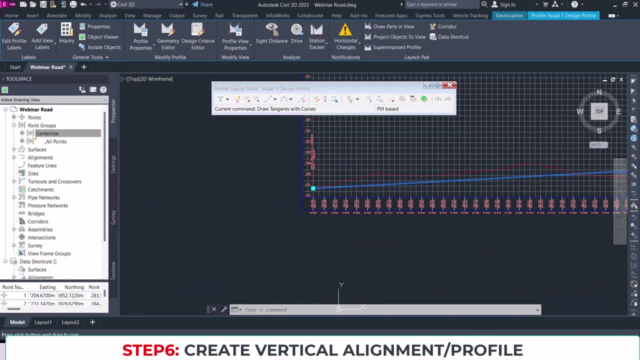 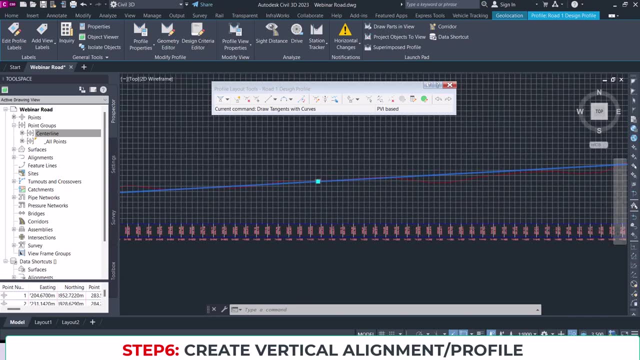 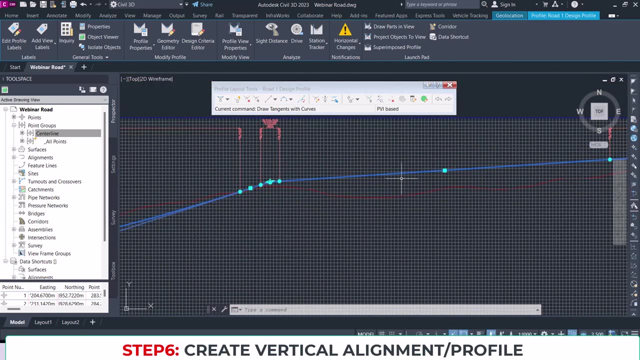 suitable for you. okay, like here: now i have some cuts. here i'll be having some figure, then i'll be having some. uh, just like that. you can just go like this and i'm gonna rotate it ó keep adjusting this until you get what you want. so for the policy class, let me just stop here. 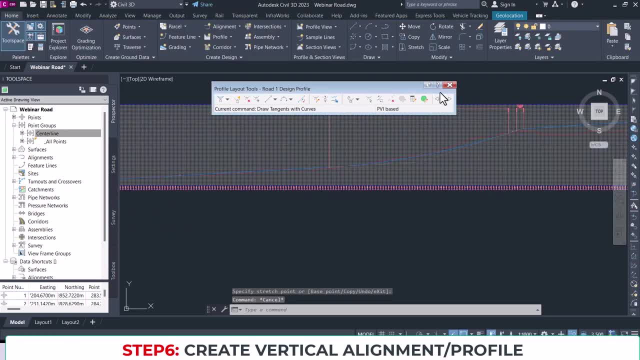 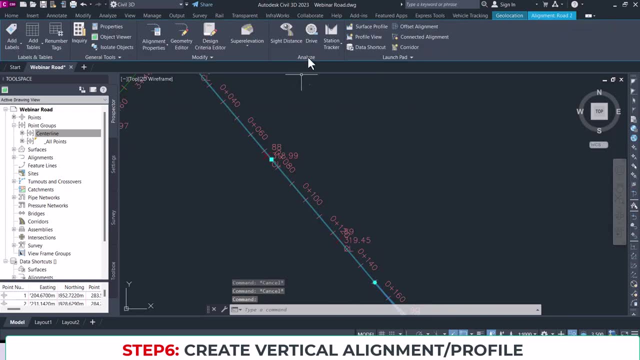 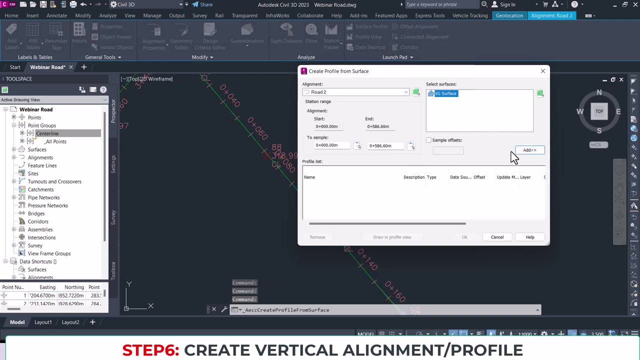 editing the thing here, okay, so let me close this. so i'm done with this road one. let's go to route two. so the same thing. you click on this and then you create surface profile. okay, then you just add the surface and then draw in profile view. when you draw a profile view, you go to: 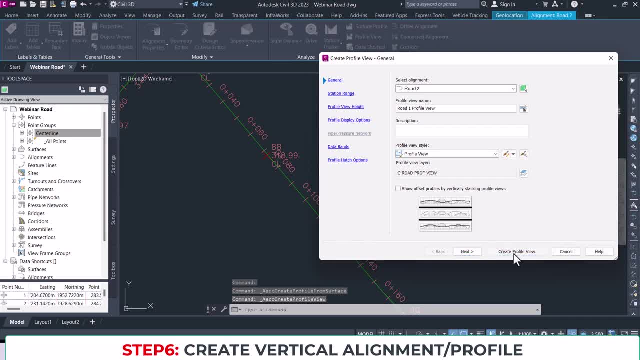 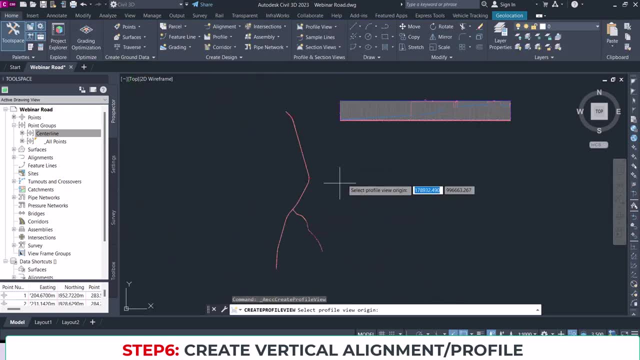 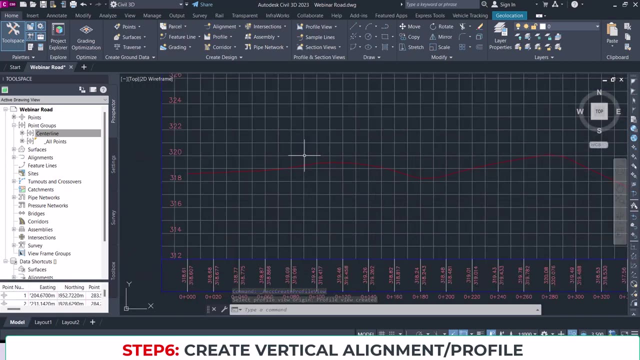 leave everything by default here, just like the previous time. then create profile view. all right, so once you've done that, you can now just click it. find it somewhere here. okay, this is the existing graph profile for the road tool. so we go to design the road. so profile creation tool. 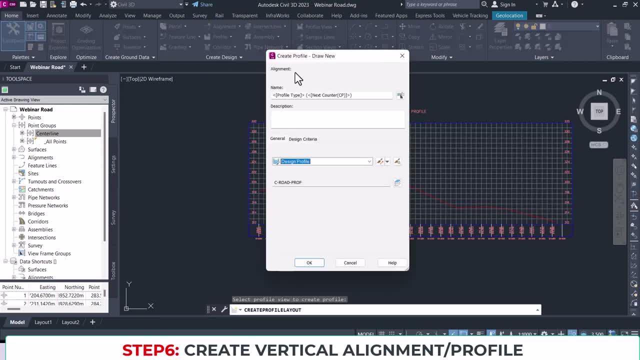 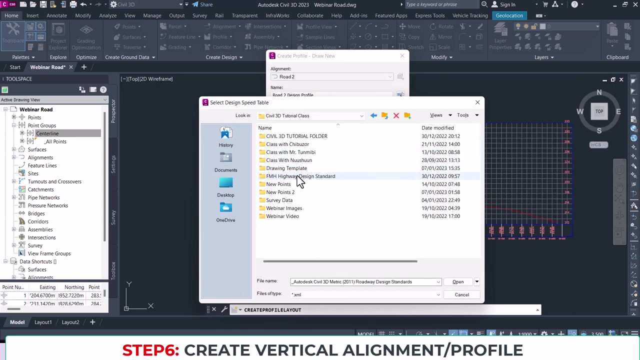 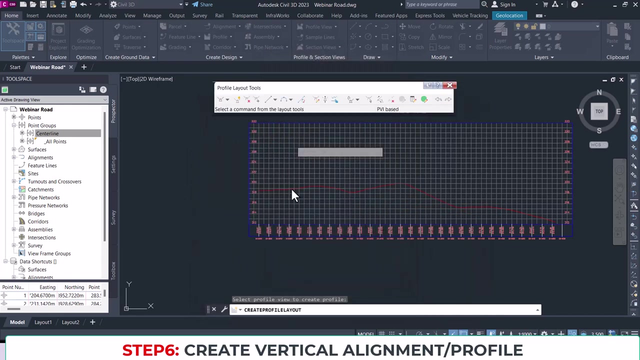 we select it, okay, and then populate everything here. let's give it a name to design profile. okay. then we use our criteria based design. again, we have to import it. okay, let's go through here and save this, then open it up, okay. so then i press ok again. if i see this profile now. uh, after studying this profile, i found out that 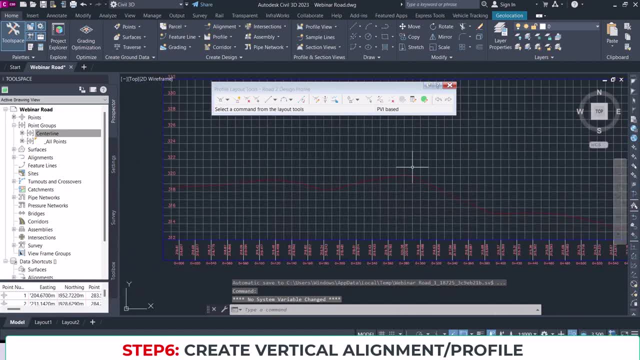 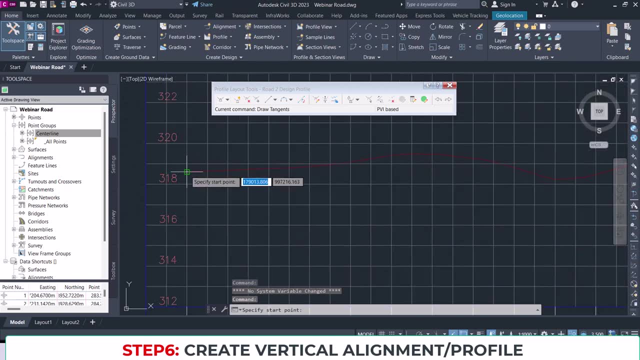 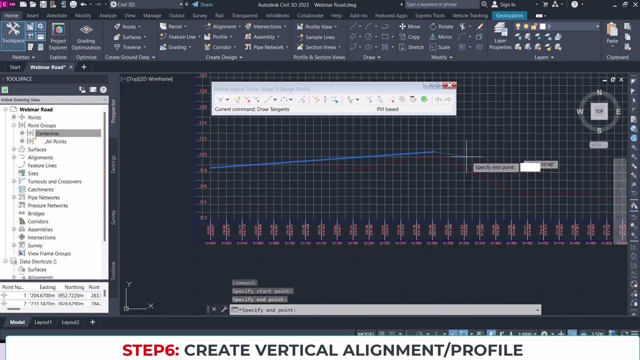 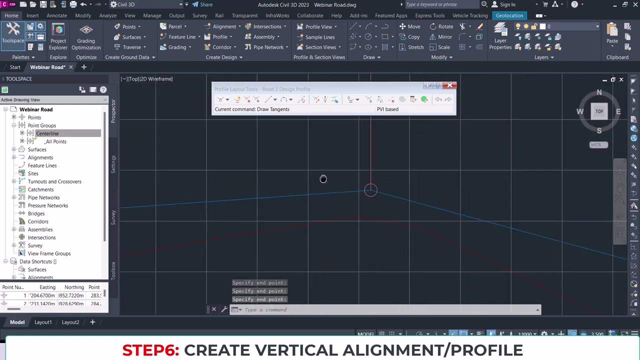 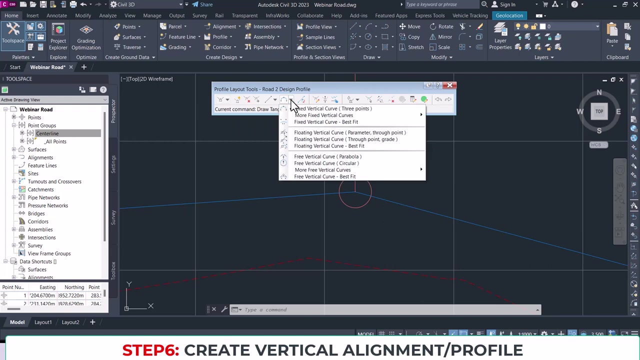 i can just have a straight up from here up to here and then down to here, so let me click that from here. i have here and then down to here. enter okay, oh, i did not use uh tangent with curve, but no worries, you can always add the curve by just. 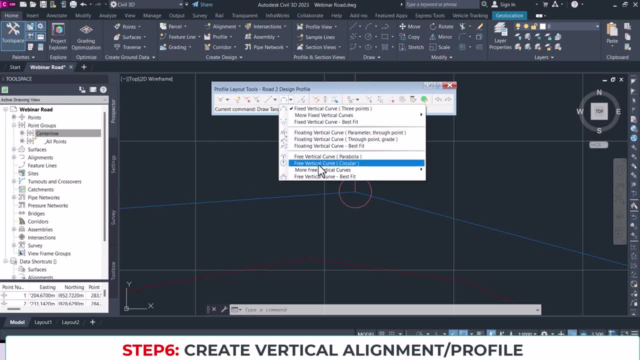 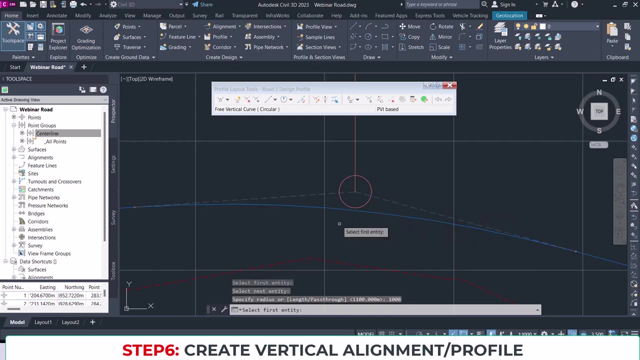 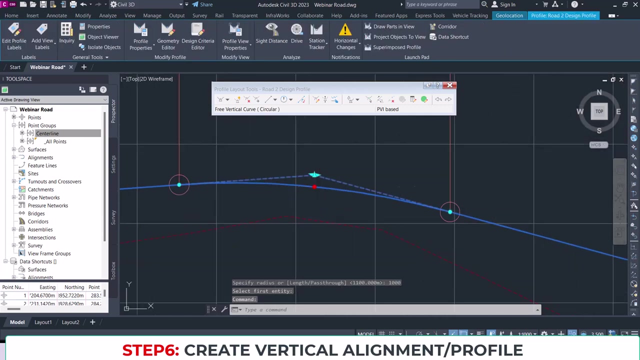 coming down here and then find free vertical curve. you know you can just do that: you click this alignment, click alignment and then specify the radius. let's say one time enter grid, so it's giving us a call. but still i don't like the. the one thousand is not enough for me, i can just drag. 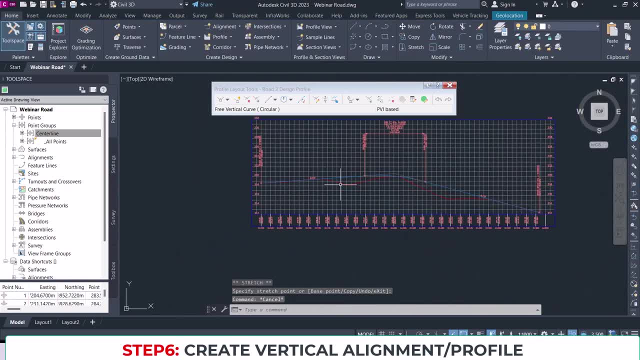 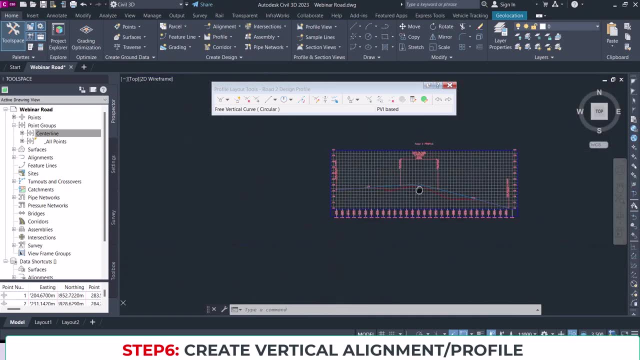 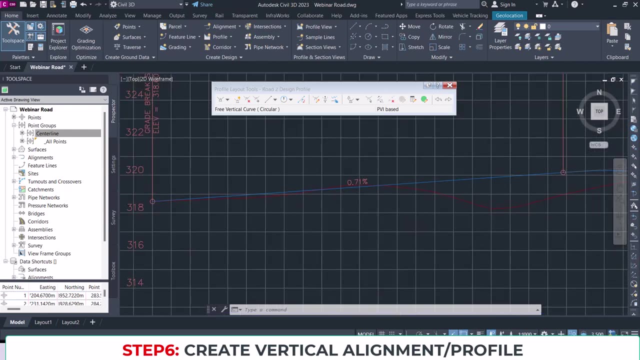 you know up to here and then, like like previously i told you, you can just adjust it to wherever um, however suits you best, but the code will be showing you whenever it is below standard. okay, whatever is the new standard, all right, so that is it. that's how you create your design. 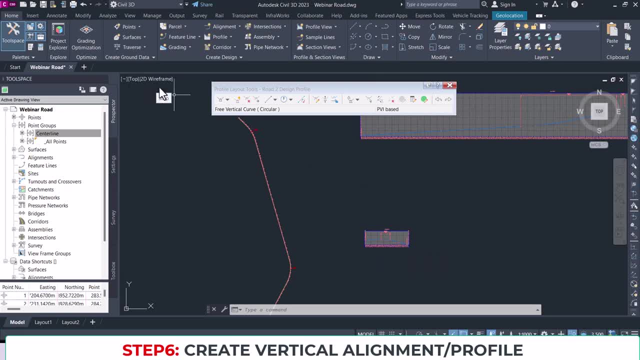 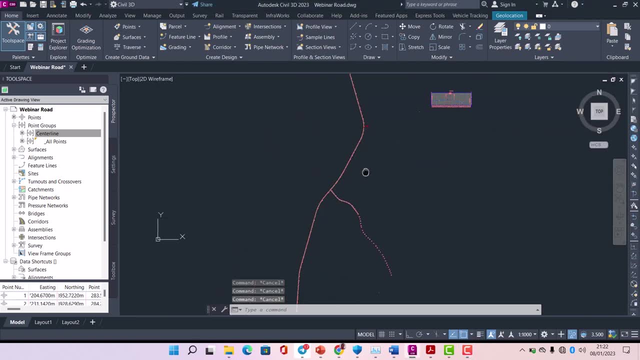 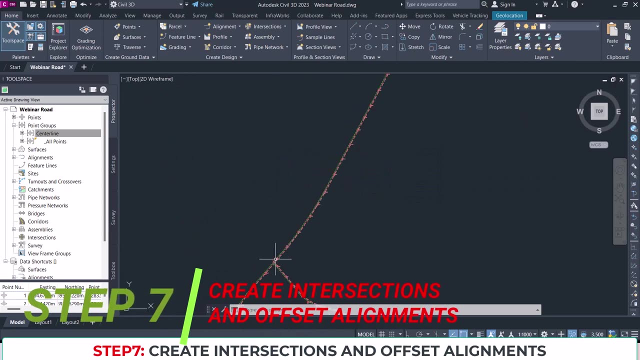 profile. all right, so let's move on. all right, so once you are done with everything, you just close this. the next thing we are doing is to create our intersection. now let me quickly show you something on the profile. you remember. you realize that these two roads are intersecting. 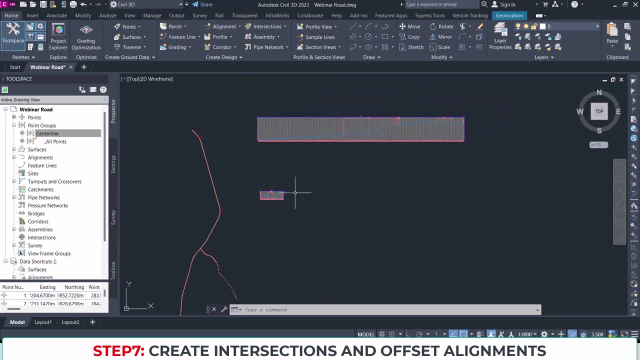 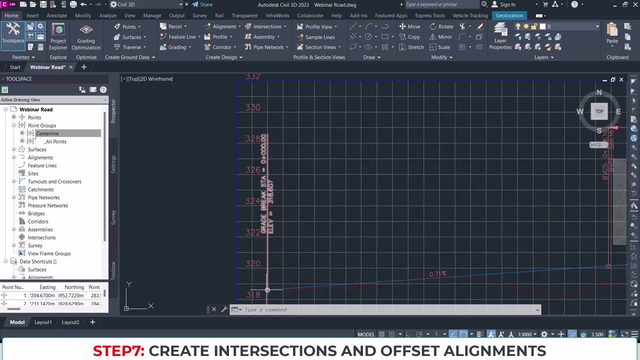 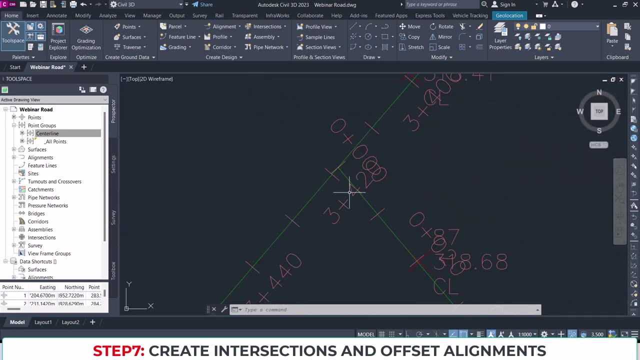 right, they are intersecting. they are not independent of one another, so we designed these ones separately. but that does not mean that. how do you, how are you sure that the level here is the same as the level where this road is intersecting? okay, let's look at it. these 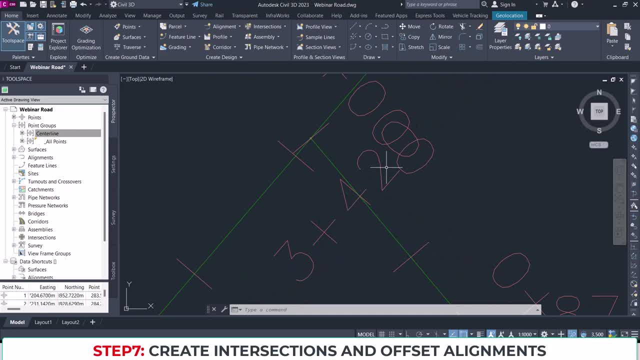 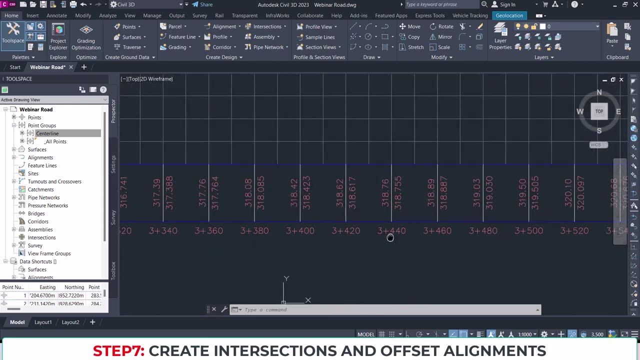 roads are intersecting at about change: three plus four twenty on one on the one row. two is intersecting with one at channel three four twenty. so let's find that where it is uh, three, four twenty. okay, three, four twenty, you can see. all right, you don't have to do it manually and be checking it. 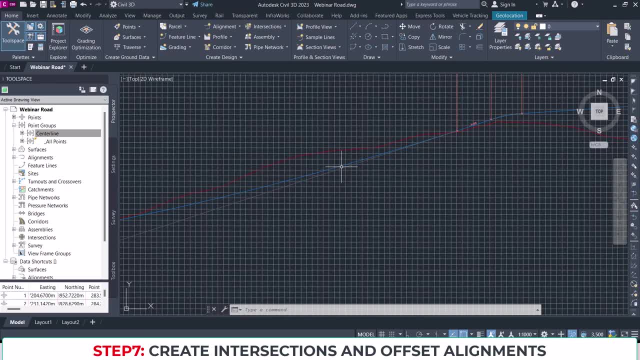 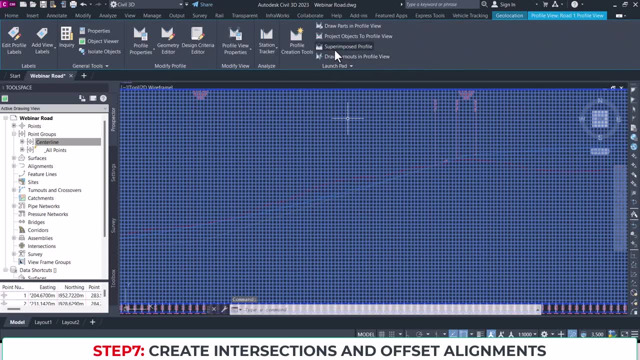 it's a way you can put. it's a way you can put: bring in download to profile here and see how it is looking. so let's just do that. if you click on this grid anywhere, you'll find somewhere up here that shows you superimposed profile. then go to. 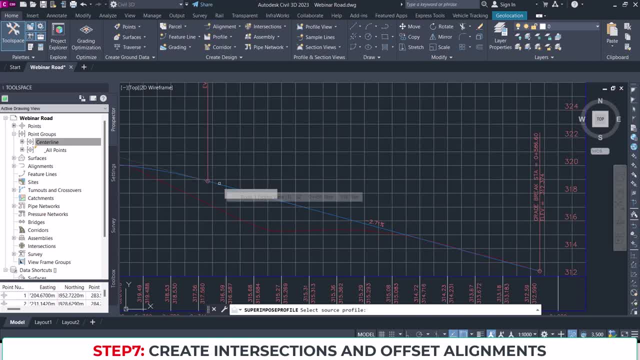 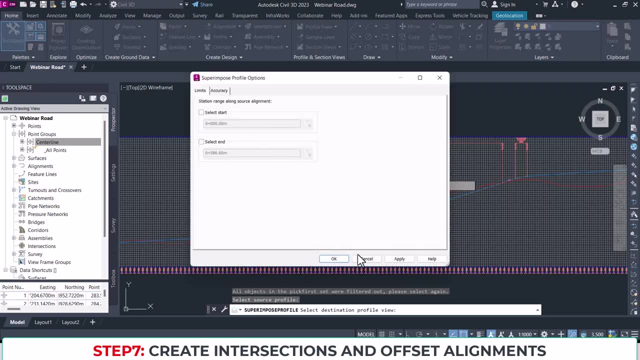 row two and then click the design profile- okay. and then come back to this place and then click anywhere on the grid. it opens up this ribbon and allows you to, you know, select whatever you want to select here. i won't go through all these things, but i just want. if you just want. 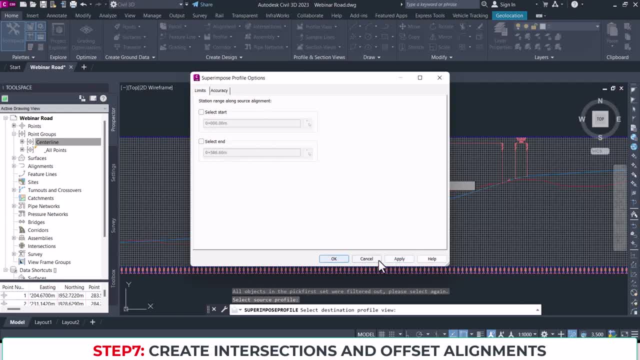 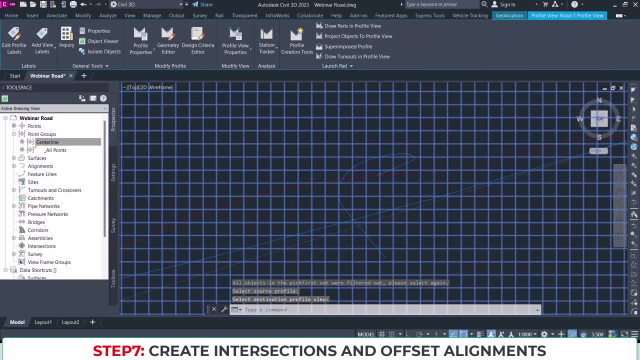 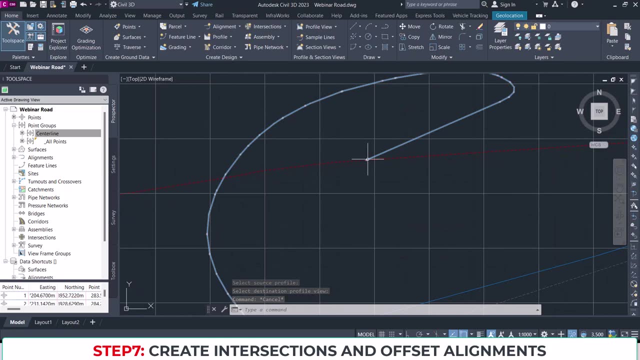 to have only some sections shown, but i want everything shown, so let me just press apply okay and press ok. so now you can see how would. two is on one, okay. obviously the levels are different. see where this one is intersecting. so these two levels have to be married, these two blue lines. 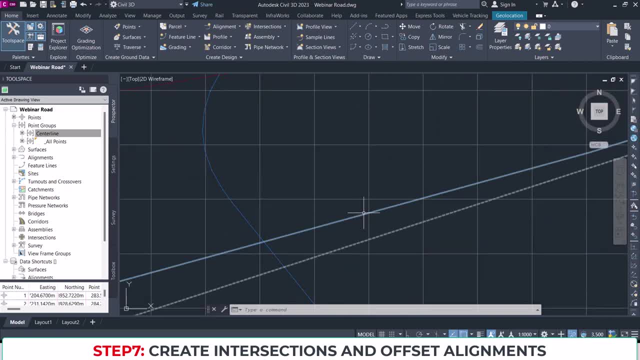 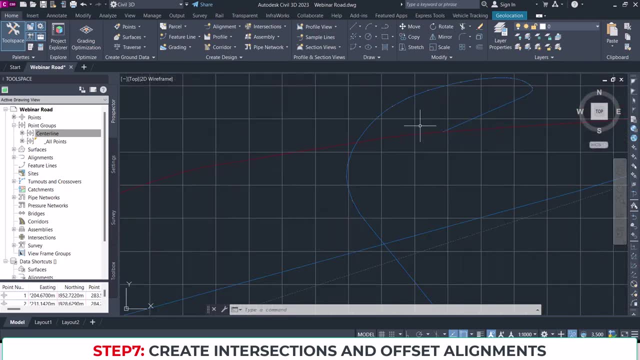 this is where the starting point is, so this one has to marry with this. but how do i do that? i cannot just drag it. you know, i can just drag it, so i can just drag it, and then i can just drag it. know, i have to create an intersection. so watch this closely, as you have seen this by the time. 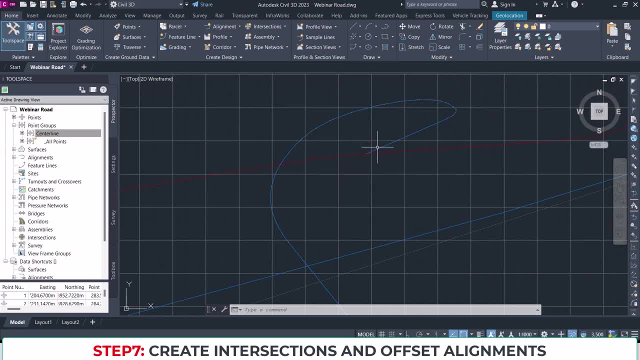 i created an intersection. these two will join. this one has to go. since this one is the one intersecting, it has to go down to meet this row, and so if i want to adjust it up back, i have to adjust row one up, and then row two automatically follows right. so let me go and create an. 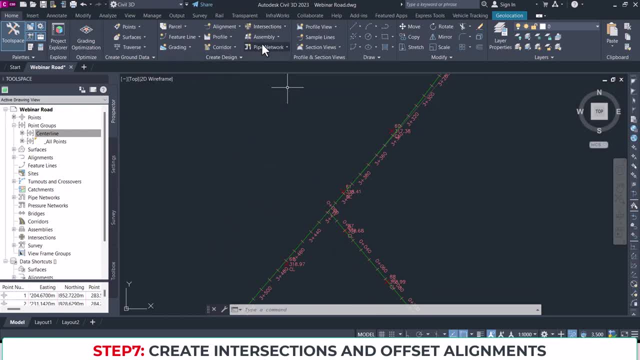 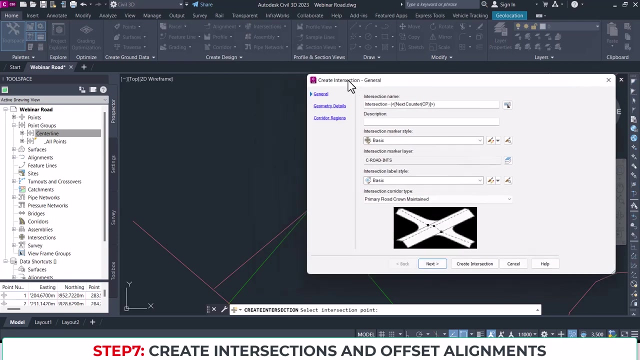 intersection, so i find intersection here on the home tab and then click on intersection- create intersection- so i find where it is intersecting and then click. remember this one of the special features of this design. okay, because it's not quite an easy thing. not everyone covers it. you know, i'm taking my time to do this because i love you all and i 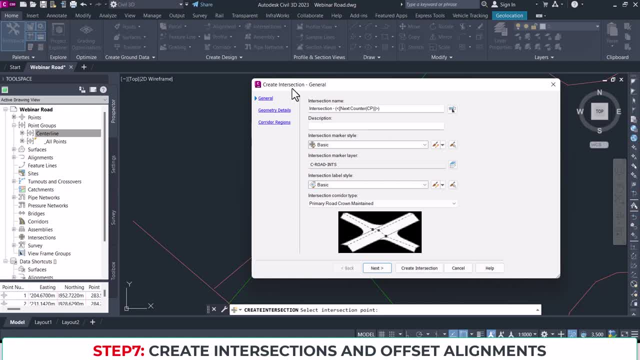 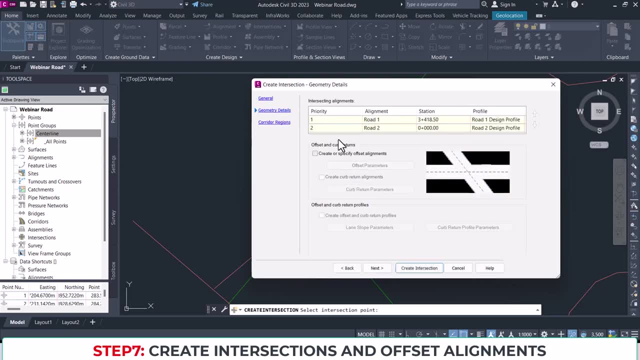 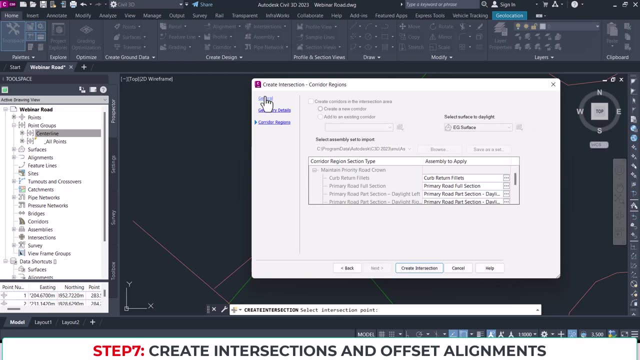 want everyone to you know be proficient in what you're doing. all right, so here i will just create an intersection. i don't need to create all these offsets parameters. i will not go through all the reason why, but just follow me, okay, and then automatically all these things are unchecked. so i just want to create an intersection. 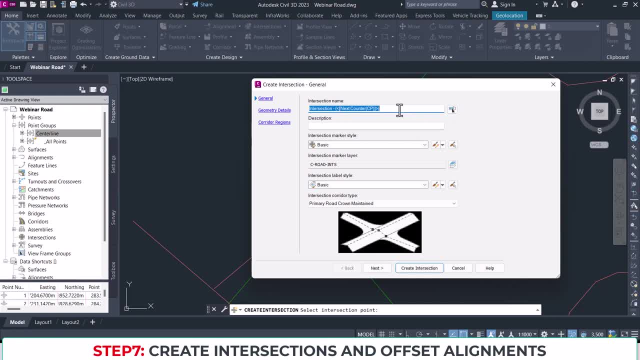 so i can name the intersection. uh, so today it's just giving me a template whereby if you just name it intersection one and then if i'm creating another intersection, if you name it intersection two. okay, so if i want to add a description, i can add it here. if i want to select a marker style, 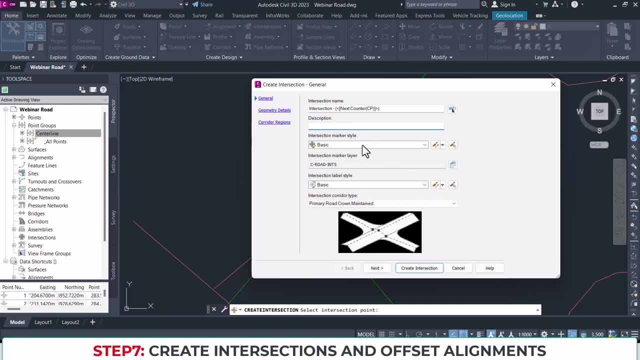 but i'm going to leave it at okay. so if i want to add a description, i can add it here. so if i want to add a description, i can add it here. so you can always create any of your you know default, you know views if you want, but basically leave everything by default. 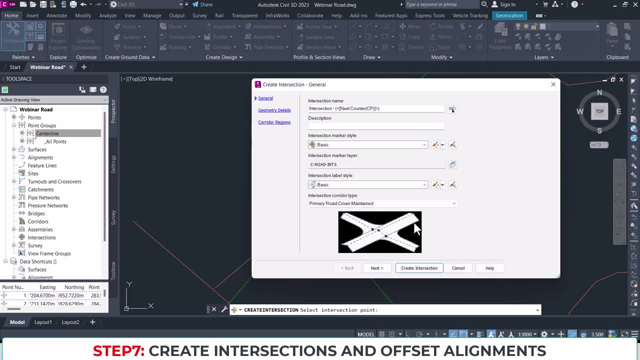 this route is an intersection whereby the primary route, which is the new, that is, travel at 100 kilometers per hour- is crowned, okay, while the other one will just be joining it, uh, without being crowned at that intersection, okay, but if both of them were roots that are driven at 100? 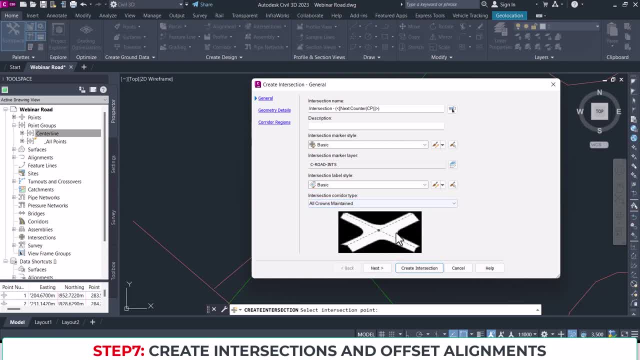 kilometers per hour together. i would select this option and then i'll just leave everything by default, so you can always create any of your you know default views if you want, but basically leave everything by default, so you can always create any of your you know default views if you want, but basically leave everything by default. all roads will be. 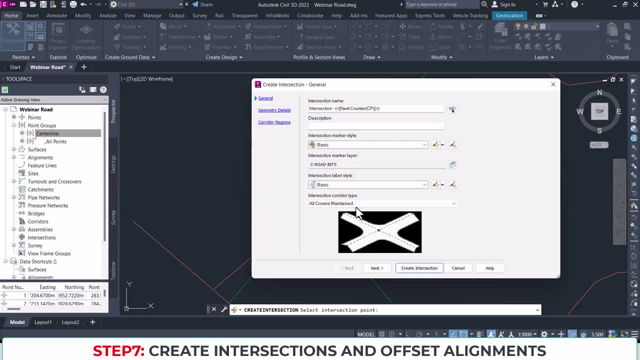 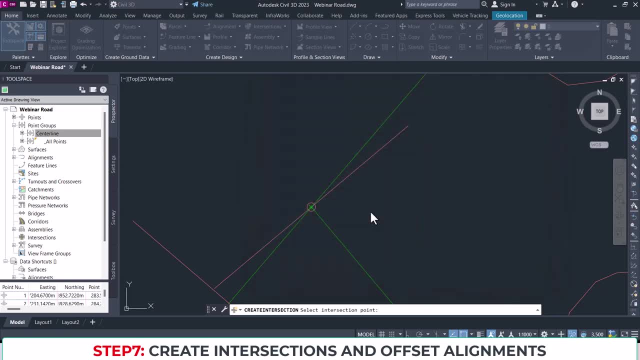 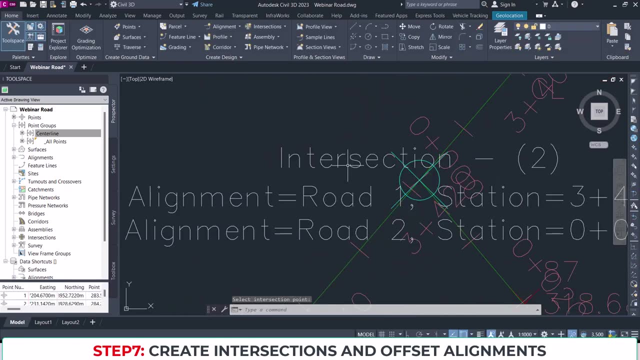 put on coupled, so it will be crowned at the center. so, but now, since the primary road is at the highest speed and those sources, i'm going to see this problem. so let me create an intersection. so, once i create this intersection, watch what happens. okay, automatically names it for me. um, okay, it should be one here, but never mind, okay. 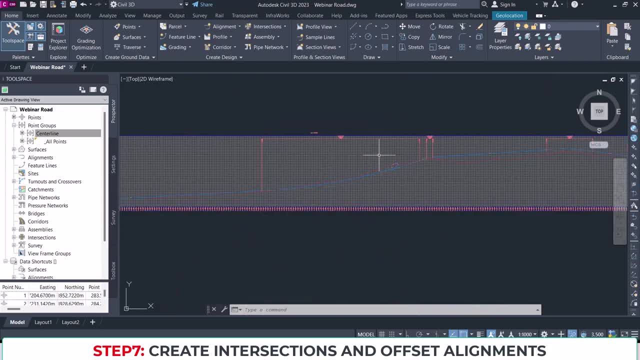 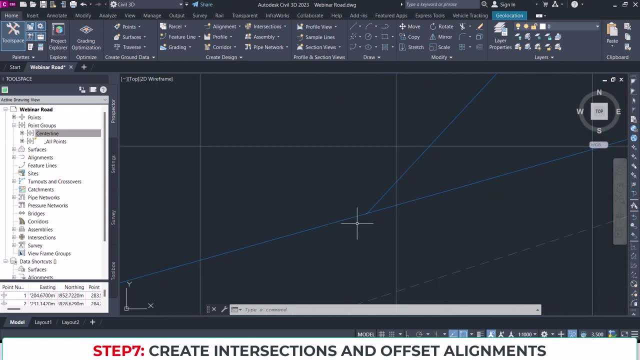 so this is the intersection. let's go back to our profile and see what happens. tada, you see this go. I filter all the name and actions on the problem section. see what happens. tada, you see. this profile profile has automatically come to marry the intersecting where it is intersecting. so anytime. 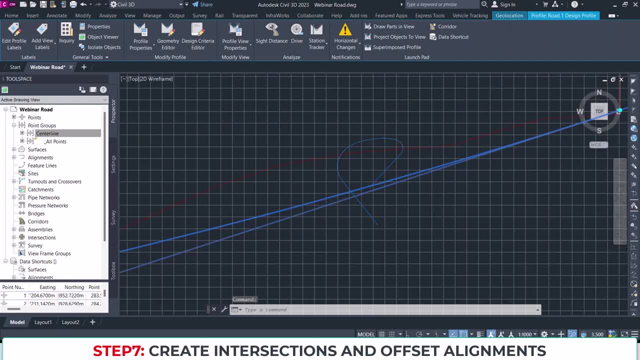 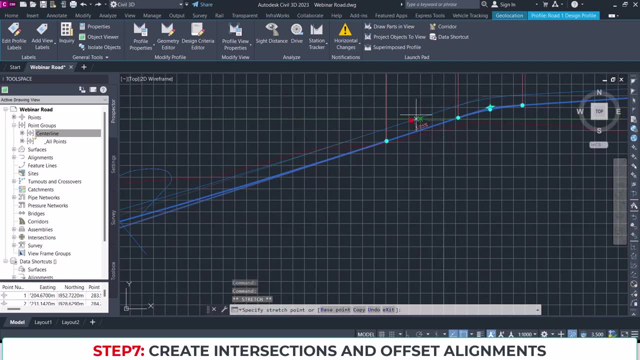 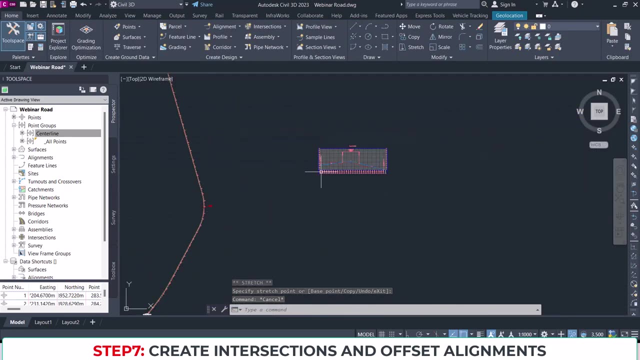 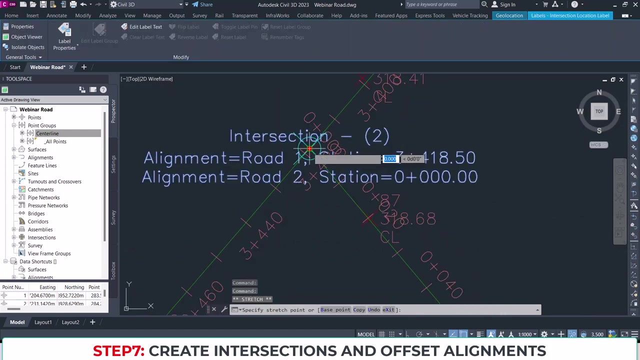 i make an adjustment, both of them will go up. let's say, i want to adjust this one upwards. okay, let me adjust this profile upwards. see what happens. great, you see, this one is following it. so it has to be intersecting in both alignment and profile. so that is the importance of creating an intersection. wow, i'm teaching you all these. 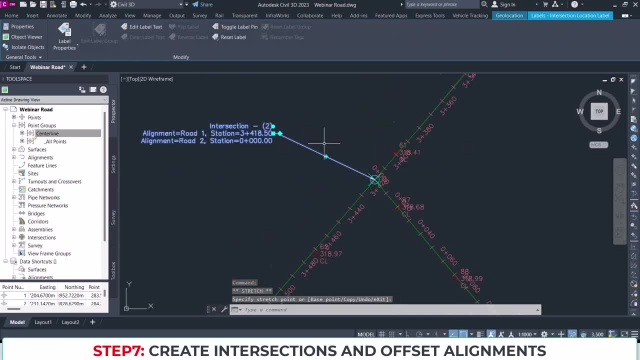 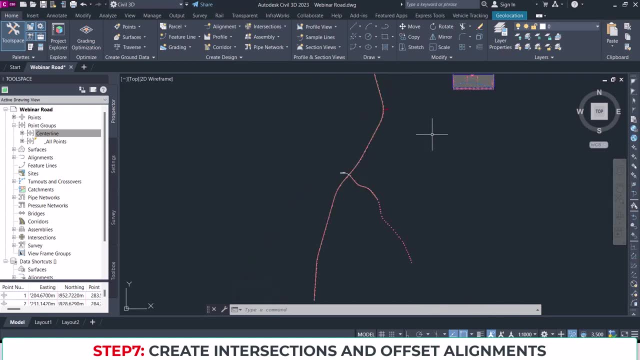 things for free, yep. so i spent a lot of time learning this myself. when i was doing it, i was always worried. there was a time i was doing it manually even, of course. by the way, i have designed routes on autocad or just normal autocad without civil 3d, and i do that always. it's quite small. 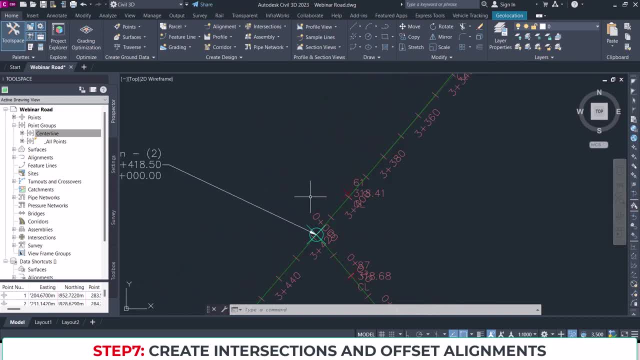 it's quite sweet, but it's not automated. that's where the issue is. when you're doing review revisions, you suffer. or civil 3d: you can make revisions fast, you can design a large network of route fast. that's why civil 3d is powerful and besides it's also- uh, being compliant. so 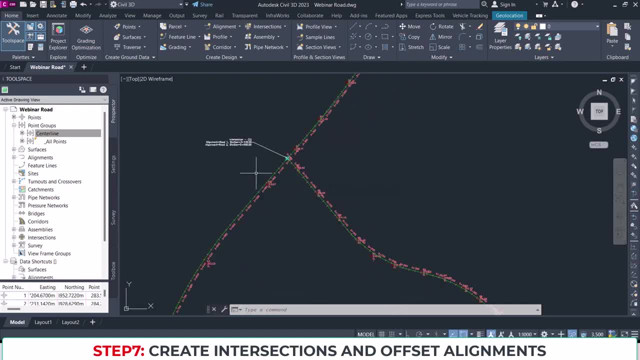 uh, you know i'm a big enthusiast, right, so i have to upgrade. i have to upgrade a long time to civil 3d. so that is it here. okay, we are creating an intersection. the next thing is to create our offset alignment. all right, remember, our roadway is, uh, 7.3 meters, okay, so that means 3.65 to the left, 3.65 to 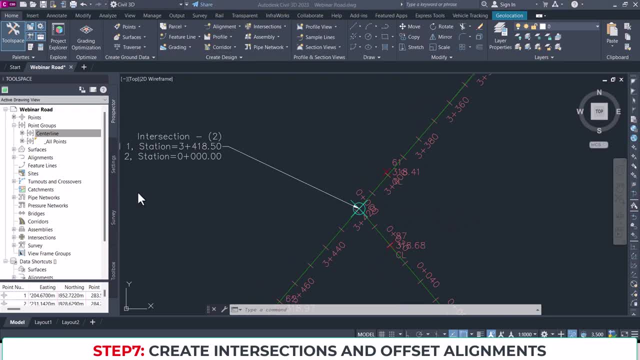 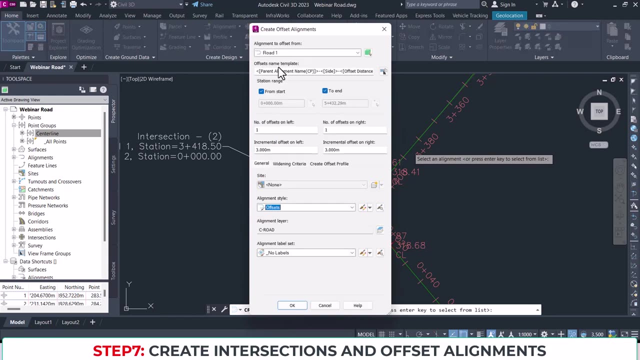 the right. so let's create that offset alignment. so where do you find that? you find that here in alignment, under alignment, you see create offset alignment. once you select that, you click the alignment. you want to create an offset? okay, and then it opens up this: okay, you can name the offset alignment. 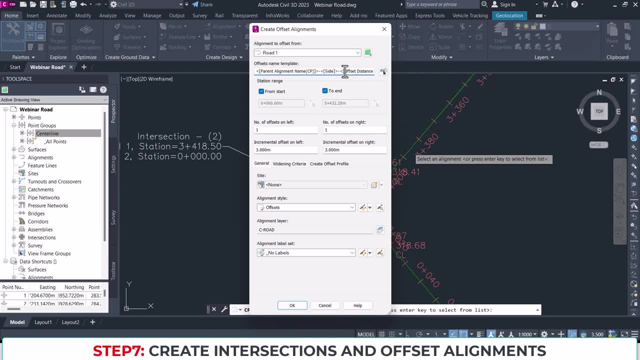 here. it is going to use this template, i, i expect. i just want you to use a template because, since you're going to be, we are going to be creating a limit both to the left and to the right, so automatically to be naming it left and right for us using this side here. 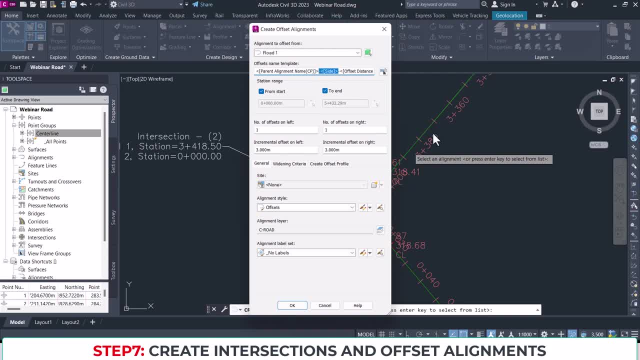 that you are seeing. so this is a template that automatically knows that. okay, this is the left side, so it names it to the left and then it names the other one to the right. so make sure you are if you want to start from the beginning to the end to create the offsets. 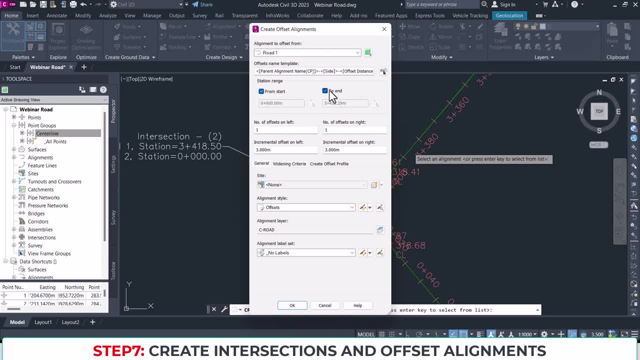 yeah, you can choose that here. okay, just leave that both of them checked. okay, now we are creating. you can create multiple alignments: offset alignment to the left and multiple to the right, but for now we just have one offset alignment to the left, one to the right. so here, remember our 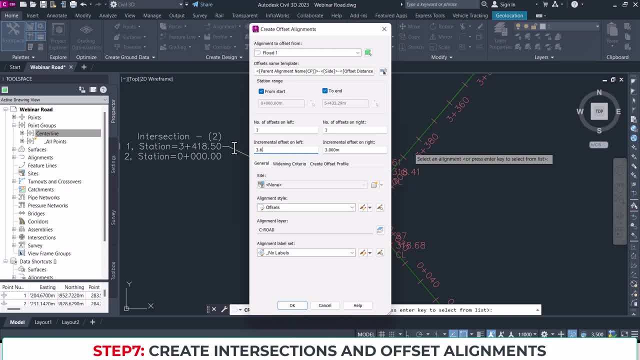 lane is 3.65, so i'm going to put 3.65 here and then also here 3.65. all right, so we can add a site up offset styles and then you can choose a level. now i don't put levels when i'm doing offset alignment. 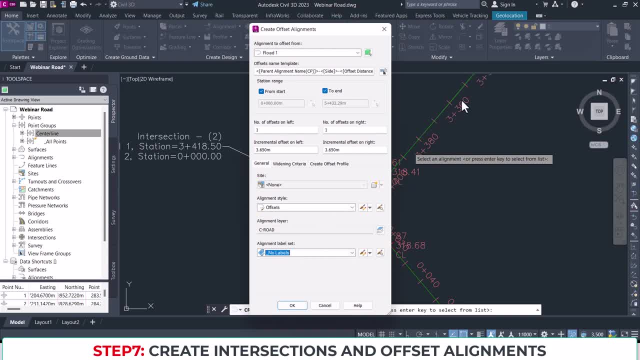 because already this level, there's the levels in the main alignment, so let's go to the widening criteria. okay, now i don't need any widening, so i'm not going to add that. and, of course, no check, no design check for that. so i will create an offset profile for sure. so, because i have a profile on. 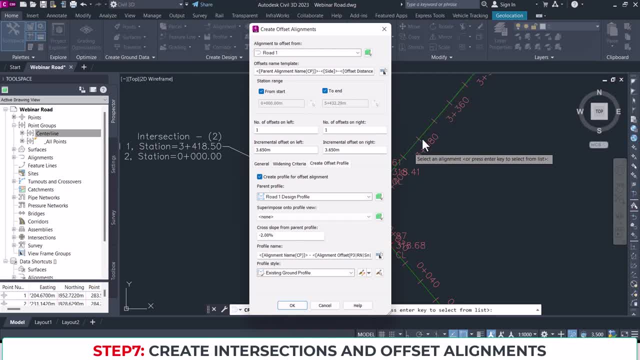 this um design profile on this center line. so i'm going to be using that very design profile. okay, and our one is a profile. now do i want to superimpose it to a row two view? yeah, if i want to, so that it will show on that profile view. 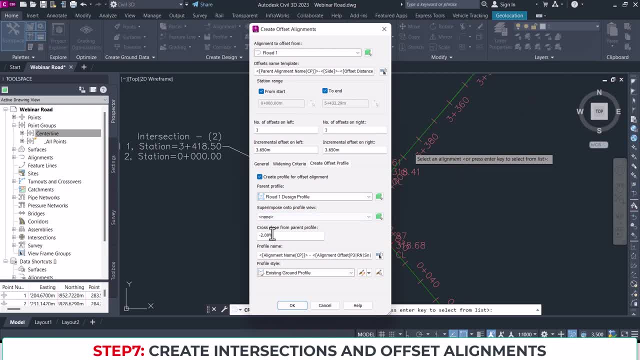 okay, but i don't want to do that for now. so, and remember, our cross look is 2.5 percent. okay if you, if you remember the review that we did. okay, if you are using two percent, you can leave it at that for your own log, but for this one it's 2.5 percent. so, and now, if you give me programs, i'm not going to apply anyKit program, but we're going to create another one because I'm not a pro. so give me an icon right now and i'm just going to call it to my page and i'm going to copy it into a profile. 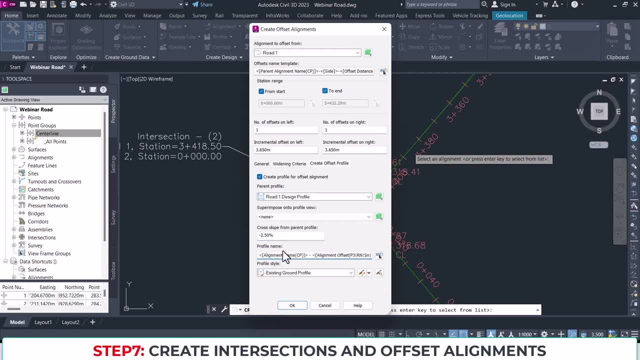 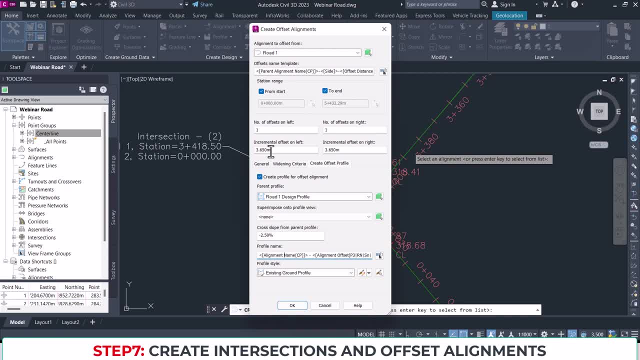 down by 2.5 percent to at 3.6 meters. okay, okay, and then it will name it okay, using this template. let's do it like that. so let's use the profile style as existing. also a design profile, design profile. all right. so because it's a design profile, so let's press ok. 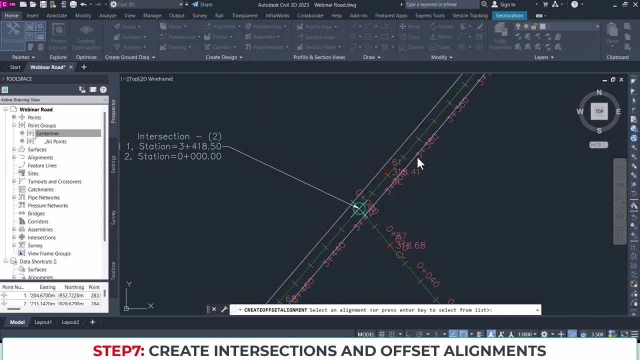 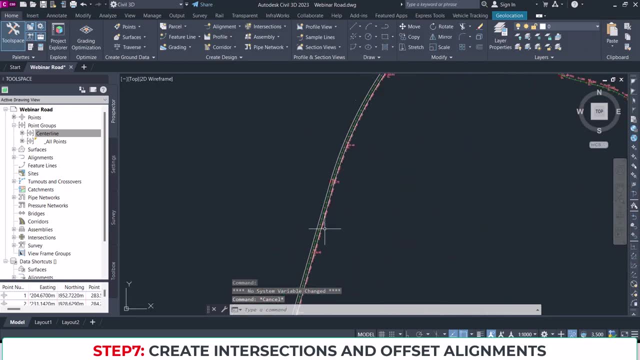 okay, once you do that, you can see that this is the offset alignment. very beautiful, okay, this is already looking as the road proposed. what does this offset alignment do? this offset alignment is dynamic. okay, when you change the center line, it also changes automatically. so let's say, i change. 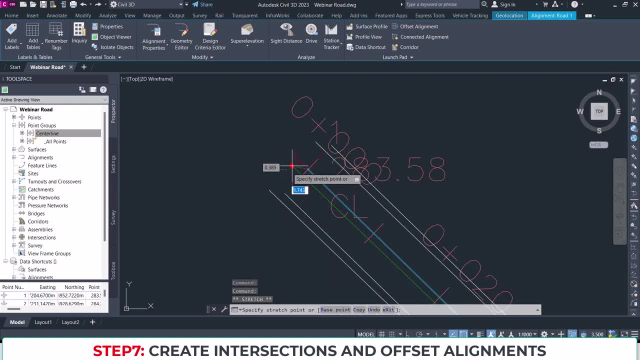 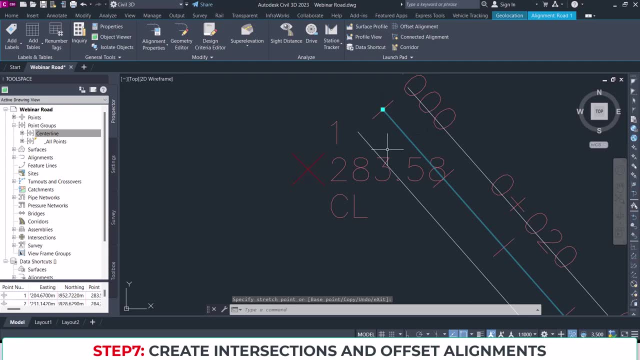 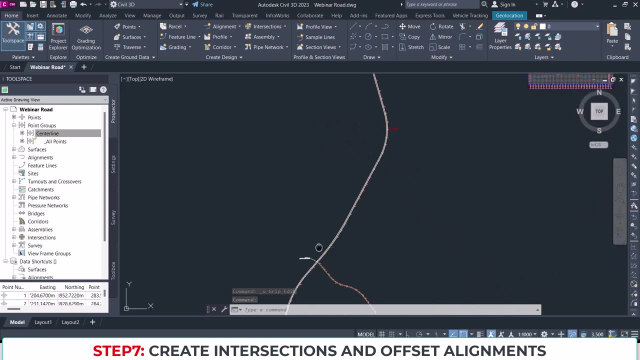 this to this, to somewhere here you can see it's moving together. okay, if i drag it, if i drop it anywhere, okay, it will, it will. it will update. so let me go back by pressing ctrl z, okay, and then i'm back. so that's the good thing about the offset alignment. so let's create offset alignment for the nest, for. 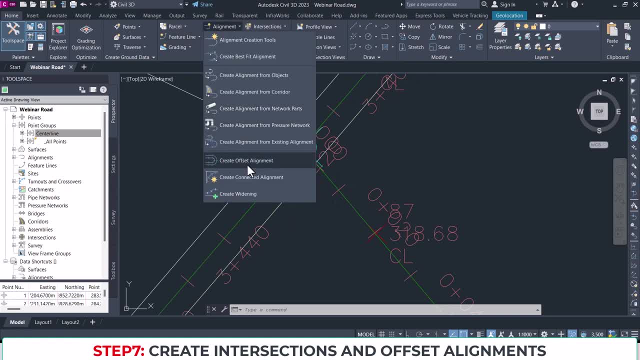 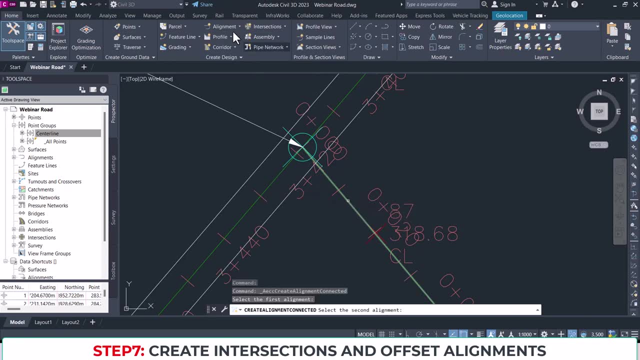 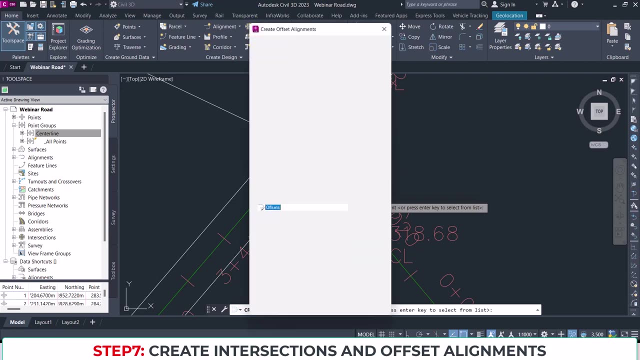 the intersecting alignment. so let's create offset alignment. create offset alignment and click on this. so, since it's the same thing- oh sorry, i'm creating connected alignment. i'm supposed to create offset alignment here- i click on this and then it opens up again, so i'm going to allow everything to be the same. okay, of course you can. 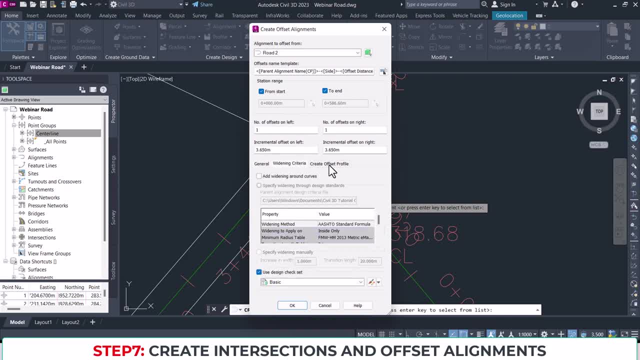 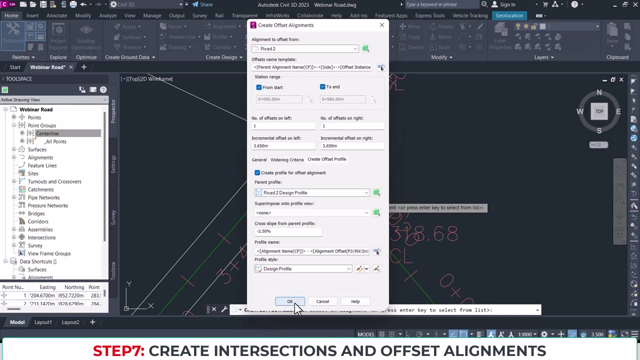 see 3.65 is already populated here for us, so everything, i'm going to leave it the same, because it was very before and stable. 3d is merciful enough to allow everything to be back, in case i want to use the same things, okay, so i'll just press ok and then, yeah, it has created for us. 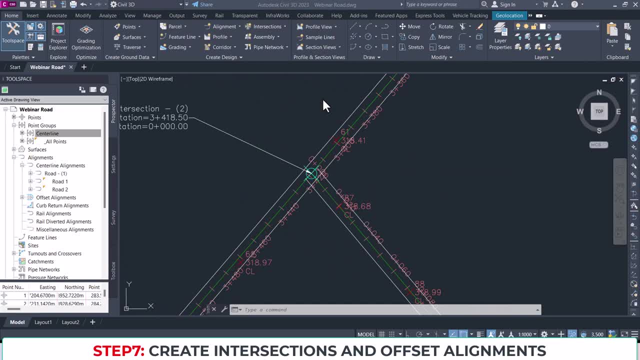 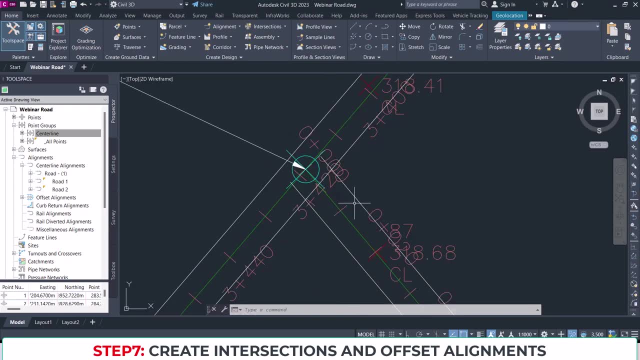 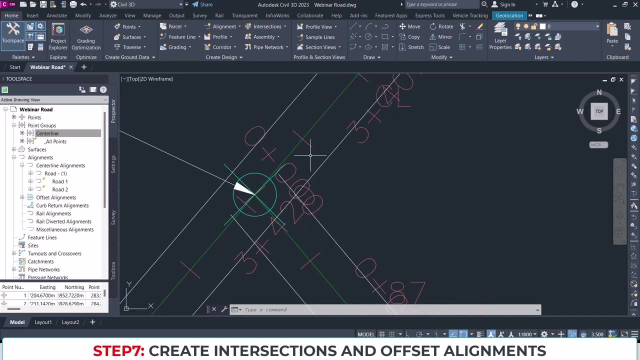 all right, all right. so the next thing i'm going to be creating is the connected alignment. okay, why is this important? because, as you can see, this is an intersection, so you have to drive through a curve when you are going to negotiate this intersection. okay, you have to drive through. 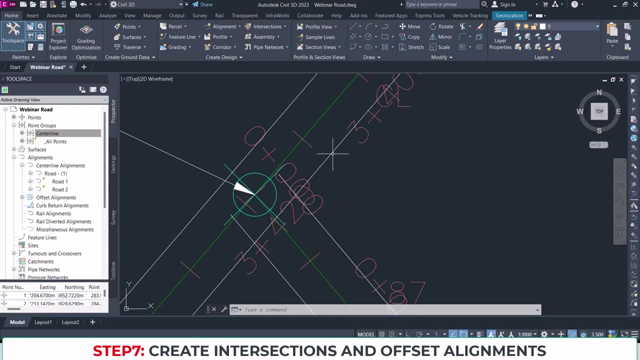 a coffee. so you cannot do that with just the normal filler command. you have to use that using connected alignment. so you find that here under alignments, you go down to create connected alignment. okay, you click the first offset and then the second offset of the intersection, then pick a side where it's going to be put, then press enter. okay, it opens up this. 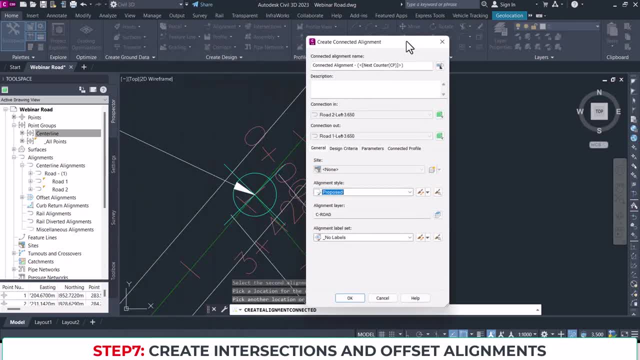 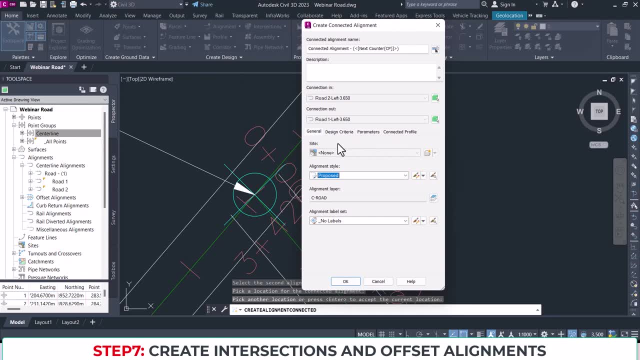 window for you. it's a little bit different for 23, 23, you know, uh, as opposed to 2018 and 19.. okay, if you're using 2022 and 2023, this, this, this platform here will, it looks different. you know where to find what to put, but it's the same thing, so don't. 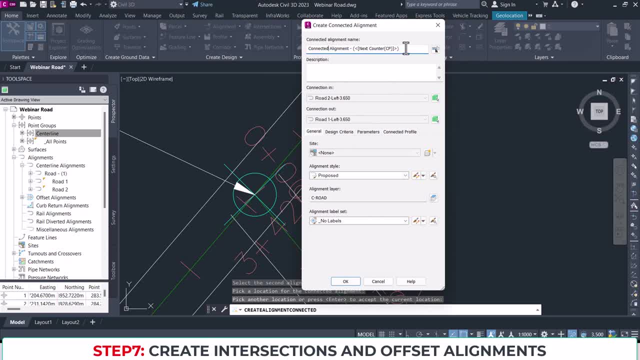 worry, so here you can name it. okay, give it a name or allow signature to just name it for you. here we can just call it. um, let's say left call return. okay, yeah, because the card returned, so let's give you. let's uh see the what we have here on the generator. 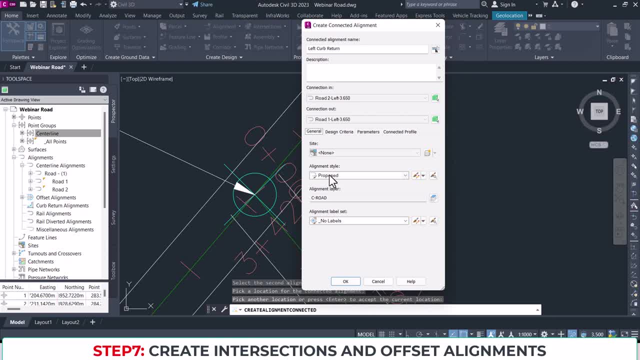 can choose a side, but we don't have any side, so we have the alignment style to be proposed and then the level side. i don't want a level, so good, i don't have. i don't need levels because the levels are noisy. so, on the design criteria, i'm not going to be using a criteria based design for 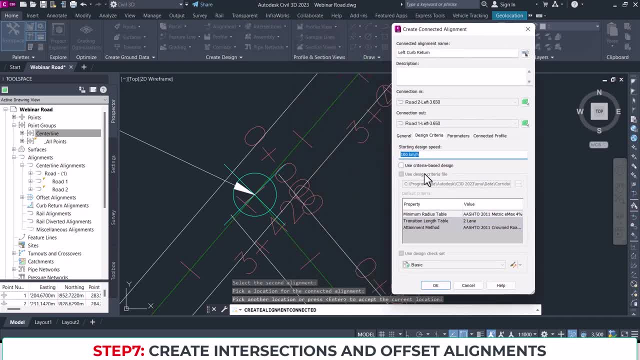 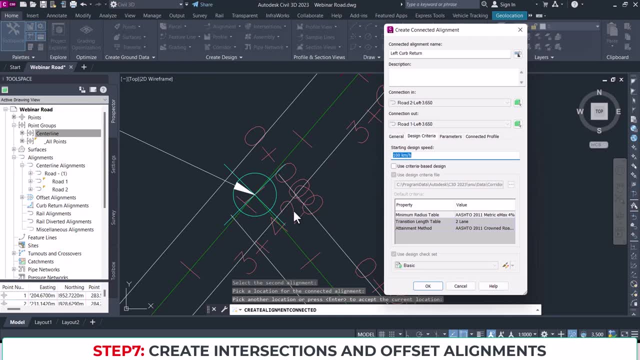 this one because, um, it's going to be judging it as if you are driving at a long speed as a speed when you are negotiating the intersection. usually you are almost at zero when you come to the intersection before you now start driving, so you just need any cup that will allow you to turn and 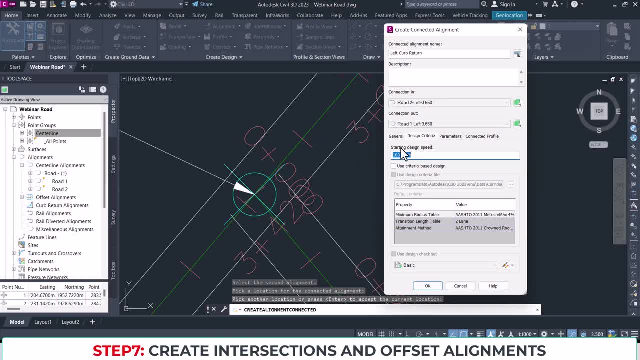 usually you know you, you consider a truck- okay, a large truck- that is about 20 meters long. so when it's negotiating this corner, usually when you're using wb, the 2f truck, to design, it's about 20 meters long, so it needs about 11 meter radius here. so for this course we're going to be using like 50. 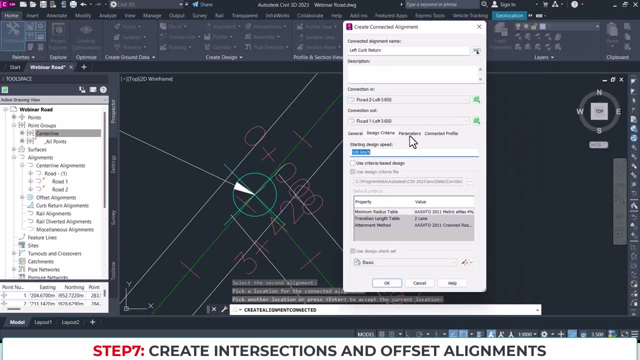 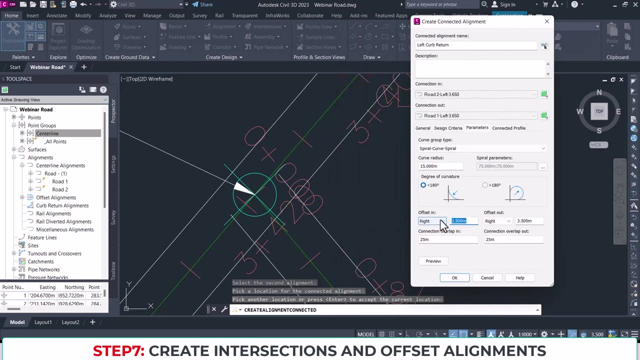 meter coverage. where do we find that? all right, you can find that on the parameters. okay, so the coverage is going to be, let's say, 15 in this case. okay so, and then we and the offsets. i don't want any offsets. right in 2018, you won't find this thing, but if you're using 2023, you'll find all. 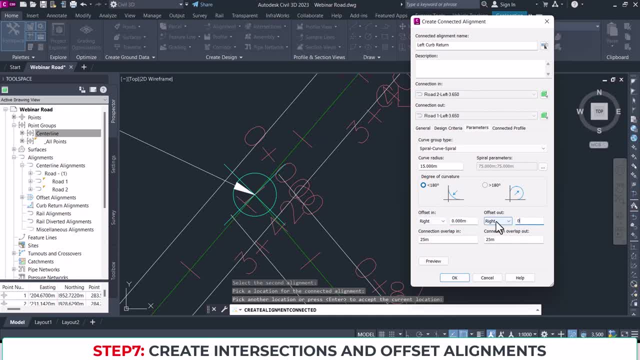 these things here. so i don't want any offset to the left or to the right. you can even press preview, okay, so it says so. we have to select a circular fillet, not spiral. so we need a circular fillet. so let's preview that. good you. 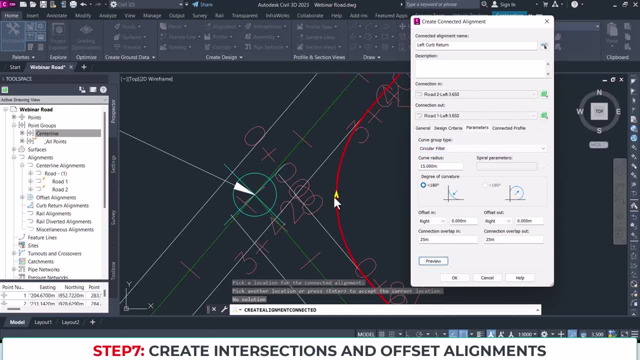 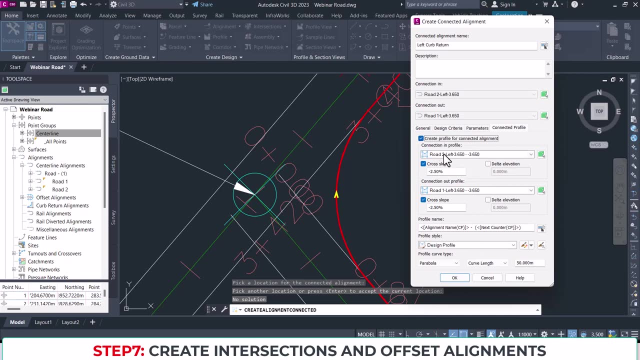 can see how it is going to be okay when it is done. so i think this is good and it's going to be overlapping by 25 meters. okay, no problem, and you can adjust that if you wish. so then for connected profile definitely is going to create a connected profile. so in this case, as you can see, the 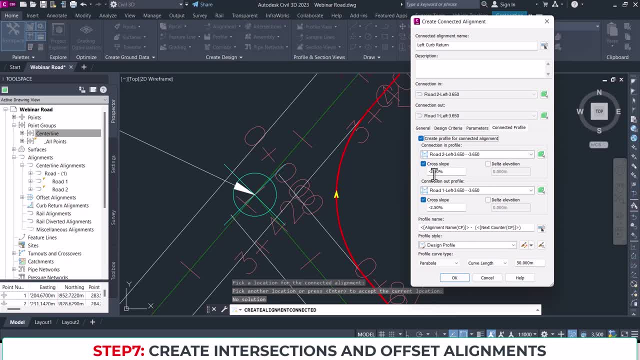 the cross slope is 2.5 percent, which is good if you, if you have it as 2.0 percent, you can change it to 2.5, because that's what we are using for our design. so, and the alignment name is going to use, you know, a profile name template. okay, let's. 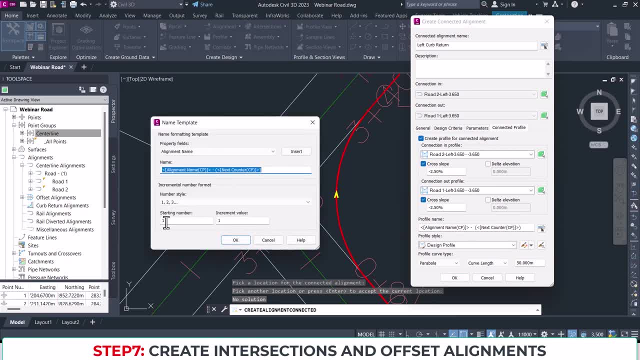 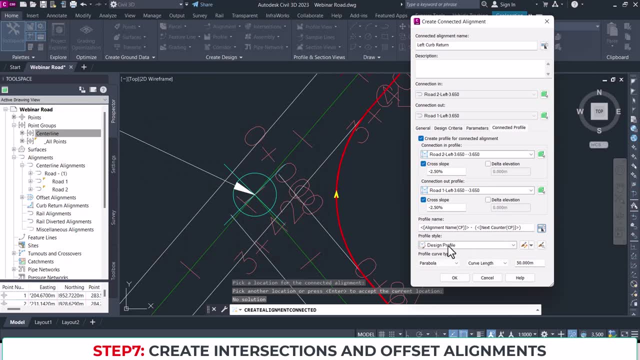 call it. uh, let's see what that template is saying. okay, starting from one. okay, now let's just have it like that. okay, so again, we are just using a profile style as design profile, then the profile curve type. okay, you're going to be able to circular. i prefer circular because, as i told you, it's easy to construct. 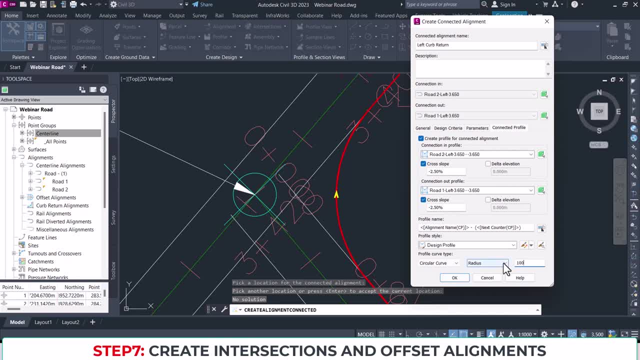 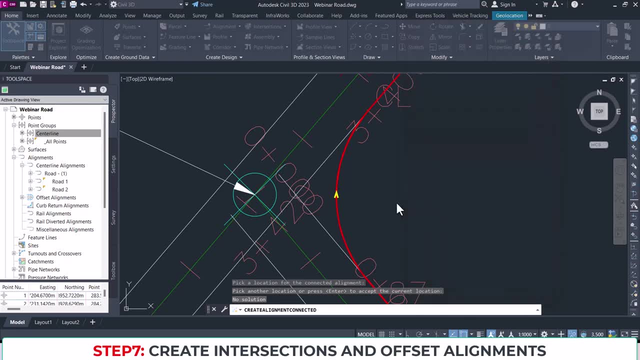 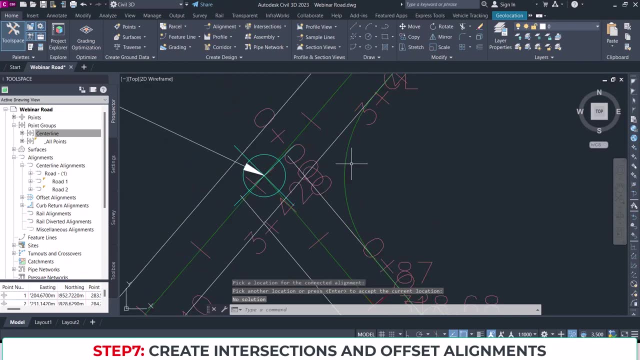 and then the radius i can just use, let's say 1000, or let's say okay, let's say 500 for this. okay, let's say okay, now great, so we have created that, our alignment. so i used the style design profile. that's why it's looking like my center line. well, actually, i would use offset profile. 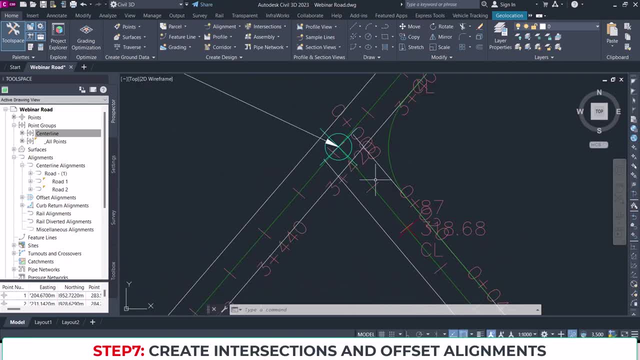 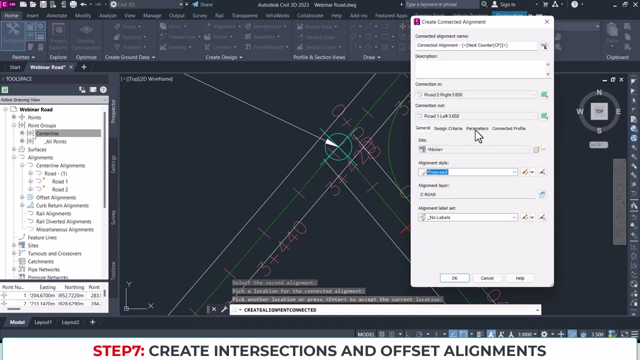 but that's not a problem. okay, then let's do for the other one. we go to the alignment and then create connected alignment. we select the first and then the second, and then find the side and then press enter. we are also going to use 15 in this time, so let's just quickly go to. everything remains the same. let's just okay. let's. 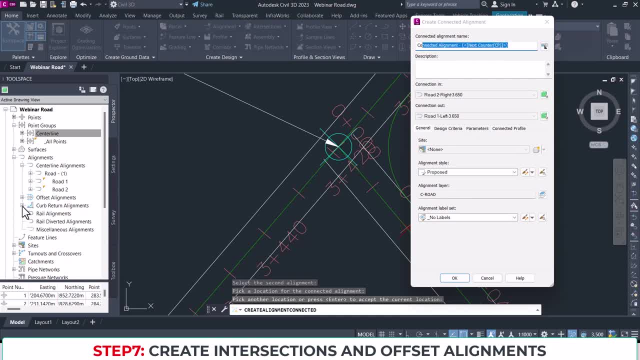 call it did. we call the other one left cobblestone, okay. so we call it right cobblestone, right. so let's call this one left curve return. so let's leave everything the same. it will almost be the same. in fact, everything will be the same because we have: signature is messy for from us. we're not just, yeah, be doing. 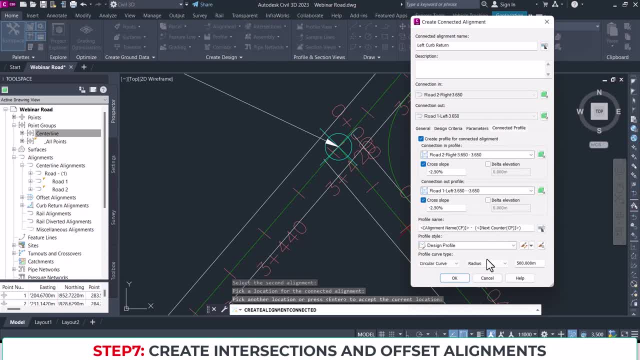 it again. so the connector for everything just allows us to use that template that was there before. now i'm going to just use- uh, you know what's what? i could have just used all this nails, let's say layout okay, and then everything will keep the same. 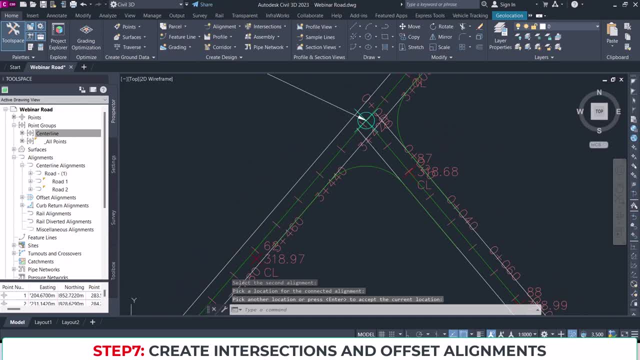 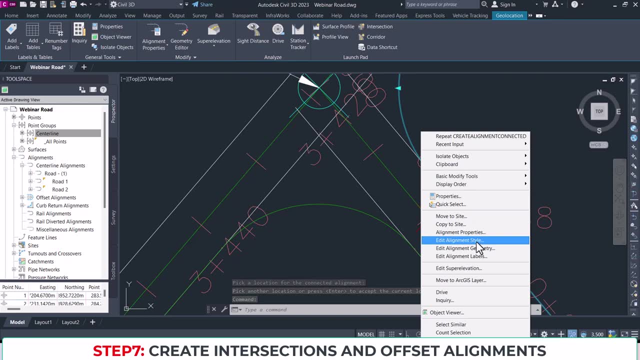 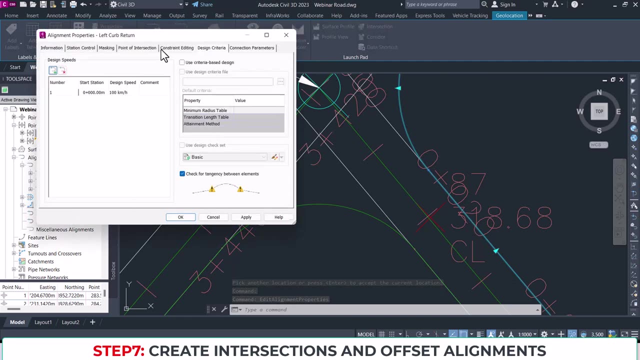 all right, you can see. okay, still green. you can make it white. you can change the color to white. you can always right click on this and then go to alignment properties. okay, once you have this alignment properties open, you can select. okay, sorry, you can select how it will look. let's call it intersection basic. 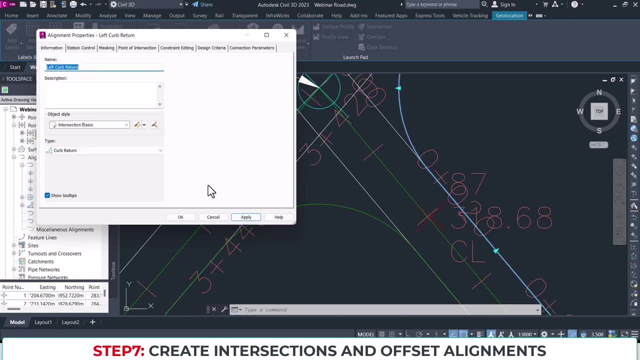 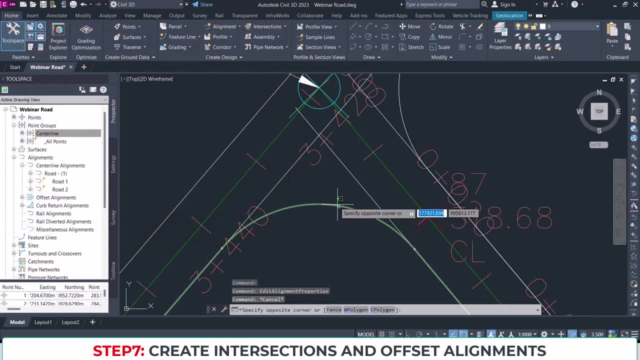 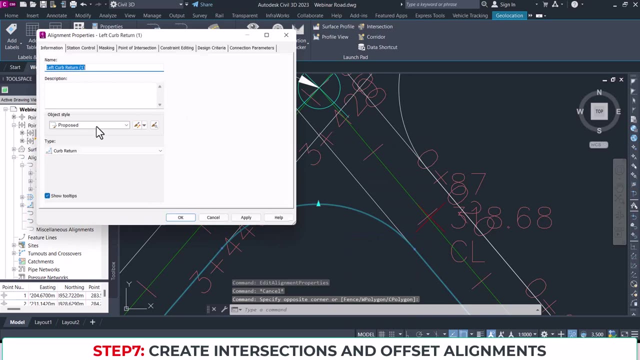 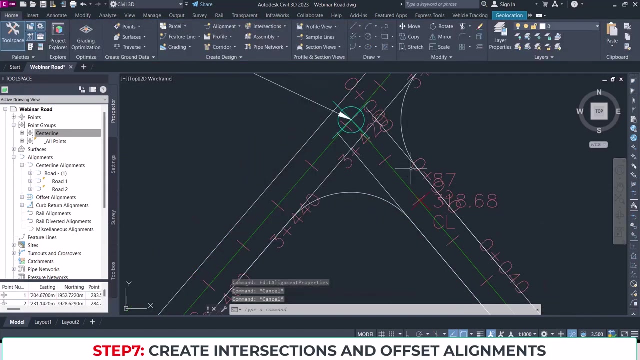 okay, apply that gives us that white one. i like the white. okay, and also this one. you can change it from this one alignment properties. all right, so you can change it to intersection basic. that's okay. all right, so that's. that's that right away. okay. so let's say we're okay with this. 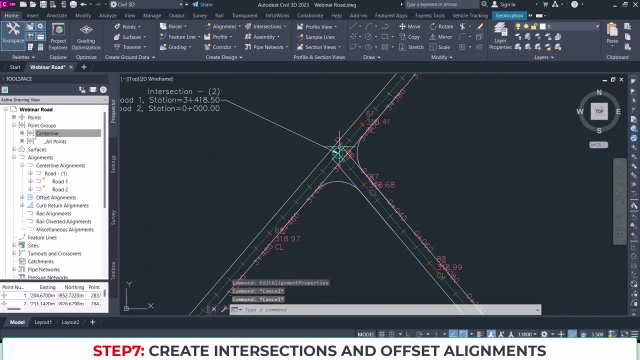 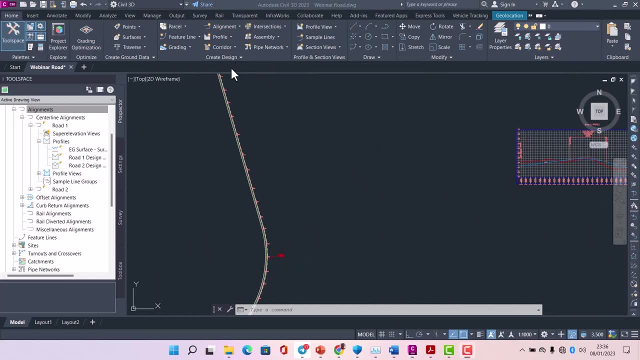 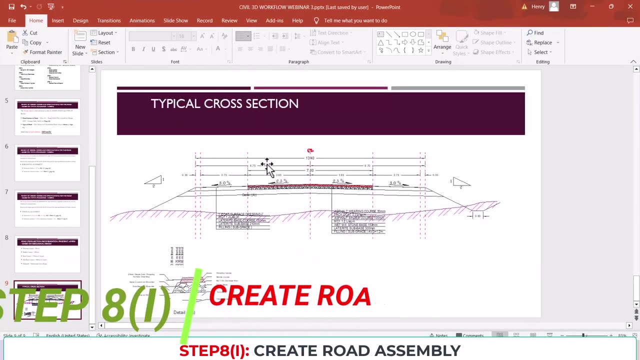 so we can now move on to the next thing. so look at our road. it's looking fine, is it not? all right? so the last thing we are going to do is, on the design steps, is to create our road assembly. okay, so, if you remember, uh, this is how we want the typical cross section to look like. all right, so try to. 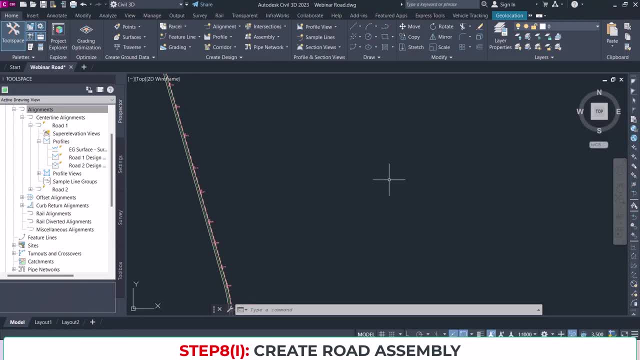 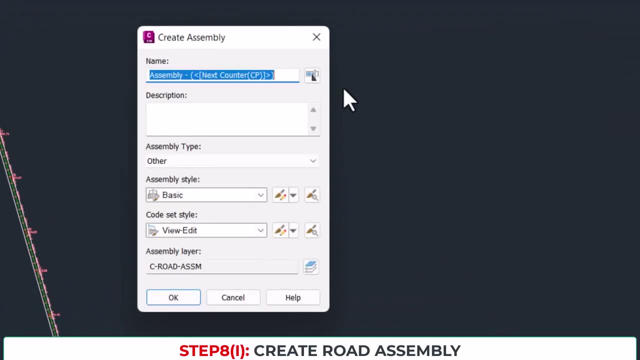 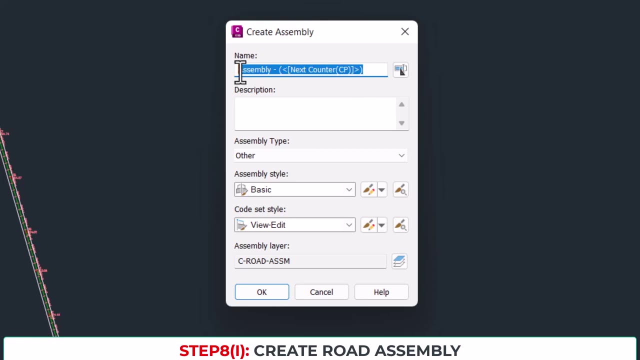 model this into silver here so that we can create our corridor from there. so let's go to assembly under the home tab on the print design and create assembly, all right, so if you look here you can name the assembly or use the template. the same 3d provides for you, but because we are going to have so many, 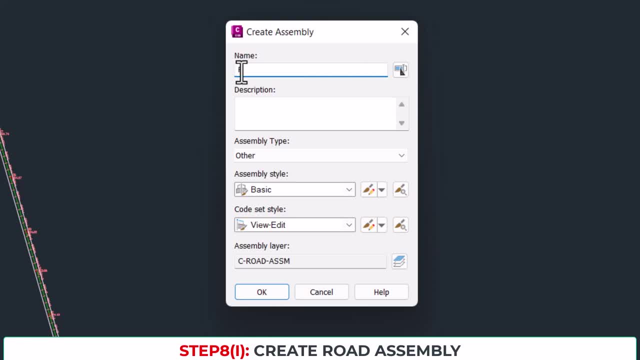 assembly. i'll show you why shortly. let's call this full assembly, the one that will have all the parameters together. so, and then we are going to name, we are going to give it a type on the divider, crown, wood, and then we'll choose the elements- sorry, assembly style to be basic and the 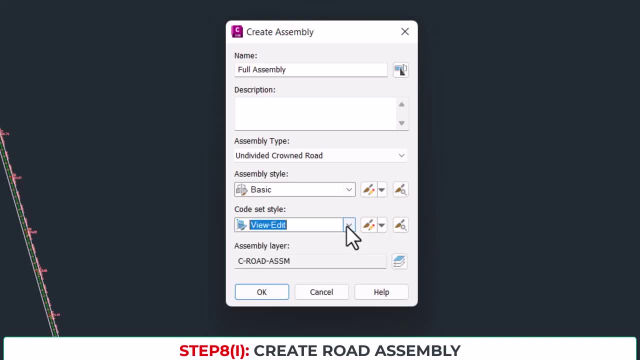 code set. let's use view edit and like it for some reason. but i have my style, which you can also create yours by using this create new here. but we're not going to that, so let's go. it's okay. so you choose somewhere within your drawing, anywhere that you can locate later. 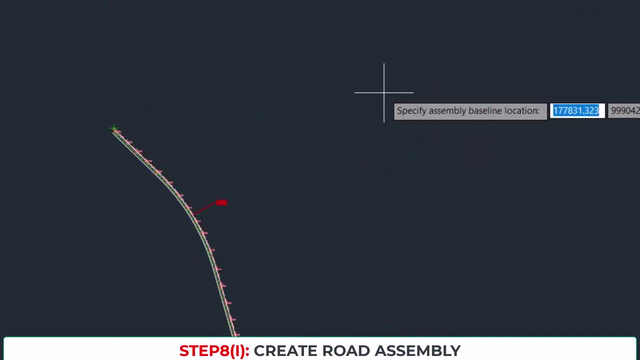 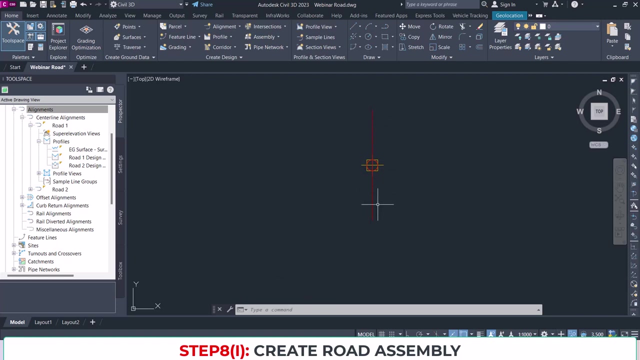 okay, i will choose to do it close to my start of alignment, somewhere to the right of it. all right, so then i'll click uh there and that's able to zoom into the center line. for me, this is the center line, the baseline for creating the alignment, all right? so, uh, sorry, creating the. 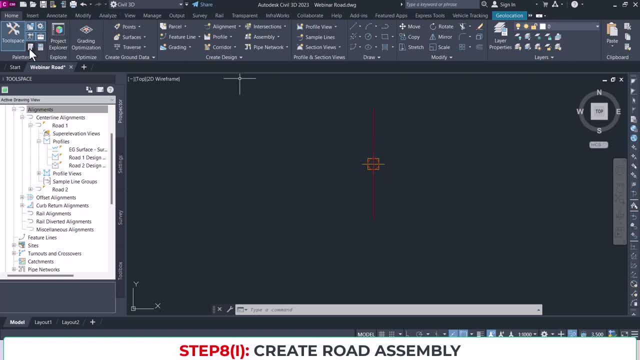 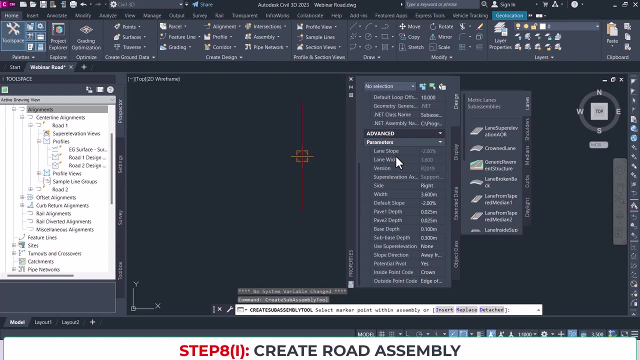 assembly. now let's bring in our tool palettes. you click on this place and open up your two palettes. so, uh, we're going to start from links. okay, we'll choose lane super elevation. so it brings up this properties window allowing you to put in all the uh the statement, remember, in? 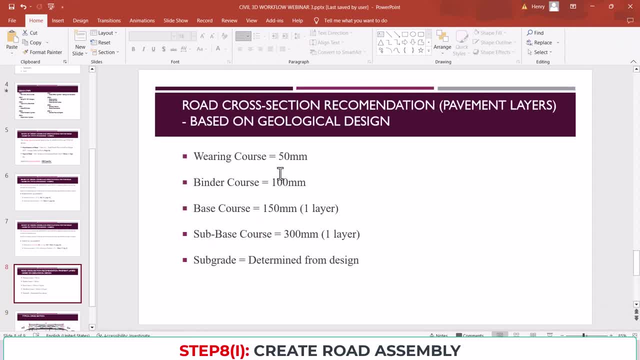 in the cross section. we have a wiring cost 50 mm, binder 100 uh base cost 150, serv race 300 and then sub. doesn't it design by cut and fill? so let's start. we are going to model to the right first, so let's start area model. so we will have a channel in this channel. so let's start on window. 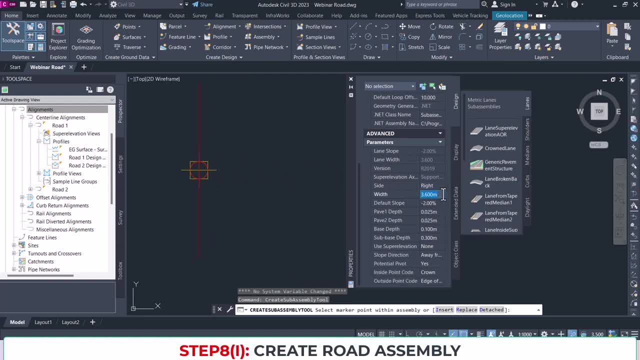 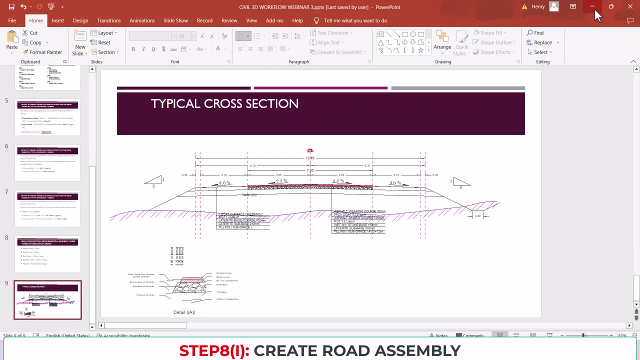 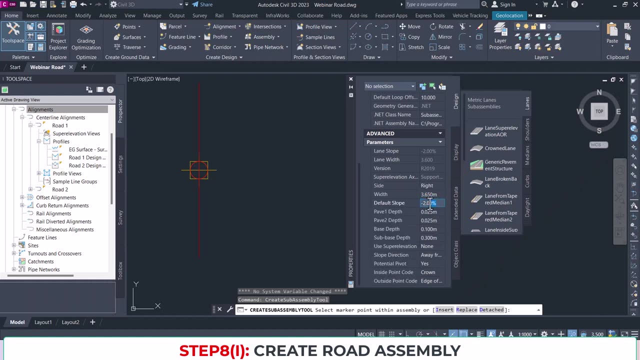 let's model to the right, then our width, if you remember, is 3.65. okay, let's look at the drawing: 3.65 and then our shoulder, 2.75. all right, so our width is 3.65, then our cross loop is 2.5 percent. 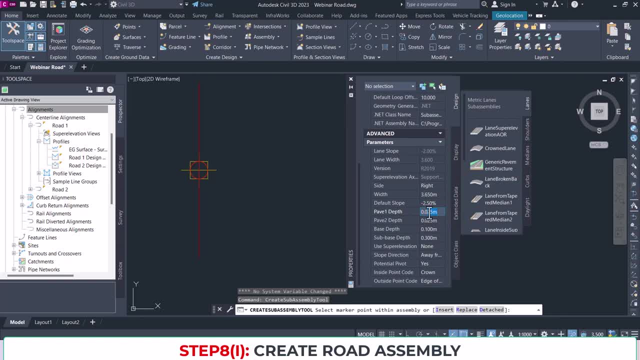 all right, so our pavement depth is zero point. the first depth is, uh, 50 mm, which is 0.05 meters. the second one is 100 mm, the bender, which is 0.1, the base depth is 0.15 and then the sub base is 0.3. great, so leave the every other thing you know as it is. so let's click. 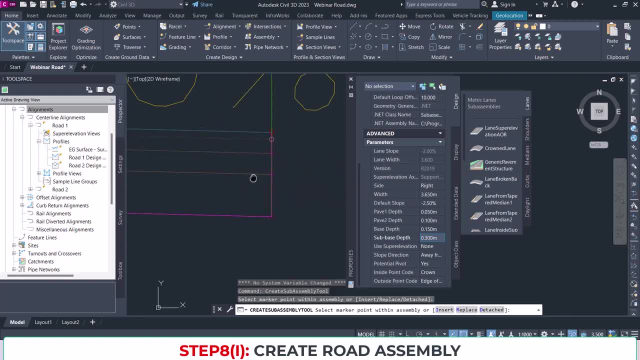 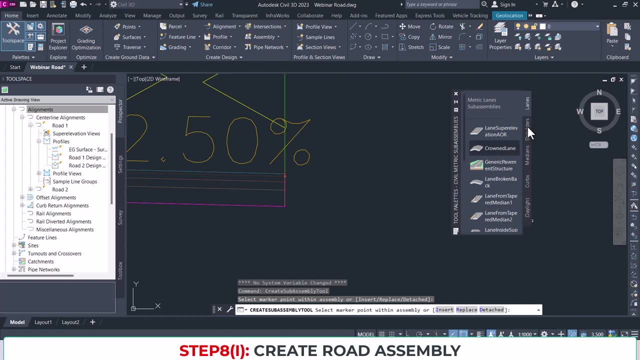 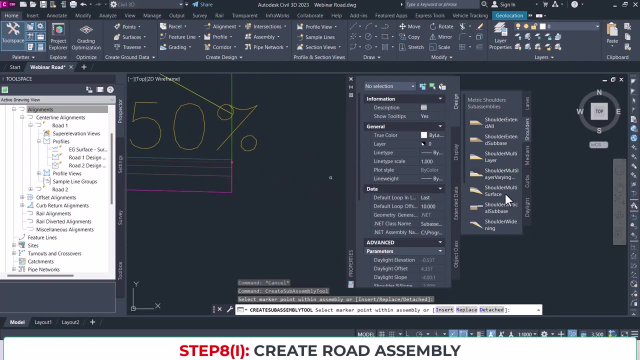 on this. so, as you can see, it brings it up for us here. so the next thing we are going to do is to model the shoulder so you, if you see, you can see should- okay, here is shoulder. so you choose shoulder, extend. all okay, that's the option you can choose. you know there are many, but for now we're using shoulder. 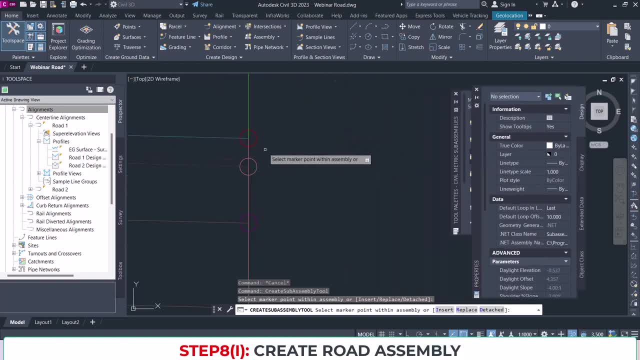 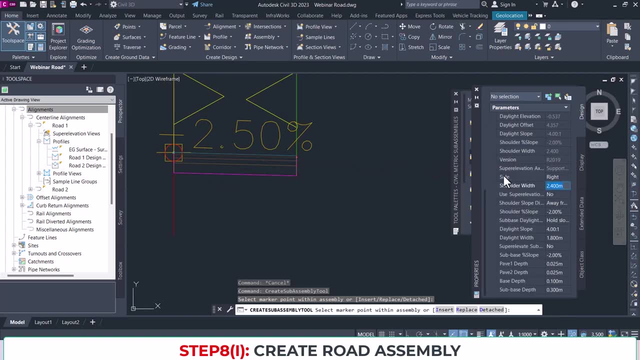 extend. all okay, so let's click. uh, we're going to extend. before that, of course, we are going to adjust our parameters. so, uh, shoulder width. well, the side is right. the shoulder width is 2.75 from our proposed cross section. okay, so away from crown, let's have it 2.5 percent here. 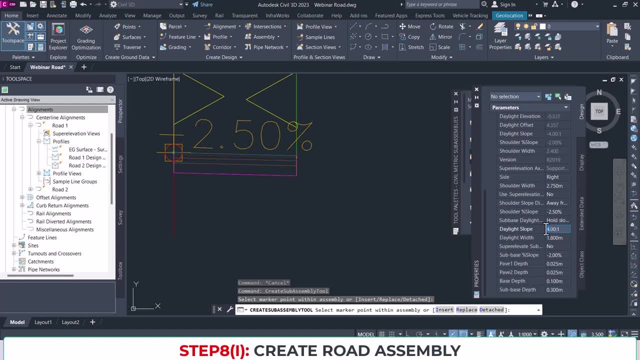 and then the daylight slope- remember it was two is to one. in the cross section we're using the length of the column brightness in this section to is to one, and then we have the cambio objection material displayed. better capture all these things related to you know how it is. so we have this. two point five. 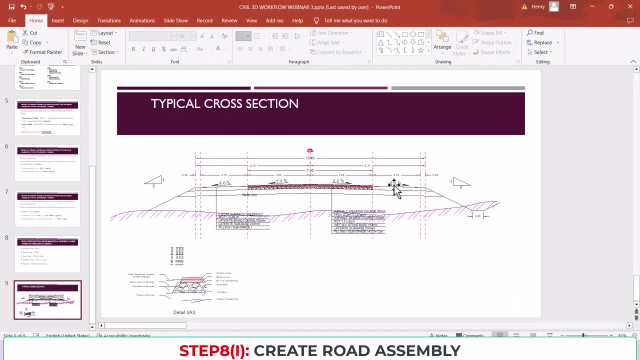 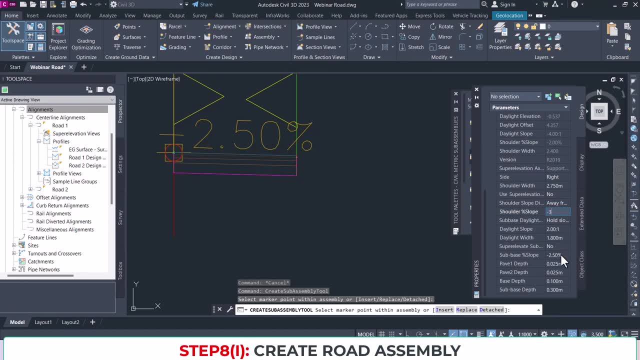 percent. okay, i forgot, i think in the shoulder is three percent. okay, yeah, i'm sure that three percent. so let's just give it three percent. yeah, three percent here show that this low three percent two. all right, so where do we go? that's all the production action procedures described and what is remaining? nothing. so let's extend. 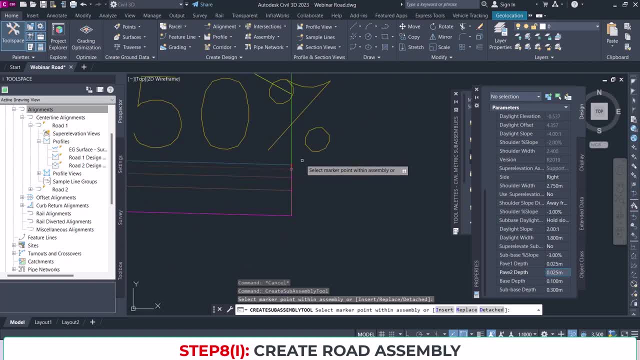 shoulder. now you know, actually we don't have asphalt, okay on the shoulder, but I'm still going to just put asphalt and I don't want to go into all those complicated thing. if I don't want asphalt, I can just make it zero. okay, because normally in Nigeria here we used to do surface dressing, just surface. 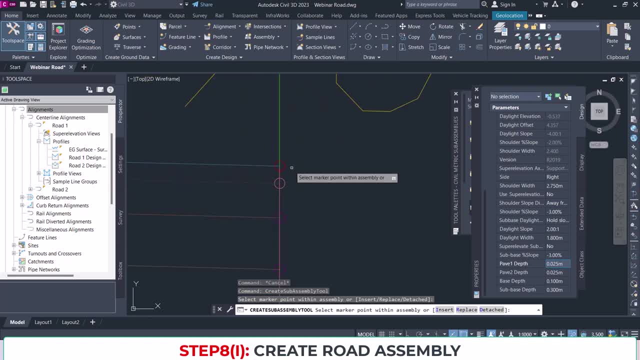 dressing on our shoulders because there is not a travel way. okay, it's just service lane something. I mean, it's just a temporary area, so let's click on this node here and then it extends our shoulder, okay. okay, something out of place here should be: should be 150, but nothing. 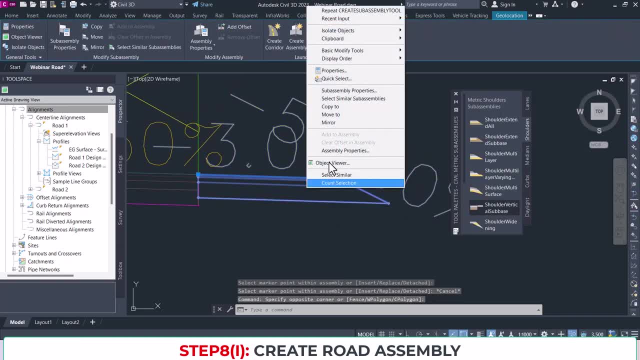 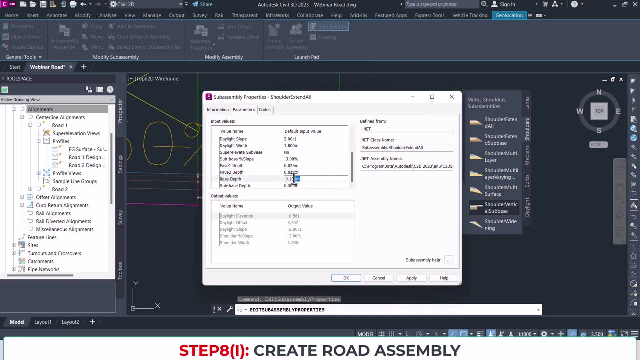 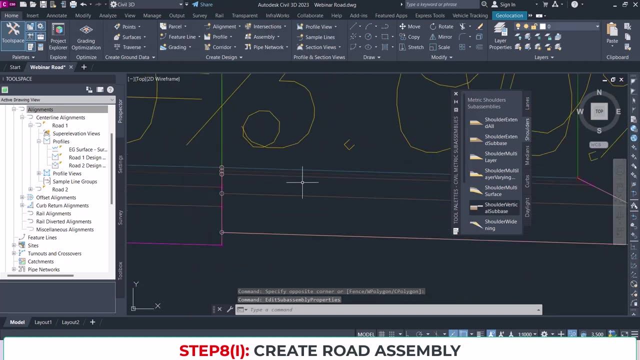 spoiled. you can click on it, right click, and then go to surface assembly properties and then here was supposed to be 15, so let's make it 5 and then press ok. so, as you can see, there's still some things that's out of place. okay, maybe it was. 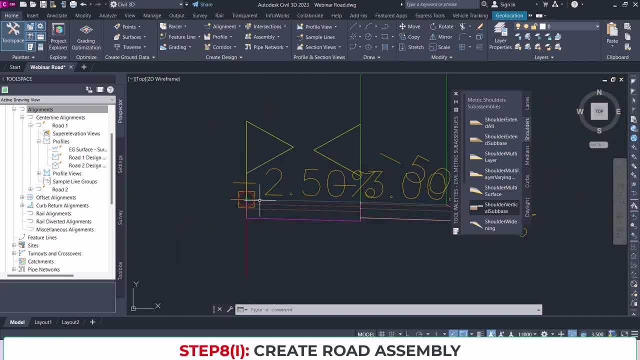 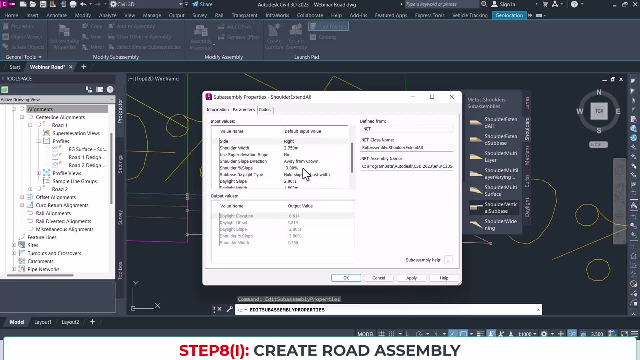 when I was creating this one. okay, okay, let me. let me adjust it again. some assembly properties, if it's not really look as you want, so you can always be adjusting. okay, the first depth is 0.05. yeah, that's a mistake. the second depth is 0.1, and then the third one 150, and 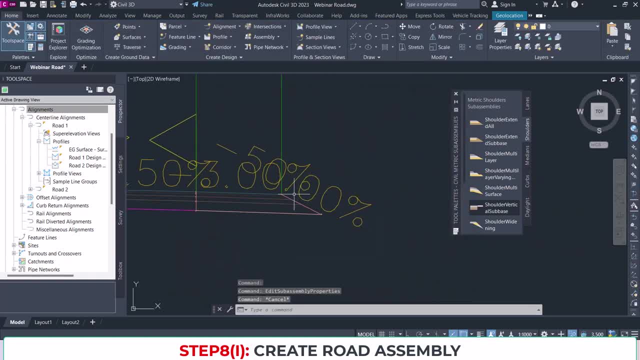 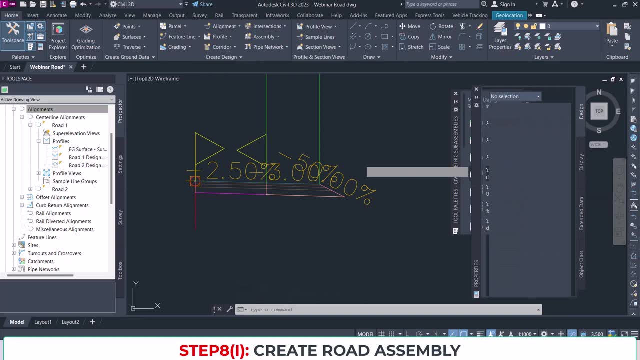 then about: okay, great, so you can see it matches very good. so the next thing is to add our daylight. so we use daylight general, so you can adjust all these parameters. but I don't want to go into all these things always. I'll bore you. but you need to have it to be at. uh. 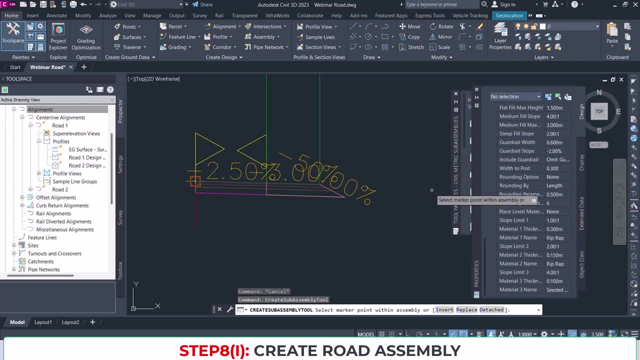 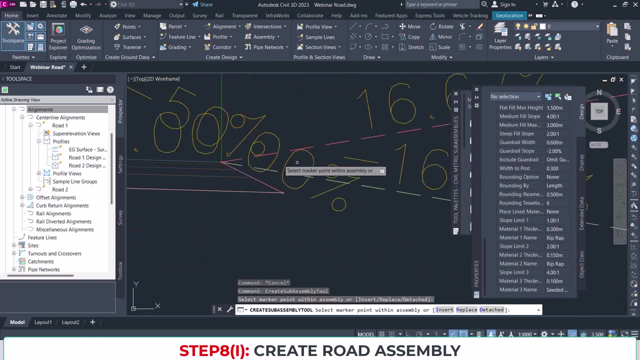 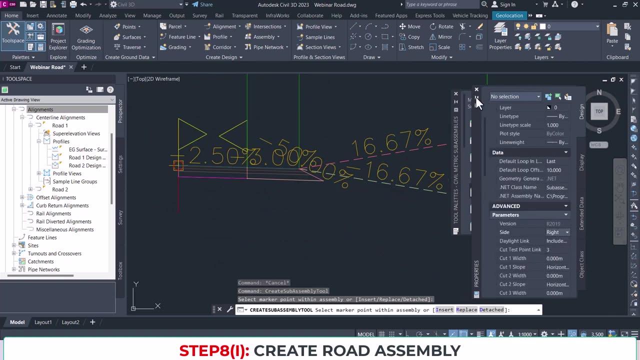 you know, slow cleaning to be two is to one, so, but I'll just put it there for now. this class is already longer than I wanted it to be, so just click on this. okay, you have your daylight. of course, it's to the right. okay, it's to the right here, right here, as you can see. so once I've done that, okay, I can just. 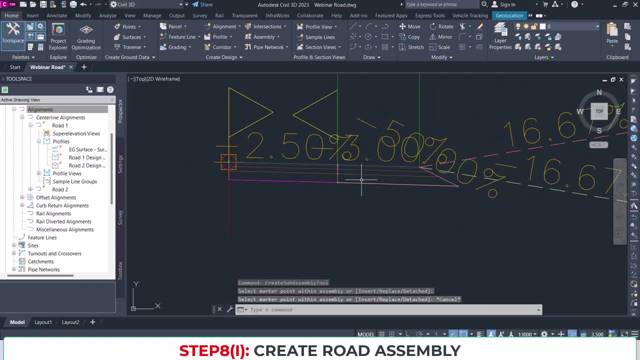 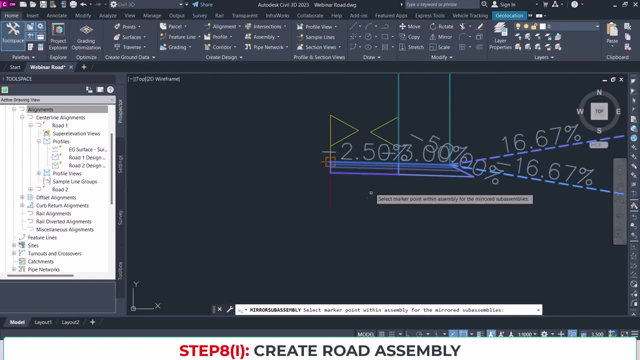 close everything I've modeled towards the right. I don't need to model the left also. okay, I can just mirror it. so what? I'll just do? I like everything and then click on it, and then I'm going to go to my middle and then click my middle baseline so it mirrors everything to the left. so very great this. 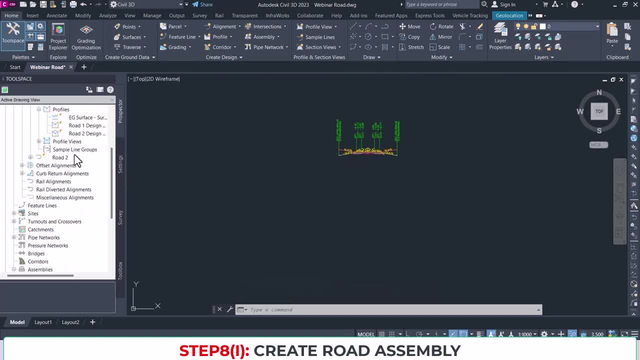 is my first assembly and it's called full assembly. if I go to my prospector tab and go to assemblies, I can find that full assembly here. all right, so great, so um, I can now, you know, create my corridor, but before I do that I would need some assemblies. I'm going to just create it. 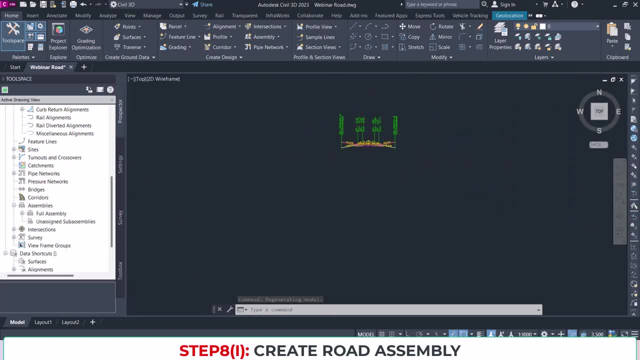 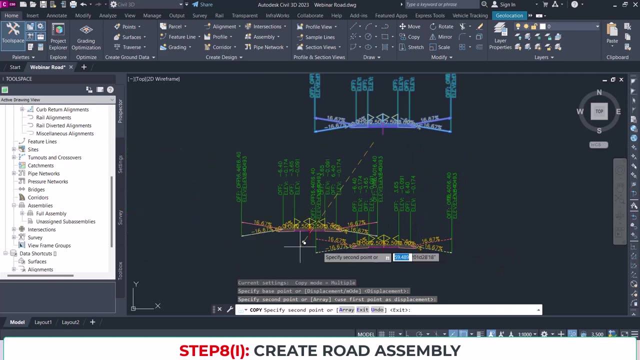 right away and I'll show you where it will be used. so I need half assembly to the left, half assembly to the right. so I can do that by modeling the whole thing again or by just simply copying this assembly. copy downwards as I'm copying it downwards: watch closely here. you see, in the um. 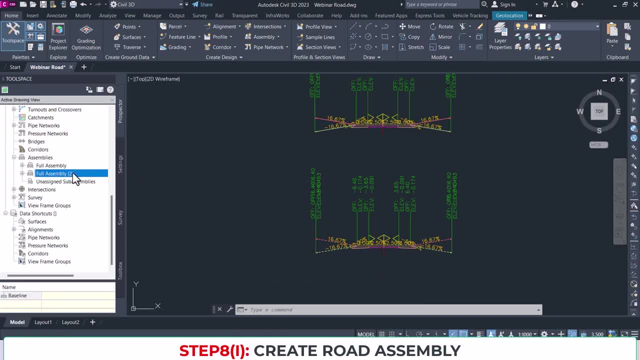 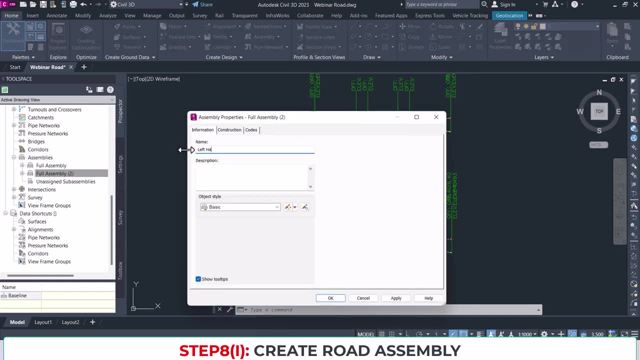 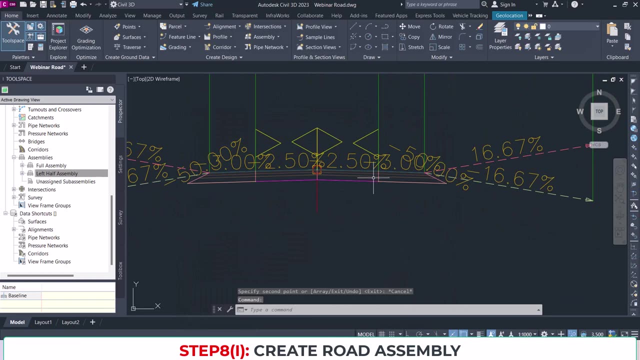 assembly it. it names it as a full assembly tool, but I'm going to name it again. give it another name, uh, as um left, half assembly. okay, and then I'll press: okay, um it left, because I'm going to delete all the ones that are to the right. I'll click all the links to the right and delete them. great, so I have. 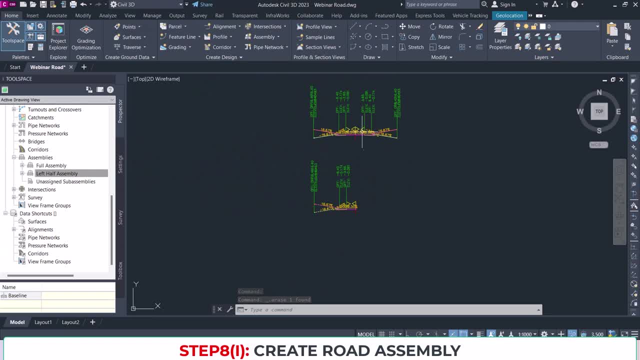 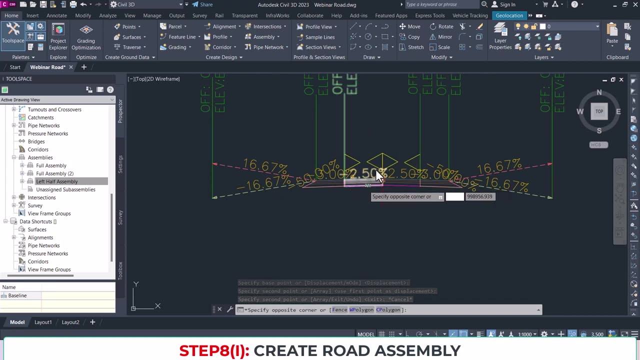 a left half assembly, all right. so what do I do? I also have to create a right half assembly copy and then create, um, delete all the ones this way. okay, I'll delete everything to the right, okay, one after the other. so that's all, everything to the 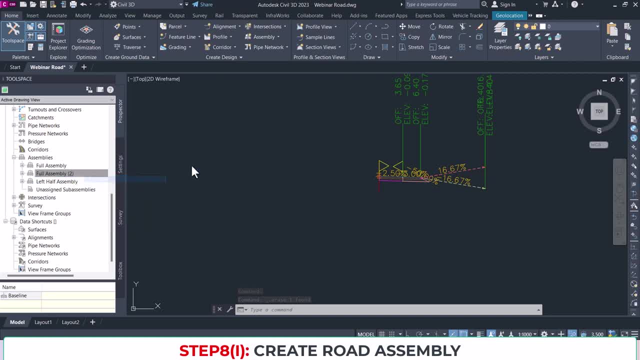 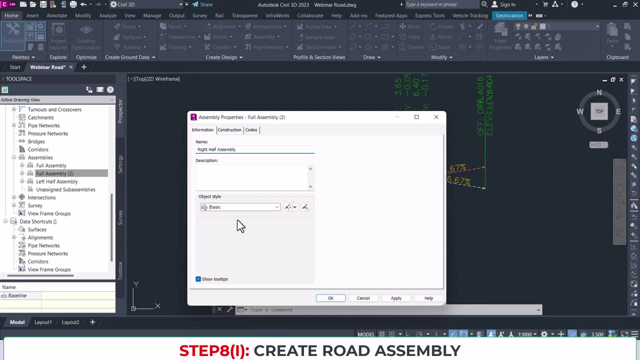 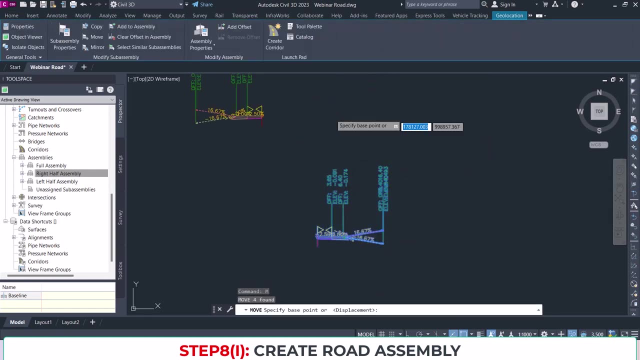 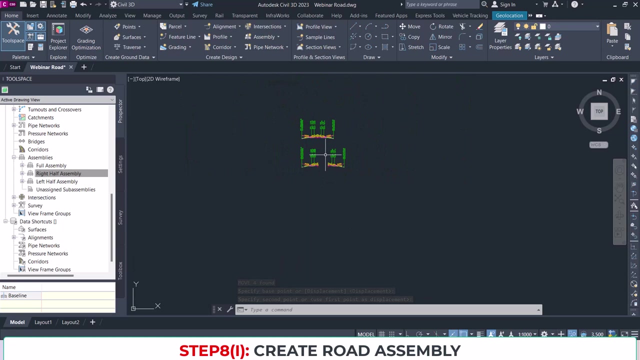 left, so I have already the right. so I will rename it to right. half assembly right, have assembly great. so I have have something to the left, to the right, so of course I can move that. so I'm going to create a curve returns assembly. that one is a little bit tricky, just follow me. 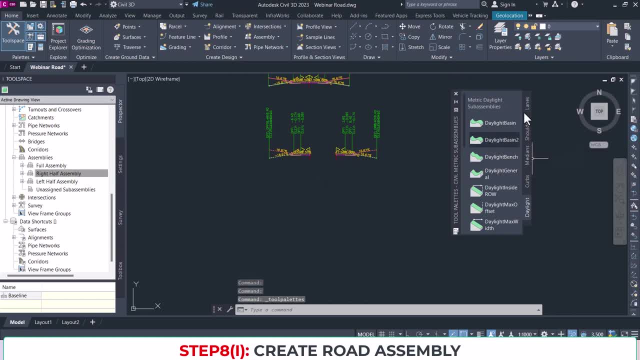 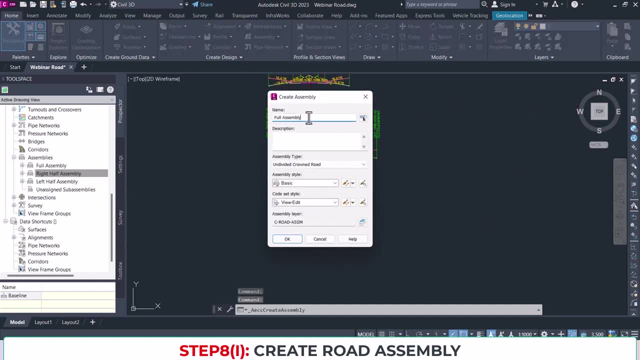 and since it's a video, you can always watch it back again. so I'm going to- yeah, sorry, I'm going to create assembly. this again: create assembly. I'm going to call it left curb return. okay, and everything remains same還左右一樣. 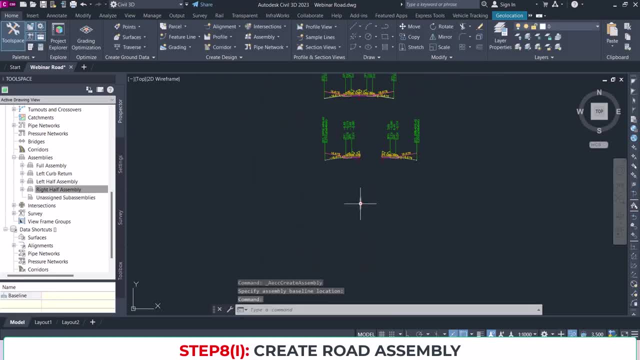 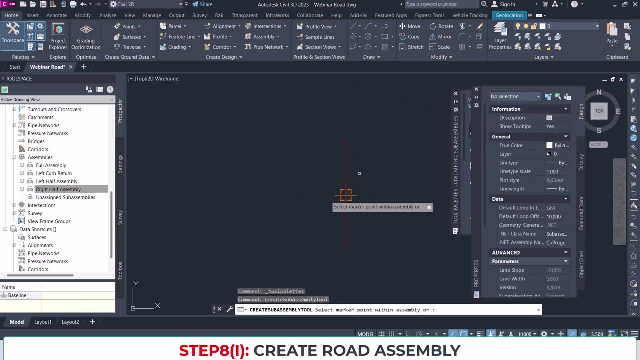 everything還一樣, okay. and then i click on it, it zooms in for me, okay. so i open my two palettes again and then i go to lanes and then model means qualification. now, this time, as i'm walking to the right, i'm 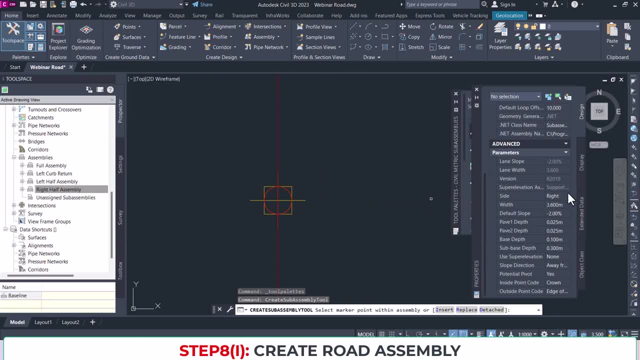 actually walking towards the left, okay, because you'll see that in a moment. so i'm working to the right and my lane is 3.65 meters, okay, and then, if you- my cross slope is now here- i'm going to choose, you know, two percent. okay, i'll show you why i do that. i want to not be minus two percent, so 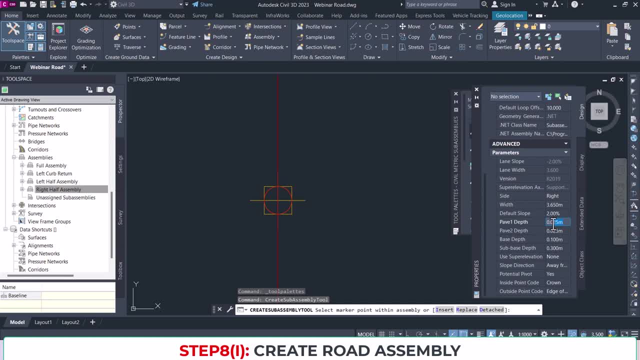 let's, uh, have all these things as we have it in the previous one: 0.1 here, 0.15 here, and then sub it at this and then everything. so let me click on that now. yeah, you see, it's sloping towards this side. oh, i put it two percent. it should be 2.5. i can also adjust that here once i've created it. i. 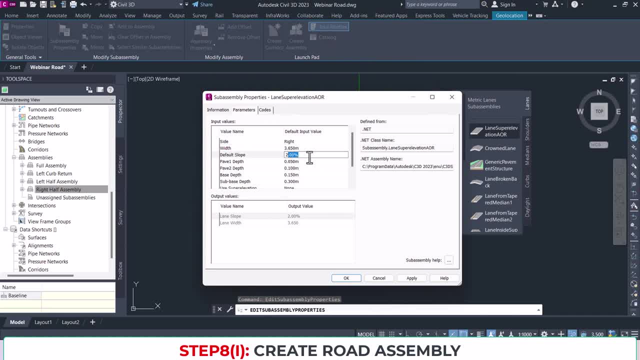 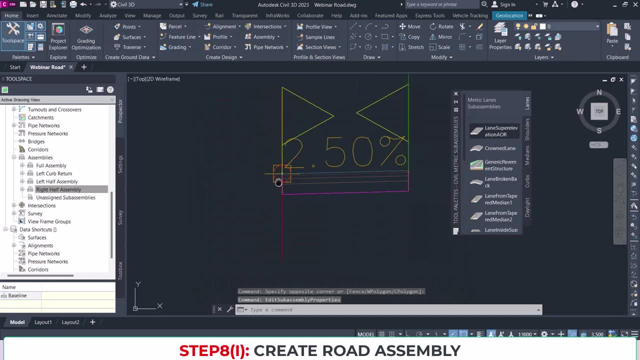 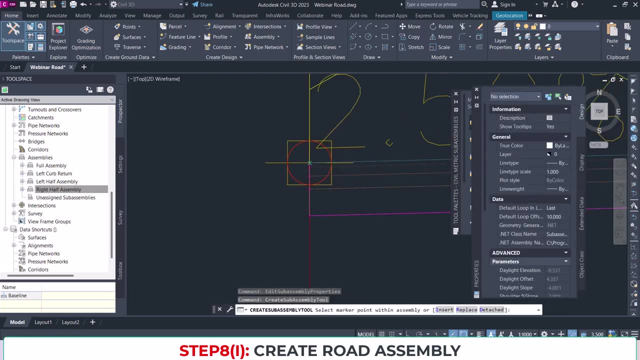 can just adjust it here to 2.5, five, five, five percent. so press, okay. so now i'm going to be putting my shoulder to the left here. okay, so my shoulder is going to be shoulder extend all and going to be putting it to the left. okay, just follow me. 2.75 and then the cross low is three. 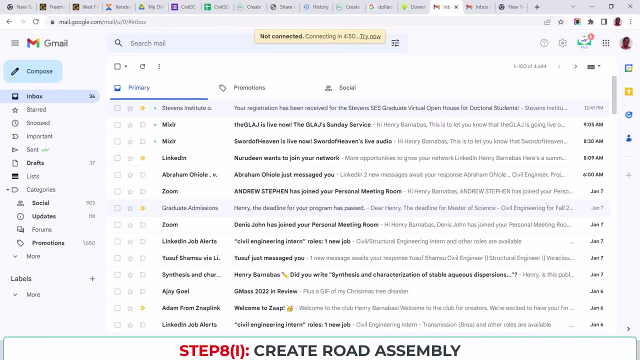 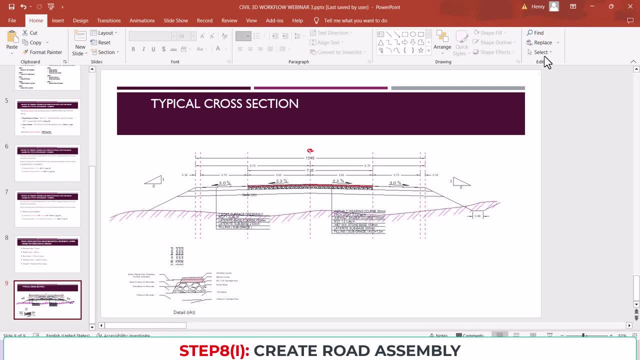 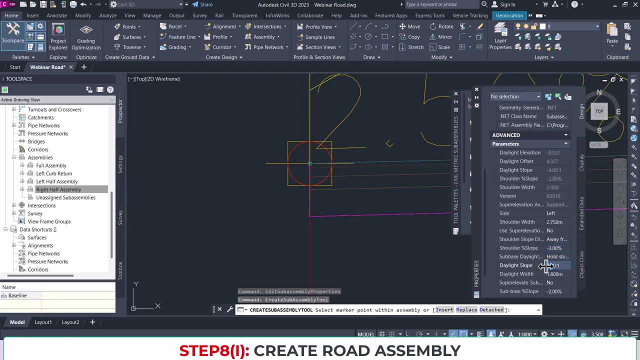 percent for the shoulders. okay, i believe it's three percent. sorry, this is the shoulder. okay, this is the shoulder. three percent. i forgot in the previous one. we're going to adjust that, all right, so, uh, then the daylight slope is two is to one, okay, and the depth? oh my god, this is not mess for in this case, so i have to put in everything again. 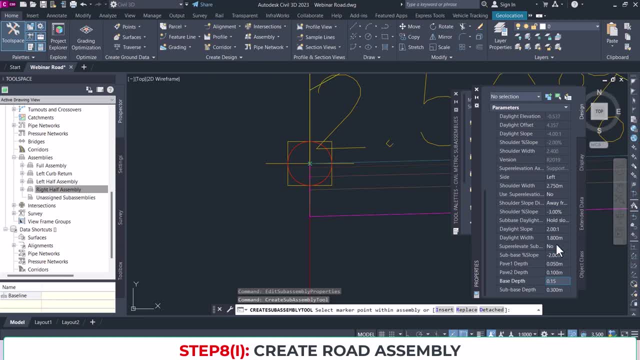 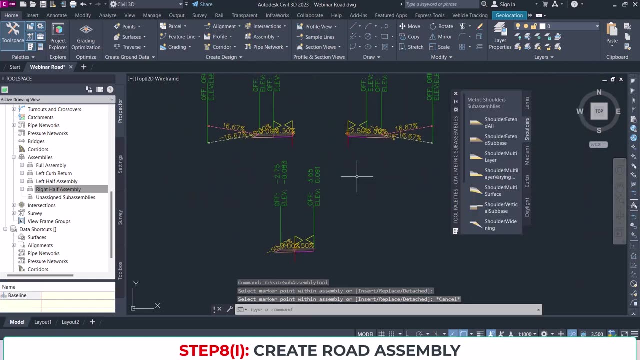 so, and this one is 0.15. all right, so there we go, okay, so i think everything is fine, so i'm going to extend it to the left, so i'm going to select this, okay. yeah, so it's selected to the left. now, as you may notice, these things look big, the description just because of the skill. okay, if i 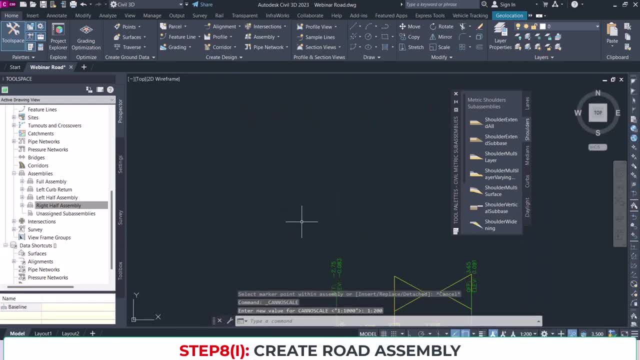 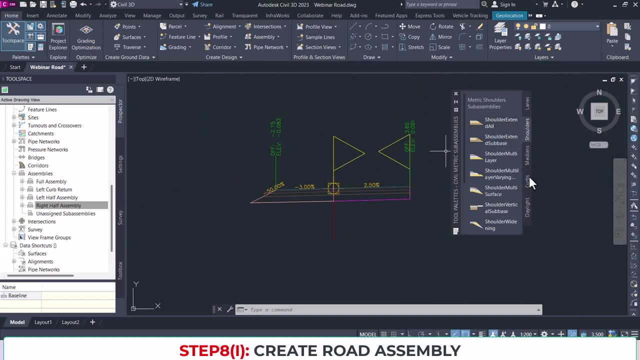 choose that. if i change it to the left, it will go to the right. okay, so if i change it to the left, i reduce it to. one is a 200. okay, it looks nice, better, okay, so let's add our daylight daylight. okay, what's daylight? we have daylight, general, okay, and it's. 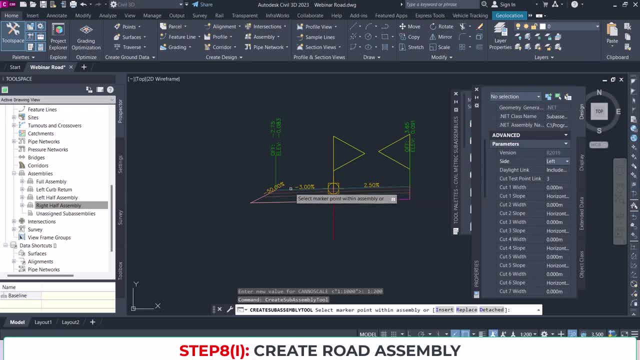 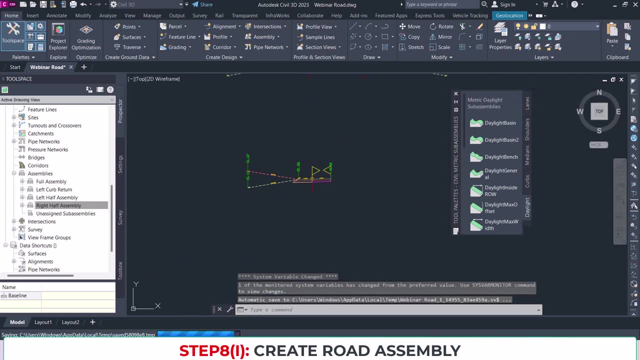 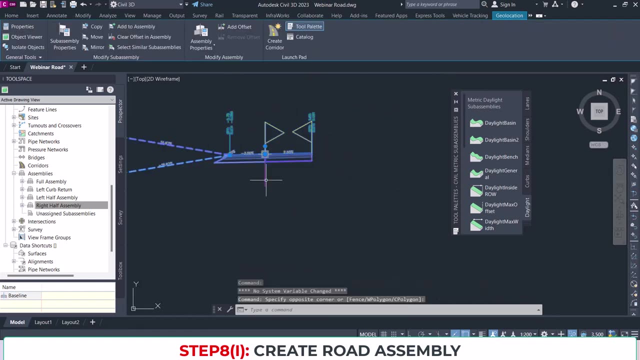 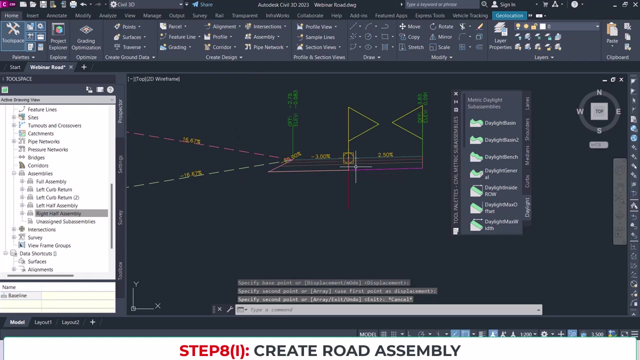 going to be to the left. okay, just put that here. all right, so that's my left carb return. I can model the same thing to the right. okay, well, let me try copying this and then mirroring everything. okay, copy this. okay, and then new this one, mirror this one, mirror it and then the one. then select this one. 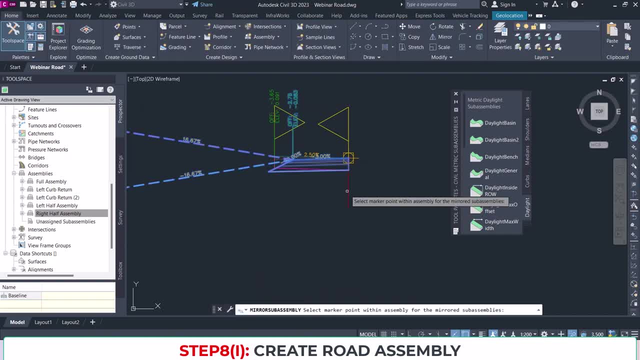 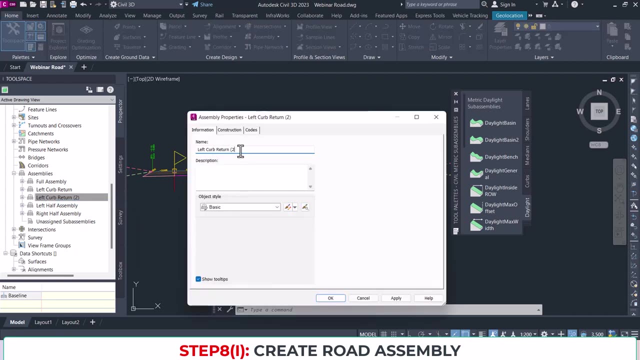 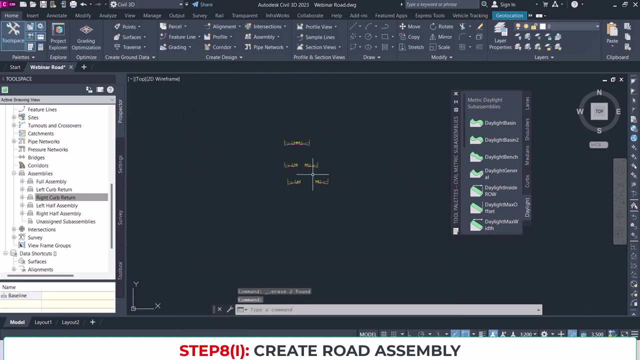 and this one, okay, and then delete the ones middle. so I've just created and awful right, so I'm going to call it, rename it. I'm going to call it, go to okay. so this are the assemblies I need for my corridor. first of all, I'm going to create the corridor. 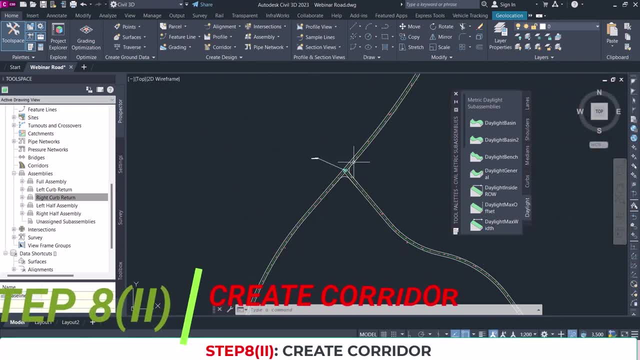 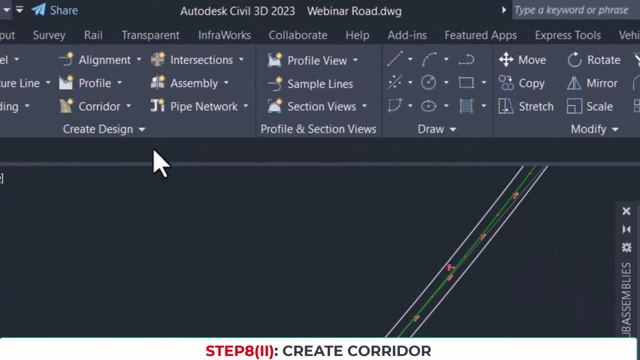 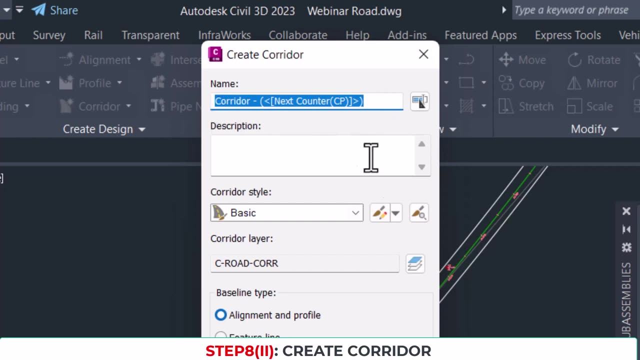 for the name and then two. okay, so let me go to create corridor. i'm going to create corridor, then, uh, we can have a template, but you know we need only one corridor actually, because every corridor, the intersecting corridor will be tied to the main corner, so i'm just going to call it main corridor. 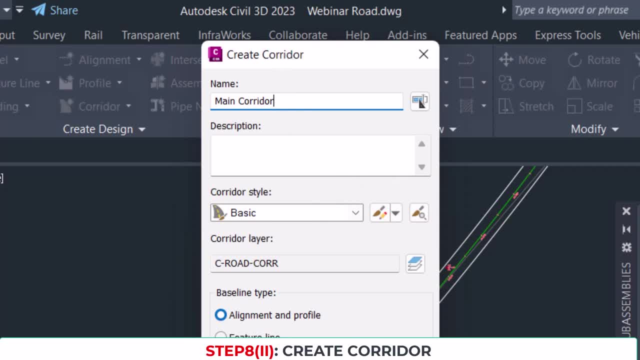 simply all right, i'm not going to create another corridor, i'll just add a region and baseline. you'll see that shortly. so i'm going to use just the basic style. i don't have, you know, unless you want to create a new one. this controls how it looks, so, uh, and then it's going to. 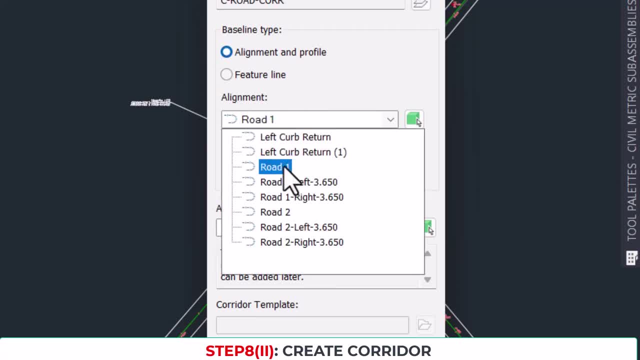 be an alignment and profile, then which alignment we need to do on the one, and we are going to use the design profile. oh, we are having two profiles here. what does this mean? okay, this one is the superimposed profile that we we did. let me go back and show you that, okay. 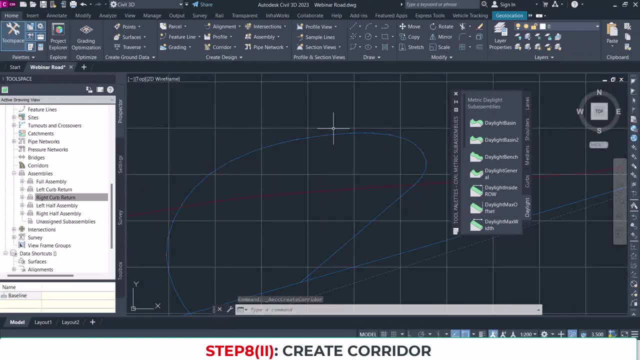 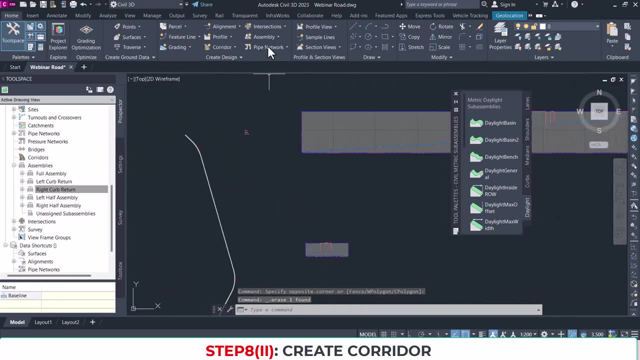 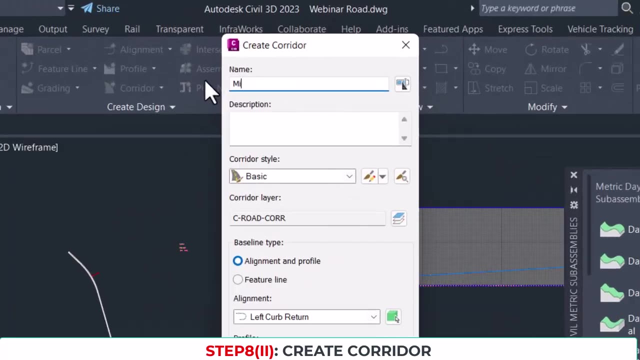 you remember we had this superimposed profile. actually, when we were done with it, we should have deleted it. so let me do that now, once i delete it, okay, and go back, uh, to creating my corridor. okay, i will not find it again, so let me call this main. sorry. 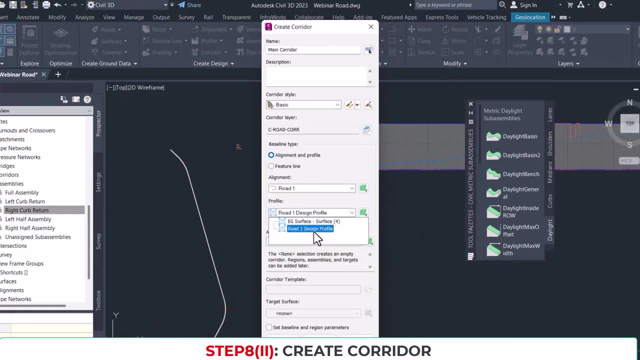 and then everything back and then i'll choose one. so you see, it's just that design profile. so the assembly we're going to be using is a full assembly and we are targeting to the bottom of the screen. so we are going to use the full assembly and we are targeting to the 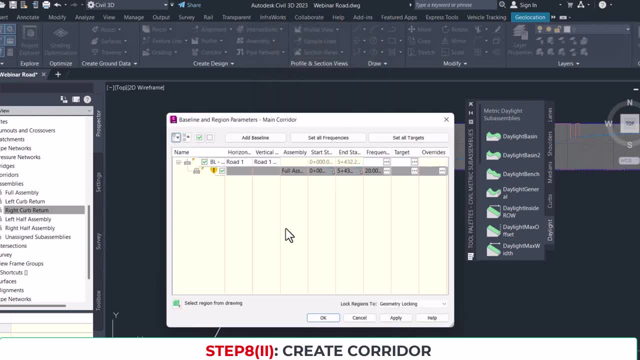 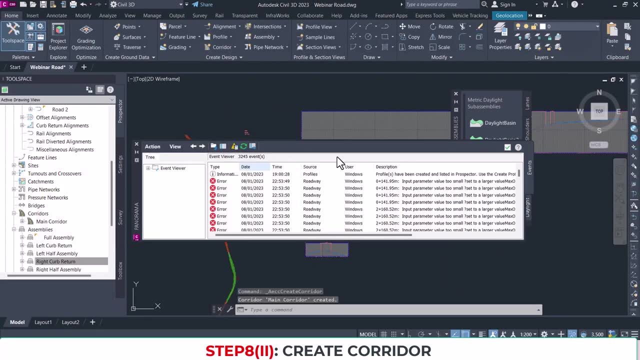 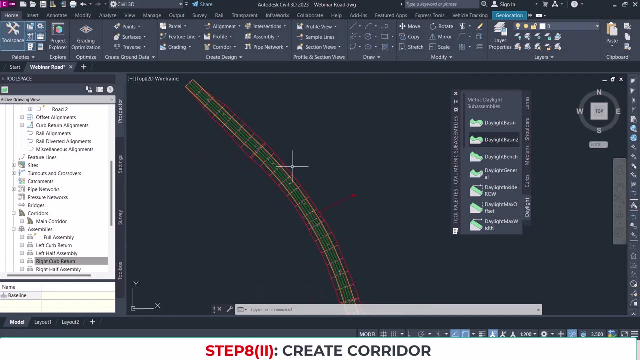 existing glass surface. so once this is done, you click ok and then you press ok to rebuild the corridor. okay, so once you review the corridor, you can watch and see how it looks. okay, already we are looking at these places. we are going to be having cuts here. that's why it's a red color, these green 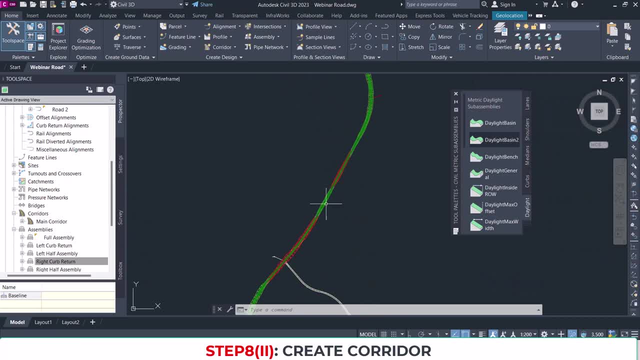 are areas of field. the red are areas of cut. okay, automatically showing what's happening already. so let's now move on to the next part of the video. let's move on to the next part of the video. let's now move on to the next part of the video. let's move on to the next part of the video. let's. 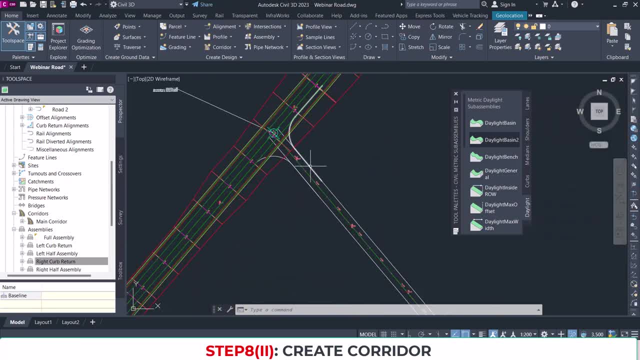 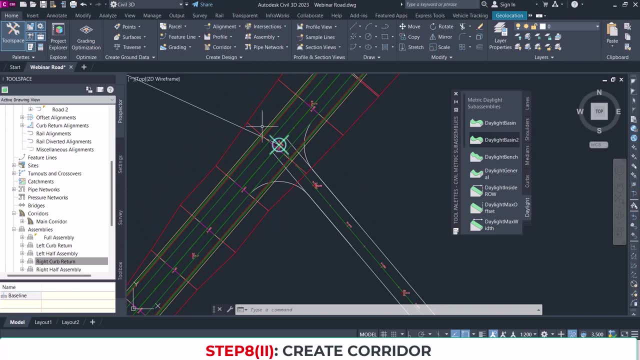 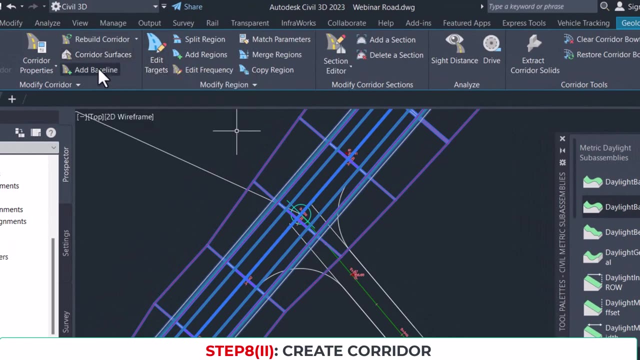 to. you know, adding corridor for this one. now you, you don't have to create a new corridor for this one, you just add it as a baseline, all right? so, uh, we are going to add click. just click on the corridor and press, um, you know, add baseline. so once you click on add baseline, now it asks you: 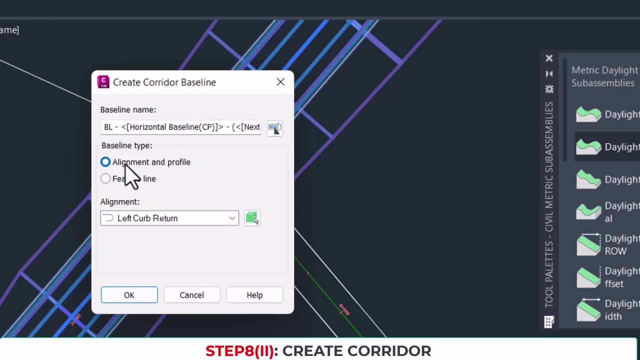 to name it, but we can just leave it to have this default name. it's going to be an alignment profile and what alignment is going to be? route 2: you can do that by selecting the drop down or, if you don't know the name, if you have multiple alignments, meaning this drawing already, you can just use this and then. 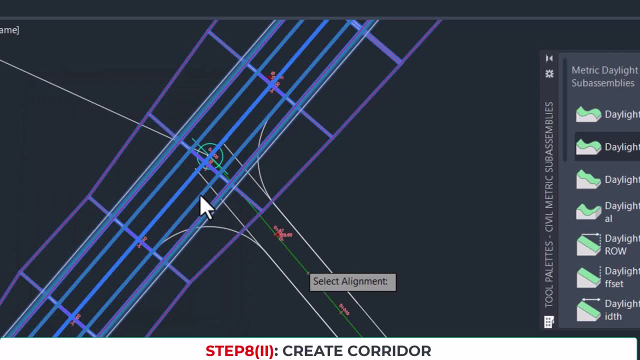 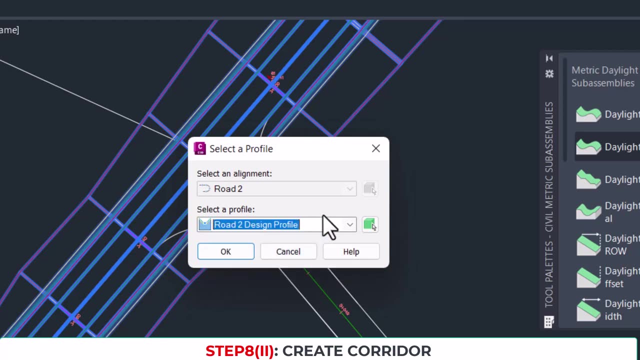 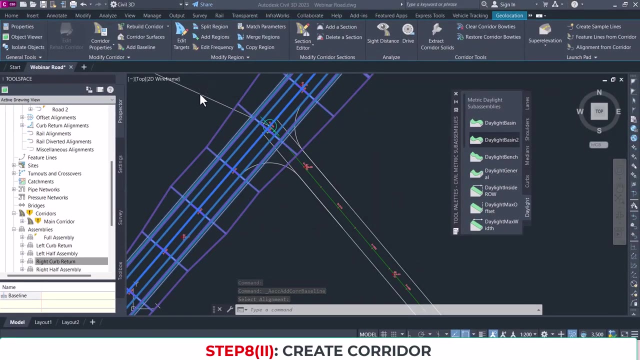 click on this and then press ok. ok, once you have done that, you have to select a profile. now the profile is going to be the road design profile, all right. so you press ok. so we have created a baseline for this. now, what does that allow us to do? it allows us to add a region still on the corridor. 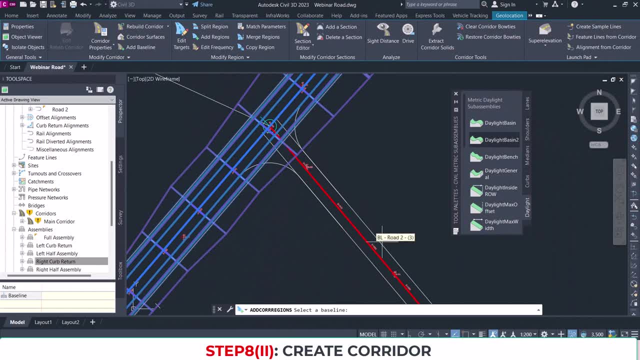 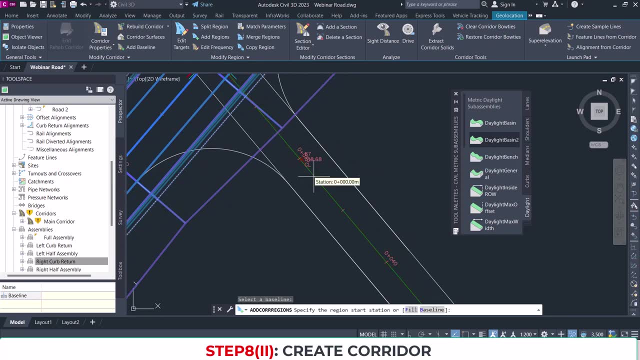 so we are going to add a region and if you hover around you can see that the baseline has highlighted. so we are now going to click somewhere before the cup return, you know just anywhere, and then that will be a starting point, and then we are going to start from here. from here, okay, and then 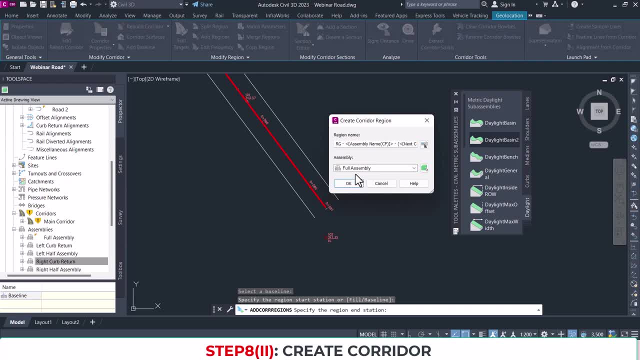 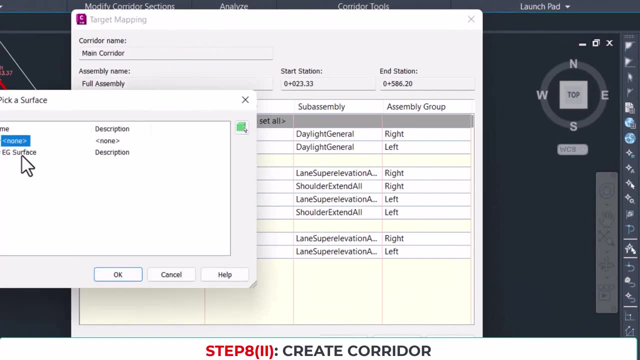 go all the way to the last point of the alignment, then which assembly i want to use? still, we are going to use a full assembly press. ok, again, here we are going to be targeting to the existing ground surface. let's leave that for now. everything should remain the same in this case, here. 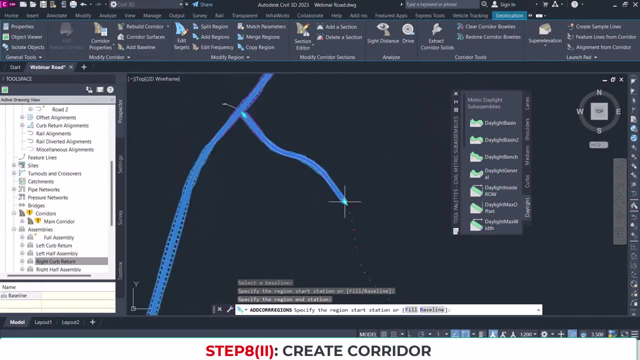 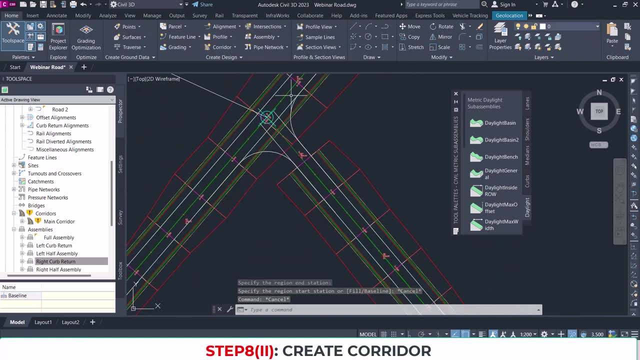 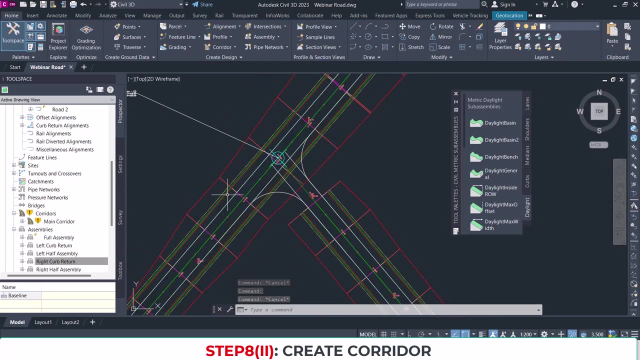 so, and then you have modeled your corridor. can you see that? right, beautiful? you can see that it is one corridor if you click on it. all of them are tied to each other. so one thing is: we are going to split this corridor at this for the road one. okay, you have to split it, you split the. 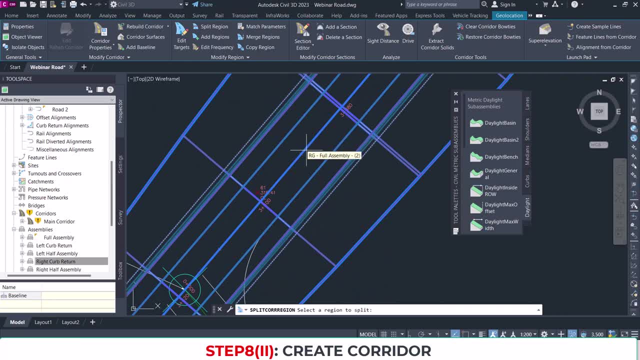 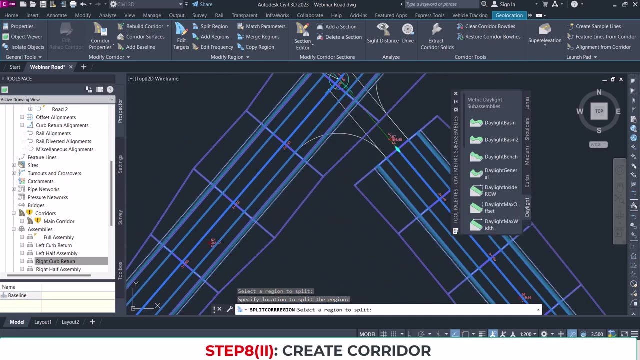 region. you see why i do that recently shortly. so just double click and click again anywhere here, okay. once you do that, it has split the corridor there. it's still highlighted. so click somewhere here, okay. and then click the corridor. click to split again. so great if you can see we have split the corridor at here and this point. so 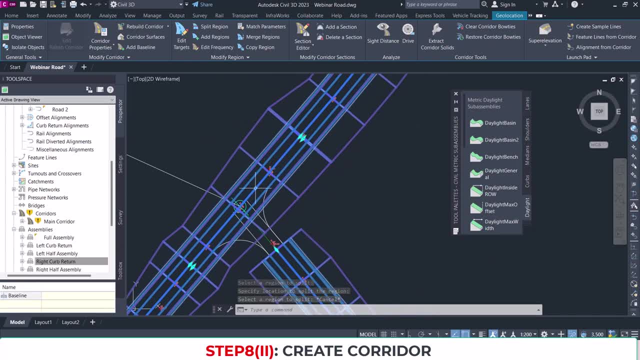 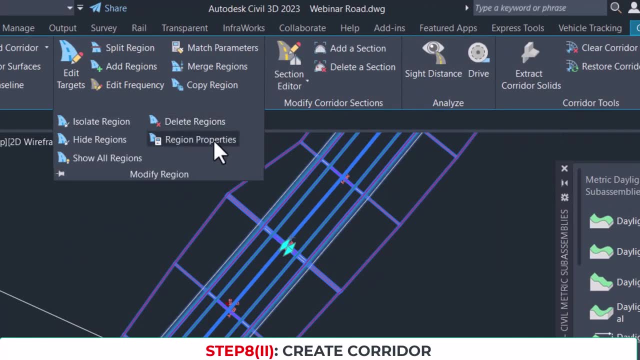 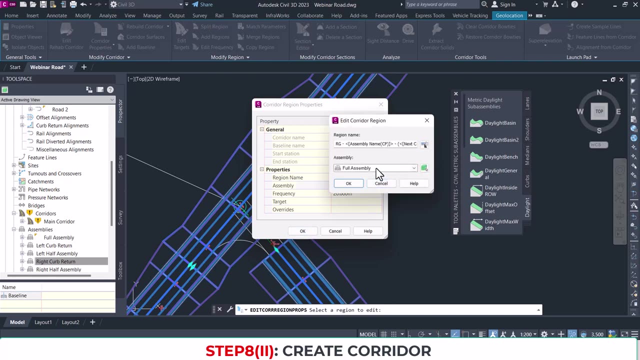 are going to change the corridor section or the assembly section- assembly for that region. so let's modify that region. okay, we just use region properties and click on this place. now you can see that we are using full assembly here. here let's choose: right half assembly. okay, right half. 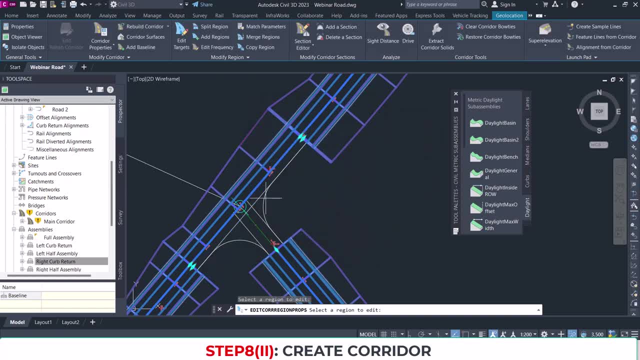 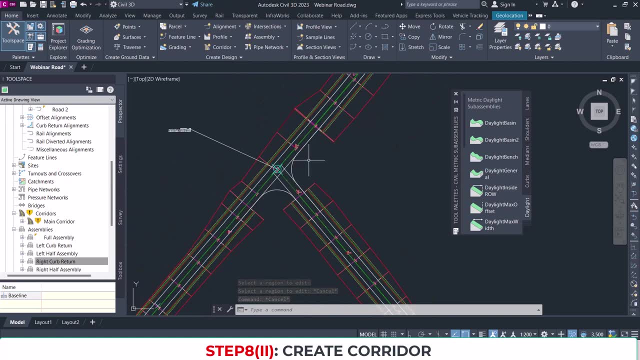 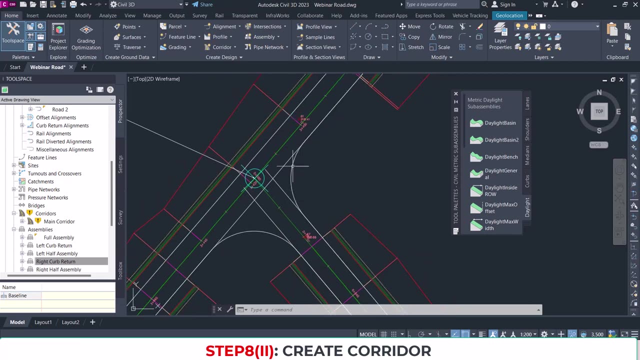 assembly and press ok, okay, you can see that it have deleted the left side and then using only just the right side, because that's what we have created. so the next thing is to add- you know, our cup return uh, corridors, okay, so let's quickly do that, but before we do that, we have to add them as 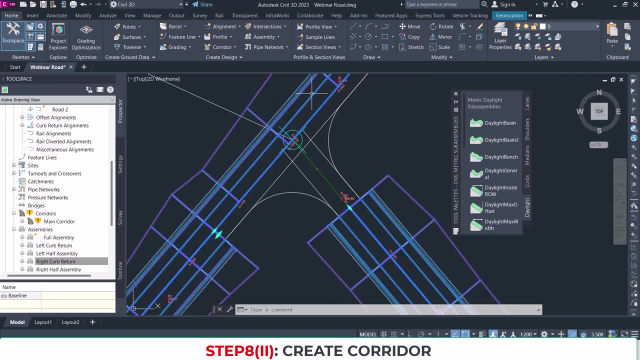 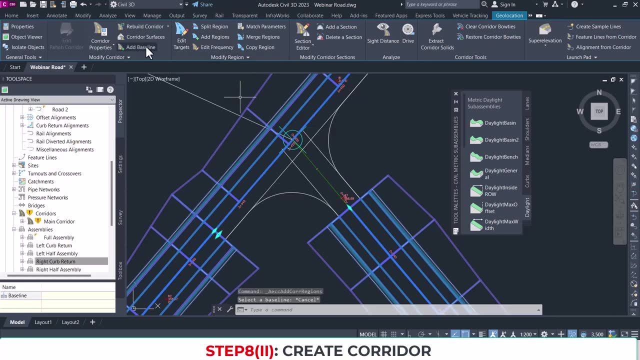 baseline, otherwise when you want to add a region, you won't see anything to add. let's say, add region. you cannot see anything on this cup returns, so you have to first of all add it as a baseline. okay, then you have to select the cup return if you don't know the name. of course, an alignment. 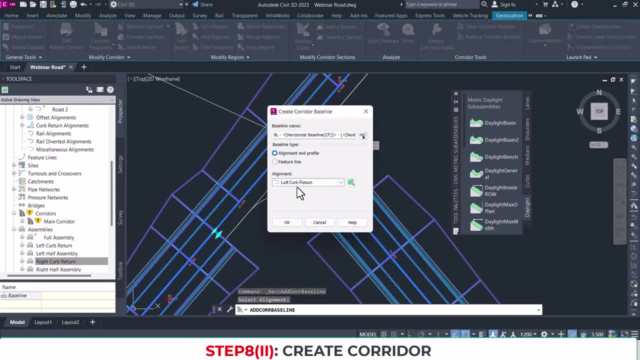 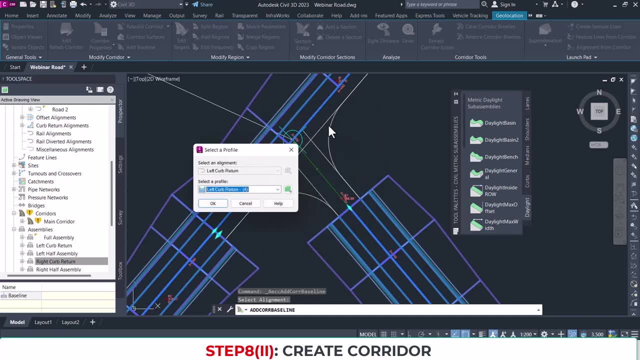 and profile. you can just use this box here to click on it and then update the name. then press ok, all right, okay, oh, we should have named it the right cup return. okay, i made a mistake, you know, originally, so pardon me for that. so we are going to use this profile, so let's press ok. so i've. 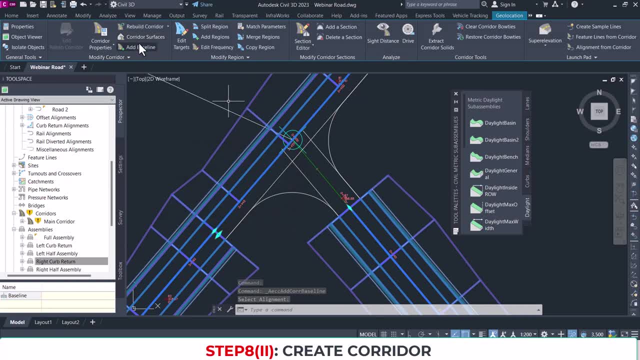 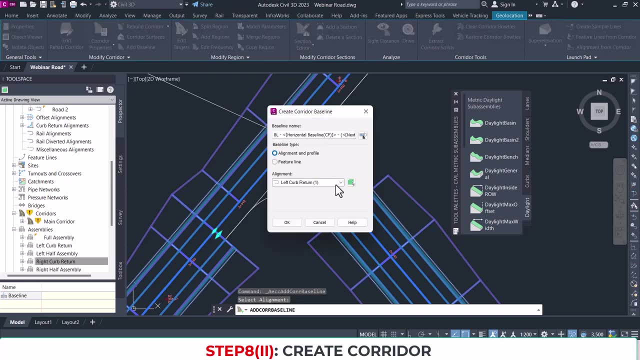 created that copy tone, so let me add another baseline, okay, so i i will select this one so you can see this the name. this one should be legitimately the left and then this one the right. okay, so i named it wrongly at that time, sorry. so, okay, so let's go on. i've created. uh, now select the profile. 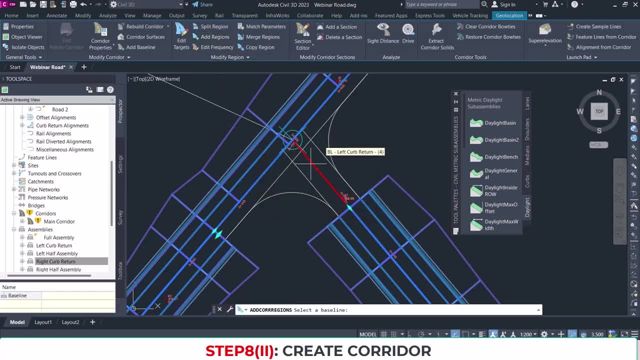 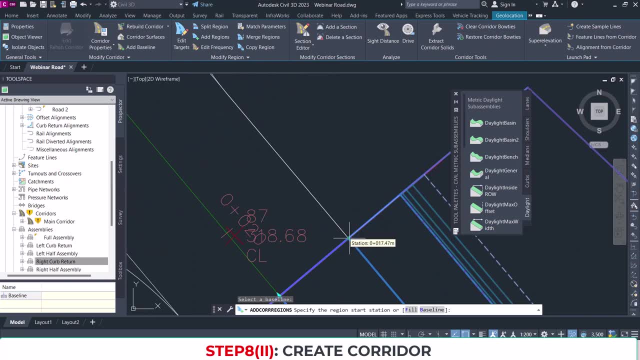 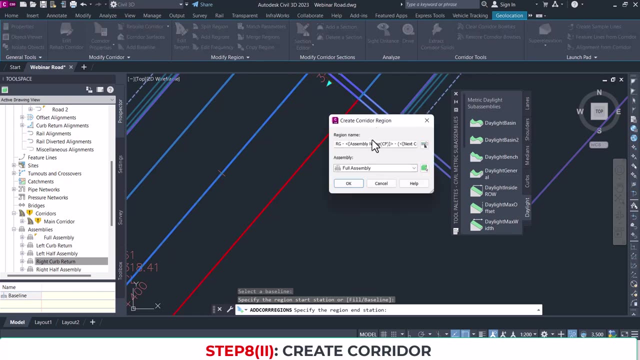 i've created a baseline. now, if i want to add a region, you can see it will be highlighted in red. so that's what i'll quickly do now. i'll click on it and then start sweeping from the intersection of this to the intersection of this. okay, great. so what assembly am i going to use? i'm going to use. 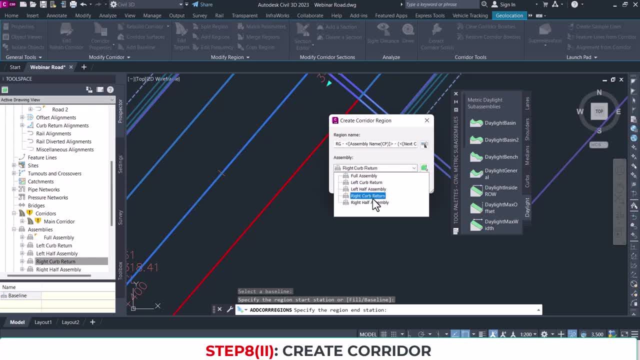 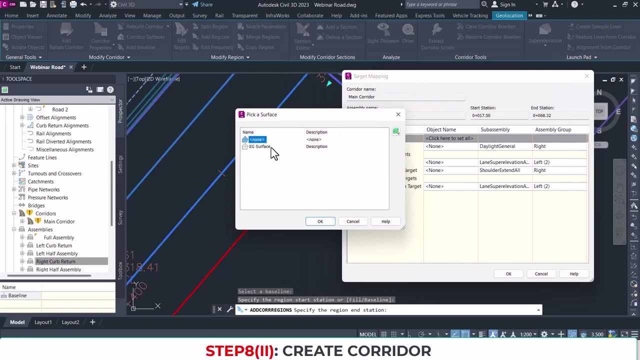 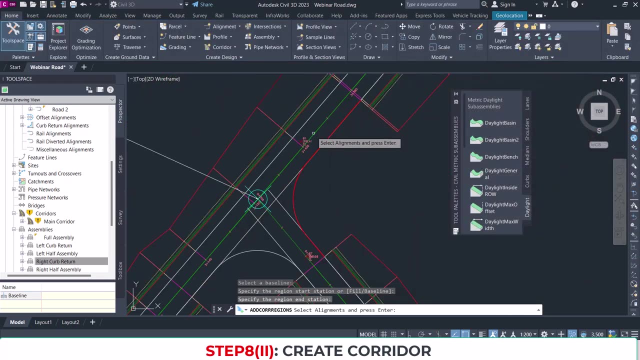 the right uh cup return. okay, i'm going to use the right computer. okay, all right. so when we are to target, we are going to target the existing ground surface and then, for the width targets, we are going to uh target the center line of this. okay, let me just use. 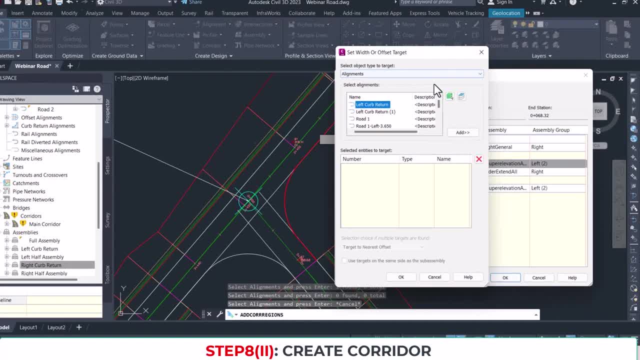 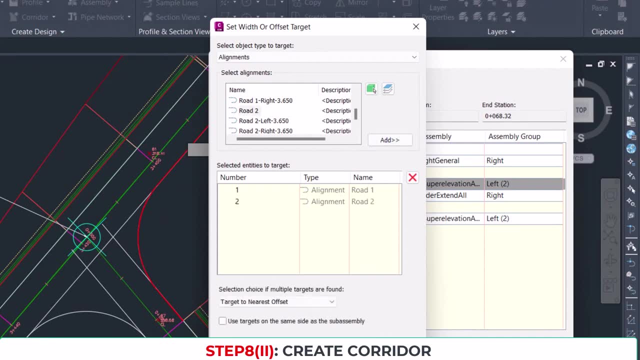 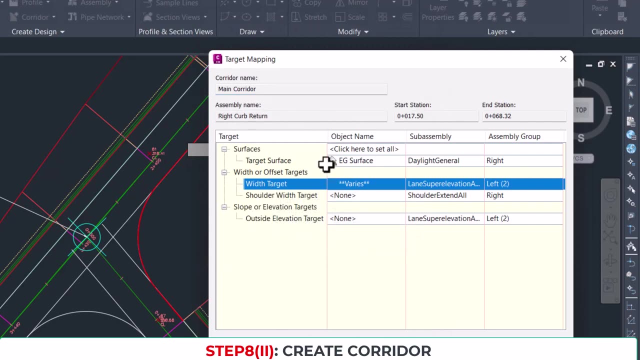 uh, okay or okay, let me not just stop on myself on selecting. let me just select with one and then add. select root two and then add okay. once you do that, then that will be the targets and then for the, we have selected the targets for the horizontal. uh, for the. 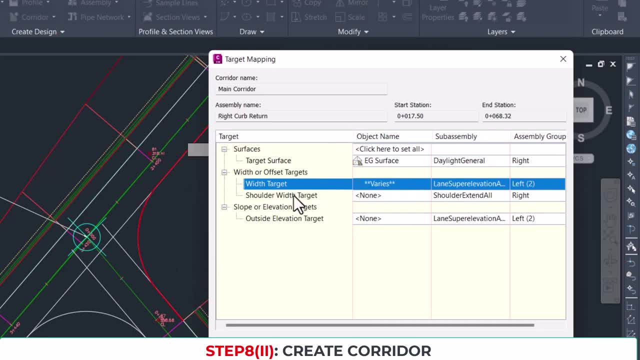 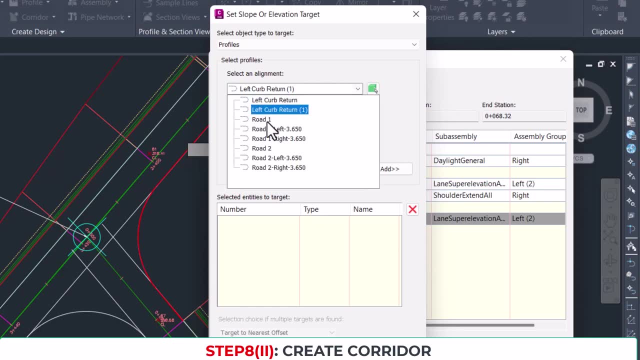 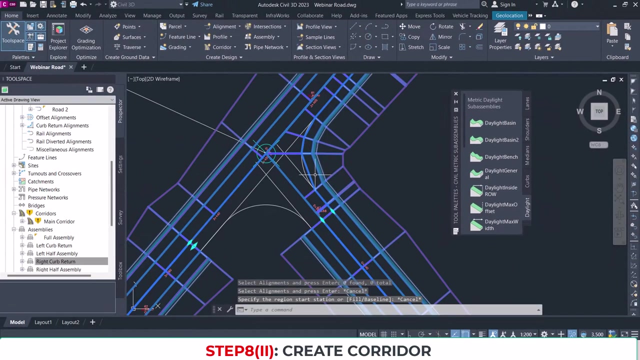 you know alignment, let's also select the targets for the- the slope. okay, for road one. we are going to select the design profile. okay, we are selecting targets for the. you know elevations, so we press ok and then press ok. great, you can see our corridor has been built around this cup return. 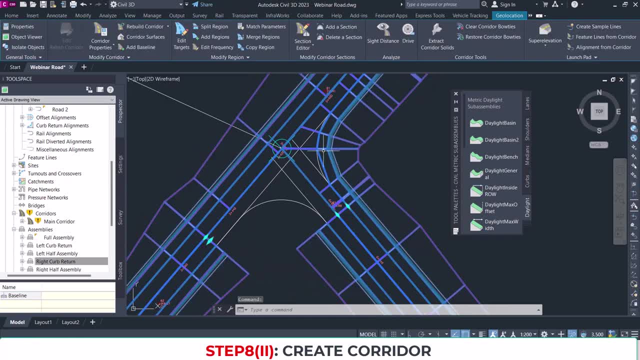 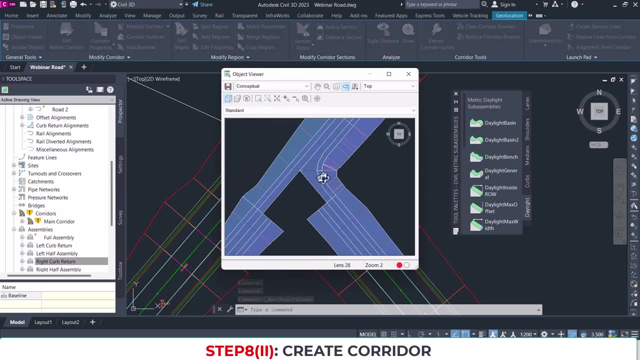 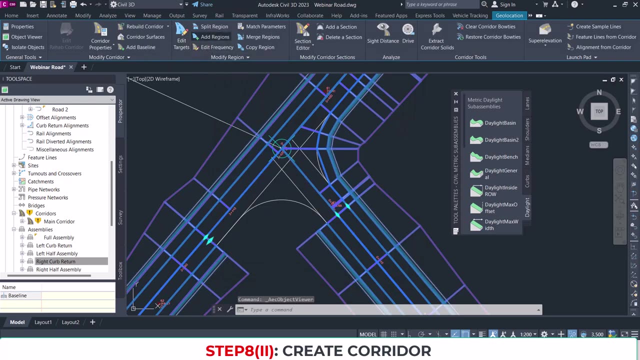 great, perfect. so let's, let's quickly view that before we are done. go to object viewer. then you go to, you can see beautiful, beautiful. so it's remaining the left one. let's, let's quickly create the left one. so again, we just go to add regions. you select here, you swipe. 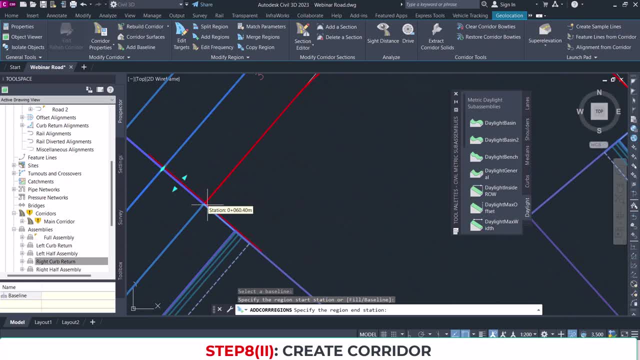 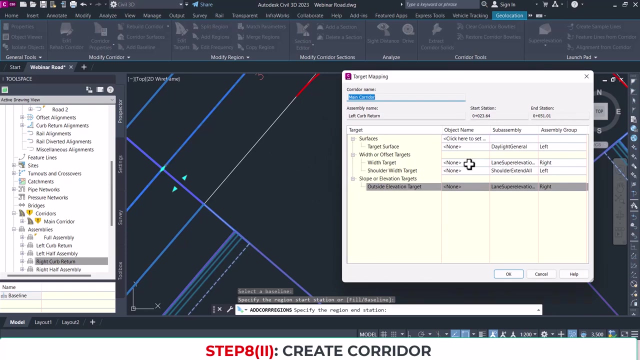 from here and sweep up to the intersection here. okay, all right, i should have an intersection snapping what's happening. okay, so i'm going to use the left cup return in this case. okay, and then i'll be using, i'll be targeting to the existing ground surface and then, for my width targets, i'm going to be using the. 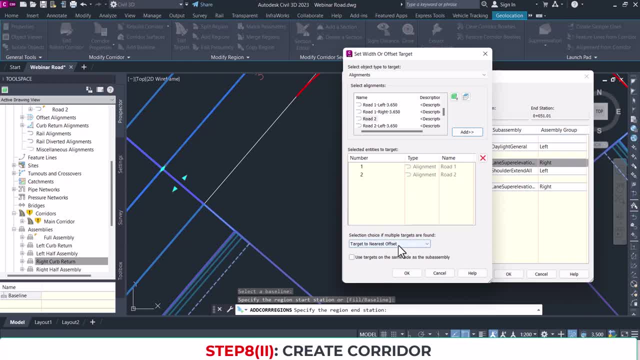 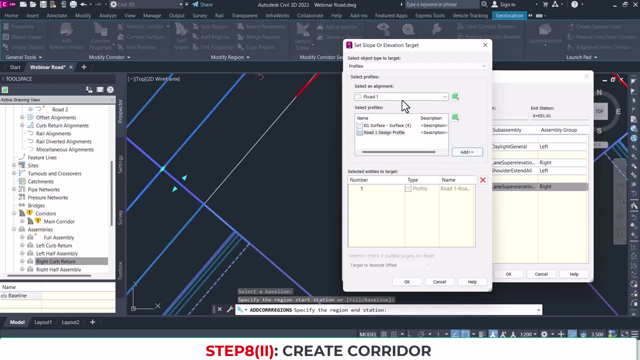 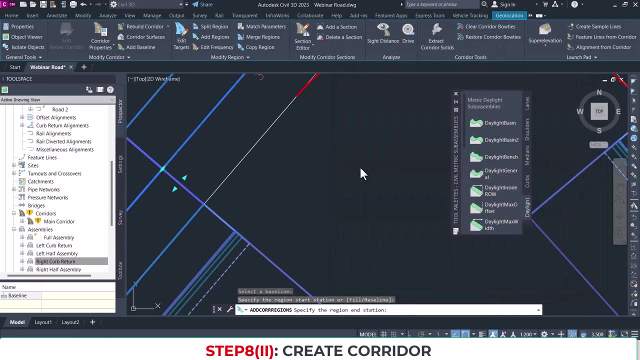 road one and then two. for my width targets- okay, and then for my elevation targets, i'm going to be using road one- the design profile- and then for two, i'll be also using the design profile, so i'll press ok and then press ok. so, as you can see, it is targeting fine for me as well. so because 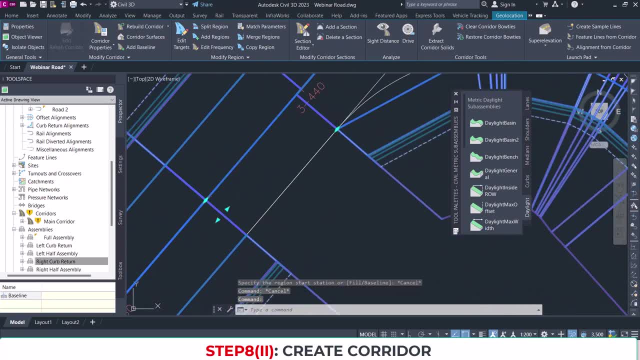 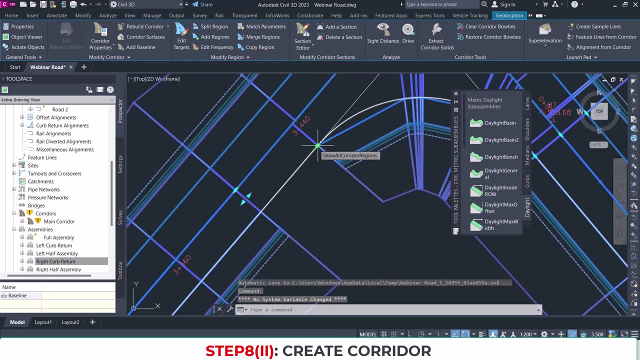 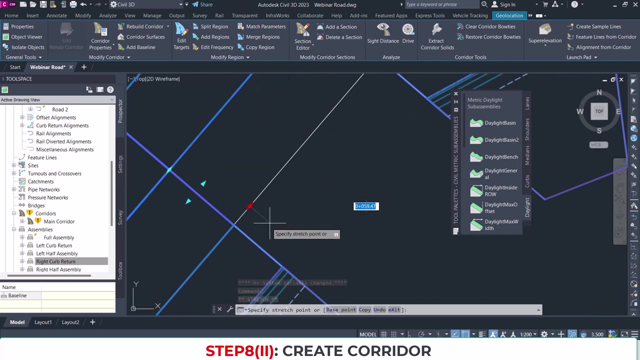 this thing, uh, so for some reasons, i do not target it well, so i'll just have to drag this to this: um, okay, what's happening? okay, it's not snapping for some reasons. okay, normally i'll just right click and then go to, let's say, endpoint. 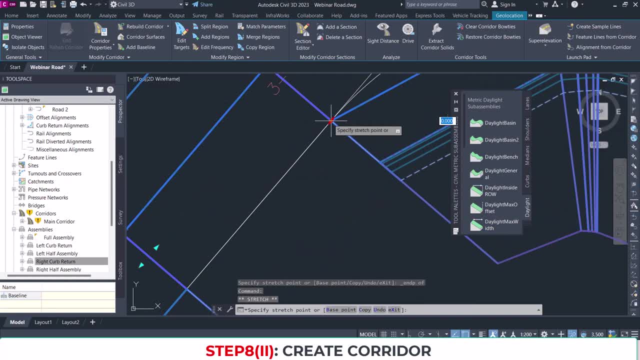 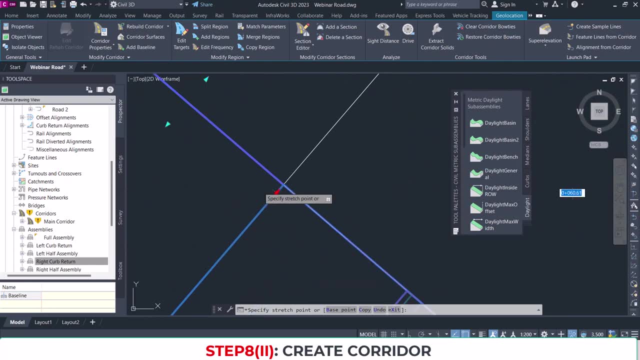 oh my god, but you understand what i'm trying to do, okay. it's just it's being slow for some reasons. you know that's what's able 3d. it requires a lot of your hard drive. even with my fast laptop i'm having issues. so let's go to endpoints. 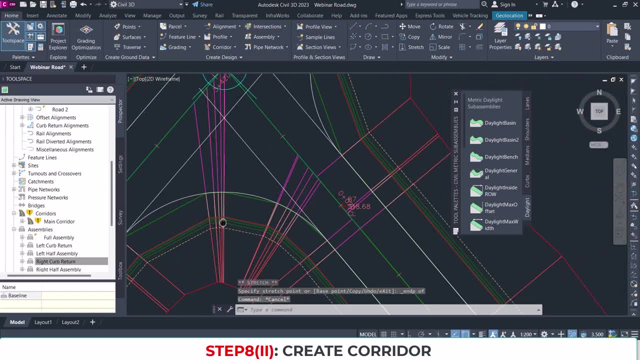 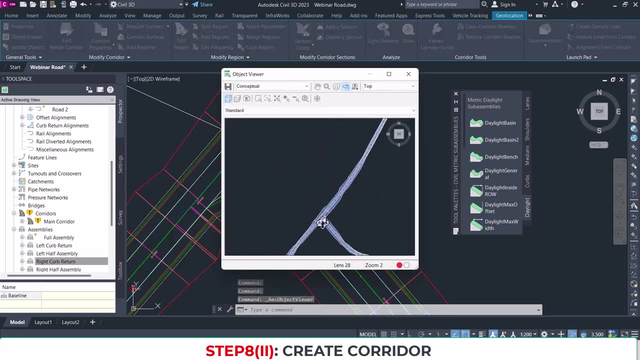 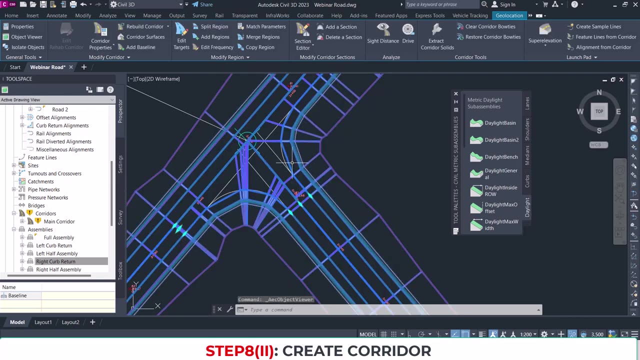 great, all right, so that is it. so you can see it has snapped. very well, let's now view it on the object viewer. object viewer: if you can see clearly, you will see that my road has come, i've intersected properly, so great. so this is what you. 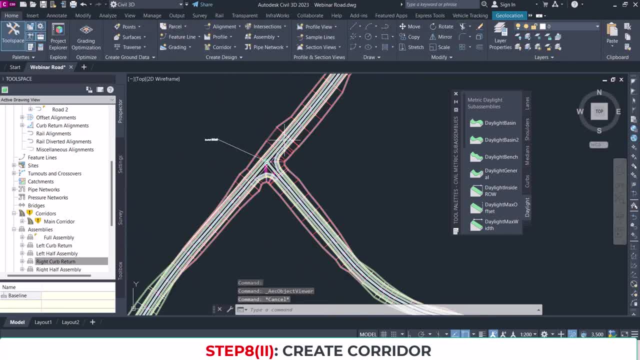 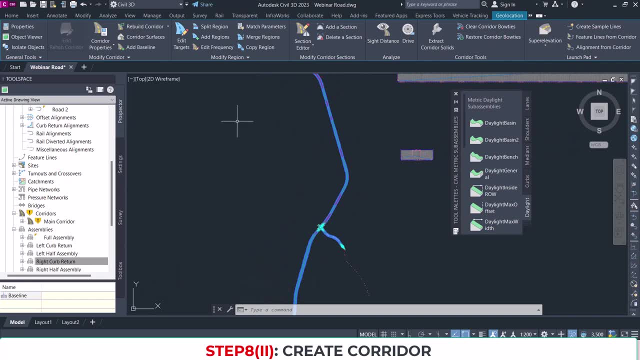 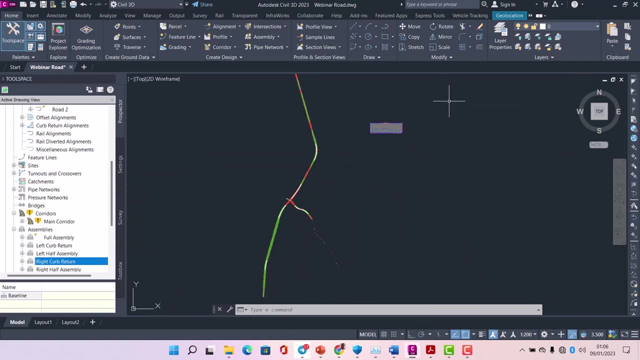 have. we have just done. we have created the intersection, so it's simply one corridor and then everything is it's all good. it's all good, so let's all right. so since we are done with that, we cannot close our two palettes. all right, so you can see everything. 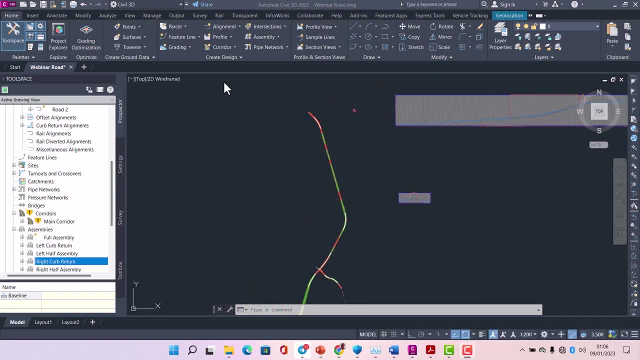 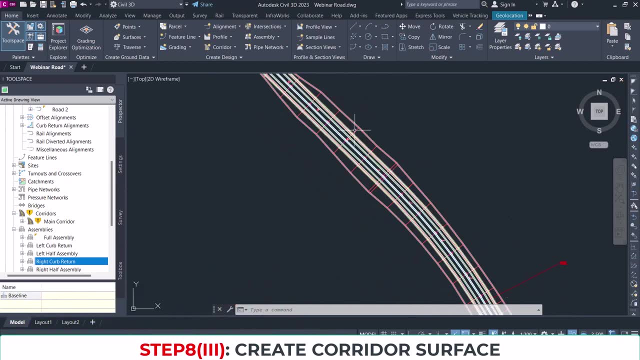 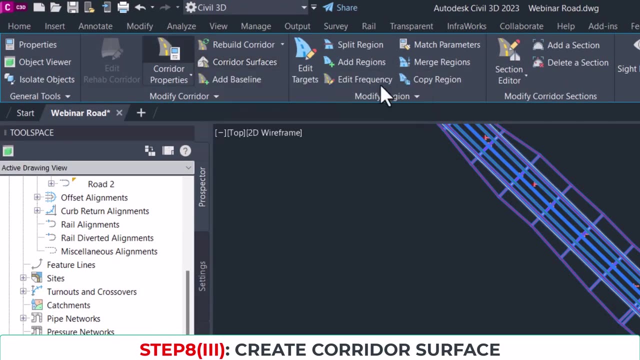 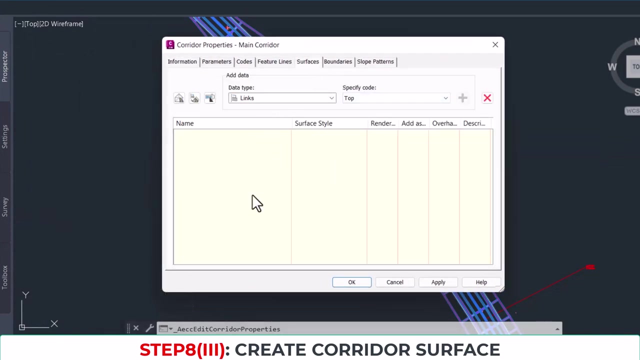 is smooth. the next thing on our design process is to create our corridor surface. okay, how to do that? you can just click. click on the corridor, okay, and then click on corridor surfaces, or just go to corridor properties- okay. under the properties, you go to surfaces and you will find this interface right here. as you can see, there is no surface of the corridor. 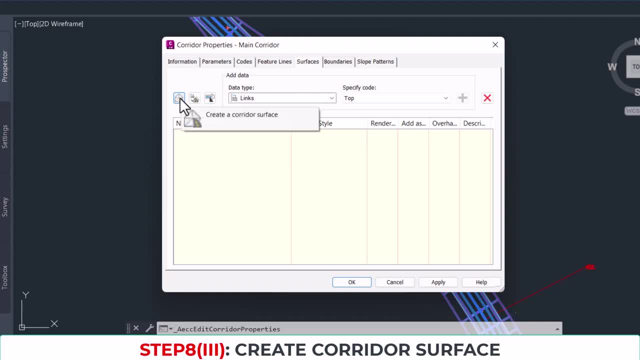 so you have to select a new surface, create corridor surface so you can call this datum surface. you call it datum surface because it is the base, it is the datum line. okay, that we are going to be using. okay, datum surface, all right. so, and then we have to add the links. we add links and we are going. 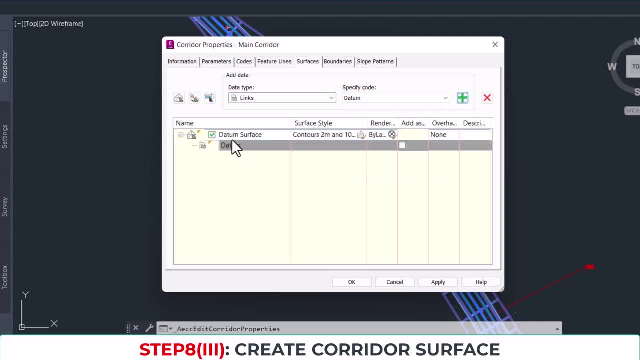 to use the datum link. we'll add the link right under the datum surface and then this under the overhang. okay, we are going to use the bottom links. all right, we are going to use the bottom links for the overhand carrier, so, and once we do that, we're not going to add a break line. okay, so that is fine. 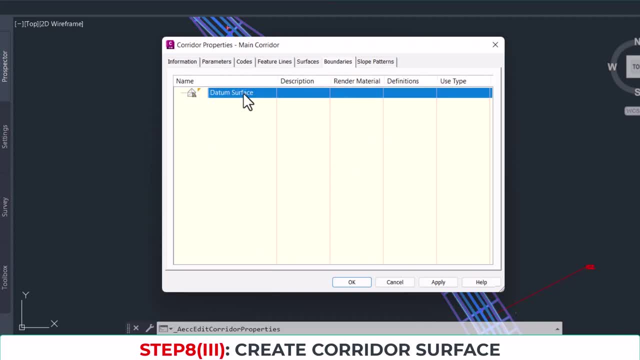 now, but we need to set a boundary for our datum surface. okay, so we have to create. use the corridor extents as boundary, which is the you know the daylight. okay, so we can use the corridor extents. all right, so that's great, so we just apply. it will ask us to review our corridor. 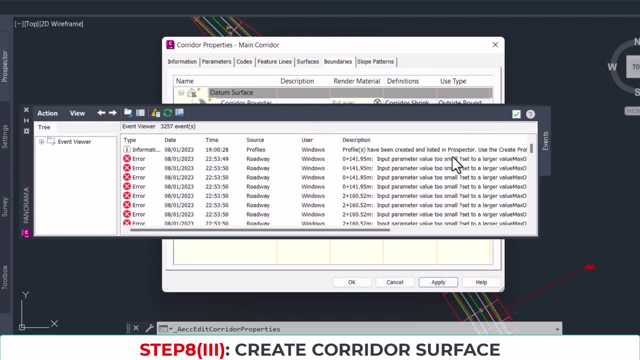 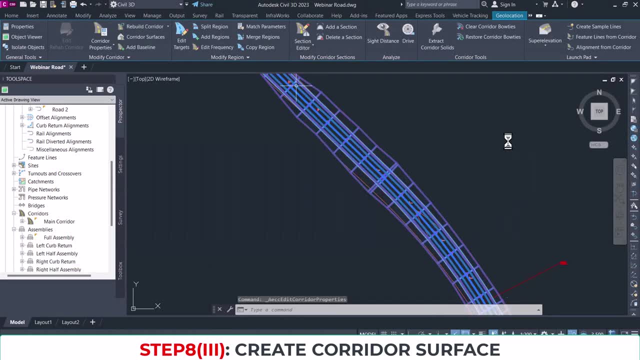 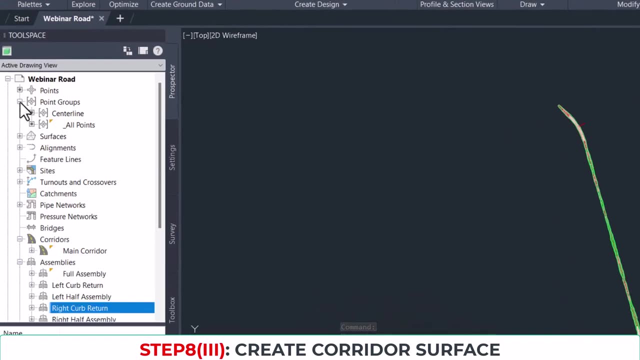 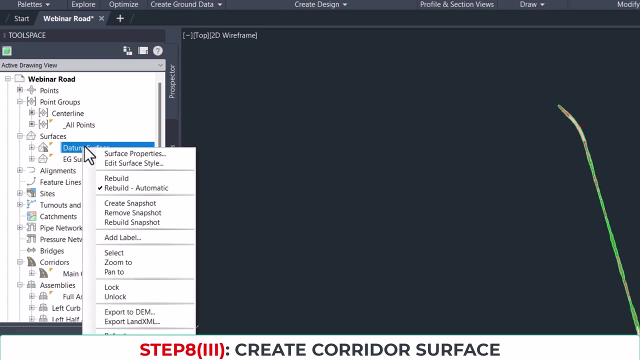 okay, and once we do that, don't mind all this. all right, so we close this and then check this. now we have created a surface, one corridor. when you go, let me you know, minimize all this, go to surfaces, okay, you will see that we have this datum surface created right here. so if you want to visualize this surface, you can just 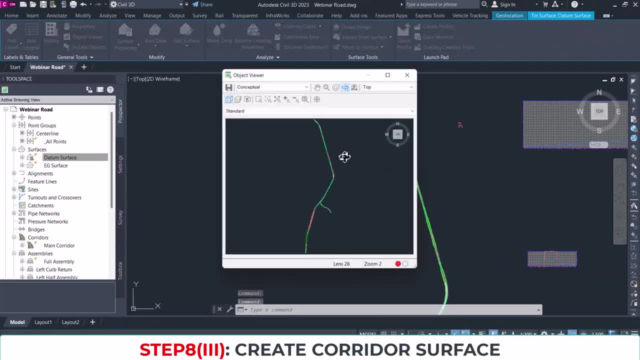 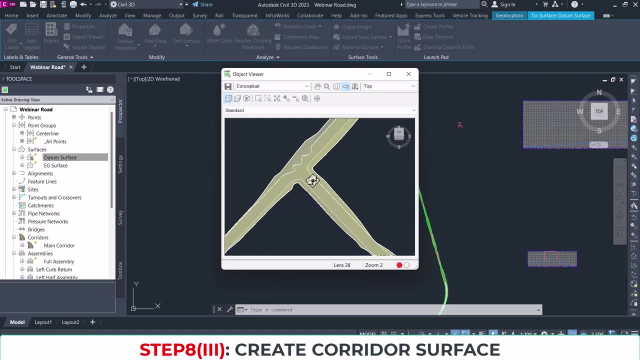 select it okay, and then go to object viewer. so you can see we have extracted the surface out of our uh corridor. so this is not our existing glass surface. this is our corridor surface right now. it's taking everything up to the. you can see there is a very smooth line showing our 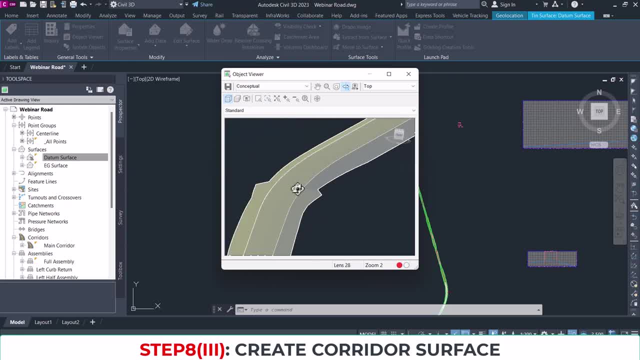 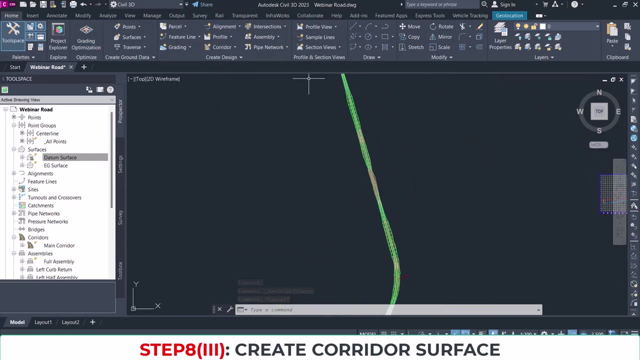 where our purpose would be, but the remaining by the side is the daylight, so showing the fields and also the cuts. okay, you know, in fact, let us drive through our road right now. that's right. i think it's about time for us to see, to drive on our road. let's just do that by you. 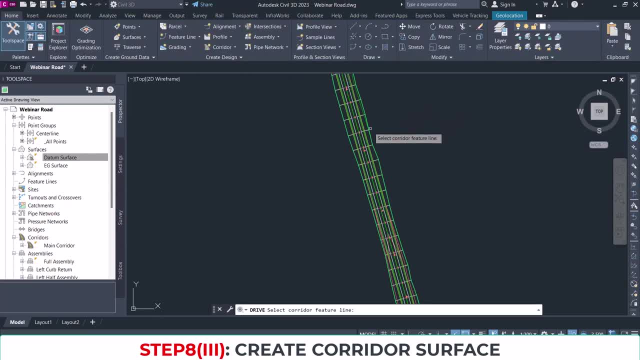 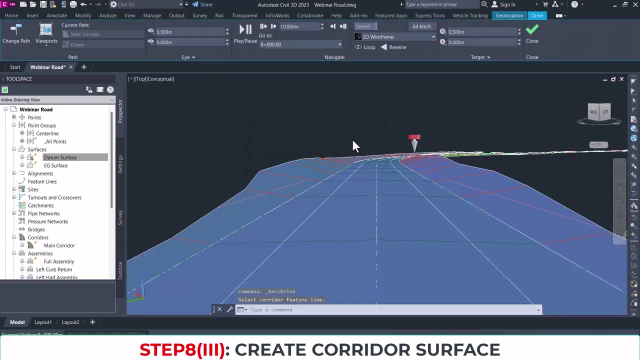 know, selecting the corridor and then click on drive. okay, i don't, i want to use drive from the at the crown. so once i do that, can you see? can you see how beautiful this is, how beautiful this is. let me drive it at, uh, yeah, okay, at the speed of 100 kilometer per hour, because that is the speed. 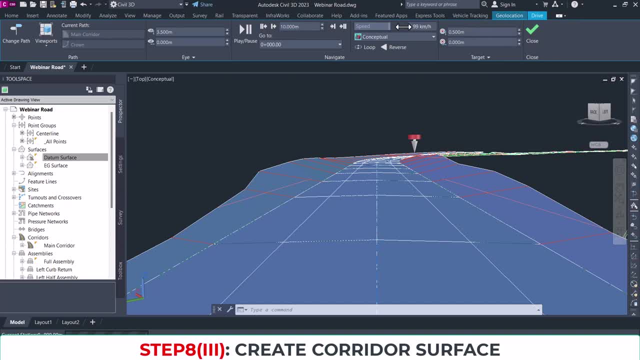 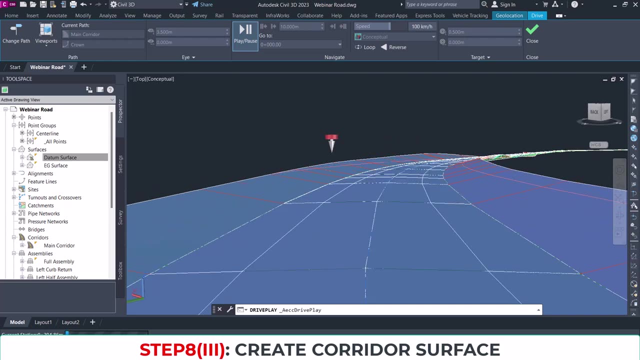 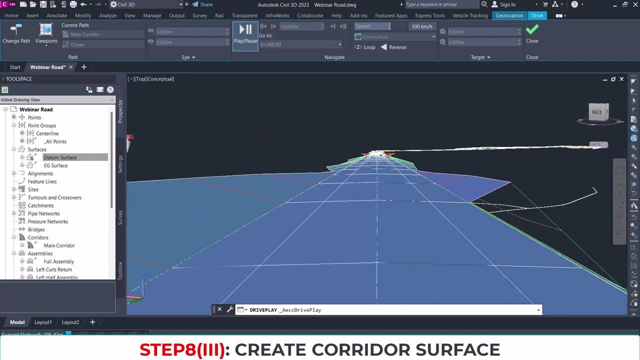 of the road. okay, okay, let me select. okay, i can just type that manual here. okay, so, let me just play right. can you see? can you see my roof? how beautiful is that? oh, my god, this is a beautiful road. i love it. so that's what civil treaty can do. so, as you can see, these are cut areas. now you come. 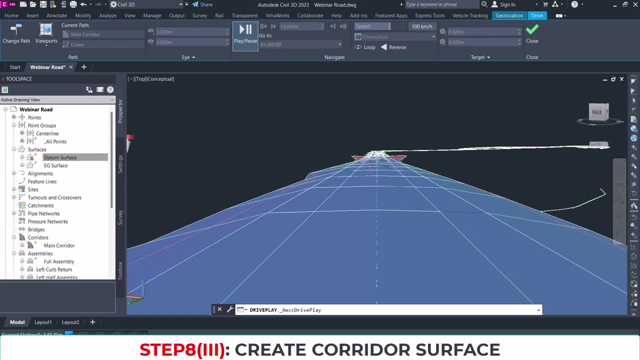 to the area of the field. so you say you can see our proposed roadway, all right, the carriage, and then the shoulder showing, and then the daylight. the daylight is showing you the cut and feel by the left and right. right, so i can do that, but let me just close, okay, and then 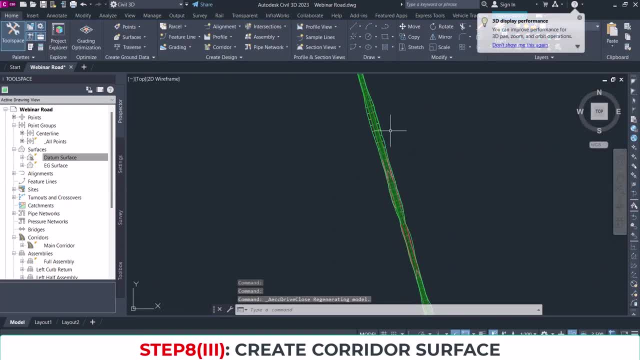 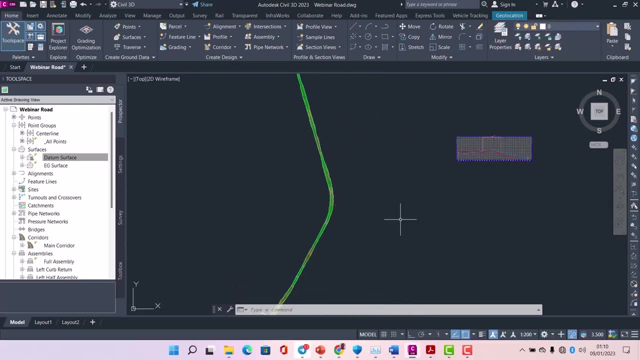 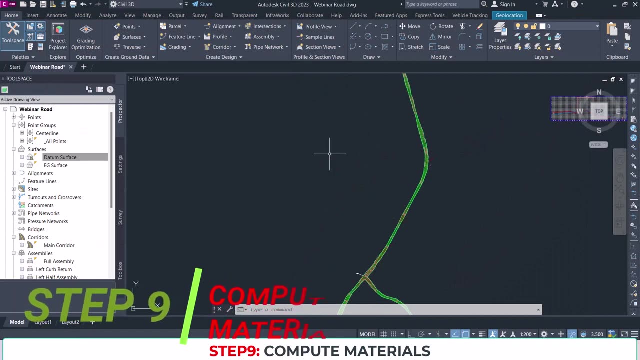 close this view, all right. so, uh, we have created our corridor surface. that was the next thing, and then we have just done that. so the next thing on our list on our procedure is to compute materials. so let's go ahead and do that now. before you compute materials, you go to settings. 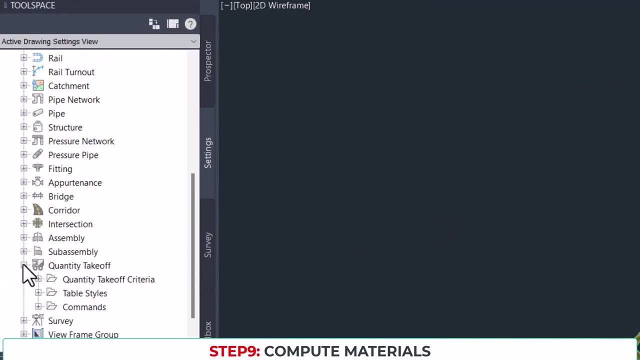 um, and then you go to quantity: take off materials, you continue, take off criteria, so you expand it and you you will find cut and fill. there are material, you know criteria that are available for you to use. okay, but usually i like creating mine. okay, i'll just right click on this and then click new. so 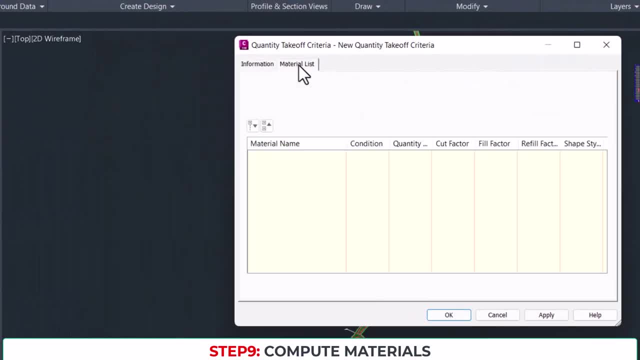 let's create a new criteria. now we are going to use um. okay, we're going to add a new material here. okay, let's call it on the information tab. let's call it um at work, cut and fill. okay. then let's go to material. let's add a new material we've got, we'll add a cut. 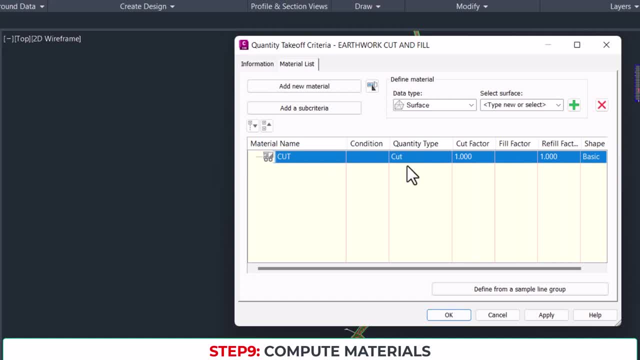 material and what is the quantity type is cut. okay, so under that we are going to be adding a surface. okay, we are going to be adding number one, the eg surface, and then we are going to add, secondly, the datum surface. okay, now, what is cut material? okay, cut material is everything that is below our eg surface, if you. 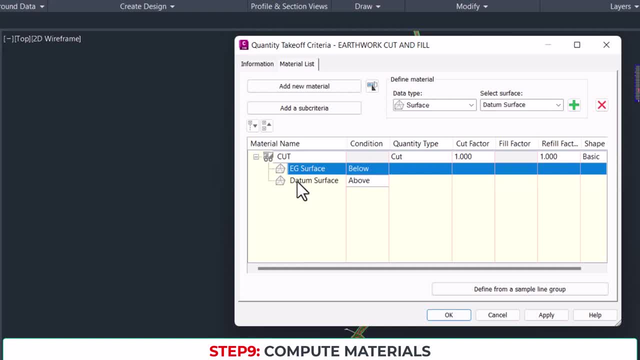 are going below a dream. so we're going to set below a g surface and if it is above our datum surface it's a cut material. so below, above, not that okay. so we're going to add a new material and that criteria is going to be called fill material. so and make sure that the quantity type 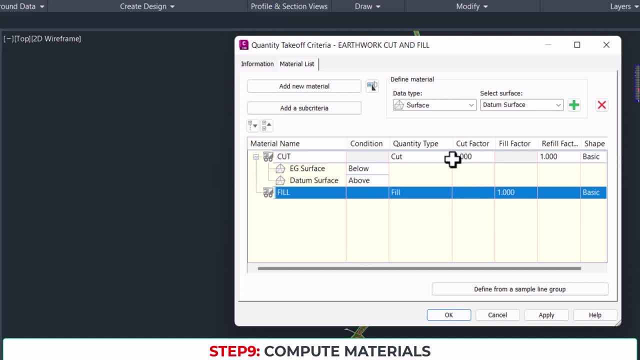 is called field. okay, so these are, uh, back to this cut. we have the cut factor. so if you want to use, you know accounts for you know when you, when you know, when you, when you are filling the material, right, we have a field factor and and cut factor. so, uh, it's gonna be less if you have the material. 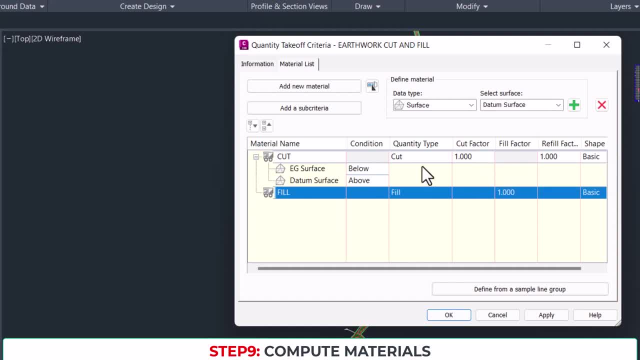 because when you compact the material, the volume reduces and things like that. but let's just keep it like this for now. okay, so still under this field, we are going to add the eg and the datum surface eg. so what we simply do is to you know, is to just um. 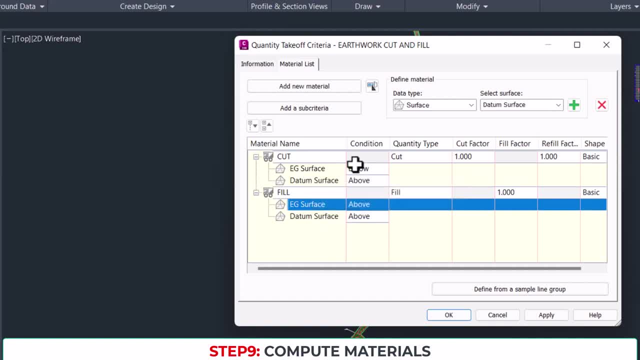 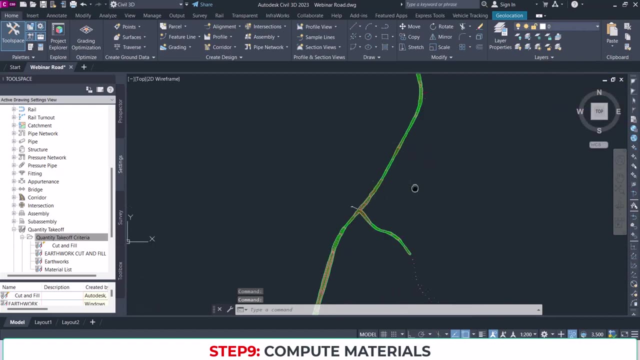 okay, we are going to just reverse this. since this one is below, this one is going to be above and then this will be below. so what are we going to do? we want to just apply, okay, all right, so then, when? when we have done this- okay, we have just complete, we have just created a criteria. 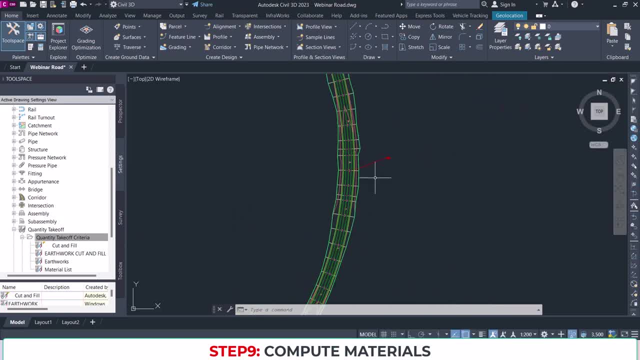 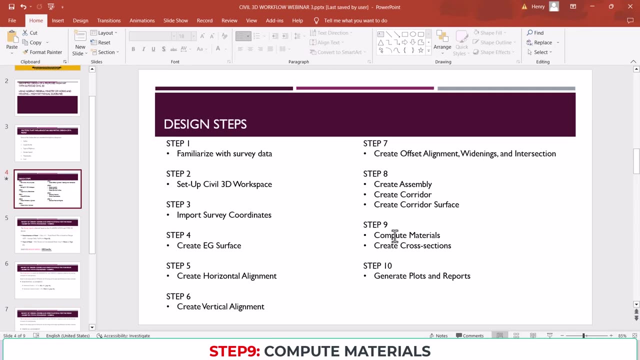 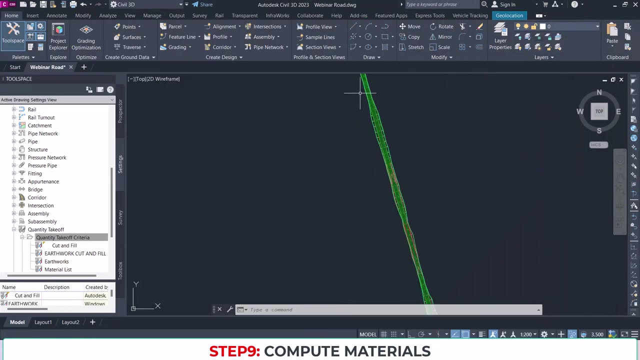 now, sorry, there is one thing that you have to do before computing the material properly. okay, you have to create sample lines. okay, and then create your sections. okay, that was supposed to come before in the procedure, you know, after step nine. that's why it's all in step nine. so you do them together. okay, but let's create cross section. that was the. 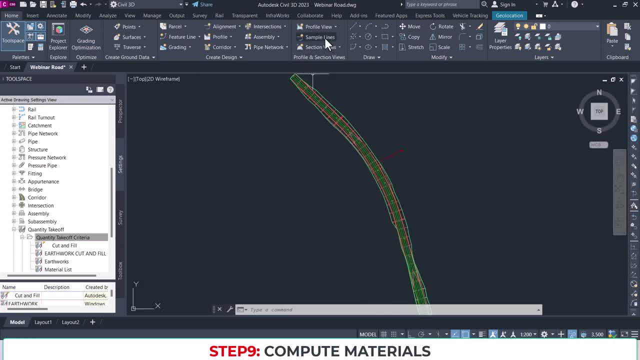 first thing we're supposed to do. all right, so let's create add sample lines. you just go to under the home tab in this site. you find the sample lines. you click on the sample lines and then select an alignment. we want to sample on the road one, so let's just press. 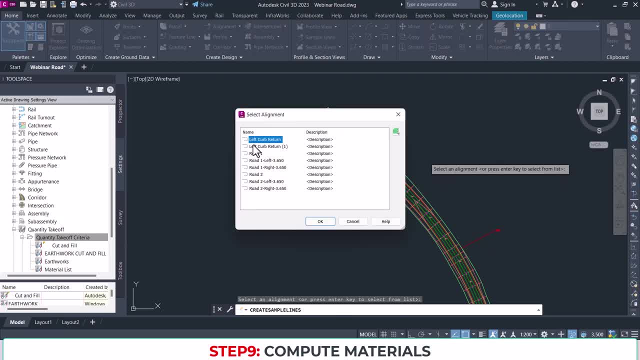 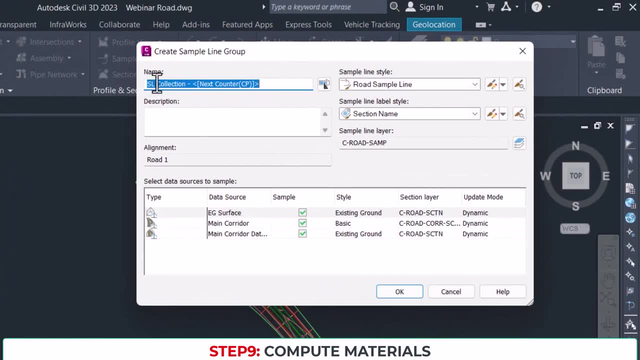 just press enter, okay, then we select an alignment from this middle. okay, we select, okay, good one, and then let's give it a name. you can just use the default meaning style, and then we are going to allow everything here open. so let's just sample all this data we want to. 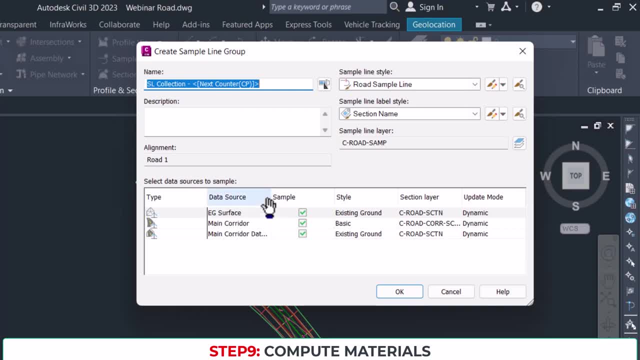 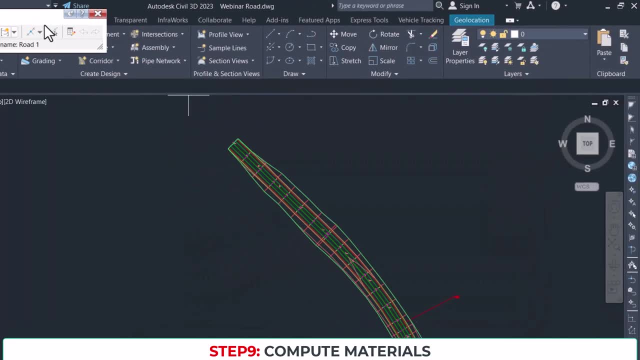 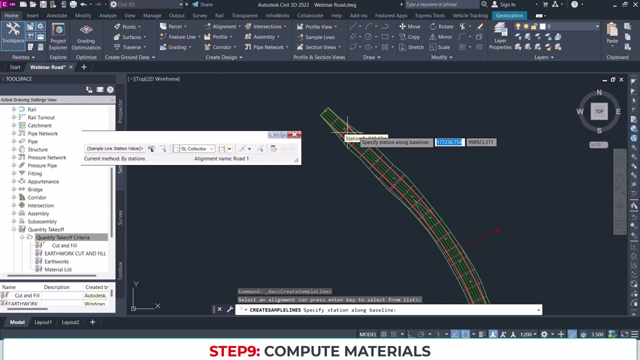 sample everything not to support the eg surface, the main corridor and the main corridor, that on surface. so i'm sampling everything, so let's press. ok, so we are going to be sampling by a range of stations. okay, and remember my changes was at um 20 meters intervals, right, okay, so we are going to be sampling with 20 meters in terms of so. 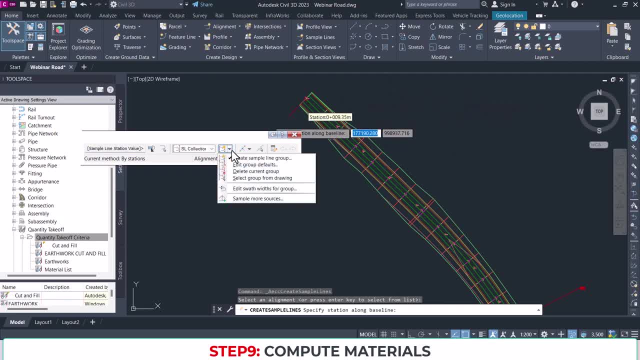 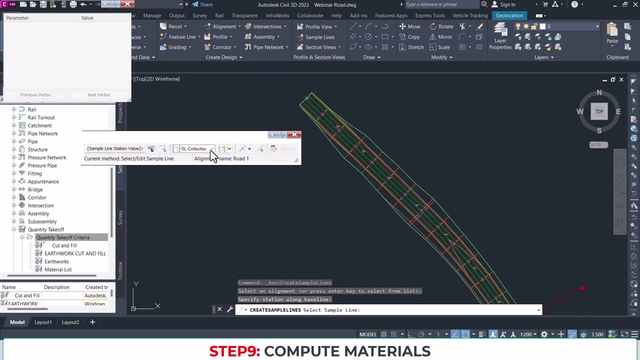 let's check. we are going to select that from here. okay, we are going to. um, sorry, we are going to be sampling. all right, pardon me, let's okay, all right, so, okay, sorry here. all right, so let's check. uh, by a range of station. okay, all right. so when we choose this range of 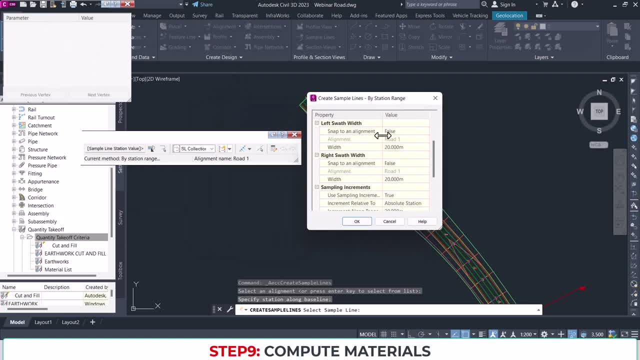 station. we are going to select the intervals. so, as you can see, we have um the okay, the station range. we want to start from the- uh- beginning of the alignment, which i will leave that as true. i want to go up to the end of the alignment, okay, so the left swap width, that is how long? from the? 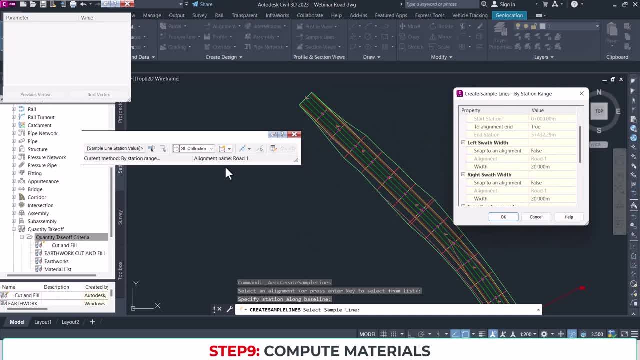 center line. is it going to go to the left? we are going to sample to the left, so already you know, our width to the left is one lane is 3.65, and then they will show that it's 2.75, so making a total of 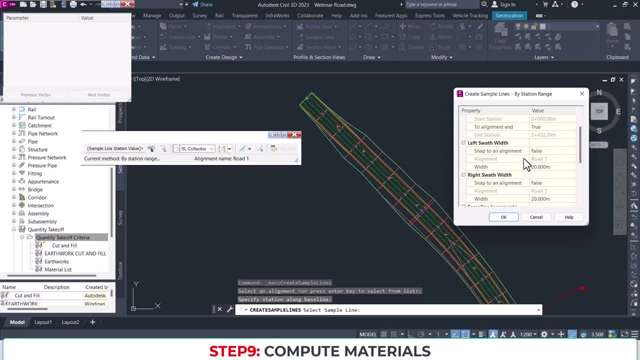 about: um, you know, six meters there about. so, let's say everything, want to sample like 20. uh, 15 meters to the left. okay, i could have just left it at 20, but i can show you that you can actually adjust it. make sure that it's beyond your corridor. 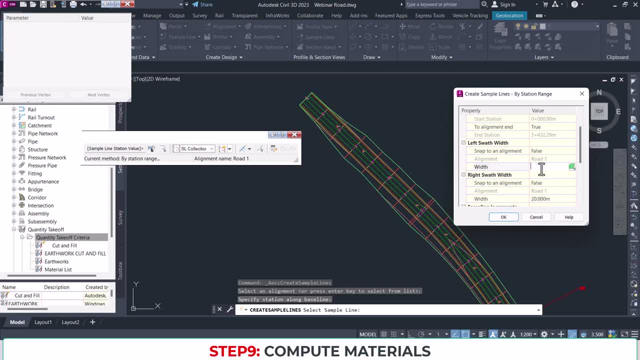 or, uh, you know width for one, one lane. okay, so let's say 15 meters. okay, then you go to the width and to the right swap width and also put 15 meters, if you wish. okay, then the increment. all right, our long tangent is 20, a long course is 20, along square is 20. great, okay, so, yep, so, and then we can. 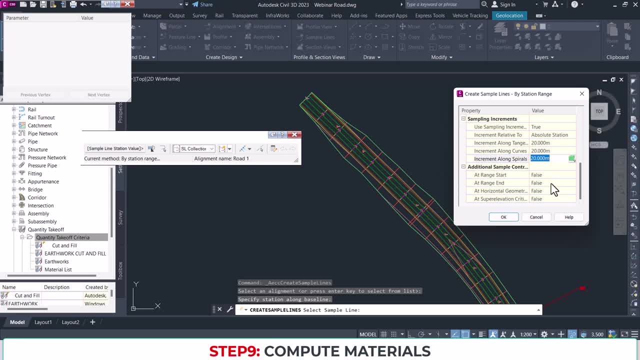 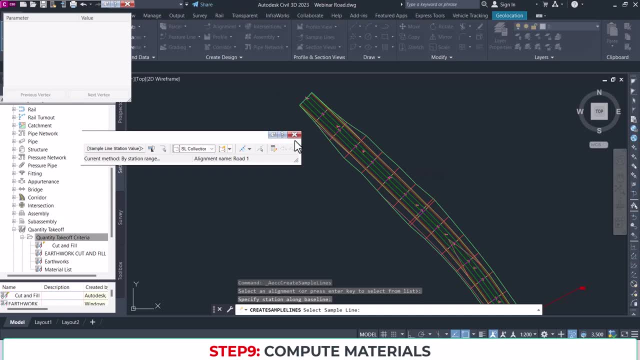 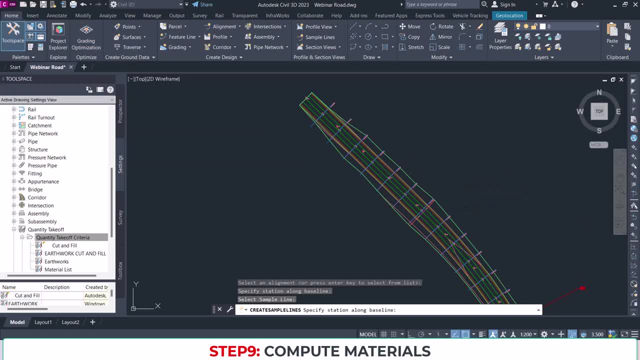 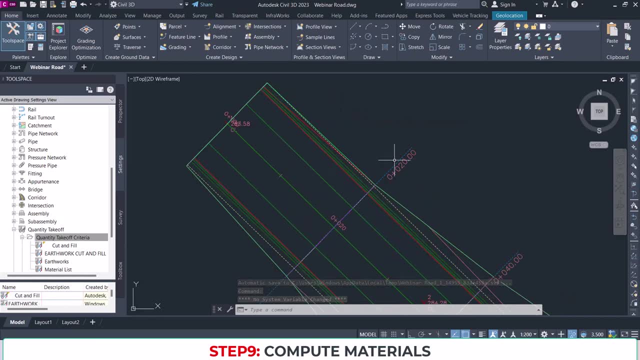 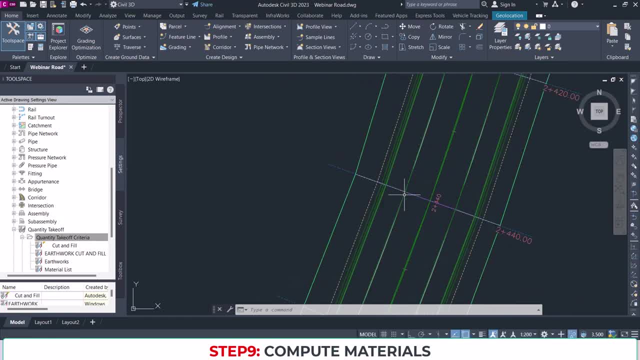 width, and then we can also see that we have sample width, and then we can also see that we have sample- uh, all our sections at 20- 20 meters intervals, uh, all our sections at 20- 20 meters intervals. now, what can we do with that? we can create section from that. 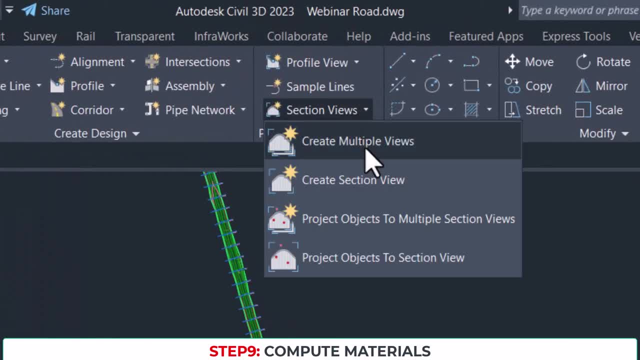 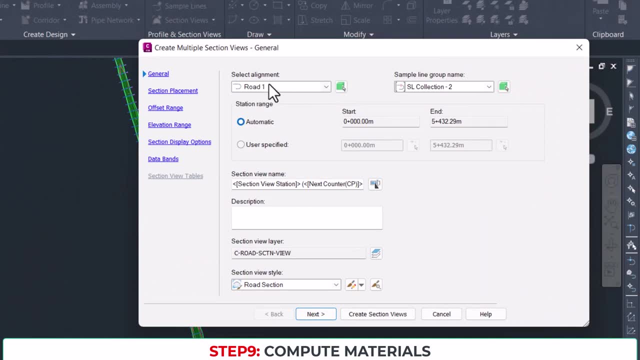 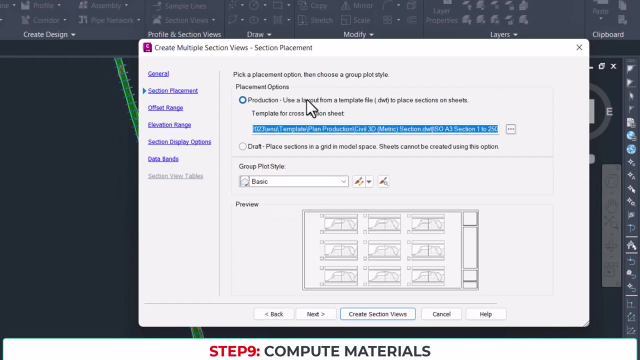 so if you go to your section view, you go to create multiple views. okay, once you create your multiple views, you open it. now you see for which alignment you select for root one and then you select, uh, the alignment collection. okay, so you this um section placement. now we are going to use production. okay, if you want to use production, you. 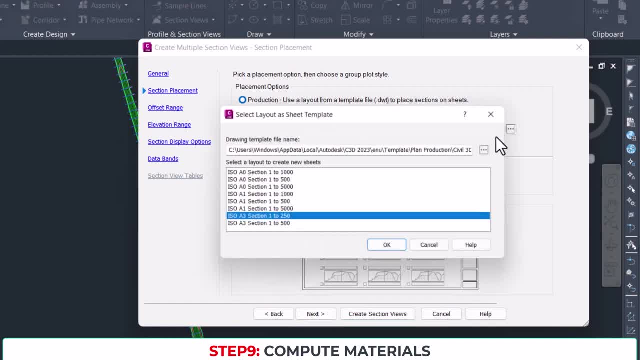 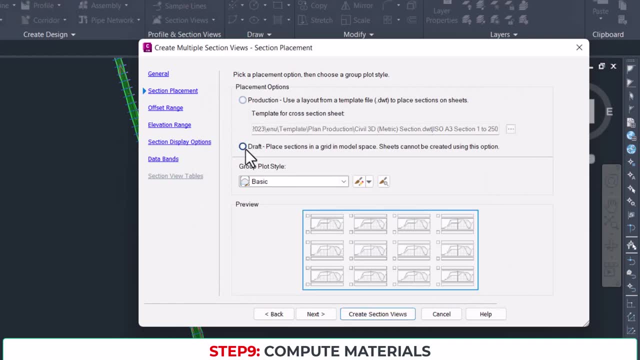 have to select a sheet. okay, you are going to select it in a sheet, but we are not going to use the shape now because i don't want to go into all the intricacies that are involved in that. let me just put it as draft. okay, just paste it and draft. now let's go to offset. okay, okay, let me just for. 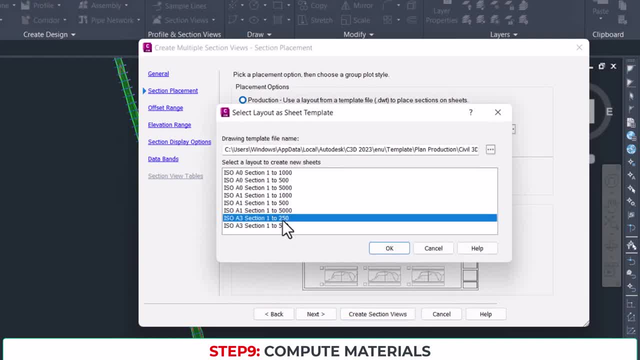 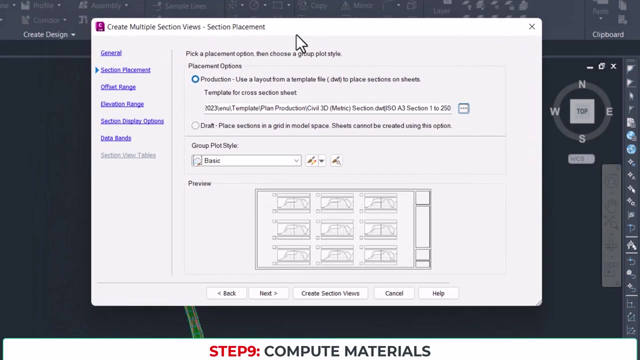 a second. put this production. okay, we can select a sheet. okay, a0, a1, a3. you will find a3. okay, i can just tell you beforehand, i have to create it myself. so, um, okay, let me use uh, a3. now, if i must use a3. okay, there is something that i should have made, an adjustment i should have made, i have. 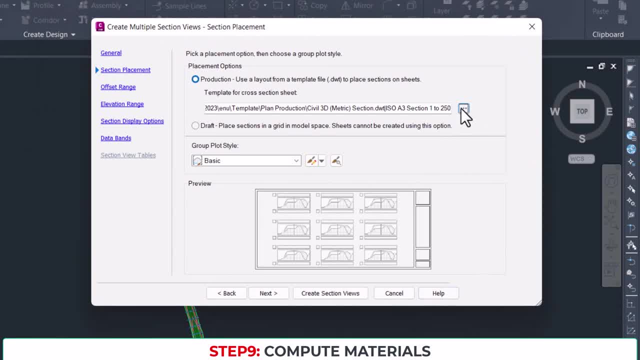 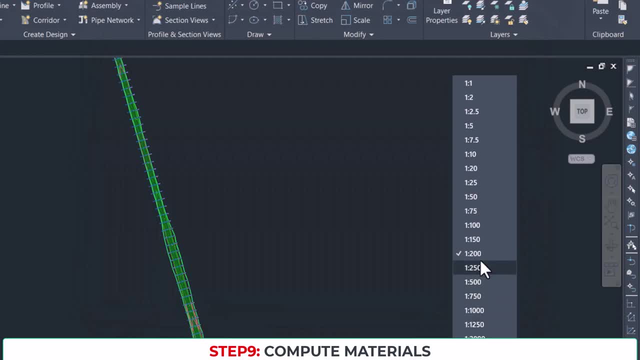 to make sure that my scale is the same with what we have here. so you see that a3 is 1 is to 250 here. so let me close this back. i must make sure that i have 1 is to 250 selected, but because you don't have this a3 sheet, i'm not going to use it, okay, please. 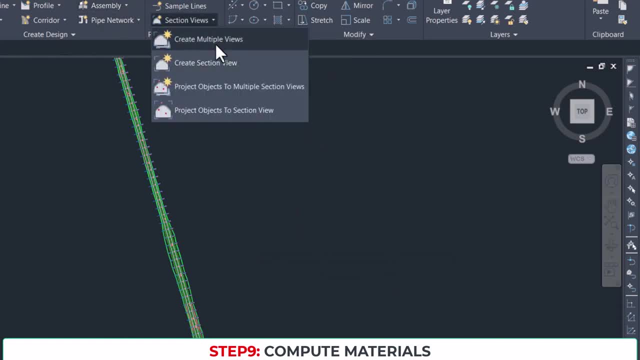 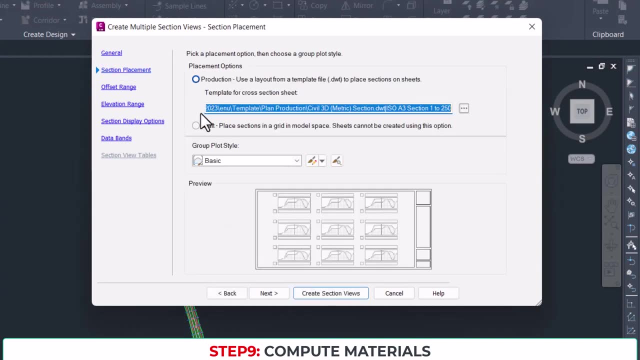 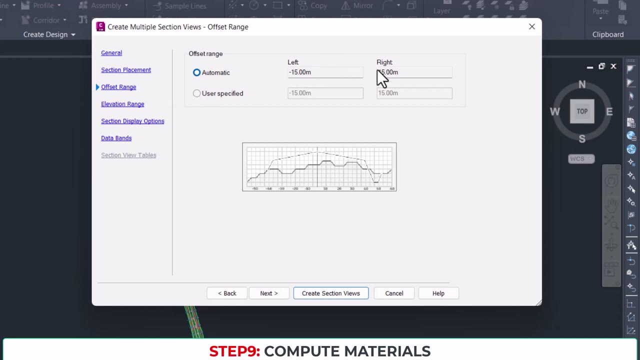 pardon me, i'm not going to use it, so let me go to the section views. create section view. let's just use um, the normal uh draft. okay, because you don't need to select the sheet in this one. go to offset range. leave it as uh. okay, this shows this. the sample line extends the 15- 15 we chose. 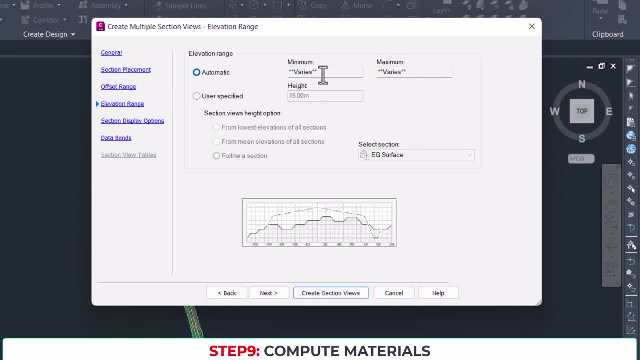 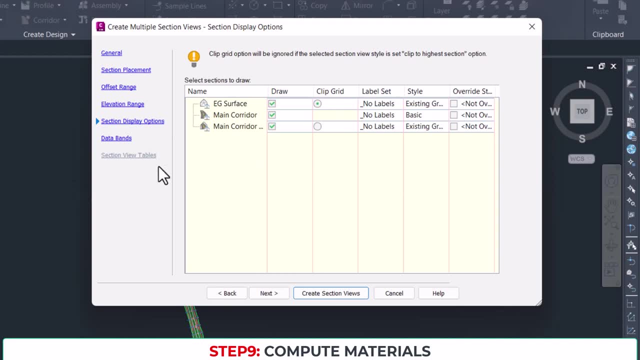 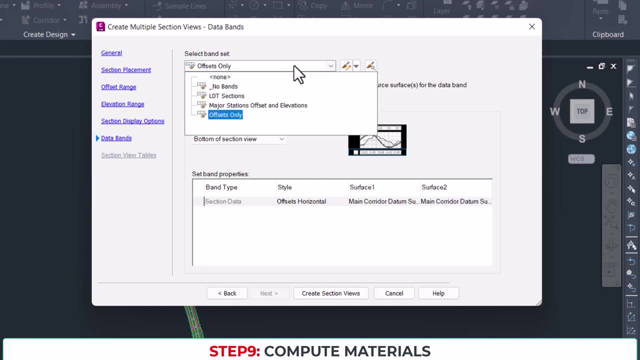 both and the swat we now. let's go to elevation. okay, let's leave it automatic. okay, then what are we sampling? we are going to view all these ones. yes, we want that. so let's the data bands. now, if you want some data, because we have calculated our cuts and fields, we can add some data bands to it. 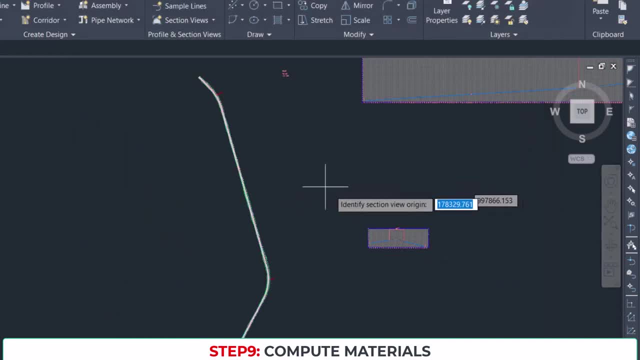 now. so let's just create section view. now you have to select a place where it will not interfere with your original drawings. okay, so let's find somewhere here and put in our section sheet. okay, so watch for it to come out. great. so we have these sections, as you can see. 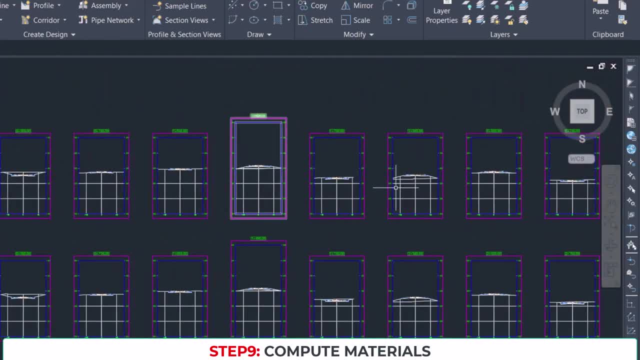 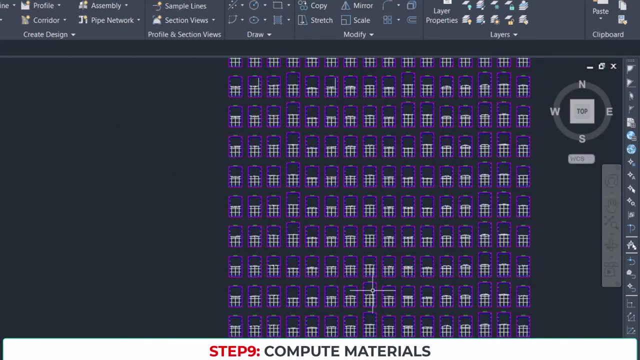 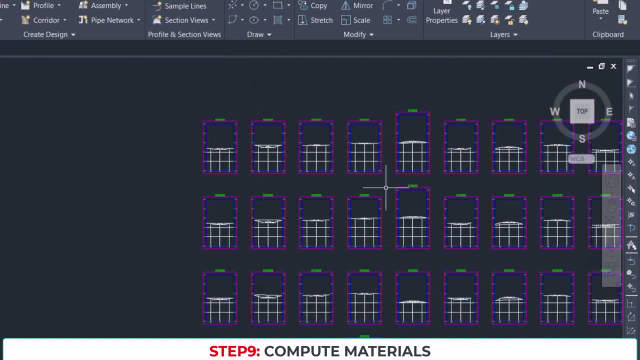 this is how our section is looking like. okay now, this is not a very great view because we are just using draft. that's why everything just comes in without title block. you know extent when you're using that production. it will bring up a title block and just use. maybe it will group like six. 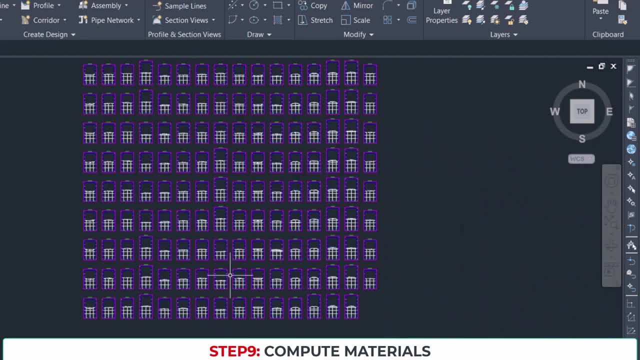 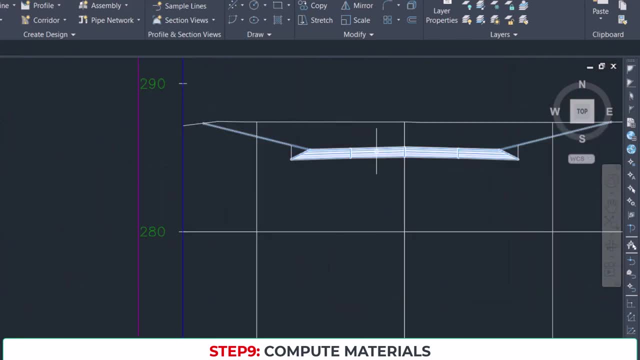 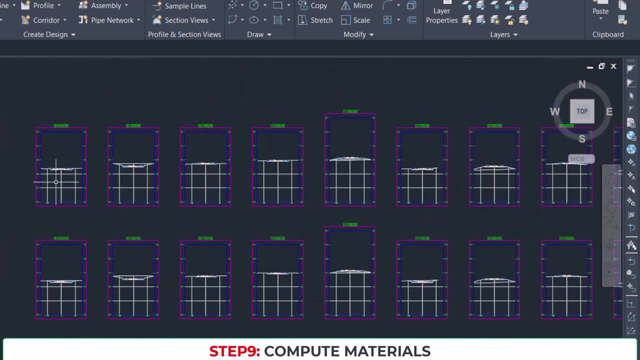 of them into one sheet. yeah, so, because you can see we have plenty. so if you keep viewing them, all of them one after the other, you would see he's showing you the cut, showing you the field. okay, for each one of them you can adjust all these views. if it's not looking fine for you, you can click on it. 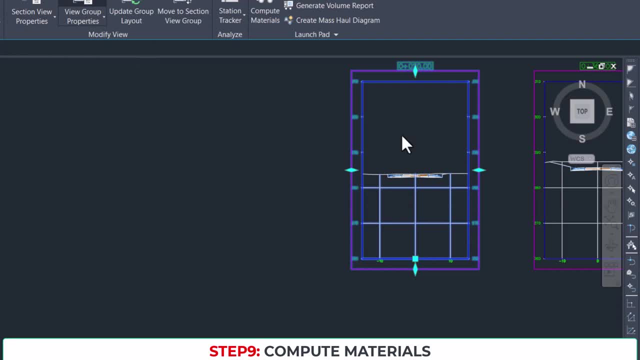 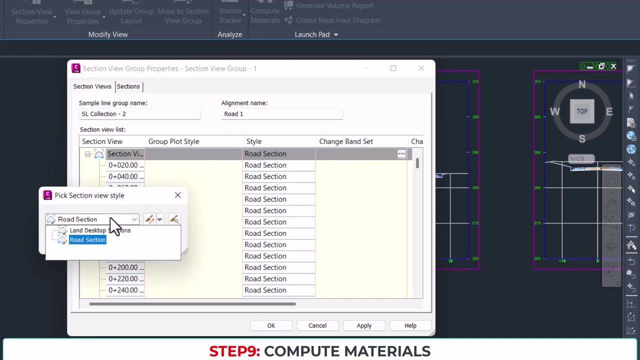 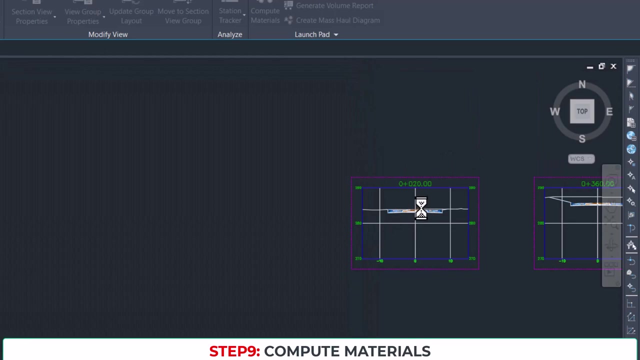 on one of them and then go to view group properties. okay, okay, you can select, you know. for instance, if you want to change the style, let's say to land desktop. okay, let's see to another view. okay, if you do that and then apply. okay, you can see. 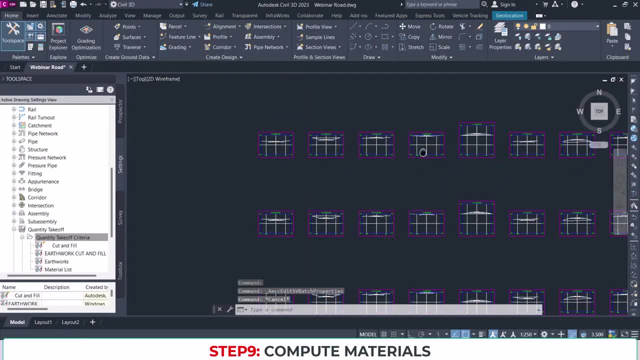 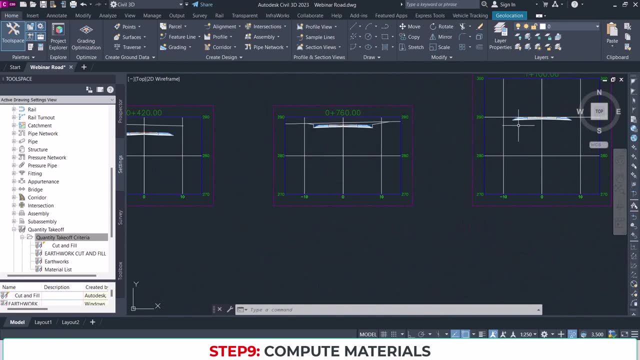 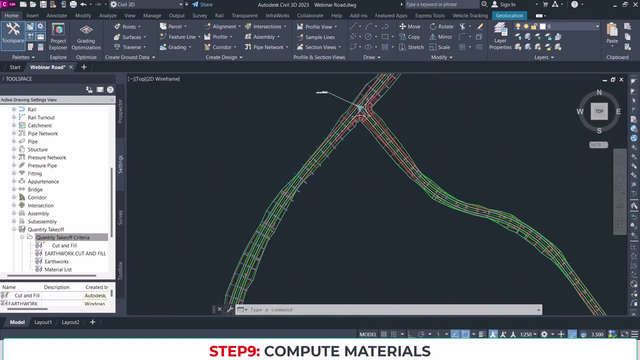 this another view style. this one is looking more compacted and you know better. all right, so you can always adjust how this thing looks like by just creating the view that you. that works. all right, so that is it. we also do the same thing for the two, okay, that is, by creating sample lines. 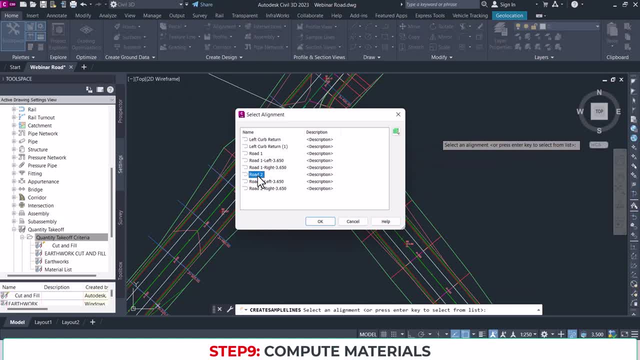 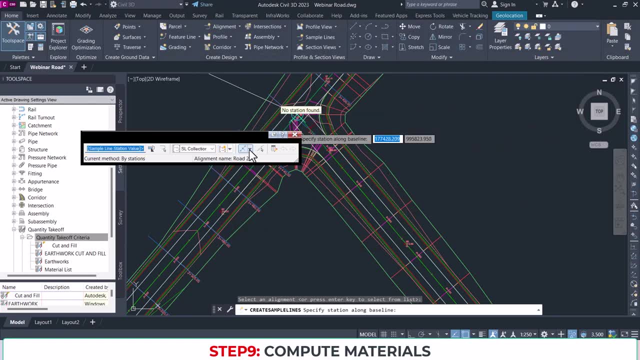 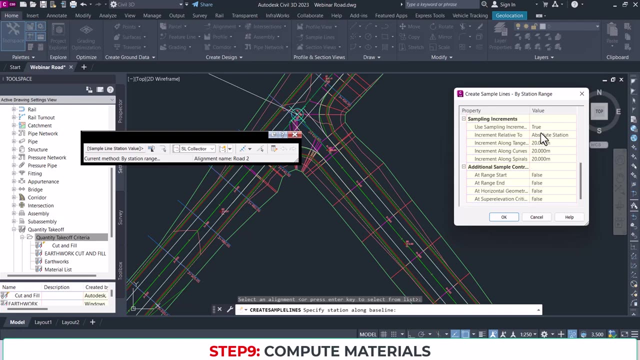 we go to sample lines and just press enter and go to and click on the two, press okay. so still press okay. everything is by default. now go to by range of stations again, then everything. i think we see three again. it's merciful to bring the previous settings. so, uh, you know, remember we. 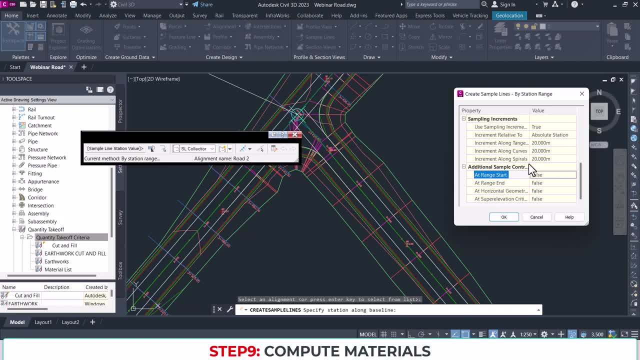 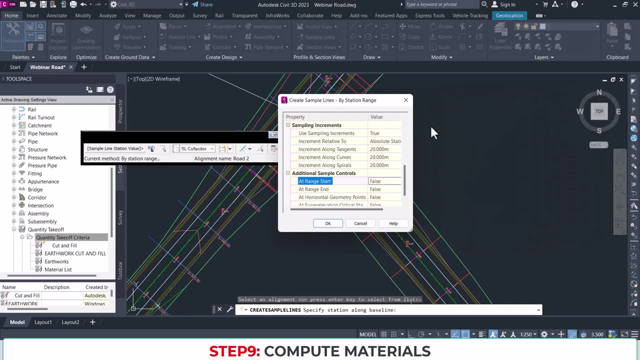 did not put at the beginning of station. okay, all right, we in the previous one, but we needed it. that's why, if you notice in the cross section in the sample view, you will see channel zero, zero. or in this case, let me put true here- okay, to start at the beginning of the station. okay, and also at the end of the station, okay. 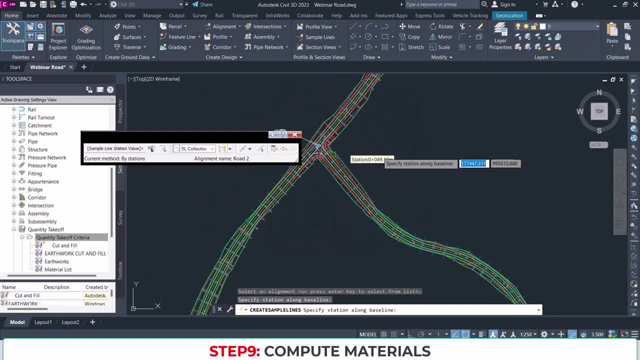 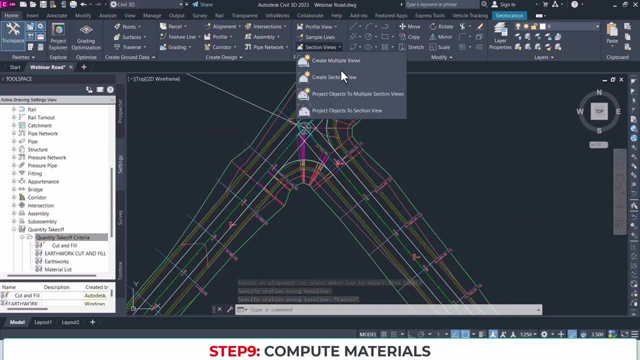 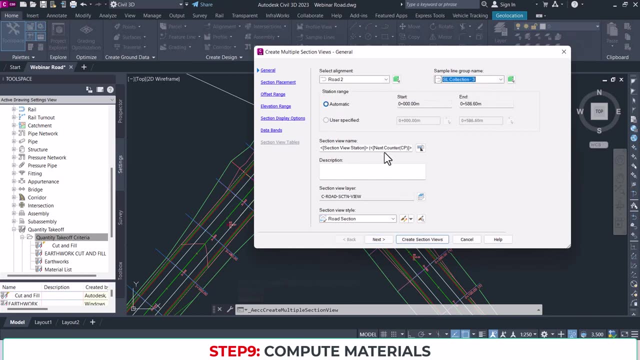 i press okay, all right. so, if you can see, it has also created sample lines for that. so we now go to create the section view, create multiple views for it as well. so we are going to use the two this time and then sample collection three. uh, that's the name automatically for the sample associated. 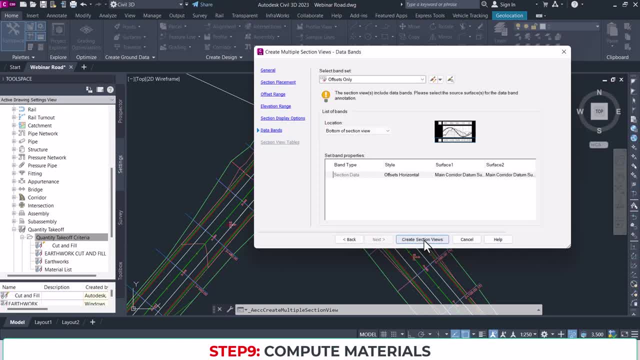 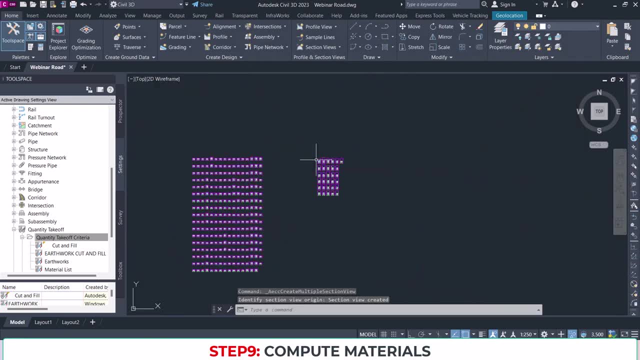 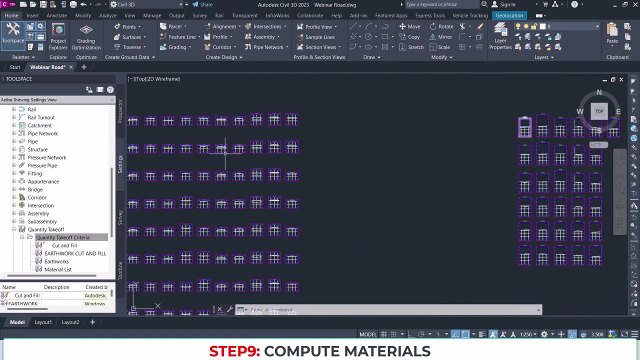 so every other thing, i think i'm gonna leave it by default. so let me create the section view again, i find, maybe to the right hand side of this, and place this okay, so again i can choose how this change. as you can see, this one is spawning all the way. that's because it is at our intersection. 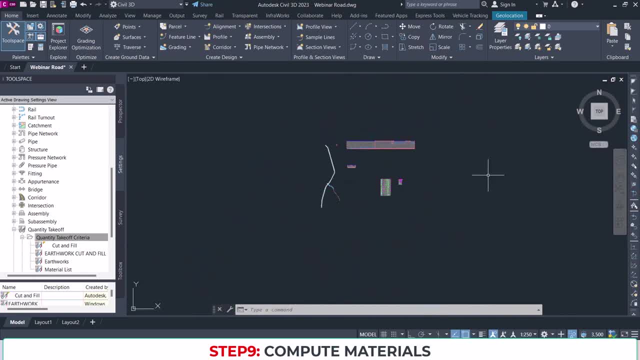 okay, that sample line is somewhere here. so that's why you see, the view was, uh, it's not showing you and things like that. so you can monitor to see if there's anything that is not showing well in this section. so that is it, that is it. that is it. so we have created a section then we can. 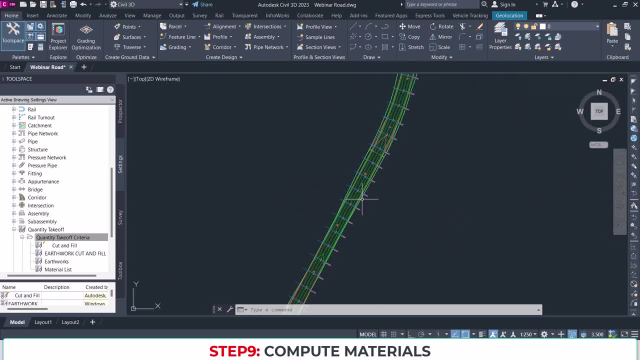 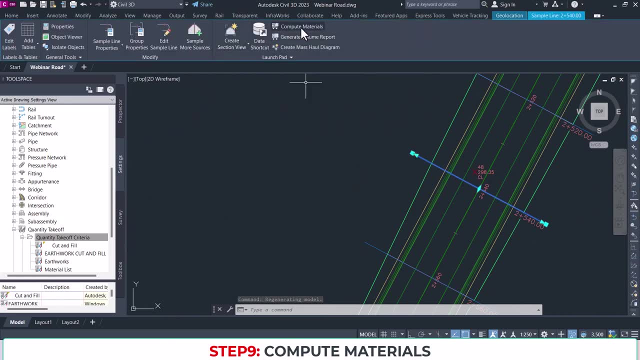 proceed to computing our materials. so how do you contribute your materials? just click any of the sample lines, okay, and then go to compute materials. okay, now we are computing material for wood one and then we are using the sample collection line. collection of this. so press ok and then, once you 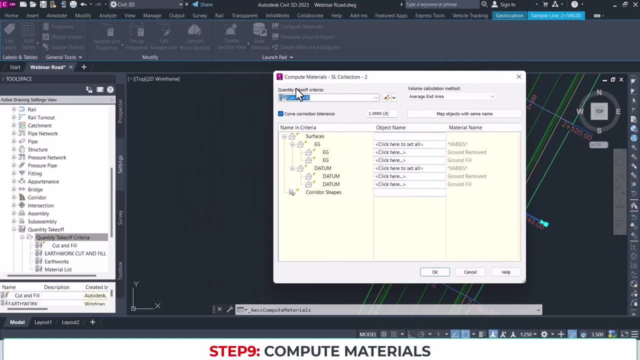 do that now because we have to. we created a quantity takeoff criteria. we find that criteria effort, cut and fill and once you find that you just use map objects with the same name, so it will map eg surface to eg surface. it will map that on surface to my main corridor. 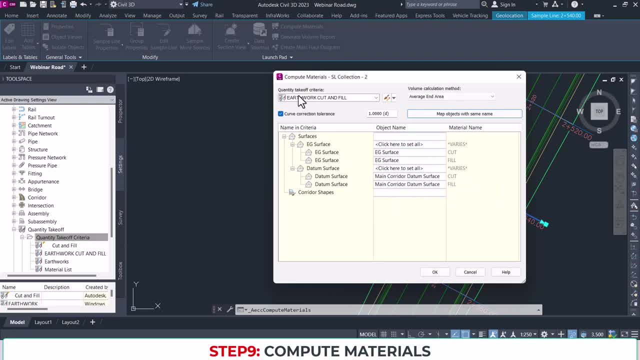 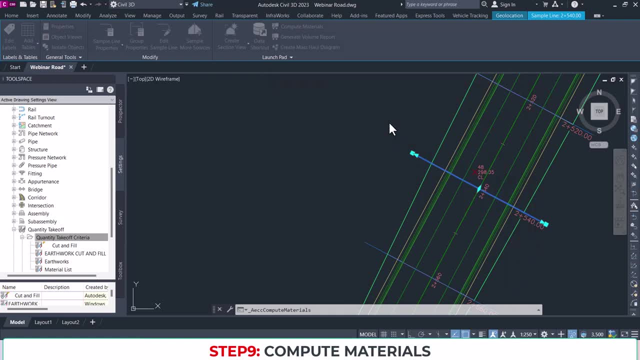 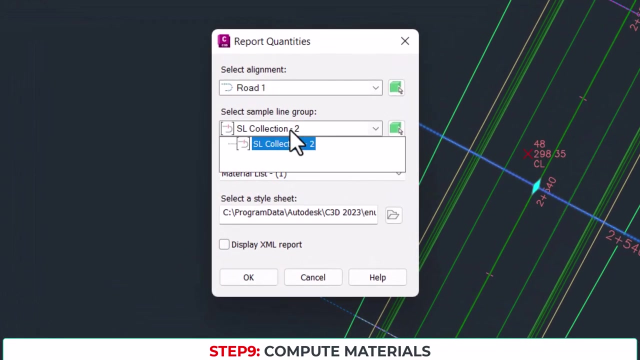 surface automatically. so once you have done that, okay, it will automatically. you create computer materials. great, so allows you to complete it. once it's complete, is great. the materials have been completed. okay, we want to. if you want to view that, you can click generate volume report. so that is one, the sample line, so it's called it, named it automatically for us at. 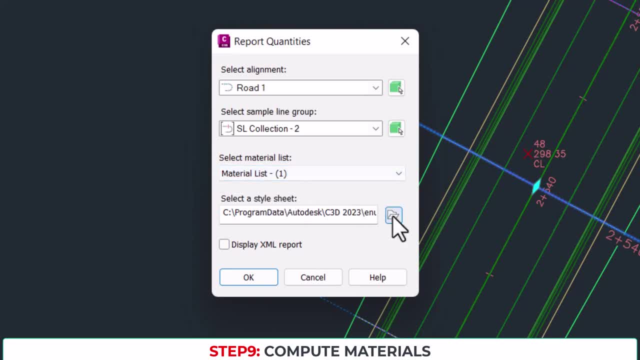 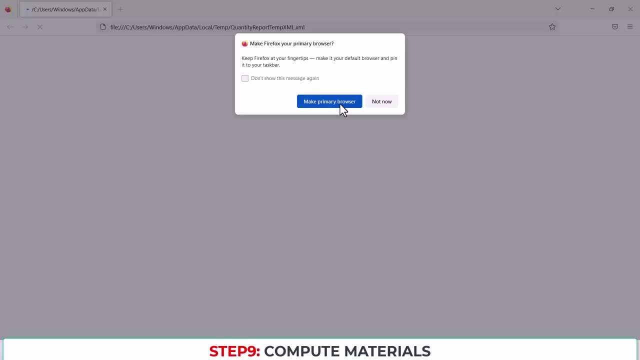 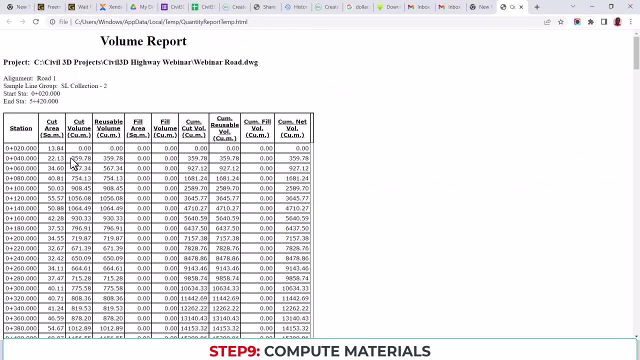 material list one. okay, then we, you can choose the format. it's an ad work, okay, and then you can display the sms report and then press: ok, oh, this, this does not look good. okay, here is it okay. okay, so that is for you can see. have to need zero. zero is not showing because i told you in the sample night creation will not check. 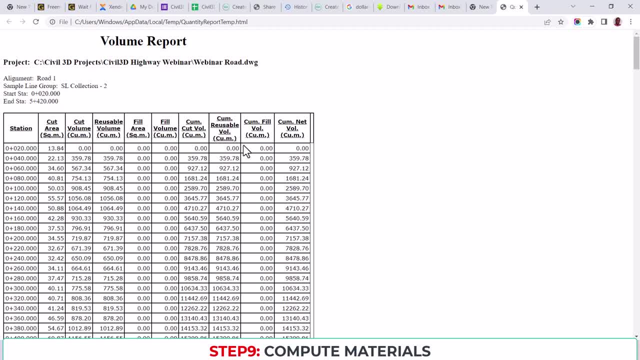 for that one. so, but basically, you can see that we have our cuts and then we have our field. so somewhere here, of this way, we will not have a field until somewhere here. if you so in the end, go to the last point, you will see that we. 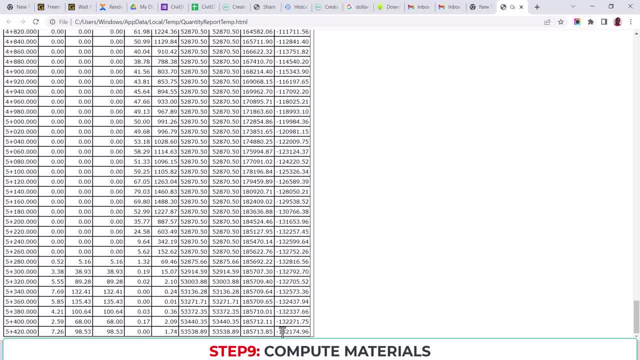 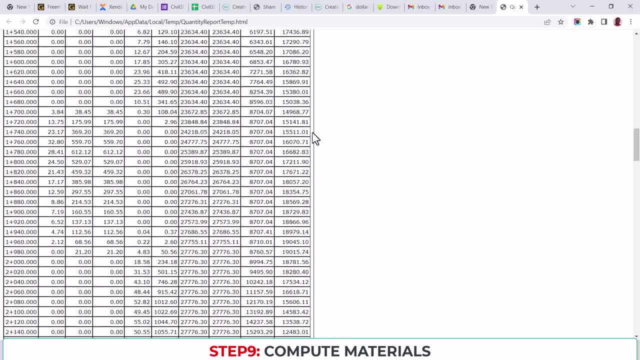 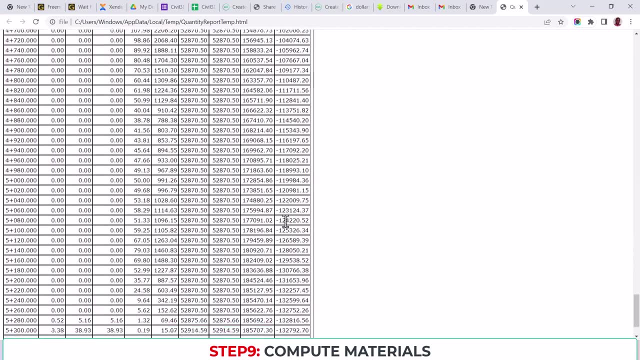 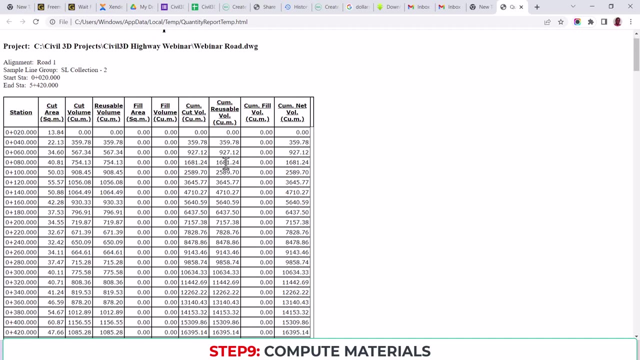 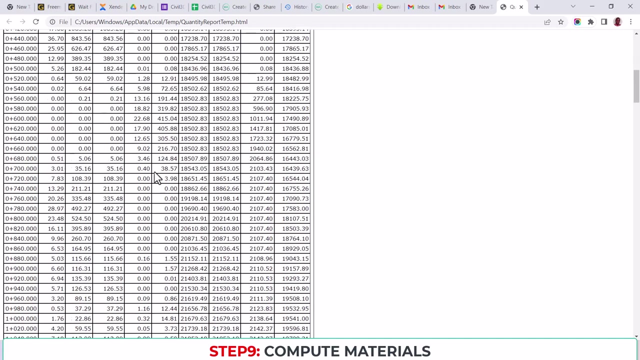 have. we are needing material. so this minus three decent vision means that you need to feel: okay, so that is it. cumulative net volume: okay, because obviously you can see that our materials, this is what material is okay, let's have a lesson. of course this will feel the volume cuts will okay. so cumulative in. 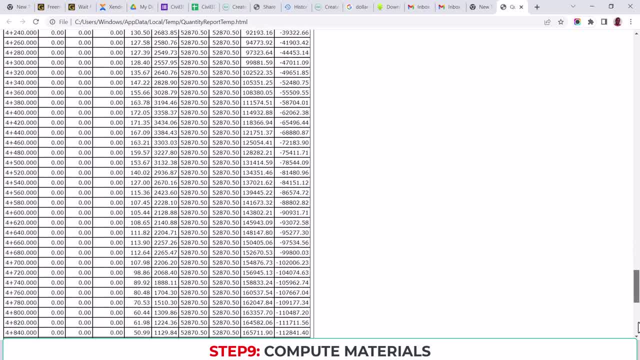 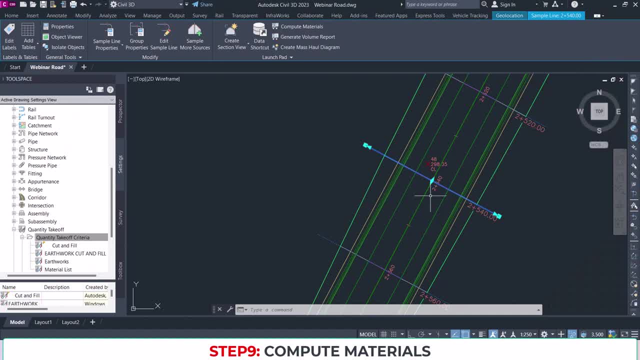 a code. so let me know, just going to explain all this. so let me know, just going to explain all this. so let me know, just going to explain all this. materials, okay, so that is it. you can materials, okay, so that is it. you can materials, okay, so that is it. you can see the report. let's go back right to you. 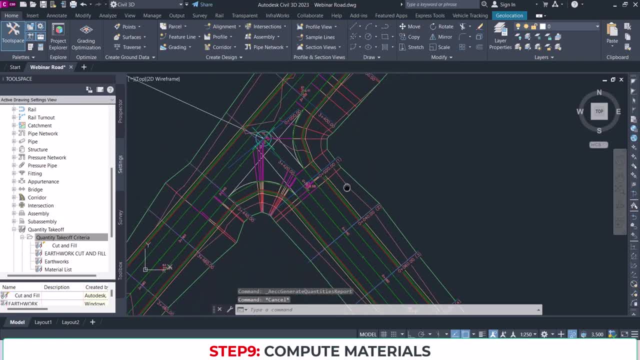 see the report. let's go back right to you. see the report. let's go back right to you. you can do the same thing for two. you can do the same thing for two. you can do the same thing for two. okay, go to me too, and then create compute. 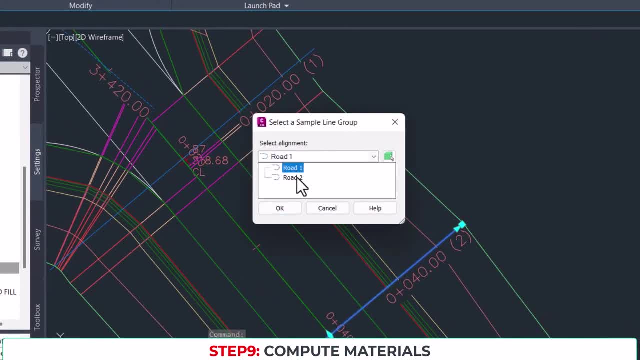 okay, go to me too and then create compute. okay, go to me too and then create compute materials. we have to select the materials. we have to select the materials. we have to select the sample line to okay, and then it's okay. okay, we sample line to okay, and then it's okay, okay we. 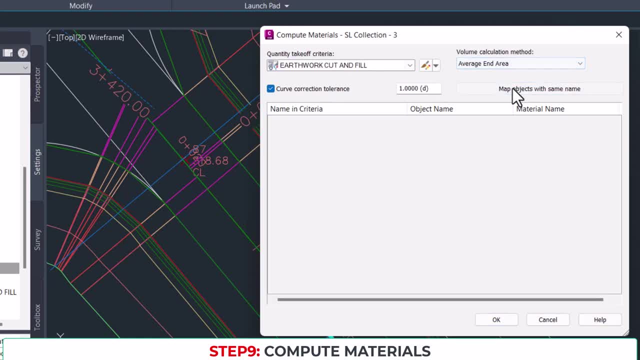 sample line to okay and then it's okay. okay, we now use our quantity takeoff, now use our quantity takeoff, now use our quantity takeoff criteria and then map objects and criteria, and then map objects and criteria and then map objects and then press okay, then press okay. 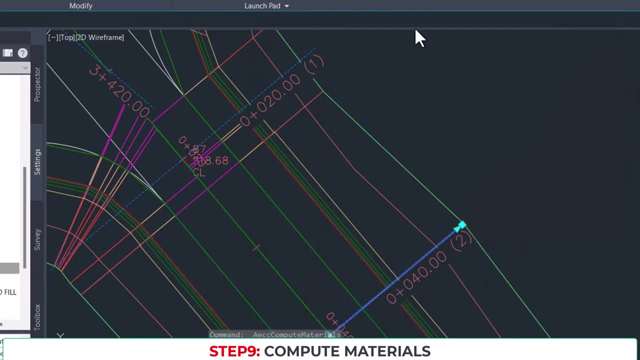 then press: okay, we have created that material, so let's, we have created that material. so let's, we have created that material, so let's generate volume report. generate volume report, generate volume report. okay so, and then you choose through two. okay so, and then you choose through two. 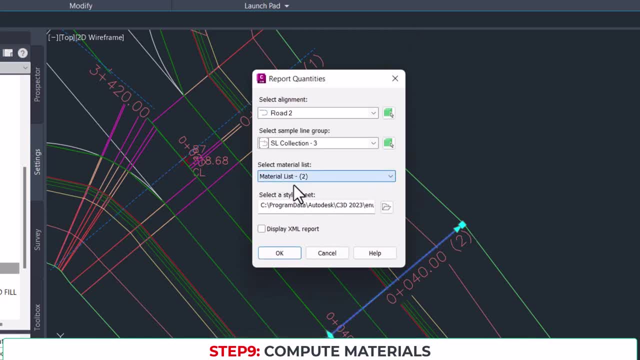 okay so, and then you choose through two, and then it automatically gives you the, and then it automatically gives you the, and then it automatically gives you the sample and collection for that, and then sample and collection for that, and then sample and collection for that, and then material is for that, and then you press. 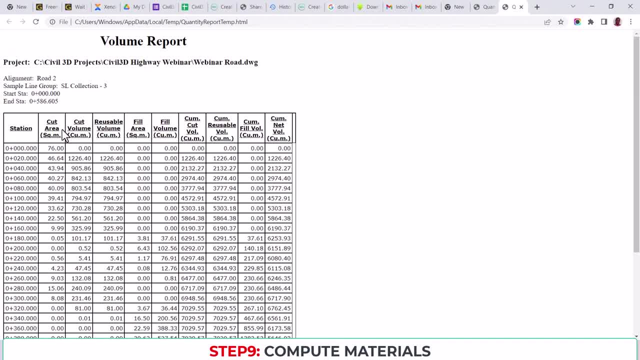 material is for that, and then you press: material is for that, and then you press: okay, okay, okay, okay, this is for okay, this is for okay, this is for road two, road two, road two. right, so you can see special, so we. right so you can see special, so we. 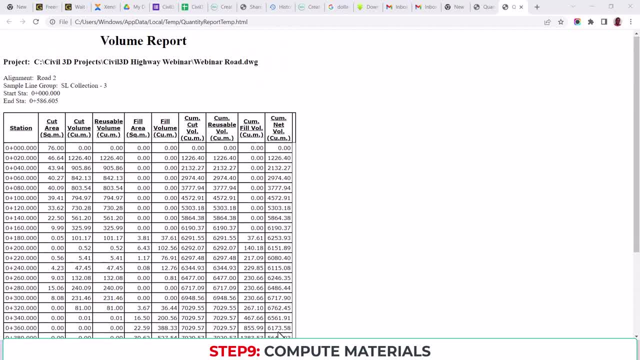 right so you can see special. so we have have have a field volume, a field volume, a field volume cumulative net volume. this is the field cumulative net volume. this is the field cumulative net volume. this is the field volume cumulative field volume. this volume cumulative field volume, this 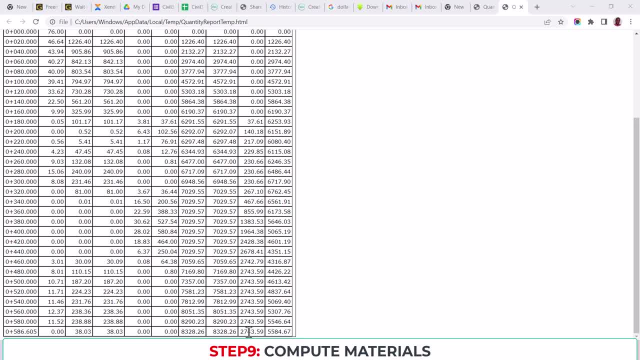 volume, cumulative field volume, this cumulative cut volume, so you can see cumulative cut volume. so you can see cumulative cut volume. so you can see that the? the field is less, and then we that the? the field is less, and then we that the? the field is less, and then we have more cuts. so we are going to be 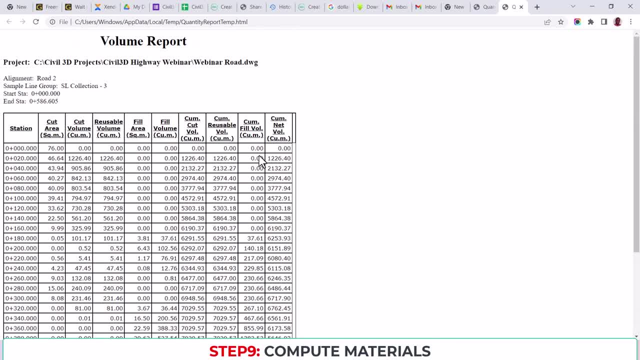 have more cuts. so we are going to be have more cuts, so we are going to be having having having more cuts in this section, more cuts in this section, more cuts in this section of the, of the of the road. so and that is it, let's go out of. 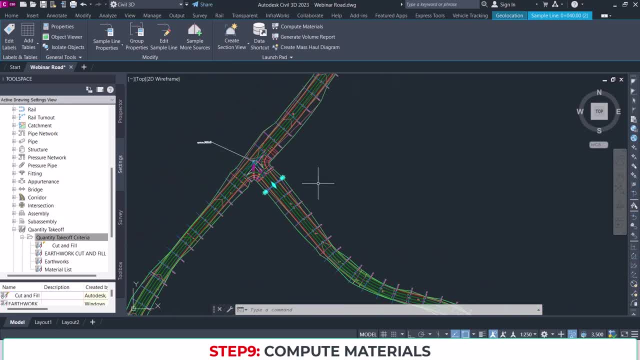 road. so, and that is it, let's go out of road. so, and that is it, let's go out of this. this, this: so great, so we have calculated our we so great, so we have calculated our we so great, so we have calculated our, we have computed our volume. is that the? 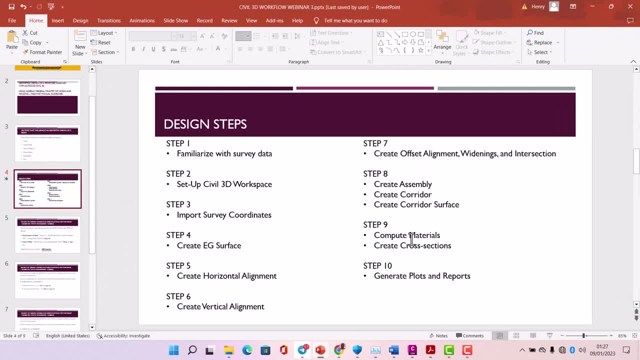 have computed our volume? is that the have computed our volume? is that the last thing? last thing, last thing: yes, we have calculated our cross-section. yes, we have calculated our cross-section. yes, we have calculated our cross-section. and computer material, so we have the. and computer material, so we have the. 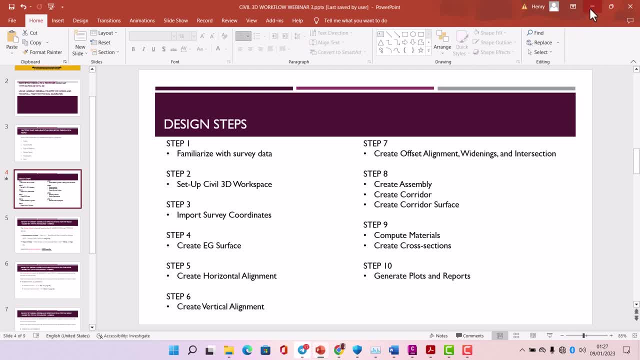 and computer material. so we have the step 10, which is to generate plus, and step 10, which is to generate plus, and step 10, which is to generate plus, and report now in this one, you can now do. report now in this one, you can now do. 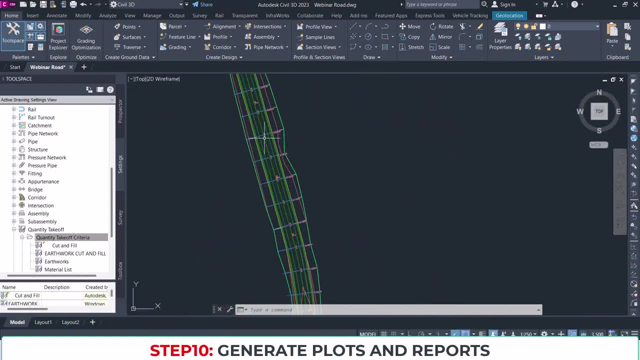 report. now, in this one, you can now do that, that that by yourself, by yourself, by yourself. okay, don't justice to this. so, if you want to, don't justice to this, so if you want to don't justice to this, so if you want to do, do. 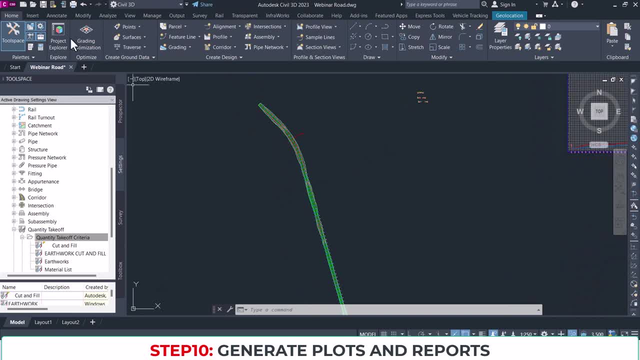 do you know generate blocks. let me just you know generate blocks. let me just you know, generate blocks. let me just quickly run through that, quickly run through that. quickly run through that. you have to create, you have to create, you have to create on the output tab, you have to create. 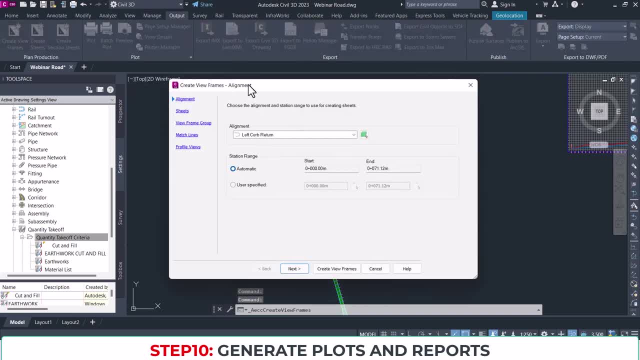 on the output tab, you have to create. on the output tab, you have to create viewing frames, viewing frames, viewing frames. okay, if you are creating viewing frames. okay, if you are creating viewing frames. okay, if you are creating viewing frames, let's do for one, only this time, and then 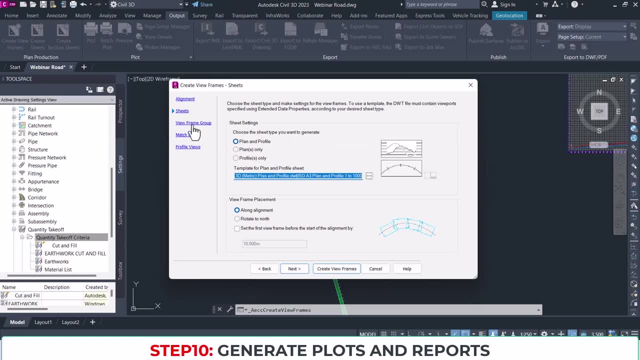 let's do for one, only this time. and then let's do for one only this time, and then go to sheets, go to sheets, go to sheets. let's do plan and profile. okay, let's do. let's do plan and profile. okay, let's do. let's do plan and profile. okay, let's do a view frame group, all these things. 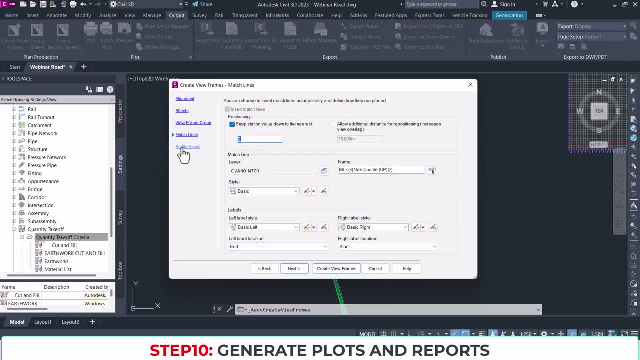 a view frame group, all these things. a view frame group, all these things. let's leave them by default. let's leave them by default. let's leave them by default, okay, and this one's still by default, okay, and this one's still by default, okay, and this one's still by default. profile view: yes, everything, so let's. 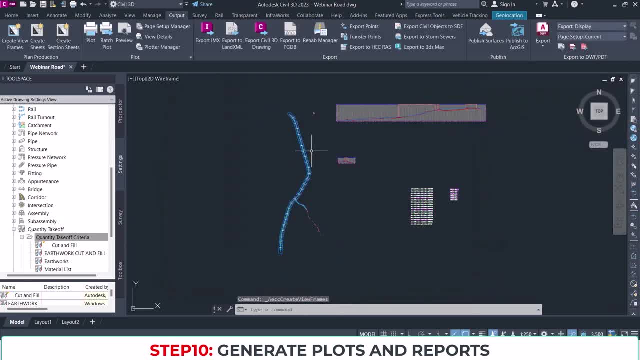 profile view: yes, everything. so let's profile view. yes, everything. so let's create. create. create view frames. great, you can see the view view frames. great, you can see the view view frames. great, you can see the view frames have been created automatically. frames have been created automatically. 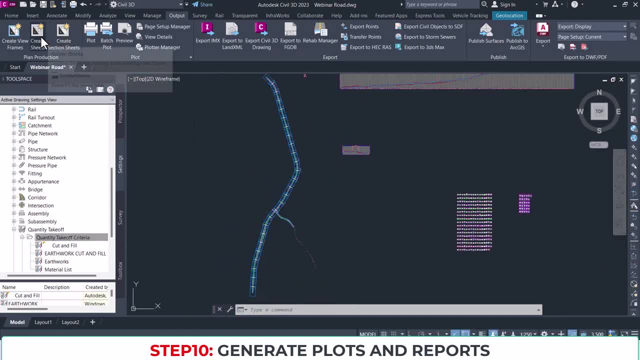 frames have been created automatically. so what will this thing do you have to? so what will this thing do you have to? so what will this thing do you have to? create? create, create view sheets. okay, view sheets, okay, view sheets. okay, create sheets, create sheets, create sheets. so we are going to use the view frame. 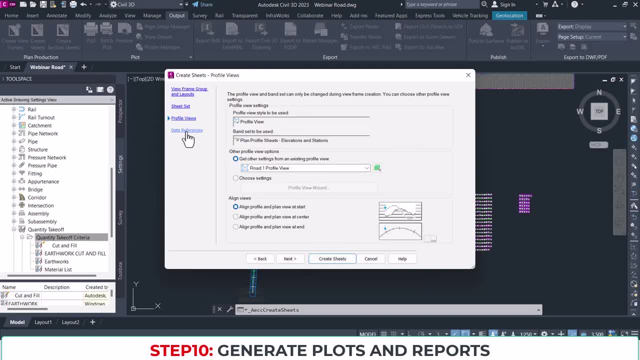 so we are going to use the view frame. so we are going to use the view frame that you just created, that you just created, that you just created- and then create sheets out of that, and then create sheets out of that, and then create sheets out of that. let me create the sheets so that you can. 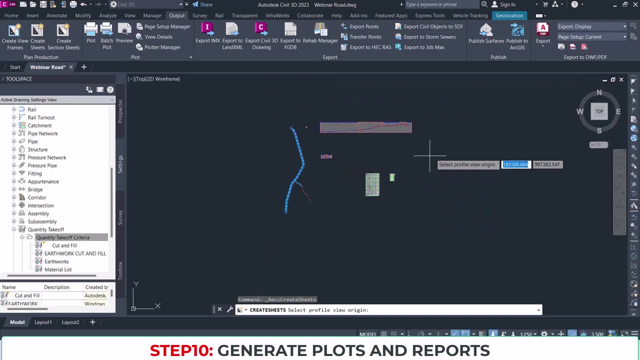 let me create the sheets so that you can. let me create the sheets so that you can see. the drawing has to be saved. so i see the drawing has to be saved. so i see the drawing has to be saved, so i should look for somewhere and click on. 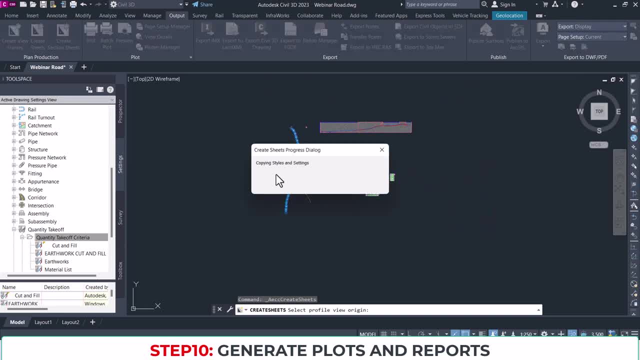 should look for somewhere and click on. should look for somewhere and click on the screen, the screen, the screen. and then it will create the sheets for, and then it will create the sheets for, and then it will create the sheets for me, me, me, automatically. all right, so let's wait for that. 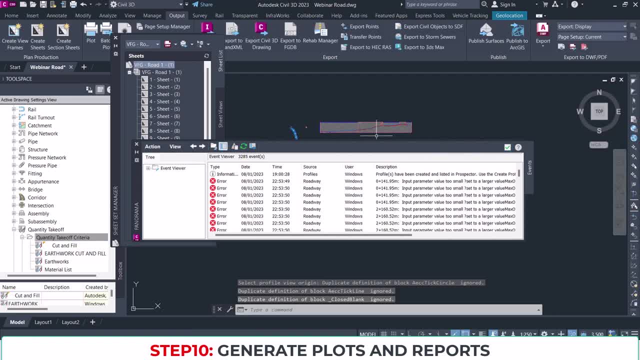 all right, so let's wait for that. all right, so let's wait for that. so great so it updated the sheets as a. so great so it updated the sheets as a. so great so it updated the sheets as a separate drawing. okay, separate drawing, okay. separate drawing. okay so. 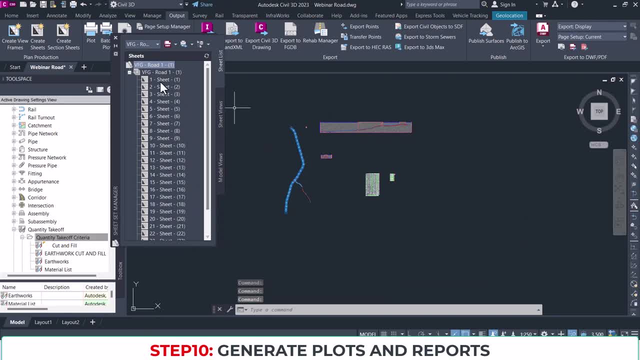 so, so it's saved somewhere in your file. it's saved somewhere in your file. it's saved somewhere in your file, all right. so now, if you click, let's say all right. so now if you click, let's say all right. so now if you click, let's say double click on any of the sheets. 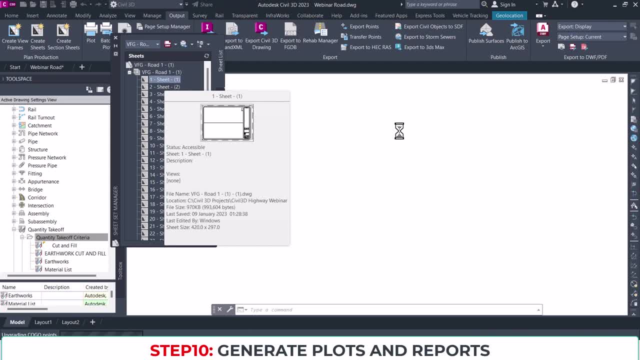 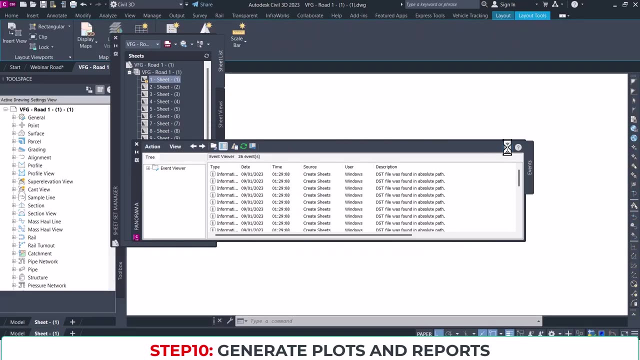 double click on any of the sheets. double click on any of the sheets. okay, okay, okay, you'll see how it looks like. how it looks like. how it looks like. okay, it's opening up. okay, all right, okay, let me check this so you can see. it will automatically bring the plan. 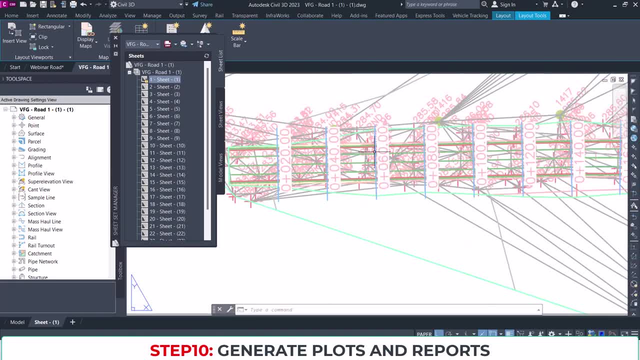 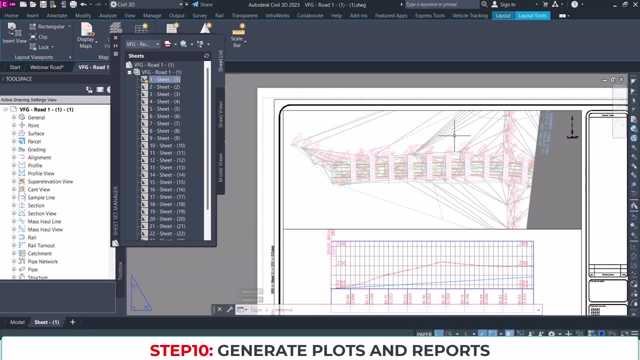 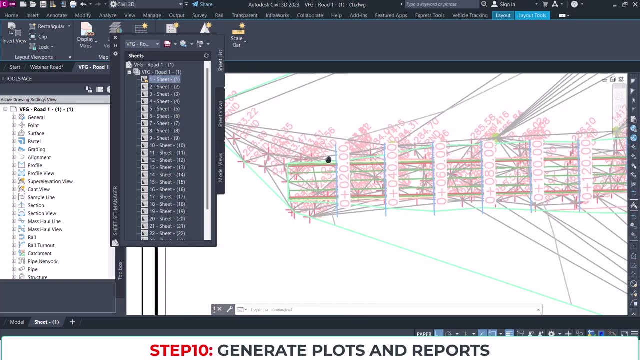 above the profile. so, um sorry, i didn't go through everything, but while i was creating the view sheets i could hide some of the views. okay, like here. if you can see the surface is showing, i will uncheck the surface. okay, in that case, so that my surface will not be showing. i also uncheck my 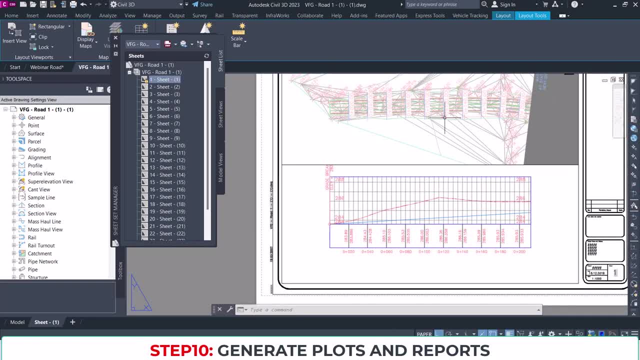 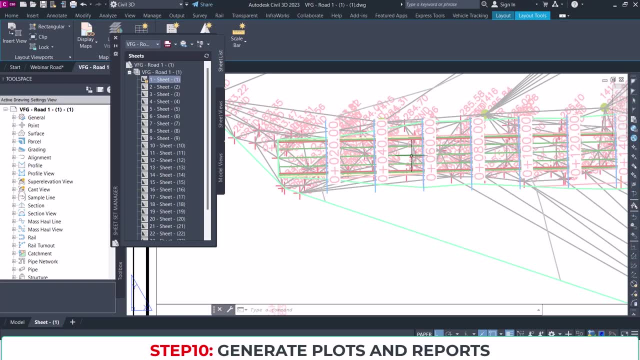 points, so that my points will not be showing. okay, so i'll just be left with only probably the corridor, or even the corridor sometimes i don't want it to show, i just want the center line and the offset alignments to show. it would have been done there. so you know, in this plot, once you have, 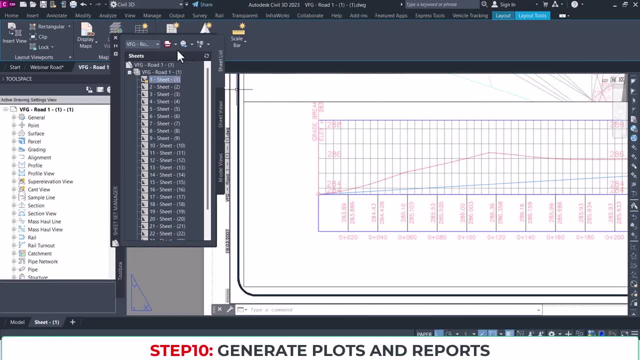 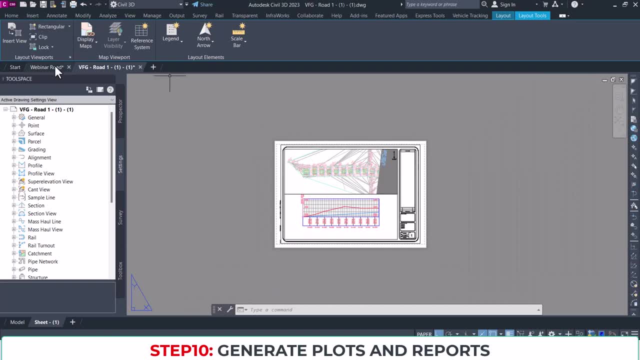 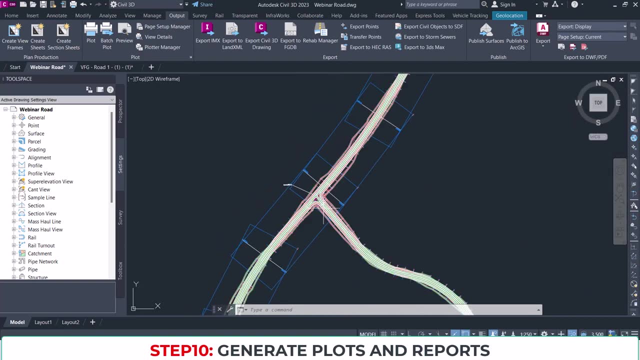 done all these things, you can now print, okay, all right, so that is that is it for this section. okay, so let's just go back to our drawing here. all right, so you could do that for row two as well, but i'll leave you up for that. we can just. 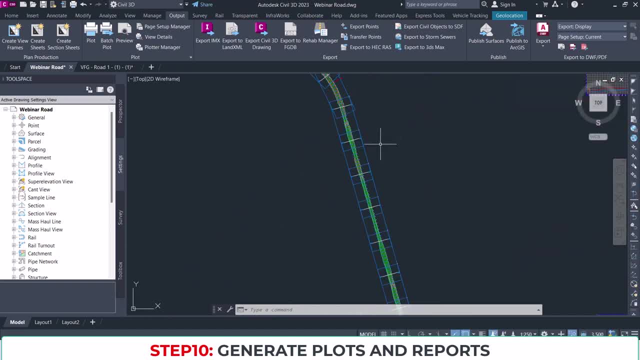 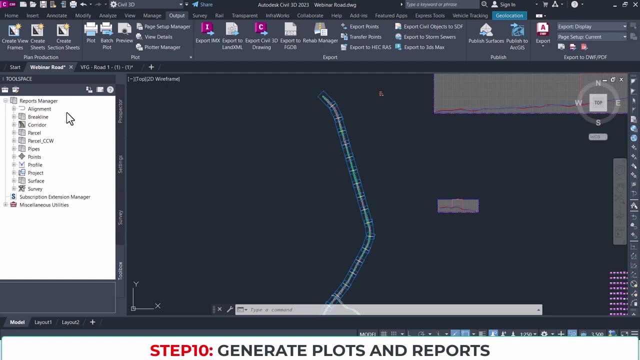 do that for you too, okay. so the next thing we are going to do is to create, uh, to generate, our reports. okay, so when you go to your toolbox, okay, you will find reports manager. check it. then let's go to profiles. all right, this is the one i use. so the one that is the best for you to use is: 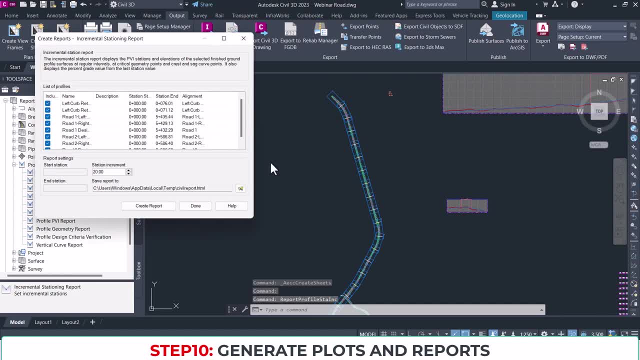 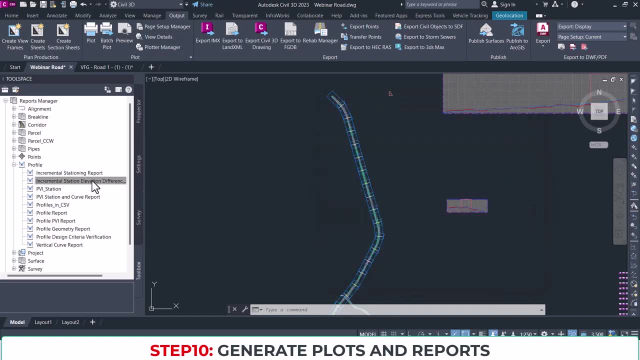 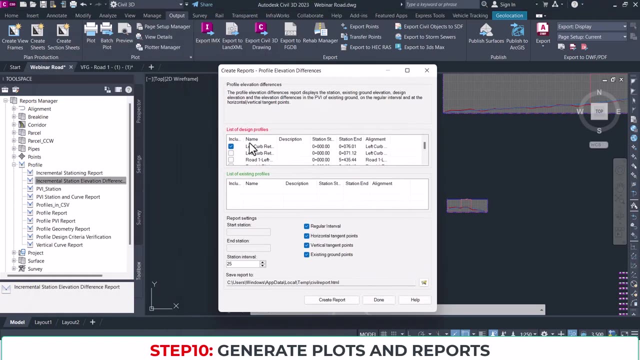 increased mental stationery report. you double click on that, okay, you just it will bring you up. uh, this, okay. sorry, i need incremental station reports, difference, all right, great, this is the. this is the. this is the one i would use. okay, so which? let's do forward one, okay. 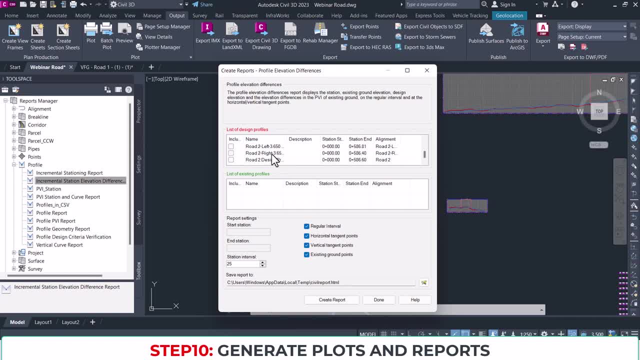 so which profile? okay, we need one design profile. okay, that's what we'll check. okay, and then we need also the eg surface, all right. so we need it as an interval of 20 meters? okay, 20 meters, all right. so, and then let's just use the regular interval, let's remove. 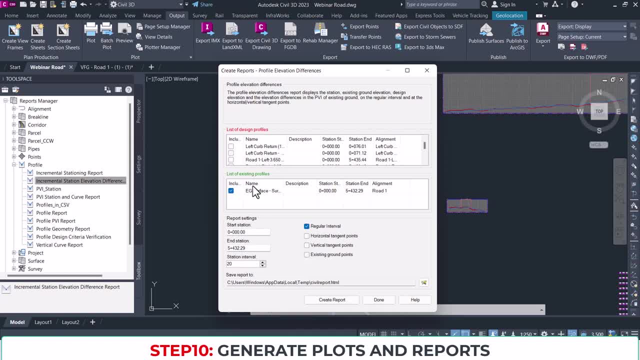 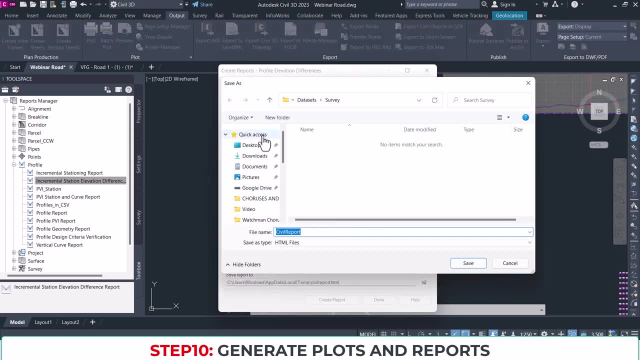 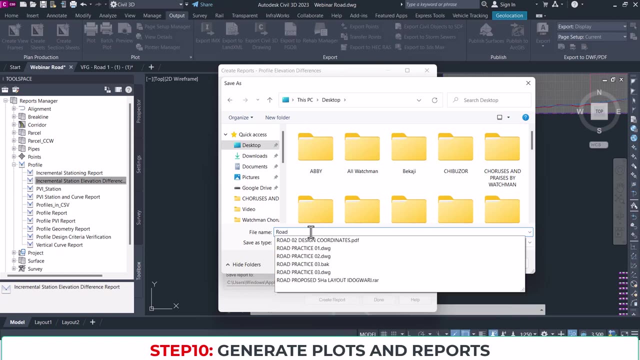 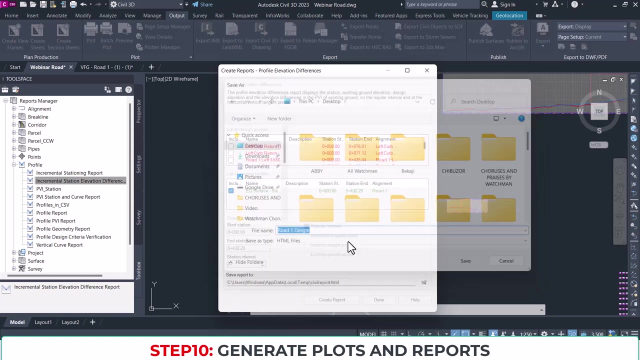 uncheck all of this, okay. and then once we have done that, we press, uh, we find we choose where we want to save it. okay, uh, let's go to desktop. let's save it as uh road one, uh details. okay, we're going cut and fill. oh, let's call it one design, all right. so let's say save and then let's create the report. 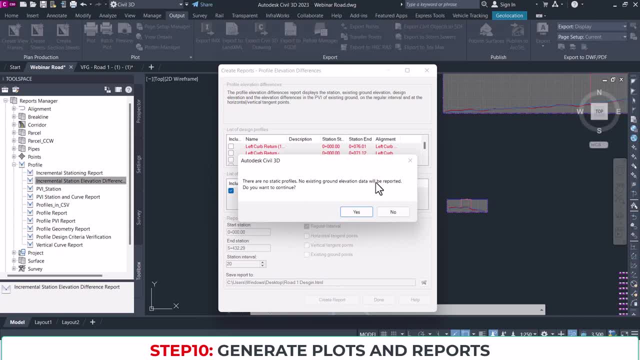 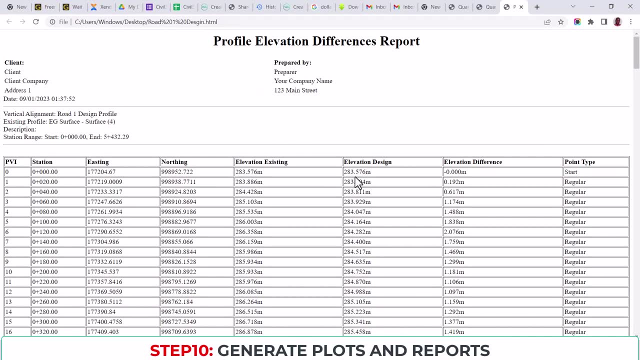 okay, no existing ground elevation. that i've wrote it. we're going to start purpose. okay, let's continue. yes, okay, so yep, as you can see, this is showing you the eastern, the noddings, the elevation for existing and then the elevation for design. all right, this is the elevation difference. 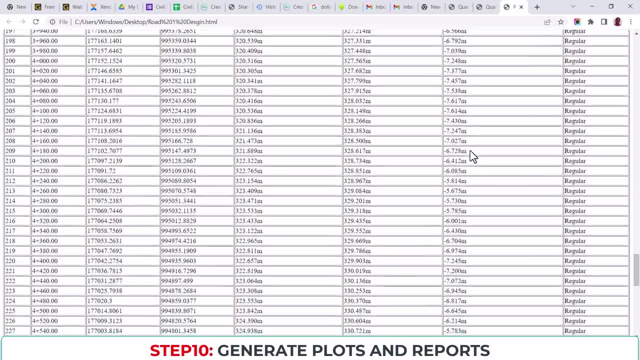 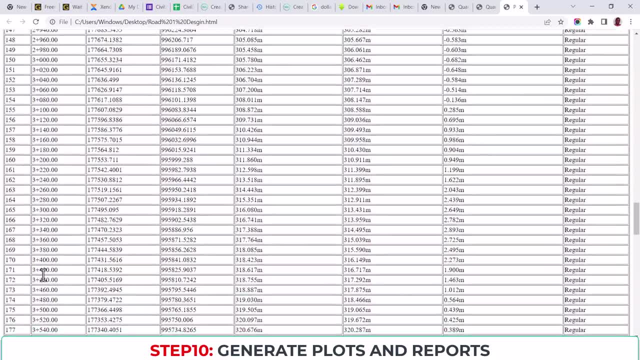 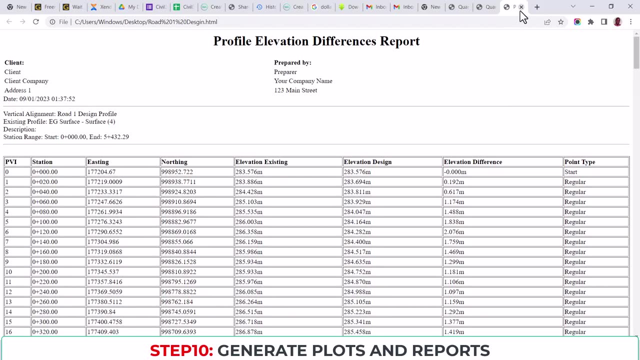 automatically showing you, okay, for every, uh, all the changes from the channel zero, zero, down up to the last change. so this is what you need. you can export this as excel, okay, and then this is exactly what you're going to give the surveyors. they will input these coordinates and these coordinates. they will input this. 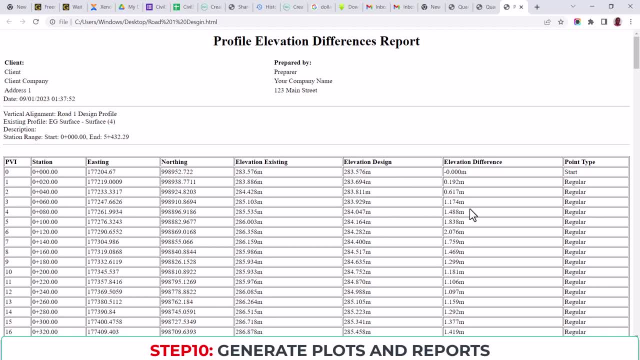 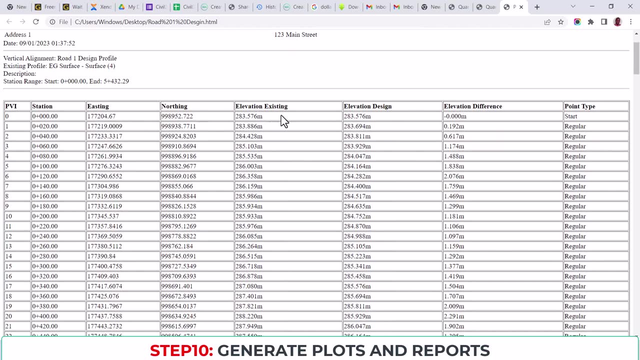 elevation design. okay, this difference is just to guide them on uh knowing, okay, you need to um the. the difference is: okay, zero and zero meters below. so it's exactly. we're matching the existing in this case. so both here, the elevation, we are going 19 cm higher than the existing ground. 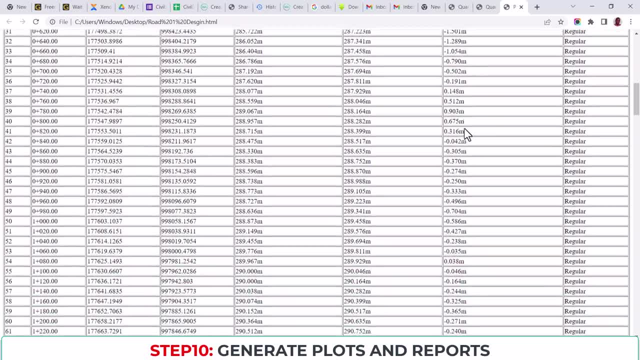 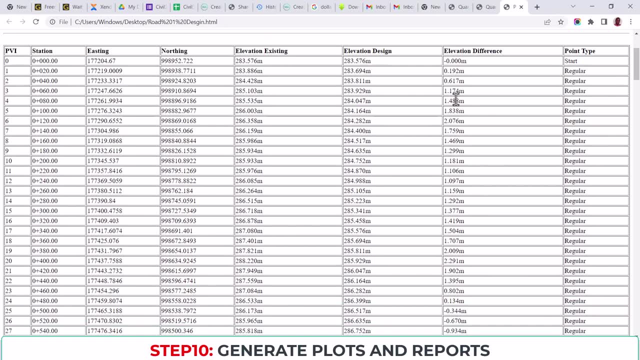 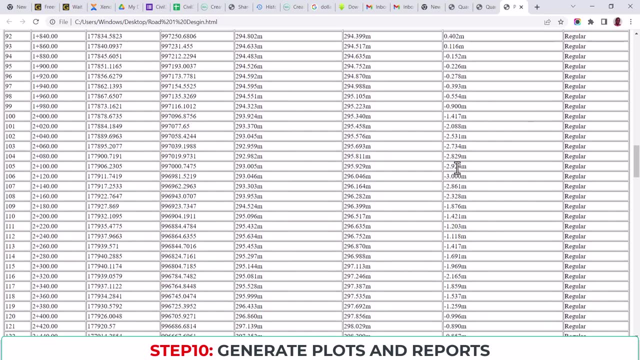 level. so with this you can even know how high or low you're going with your profile, and once you just look at it, you scroll through. so here you can see it is a field. here's the field, one meter in one meter high. okay, that's not bad, two meters, even high. so, but you don't want to go too high, let's. 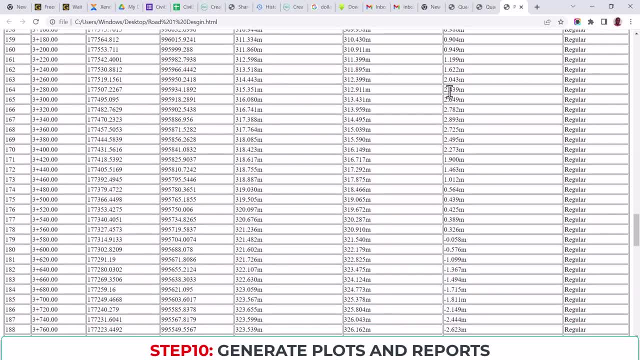 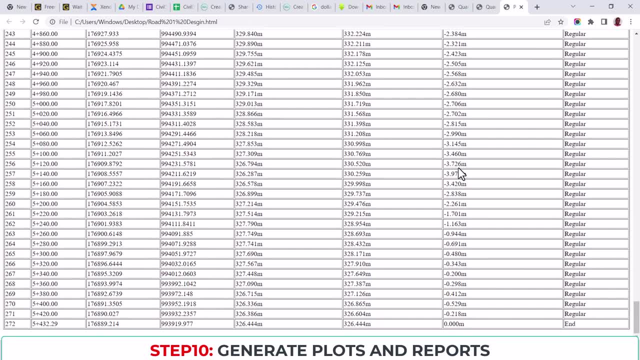 say like four meters high. i'm feeling so obviously i cannot see something like that. oh, i'm having like seven meters in cut. well, you know, remember, i've not designed the profile, you know, accurately like that, mistakenly, just like i did with my alignment, so you can do that. 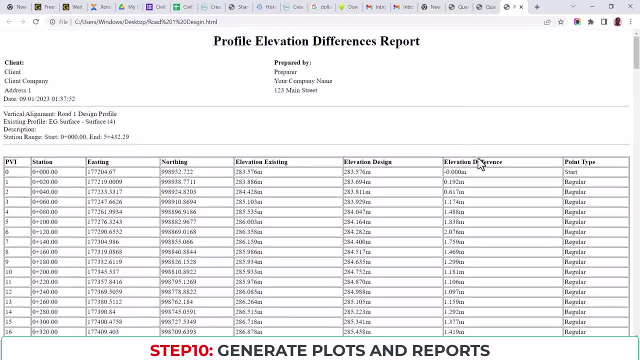 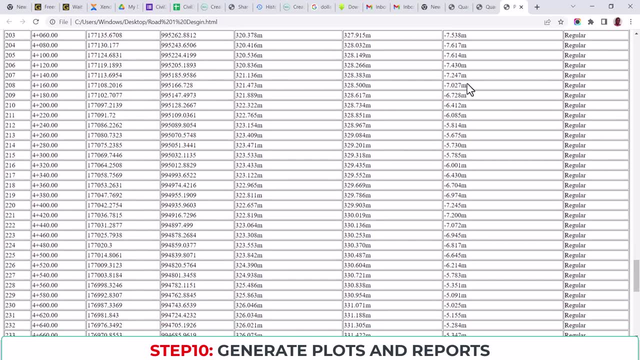 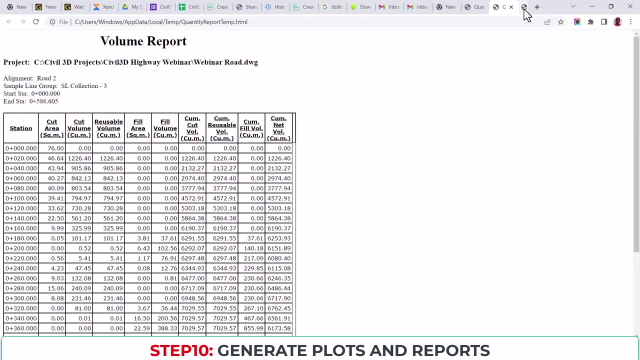 on your own, because if you're doing a live design, you have to do that properly, okay, but of course that does not mean that there are no cases where you can cut seven meters or five meters. okay, it's depending on what is available, okay, so that is what we uh. all right, that's all for the class. so 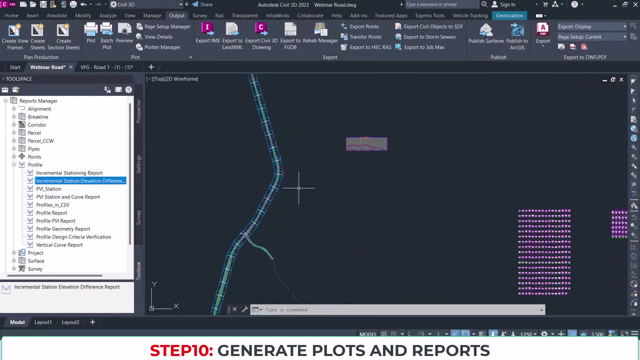 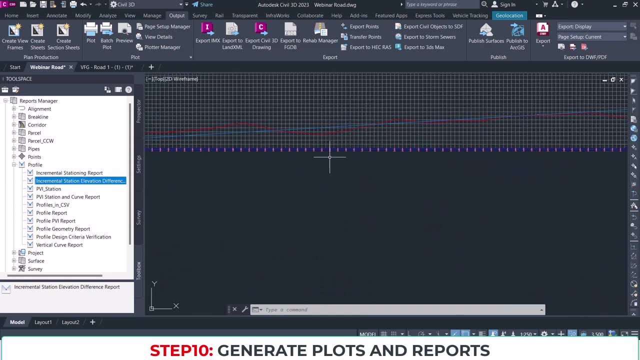 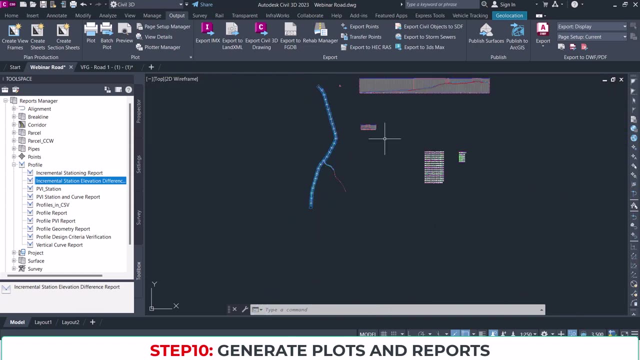 thank you very much for the opportunity. okay, to take you through all of these um things. there are so many things to just go through. okay, but just alignment, we can spend a lot of time on it. so, but this, i've just breezed through the whole design and showing you areas you can concentrate on making the design better for. 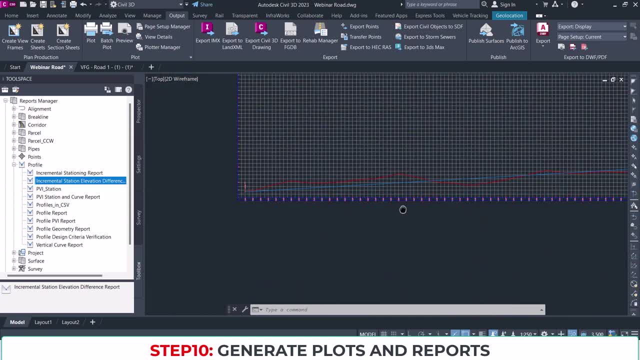 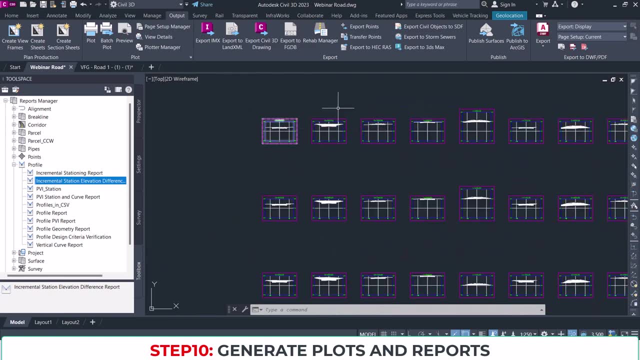 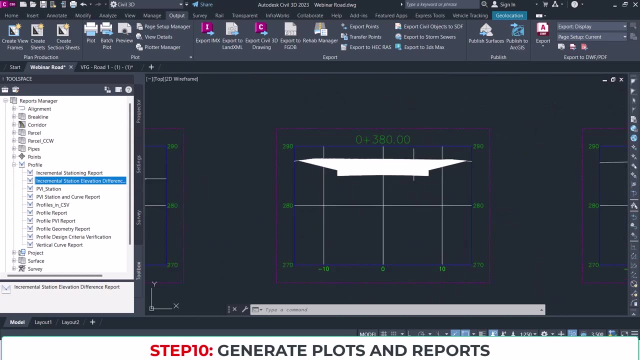 instance, your views and styles. okay, like all these views, they're not so nice, but you can create yours. you can always adjust how they look. and here, in creating the section views, okay, um, you can see, here is shaded. it's actually supposed to show right or green, depending on color view. but you can always do that and tell me your things are obtainable. 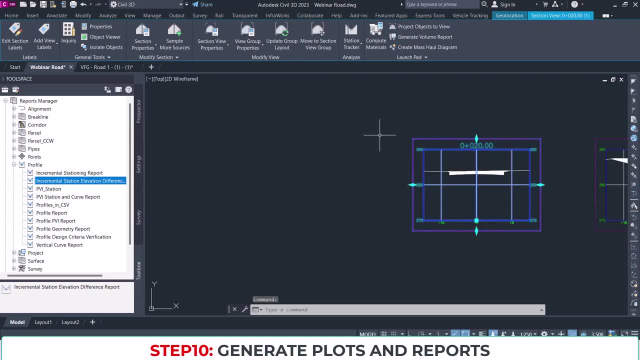 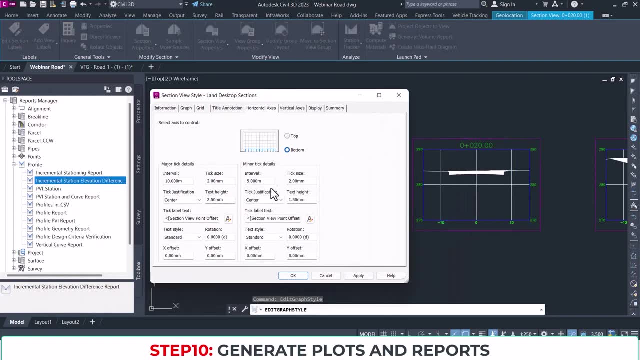 all you need to do is just click on anything on any of the view. okay, play around with it, right click and then go to edit view styles. so here you can play a lot with repair. play with all of this, okay, to make this view look better. okay, once you are done, you cannot plot it, okay. 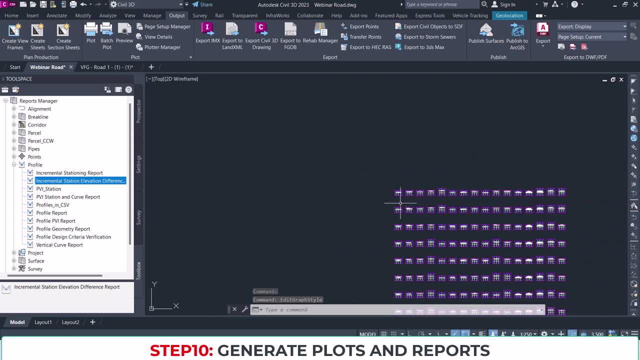 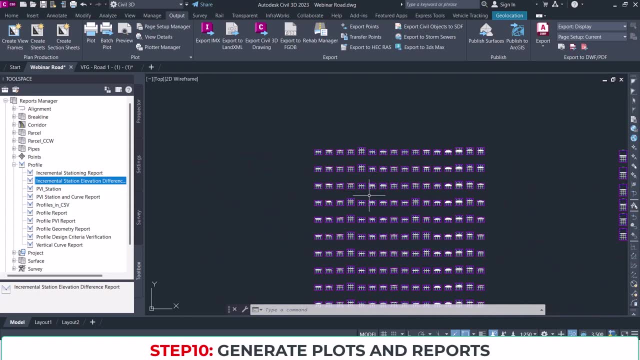 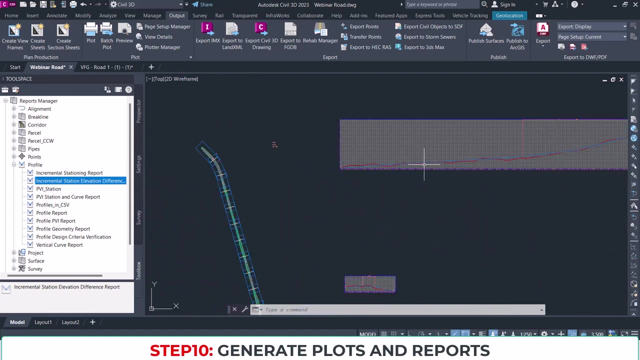 remember, we just do draft. okay, if we did it in production style, it will automatically add a touch block here for us and then, when we are creating the sheets, it will automatically lift those sheets for us. so, yeah, so we couldn't go through all that. this is the much we could take for the 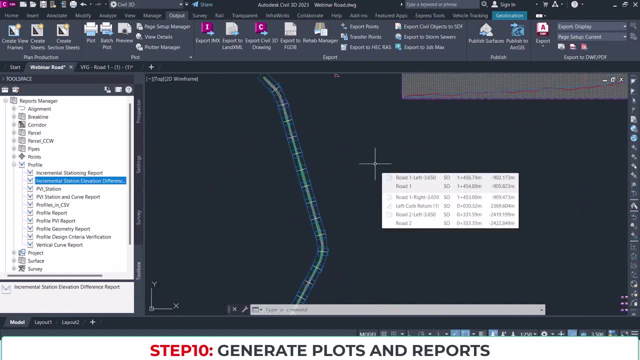 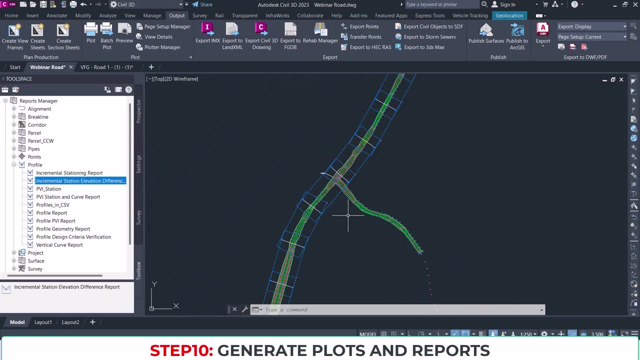 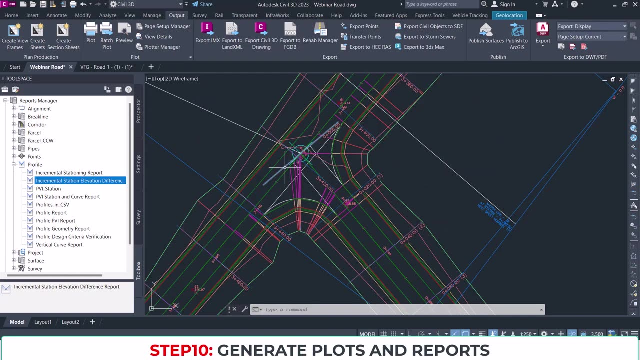 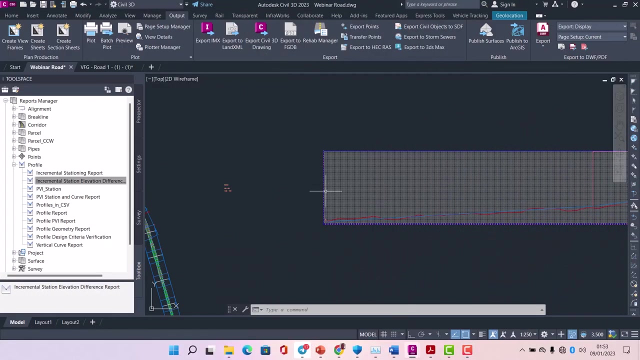 class. thank you very, very much for joining the class. i can't wait to see your designs. if you happen to, you know, do it yourself and send it to me. i'll be much happy to review it and then give you any comments that could help you develop yourself. okay, so all right, like. 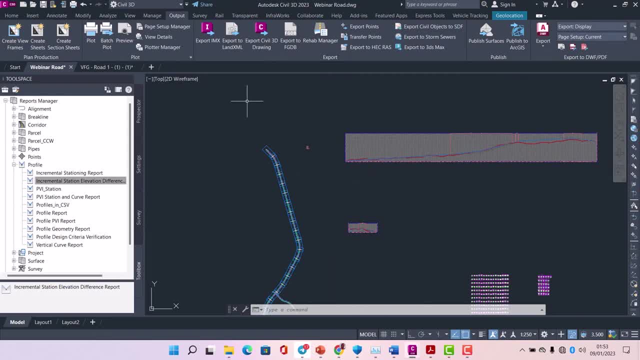 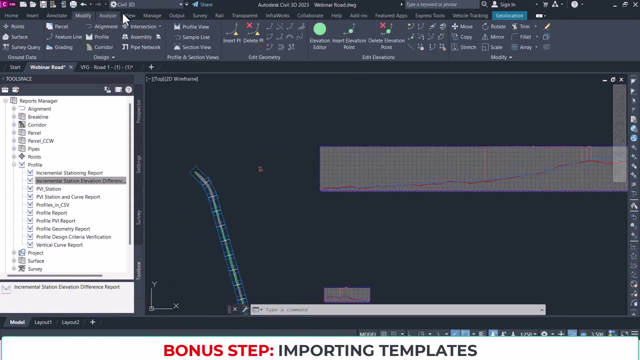 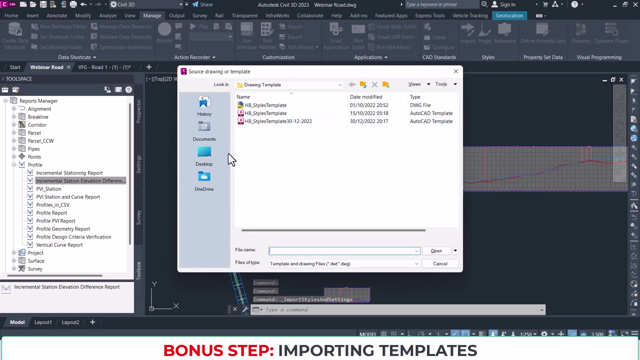 I mentioned, I'll be importing my templates so that you can see how I adjusted all these views to look fine. so let me go to you know, manage, I'm going to import my templates. okay, I have to save the drawing to do that, right? so once I do that, I click import. okay, I have my templates. no, this is not the one. 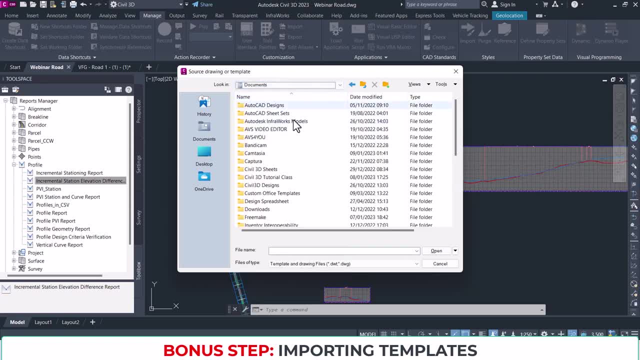 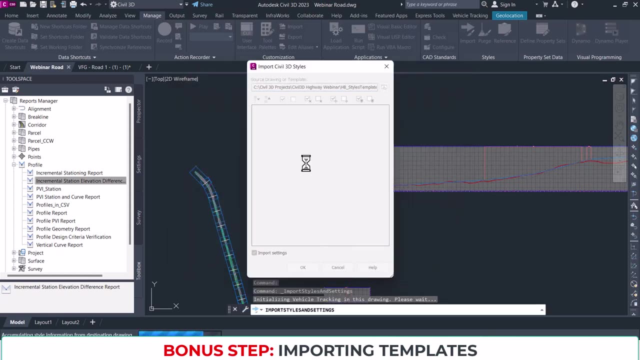 actually let me go to my documents. no, not documents. my local digs: okay, I have a civil 3d project. my templates- okay, all right, so let me open that up while it's opening. right, we're learning to. yeah, all the settings, all right. so there is it. there's, it's my 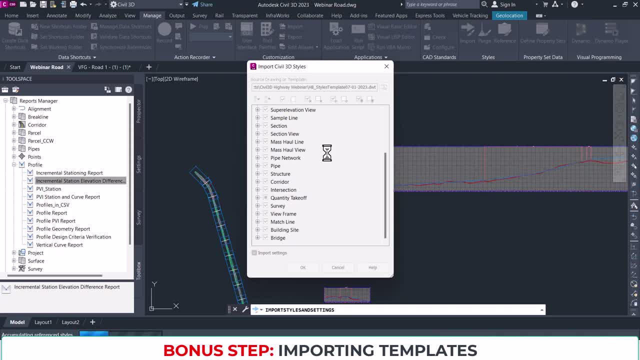 profile my. you know templates looting, okay. okay, template is simply all the design that I have adjusted, so I'll just see those as a template. okay, all right, so, and then I'll import it into any Quran. so that's if we look good, so if you look. 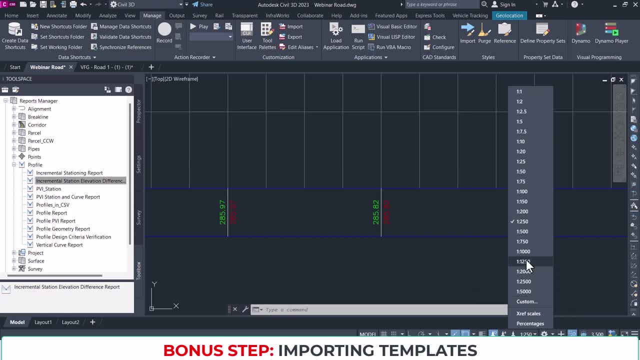 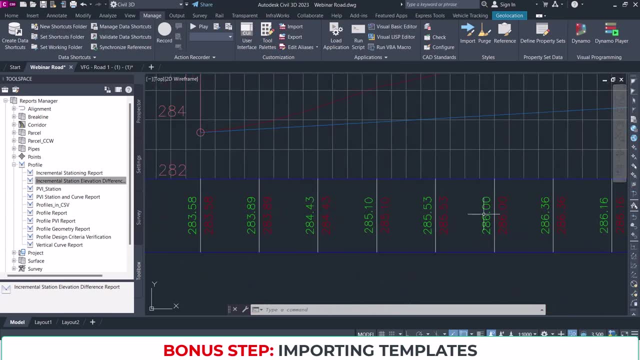 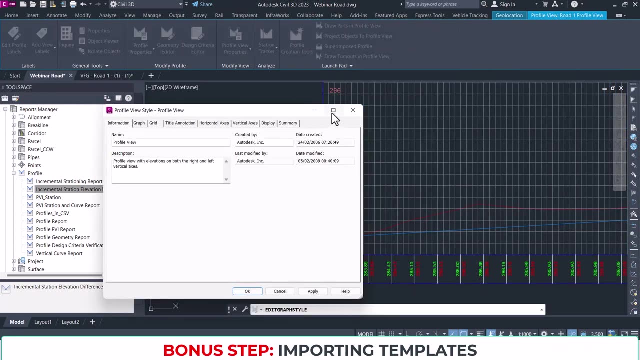 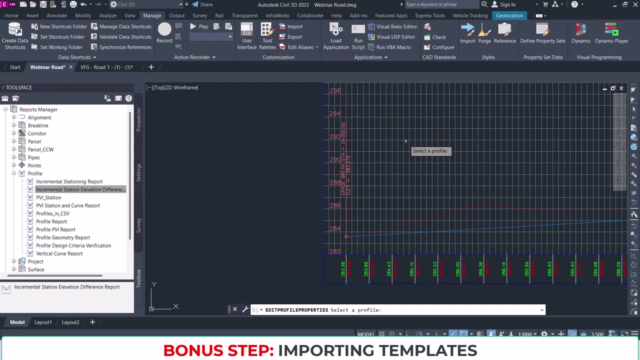 already. then we've done this to 1 is to 1000. you can see that my templates. okay, you know a deep profile view style, okay, okay, let me. let me go to profile view properties. profile view properties. oh, my god, sorry, the profile view properties. so i'm going to call it. 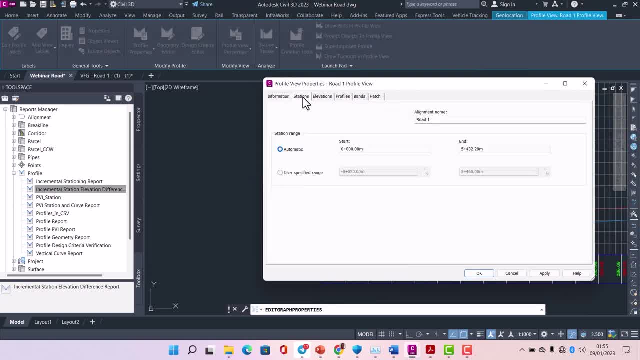 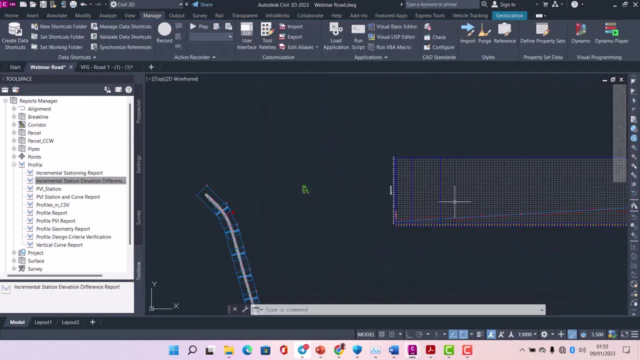 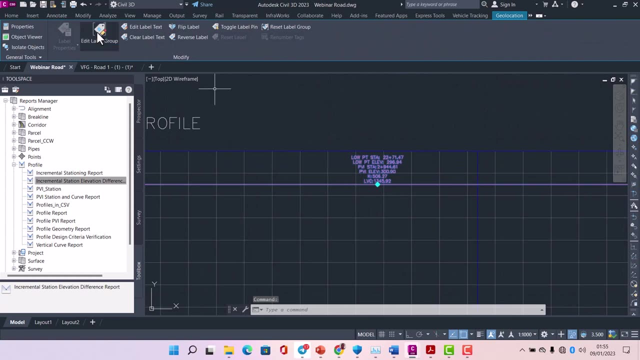 my template. my template is this: in five meters interval. okay, i usually walk on to five meters intervals, that's why we have it here, so let me press ok. wow, you can see. it looks finer right now. all right, so even for this, i have a template for this, so i can go to edit label group. i can import. 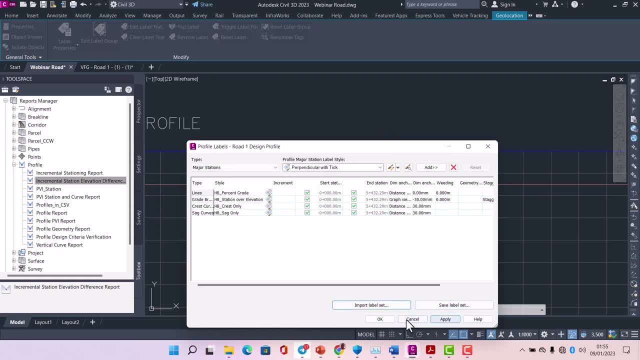 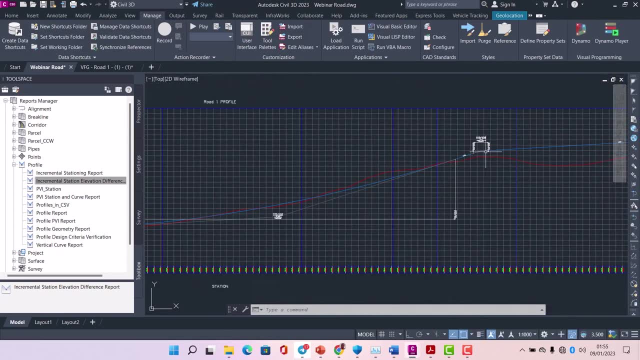 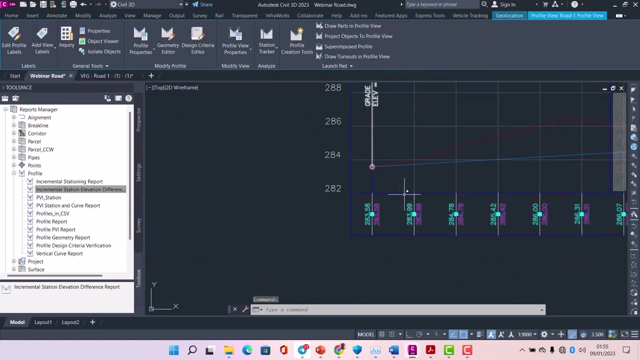 my level set. i have it on schedule reset. okay, i can press ok. so if you look at it, it's white and color, showing you the radius of the curve and showing you everything. so it's looking. it's looking better already. so even the band set styles. okay, i have my edit band style okay. 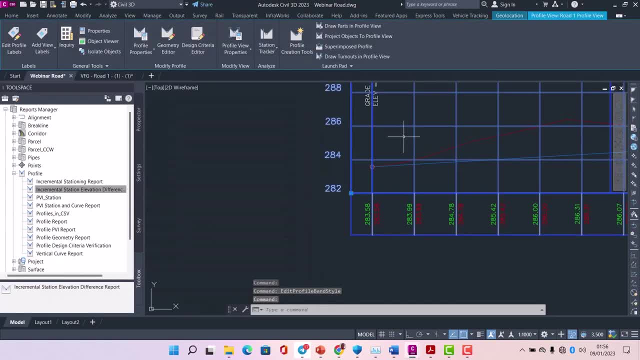 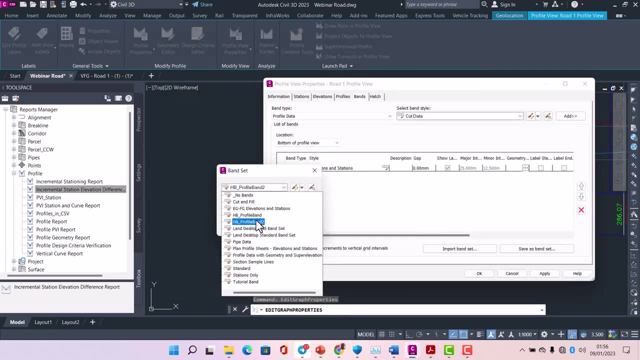 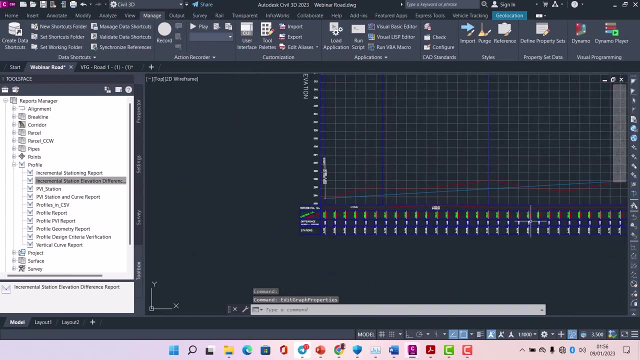 all right, so all, rather, let me go to the profile view properties. so, when we go to bands, i have my own band styles. i call it hpe band. okay, so let me press. ok, great, you can see my band styles. okay, it's showing you a very robust view. so, and as you can see, everything here is zero showing. 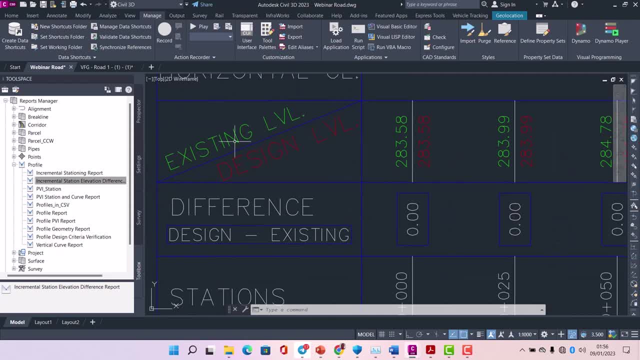 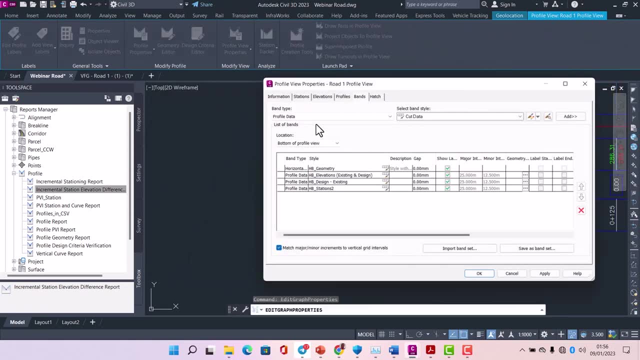 the difference here is showing zero, okay, between the existing and design. it's because i have not adjusted it, so let me go to the band styles again. okay, when i go to the band styles, i have to select the profile 1 to be the eg surface and then the profile 2 to be the design. 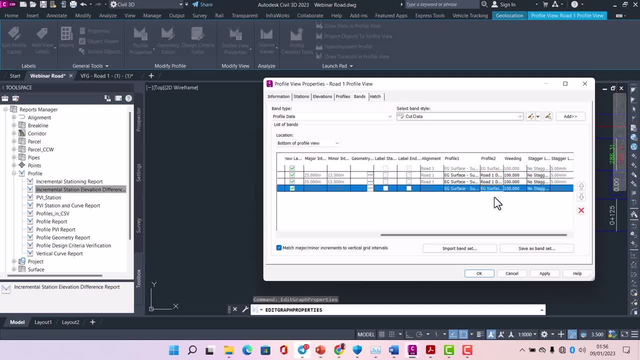 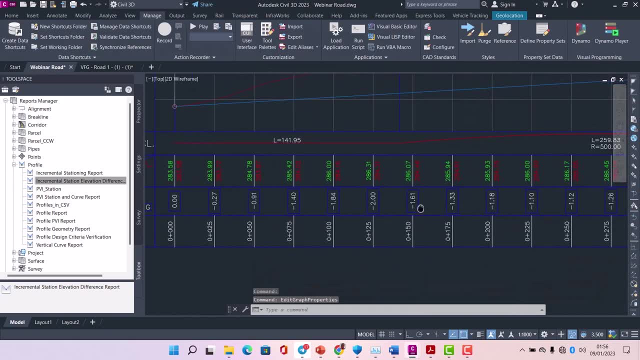 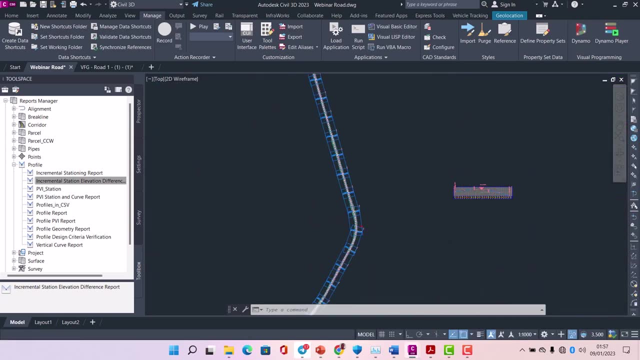 i'll choose all the profile 2 to be the design okay, and then i'll press ok so you see it's updated. so showing you all the cuts and fill that is available here. all right, i can do the same for you know, section views and of course i'll put the manually add that here i'm going to manually add. 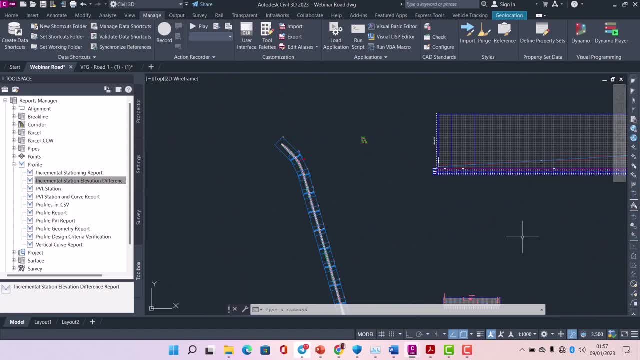 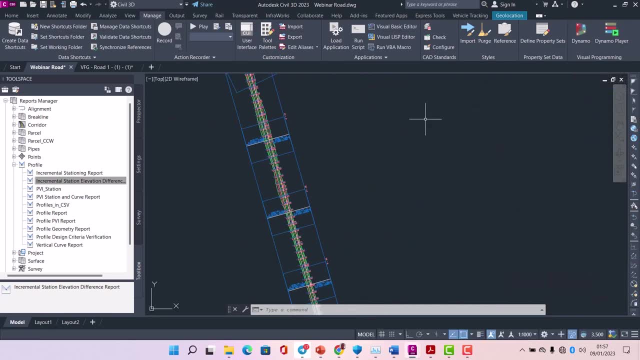 that? because i did. i did not put that when i was creating. you know, i'm just importing the styles now. well, usually before i started drawing, i import my styles and i work with it. i don't, i don't want to just bore you with that. okay, it's just something. i'm just showing the capacity of what. 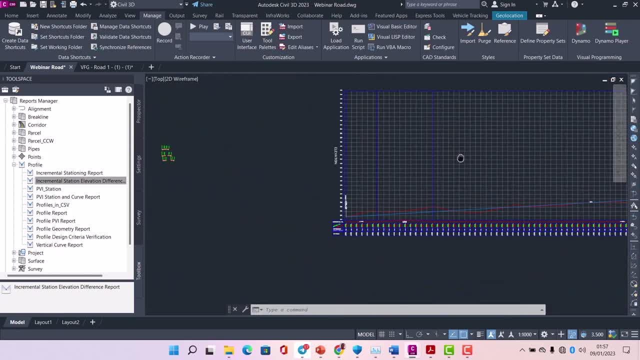 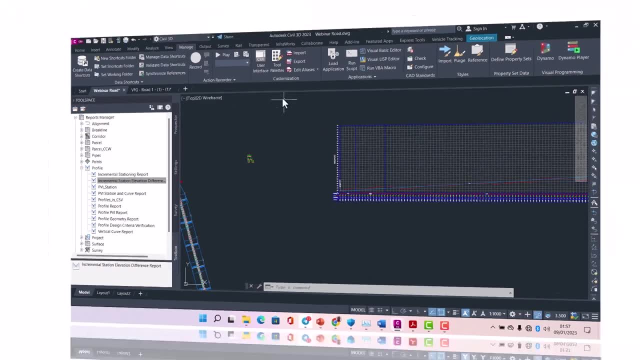 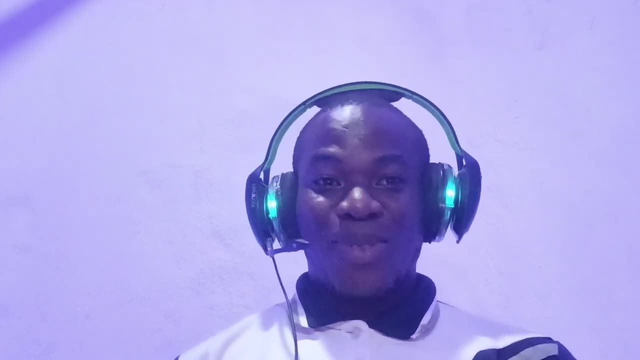 you can do. it was no, it cannot look as ugly as it was originally. all right, so that is it. that is it for now. all right, guys, thank you for joining the webinar. yeah, it was supposed to be live, but, uh, this is the recording, you know, to augment for the inconvenient experience that we had earlier. 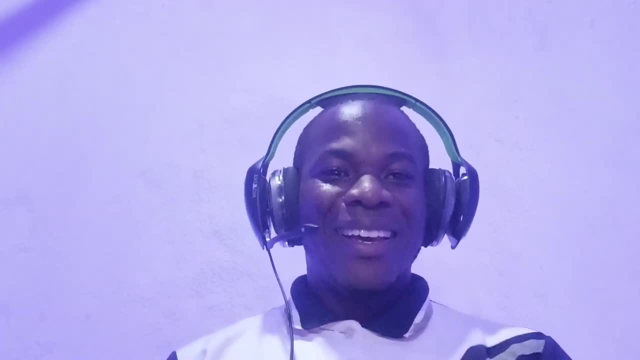 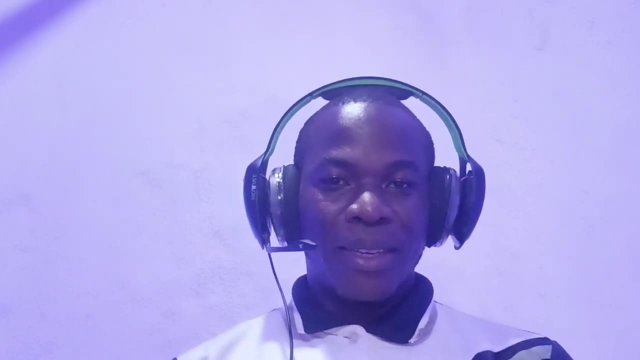 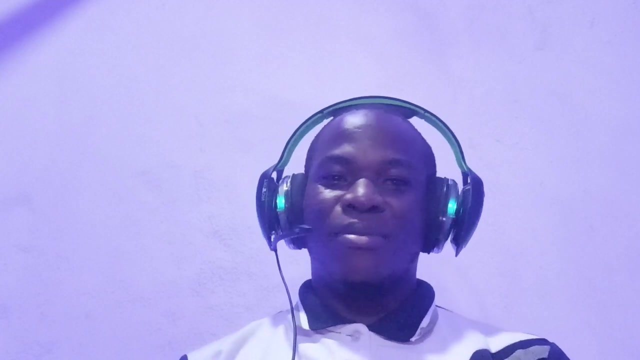 so that was it. so it was quite a roller coaster and there are so many things i i could have you know, to show you, but, um, time will not suffice. okay, to make it. i try to make it as concise as possible, but you have learned a lot, i believe. even with this, you can, you know, get the ground. 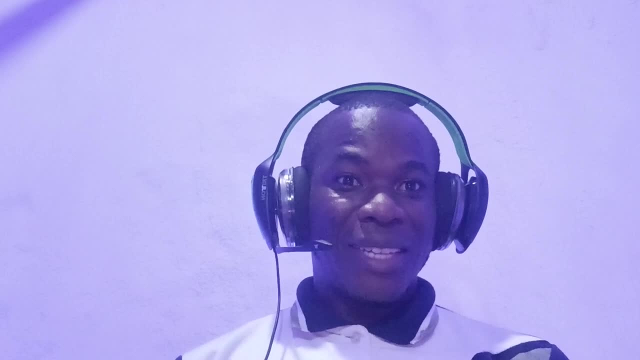 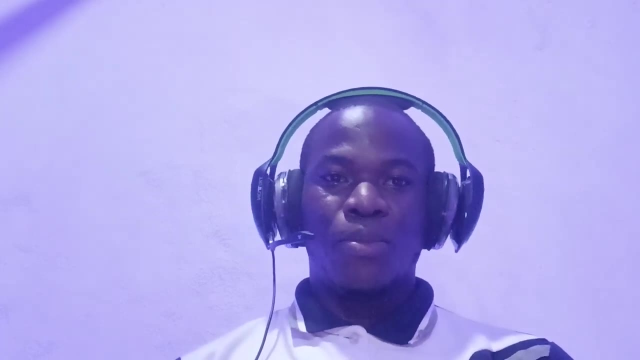 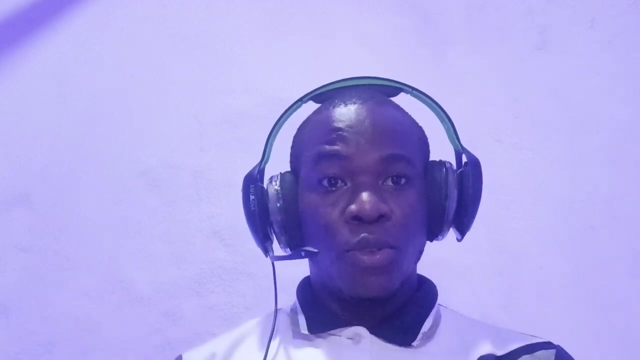 running. if you're already in design, i believe you've added, and if you're just starting, this is enough for you to just uh progress. so i would like to see my future class when i get the chance to put some things uh on it, all right. so there's uh like, for instance: uh i, i did not put culverts. 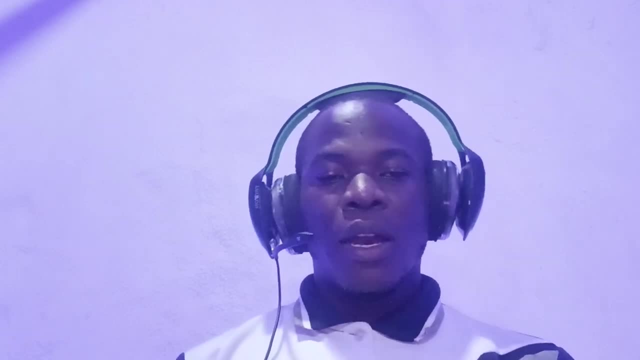 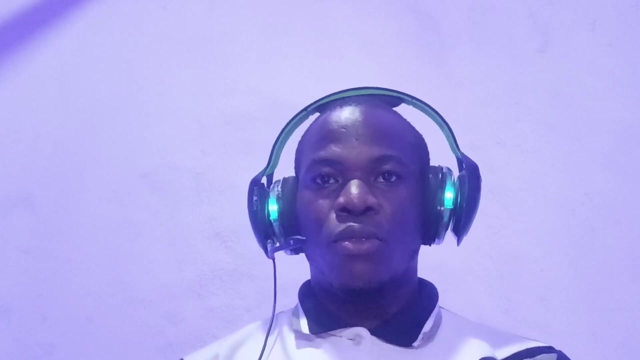 no, but you see, those places that i have streams crossing, and also the low points on my profile, those are the places i put bus curves, okay. so, um, of course, i didn't mention that in this class. okay, i mean to cover in this class, but it's something you, you, you know is part of road design.